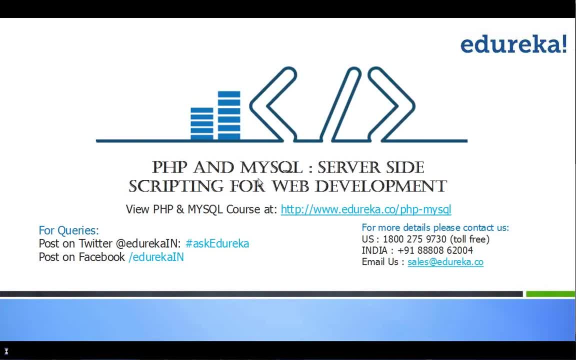 for this sessions- online sessions- and I've worked with various domains and also worked in various countries and, moreover, apart from web development, I'm into client-side development as well. So today I'll be taking a session of PHP and MySQL, where I will be letting people 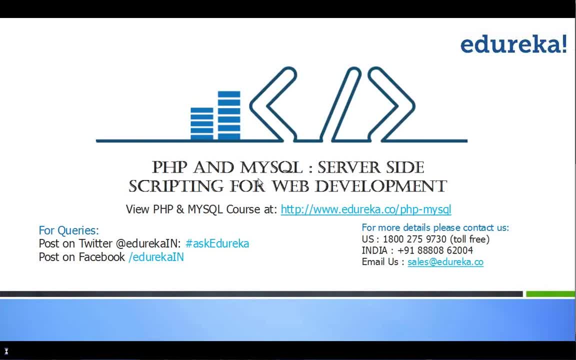 know that, how PHP and MySQL dominates the web development model And how easy it is and how you can familiar with PHP. So the topic for our session would be PHP and MySQL server-side scripting for web development. So first of all, you people need to understand what server-side means. Basically, two kind of development is there. 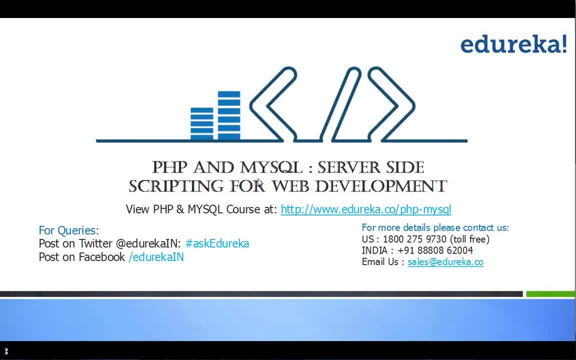 Basically, when we talk about web, basically we do server-side programming and client-side programming. So server-side means we're a web developer, We're a web developer, We're a web server is involved. a server is a system that interprets our restrictions and that. 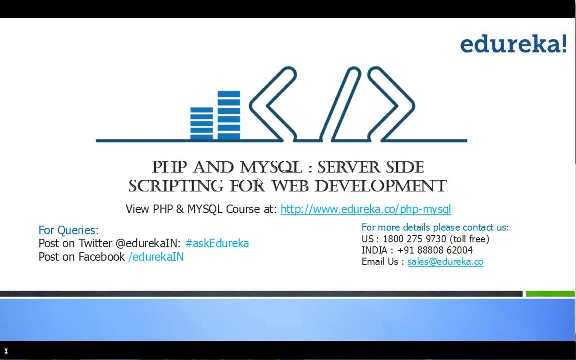 returns the result. as per our instructions, that is called a server and here in PHP when we talk about a server, Apache server is the most preferred server that is used with PHP, and if you talk about database, then MySQL is a database that best use the PHP development. 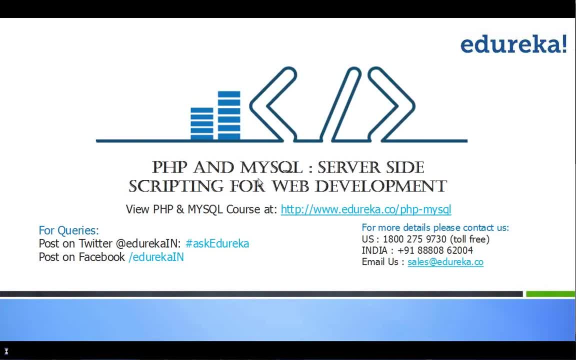 So what a database is what PHP is for and what is Apache that we will be discussing in today's session- that how we can use PHP, MySQL and Apache to develop a portal or web application that can solve or automate your problem or, you can say, your business and lot of stuff. 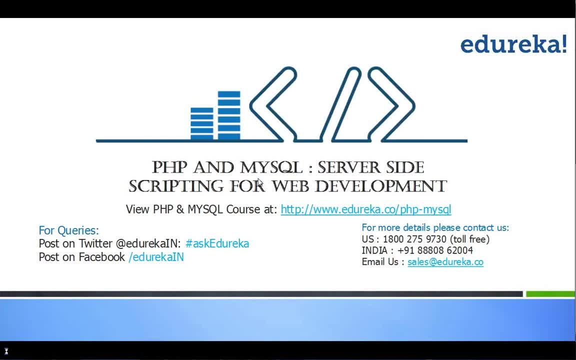 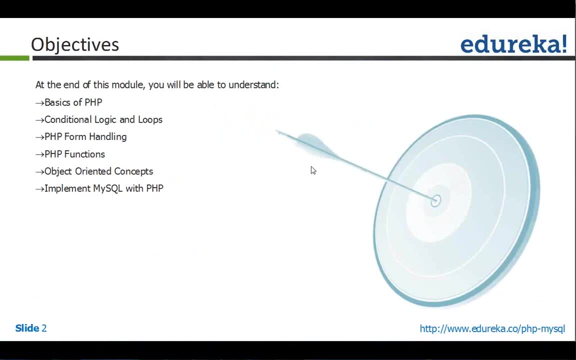 Hi Sujan. so let's start with the introduction and we'll see further that how PHP and MySQL can be used for a web application. So today our objectives would be: first of all, we'll see the basics of PHP, that what is PHP, why it is called server-side programming. 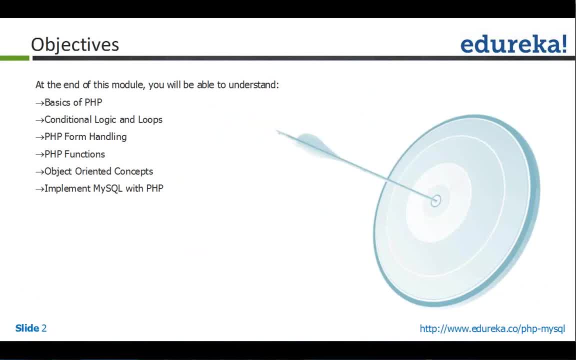 and how it is different from, or you can say how it is having advantage over other server-side programming languages. Then we'll see bit of conditional logic and those basically In your real life. you can see that sometimes you get conditions, you get you are stuck. 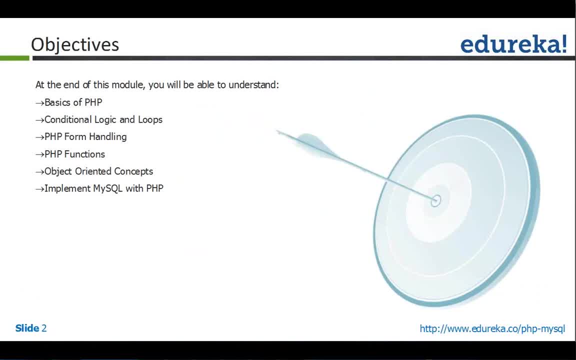 in some conditions that if this will happen, then I will do it, otherwise I will do some other stuff. So that kind of stuff that we get in real life is called condition. So the same way those kind of real life conditions can be implemented in PHP as well. 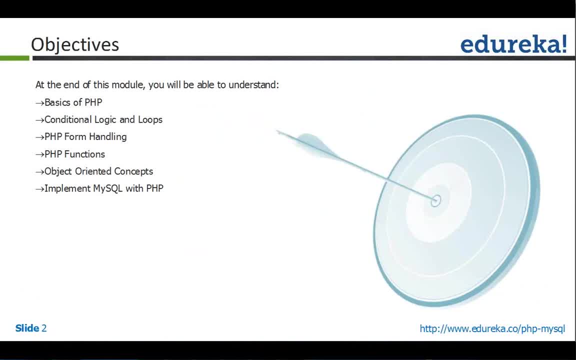 Because PHP is a server-side programming language. Okay, Sujan, You don't know PHP, but you don't know. Okay, you don't know PHP, but you know MySQL. Okay, no issues. Today I will give you a introduction to PHP. that, how PHP can be, can do interaction with MySQL. 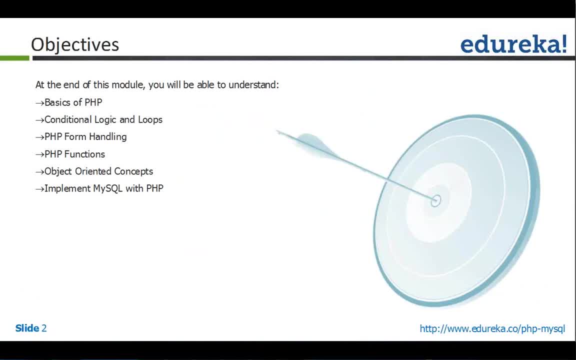 to build web applications. PHP is basically a programming language, If you are aware of C C++. basically, C? C++ are on desktop side, but PHP is on it can. PHP can be used on web Web development. that's why it is called web development. 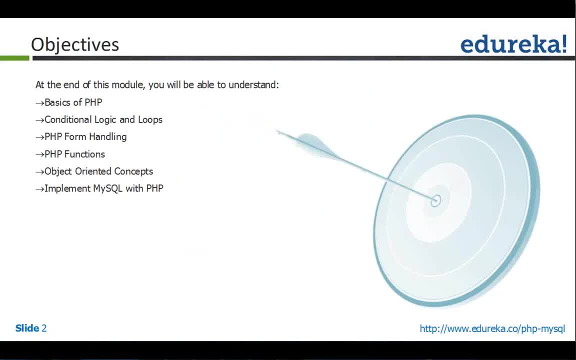 Web means where we can store our data and that can be seen, or we can have interaction with that data from multiple locations. So whatever we can put on web and interact from multiple places, that is called web development. So, Sai Kiran, you want to? okay, just a second. 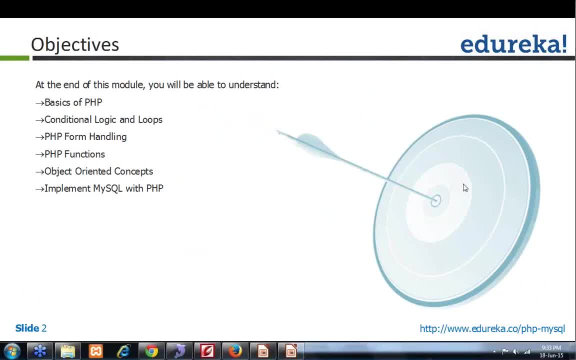 Yes, Sai Kiran, tell me what you want to say. Sujan, today I will explain you a concept of PHP and interaction of PHP with MySQL. That how we can. some of the basics I will discuss. That means I'll be discussing some of the basics of PHP. 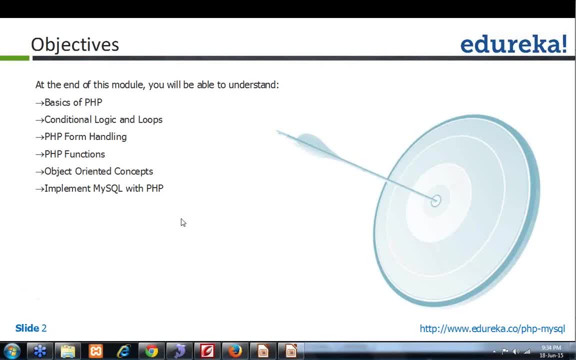 How PHP came into the market and how it became a popular web development language. Then we'll see a bit of conditional logic and loops. Then we'll see a bit of conditional logic and loops. Then we'll see a bit of conditional logic and loops. 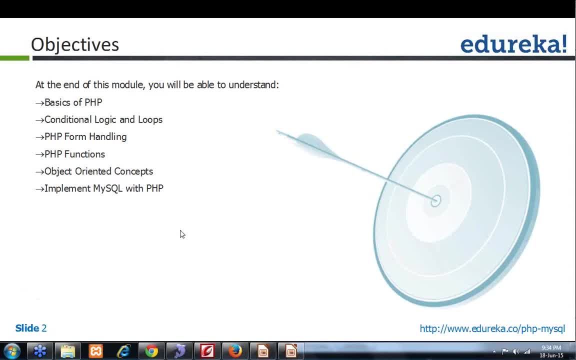 Loop means sometimes we want some information to be repeated, Like if we want to count from one to 10, so we'll be increasing counter by one and we can count That way. that is called repeating of a particular thing or repetition of a particular logic. 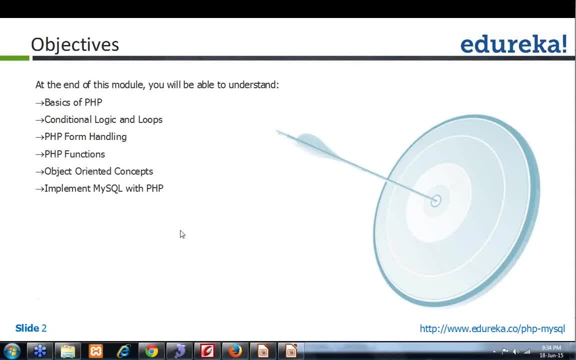 So that particular thing is called loop. Then we'll see PHP form handling Form. you might be aware of forms Basically when you go to some bank or some other, Basically when you go to some bank or some other. Basically, when you go to some bank or some other. 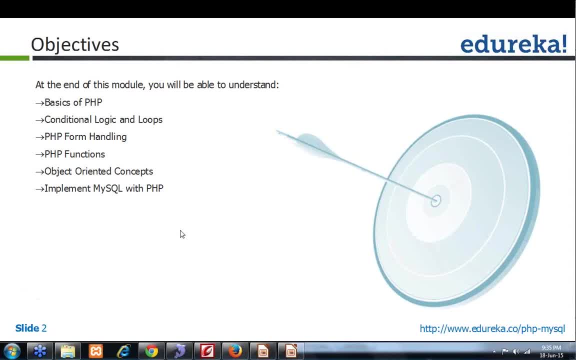 organization or some company or financial organization, any kind of organization. when you visit they provide you a form to fill up, Even in the supermarket. sometimes they do their marketing and provide you some forms to fill up where you need to provide your first name, last name. 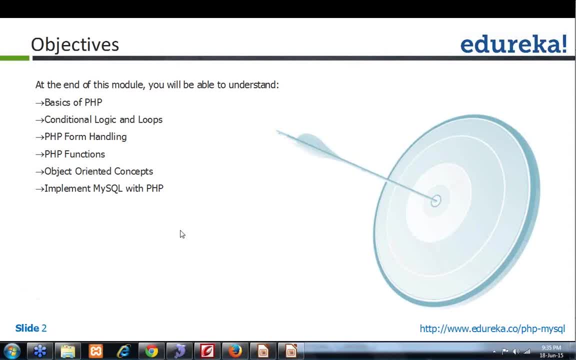 email address, personal information, some kind of business information they can ask for. If you go to a bank, you have to open up an account. You have to provide a lot of information like your residential details, your personal details and some proofs. they may ask and they may ask. 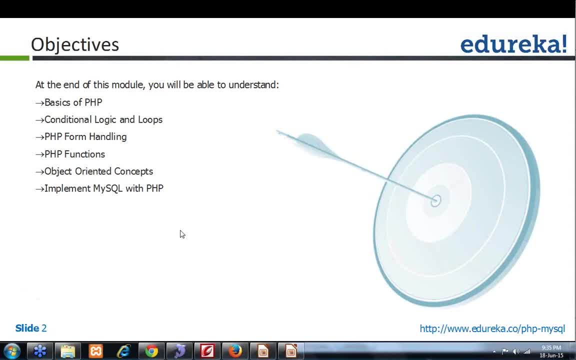 that attach the proofs with this particular form and also provide the information for those proofs. So all this kind of information you need to fill in a form So that kind of forms can also be designed in PHP into web development, For example, if you are, I think you might be aware. 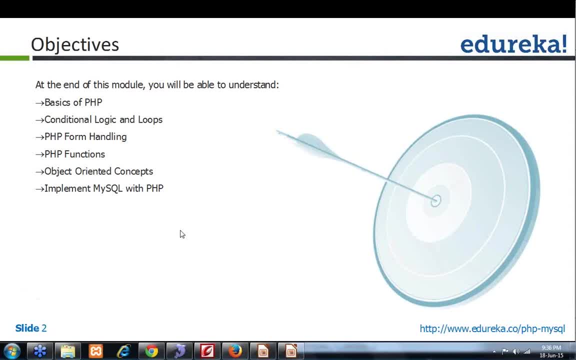 of using email accounts. So email accounts, when you have to create a form. you create an email account, you get a form where you fill up your details: your first name, last name, your expected or desired email address, your password and a lot of more information. 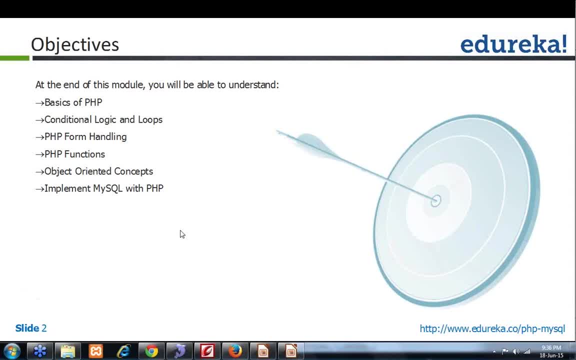 So that kind of information we fill up is called a form. So forms. when PHP was not there in the market, only HTML was there. then we can have static websites with HTML. We can't build dynamic websites. but as PHP came into the market, 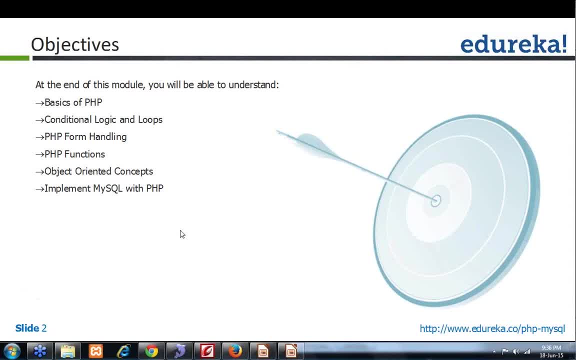 it became a dynamic thing because a dynamic web development language. why it is called? because here you can interact with the system. whatever information you will provide, you can save it, you can update it or you can see it whenever you need. 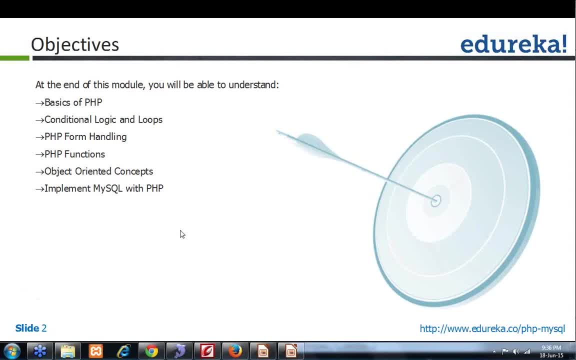 So that's why it is called a web development language, dynamic web development language, Sovic. no, if you are aware of C and C++, it is good, but if you are not, even then you can start with PHP, because starting means basics of PHP are very simple. 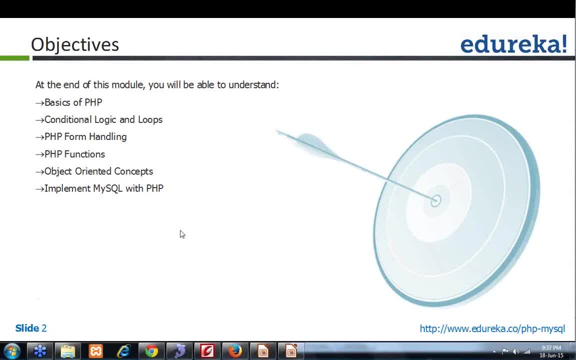 and easy to understand, So I don't think you will get any issue while learning PHP. If you are aware of C, C+, C++ or Java, that is really good. That will help you out. The same thing, the same thing, can be done with NET. 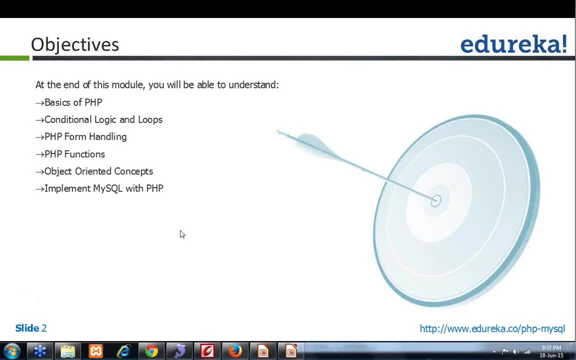 Then what is the difference? Why we should use PHP? Okay, the PHP first of all. we'll see in further slides some of the characteristics of PHP. First thing is that it is platform independent. You can develop on any platform. Second, it is easy to learn. 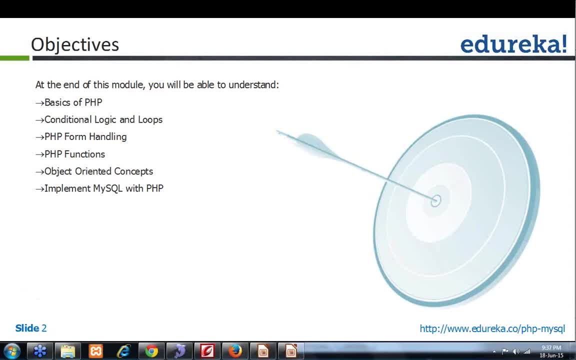 Third, it is an open source. You don't have to pay any license, buy any license, or you don't have to pay anything to get PHP work on your system And, moreover, servers where you host your websites will get for very cheap. 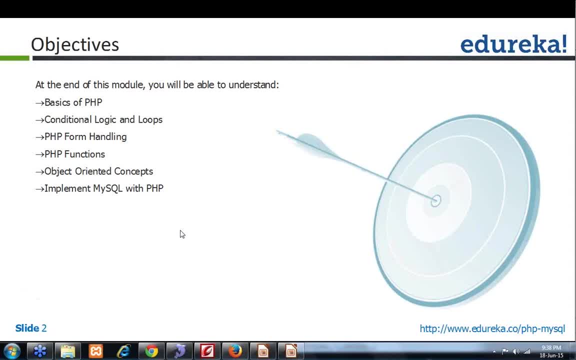 if you are going with PHP only Because most of the servers are having PHP installed on their servers by default. For learning PHP, do we need to learn JavaScript? No, JavaScript is not mandatory. to learn PHP, JavaScript is on client side. Now the difference between client side. 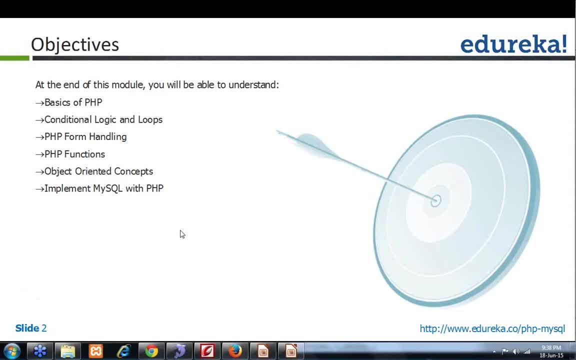 and server side is that client side means that interacts with the browser only That is browser dependent. So JavaScript is always browser dependent because it runs on the browser itself. It doesn't need any server to interact with. So client side technology always interacts with the browser. 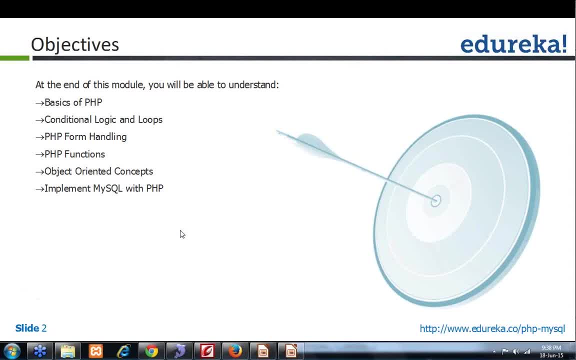 But- and that is dependent on the browser, because you might have noticed sometimes that whenever you write a code in JavaScript and you run it on Mozilla or you run it on IE, Internet Explorer, both give the different result, Because it is dependent on the browser's capability. 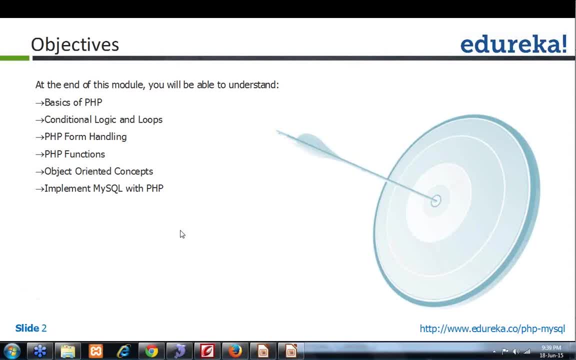 But a server side programming is that that is not dependent on the browser. You have a web server. That particular server side programming, like PHP, interacts with the web server and returns us the result, And that web server is on your server. that can be on your local system. 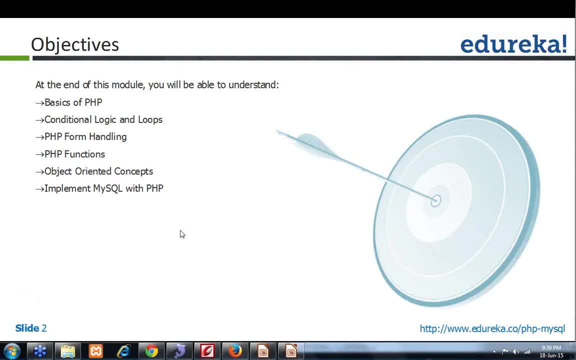 or it can be some shared system or it can be some cloud. So it depends upon your server. It depends upon your requirement, your features. So PHP, a web development language like PHP, is dependent on any browser, So JavaScript is not necessary to learn PHP. 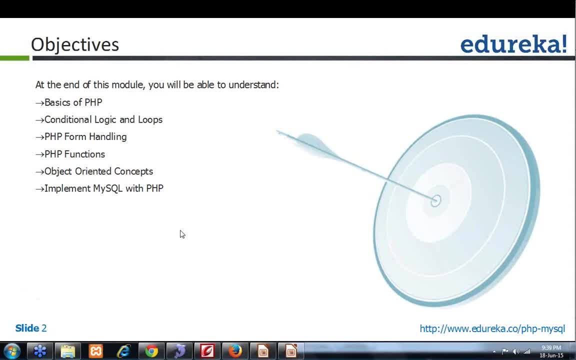 Once you learn PHP, it would be easy for you to learn JavaScript. Yeah, Mangesh, there's a question from Mangesh. is that can we take the questions and answers at the end of the session, please? Raj, your question is core. PHP is good. 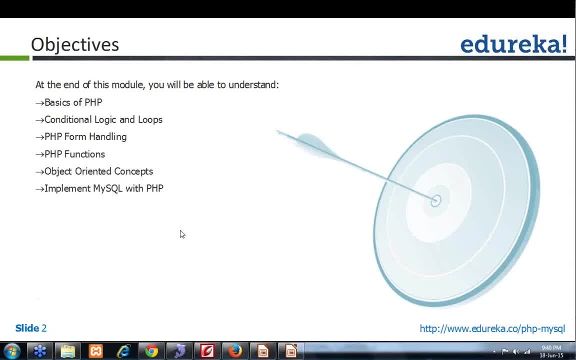 or using framework is good. See, core PHP is good for basic programming. When the question comes for readability or usability- or you can say security, then always we prefer frameworks, Because frameworks are nothing but they are design patterns that use core PHP. That means you can say: we design a particular structure. 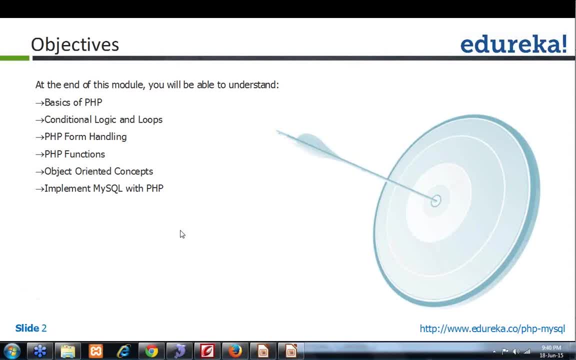 and ask for the structure we work. So framework is always better. But if you talk about speed, then definitely when you are using a framework, speed would be a bit degraded, but that you won't be able to feel because if you are having a good server, 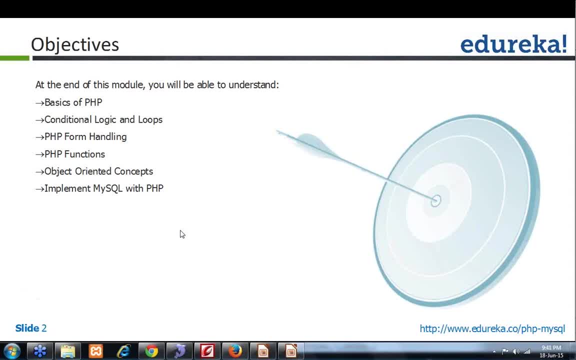 good configuration. you won't find any difference while using core PHP or a framework. So framework is better for reusability. If you want to reuse some code, you can use code. use it using framework and the wish. your question is: is PHP easy to learn? yes, it. 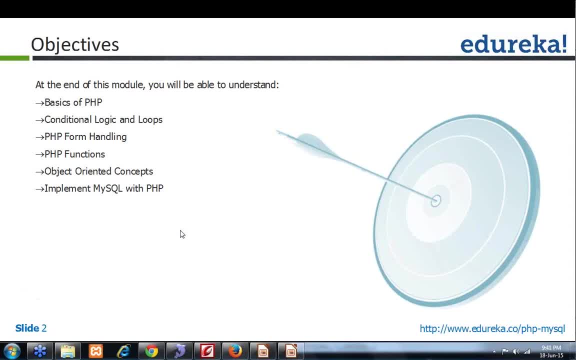 is very easy to learn, Roger. question is: which framework is best for performance? see, lot of frameworks are there in market. if you talk about good frameworks, then there are. there is y double I, there is symphony. there is an framework, then you can say Laravel, codeigniter. so lot of frameworks are there. is it better I? 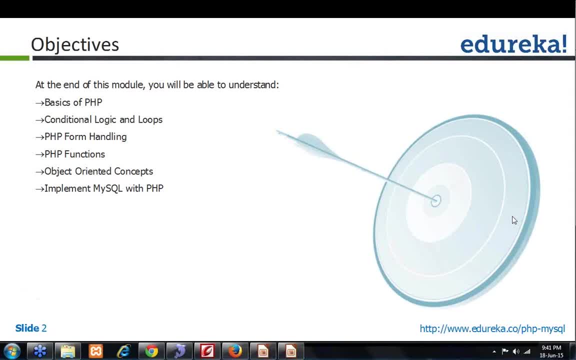 think if we first go through the session then we can discuss on the questions, because if people are not aware of PHP, how they will get the knowledge of frameworks? so let's first go with the session, then we will see into what is a framework and how we use it, because you all might not be aware of PHP. some of 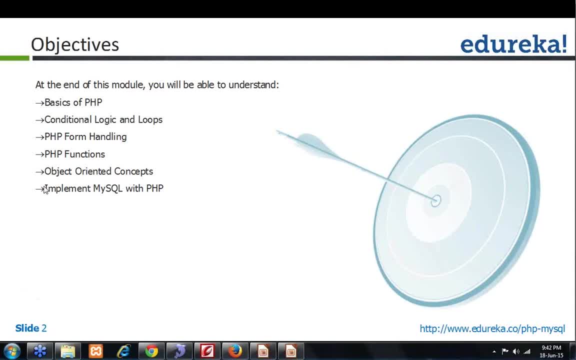 you might be aware of PHP basics, but but some are not, so it's better first let's go through the slides, then we will discuss on your advanced questions. So here are objectives. after form handling, we will be looking into functions. So function is a construct that is used. 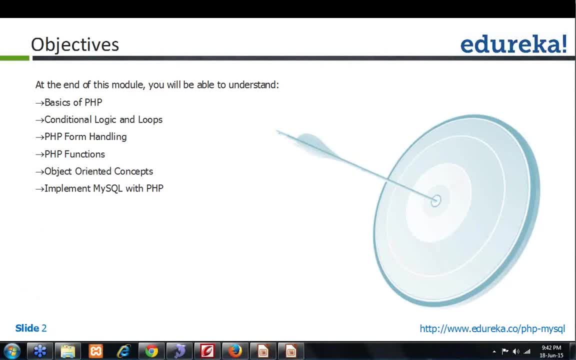 for reusability of code. There is a most basic concept of PHP or most basic block of PHP that we can use for usability Through. PHP is a server side language and HTML5 is on client side, So it is not mandatory to learn HTML5 to learn PHP. 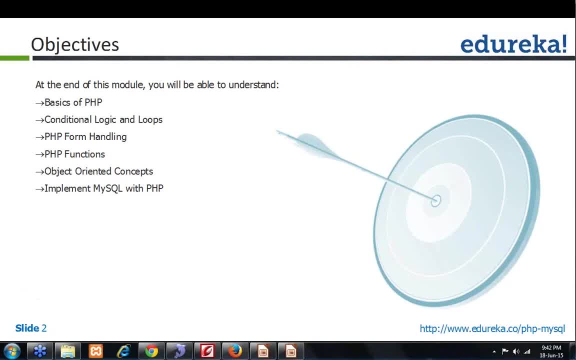 If you have knowledge of HTML, basic HTML, HTML4- even that is fine HTML5 you can use for your. if you need some advanced concepts of HTML5, then you can go ahead with it. Otherwise, basic knowledge of PHP, basic knowledge of HTML4 is enough to design forms. 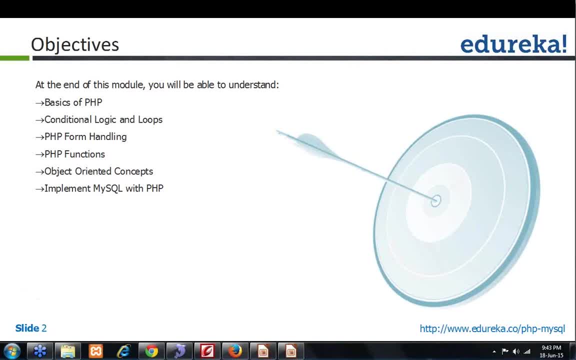 Because forms will be designing into HTML and those forms will be handled into PHP. Next objective bit of object oriented concepts will discuss, So object oriented, what object is and how we build object oriented concept that will be discussing today. Then I will let you know how MySQL can interact with PHP. 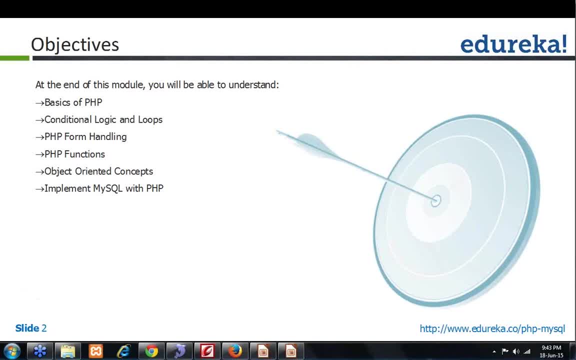 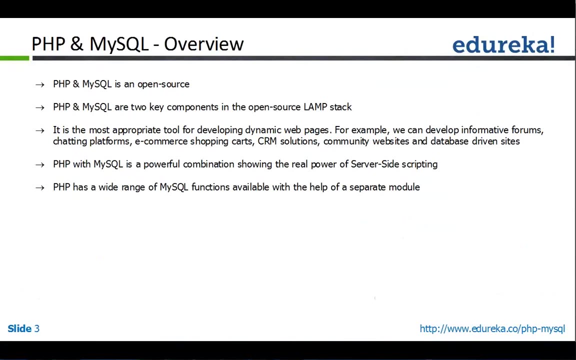 We can have MySQL server. we can write down queries over there and we can execute them. But how queries can be written into PHP and can be executed, that will be discussing today. So here is a bit of overview. PHP and MySQL- PHP MySQL: both are open source. 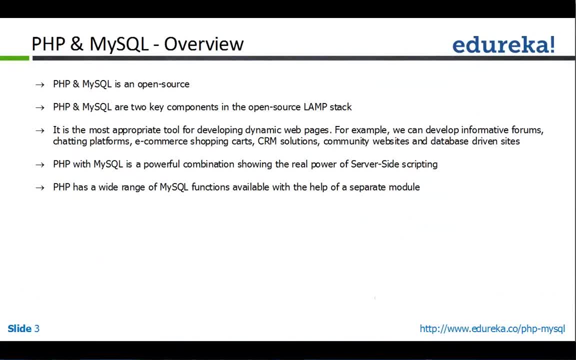 You can get it for free. So here is the answer of one of the question, that why we should prefer PHP over NET. because NET you have to buy licenses, you have to pay for it, But for PHP you don't have to pay anything, it is open source. 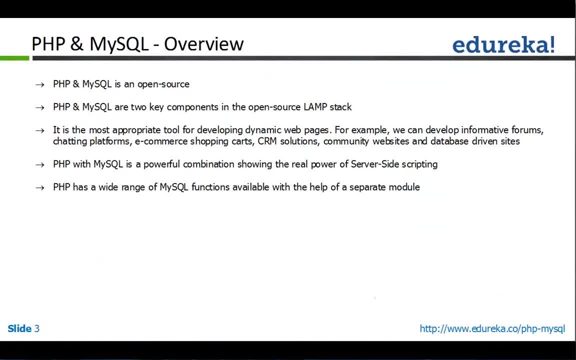 you can get it free of cost and you don't have to buy any license to install it or to work on it. PHP MySQL are two key components in open source LAMP stack. So MySQL is a database where you can save your information and PHP is a medium that let you people make. 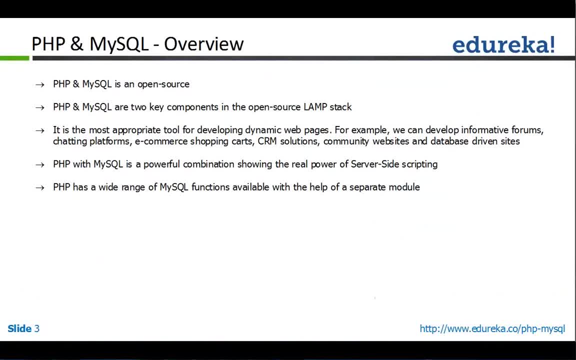 to save your data into MySQL database. It is the most appropriate tool for developing dynamic web pages. For example, we can develop informative forums, chatting platforms, e-commerce shopping- So you might be aware of a lot of e-commerce platforms like Flipkart, Snapdeal and a lot more. 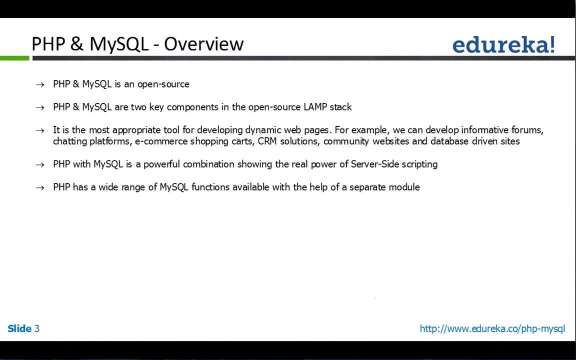 So what they do? they basically save the information into databases and from databases these information is fast based on their information saved and that is displayed on the browser, and from that information you just book your order or whatever you can do. from a shopping cart, You can buy your products and a lot of things you can do. 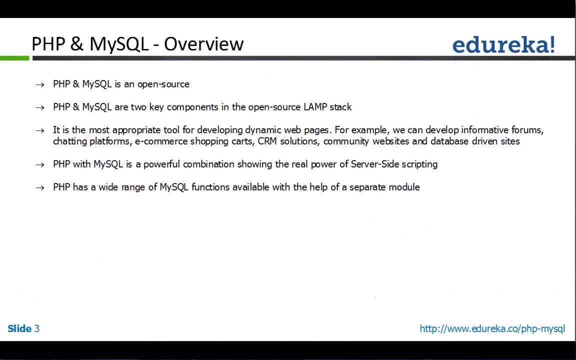 PHP with MySQL is a powerful combination showing the real power of service and scripting. So there are a lot of server side programming languages. but why PHP is dominated? because PHP is best suited with. a best database that is on the web is MySQL. MySQL can store a lot of information. 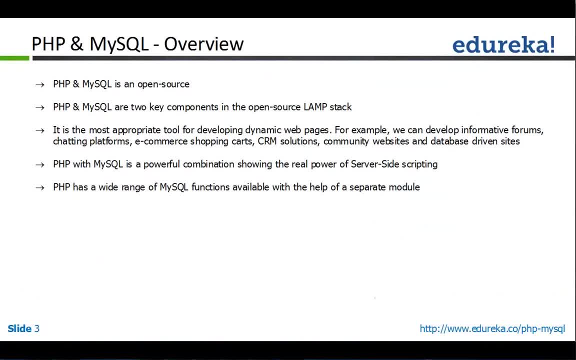 If you are using only file to save your information, how much so. if you save your information to file only, the file will be very huge and it would be difficult for you to locate a particular information. For that case, we use databases, And MySQL is a database that can save huge amount of data. 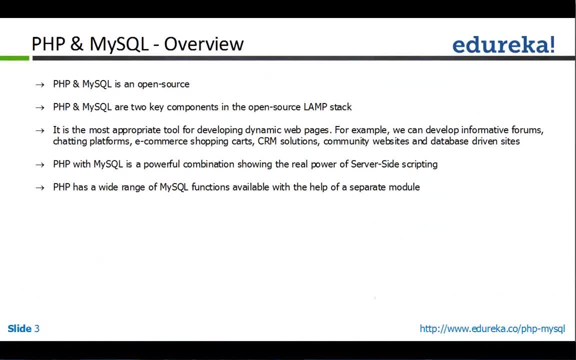 A single table in MySQL can save up to 16 terabytes, So it is huge data that a MySQL database can handle. If you save a lot of information into a file and when you try to open up that file, that file, your system will be hanged. 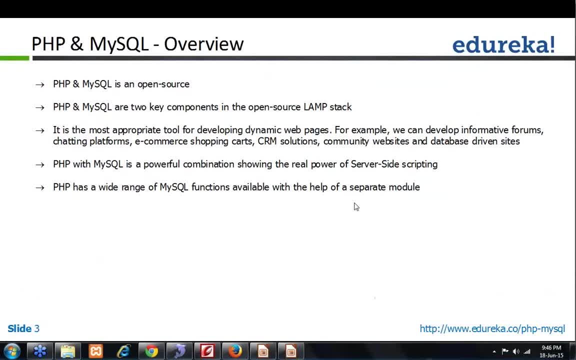 Reshma, what you are asking about, Hadoop, Hadoop- we are not covering in this session, So I won't take that thing into session because I don't want to spend time on other things. Let's first start PHP. Paritosh, you are asking, can we create application? 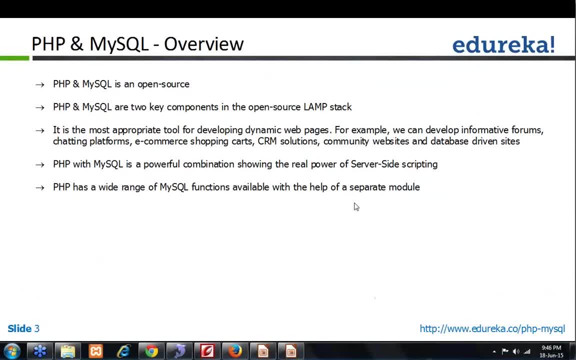 for mobile in PHP. Definitely you can use PHP for web services, for building web services, and web services can be embedded with any technology. So front-end would be in HTML5 and back-end would be PHP. That you can do for developing web applications or mobile applications. 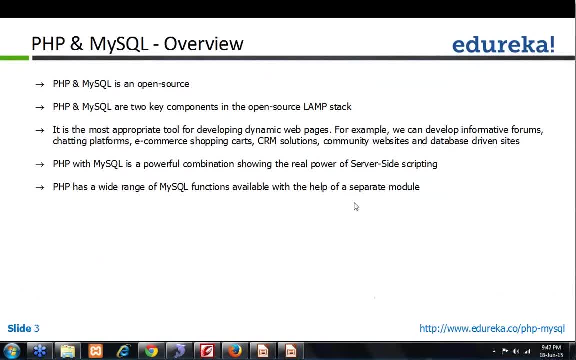 PHP is a server-side programming, So whatever you will process on your client side and based on that data, PHP will process that data and that will return it to mobile application. So building web services using PHP, you can enter the Android or mobile. So PHP has a wide range of MySQL functions. 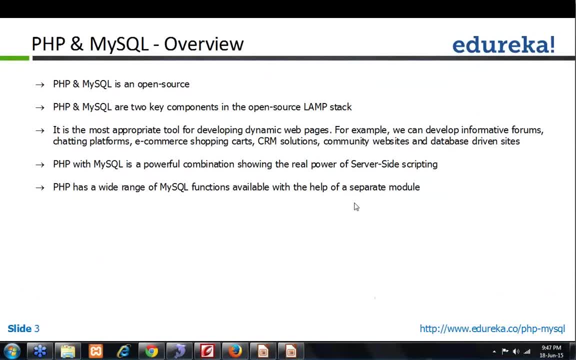 Available with the help of separate module. So lot of databases are there, like MySQL, SQL, Oracle, PostgreSQL and SQLite. but why MySQL is supported, Why MySQL is preferred with PHP? because PHP provides some internal APIs or internal functions that can be directly used into PHP programming and we can build our web applications. 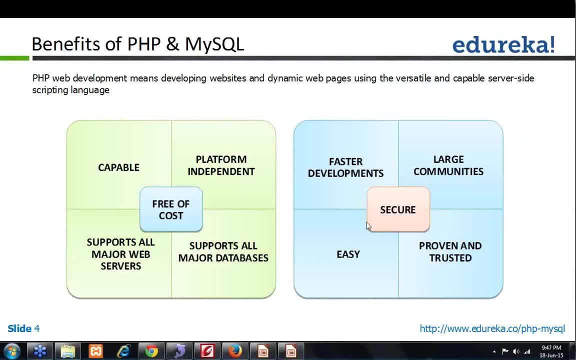 with them. There are some of the benefits of using PHP in MySQL. First of all, it is free of cost. It is capable of building large applications, small applications, So basically it can handle any size of application. It is platform independent, whether you are developing PHP. 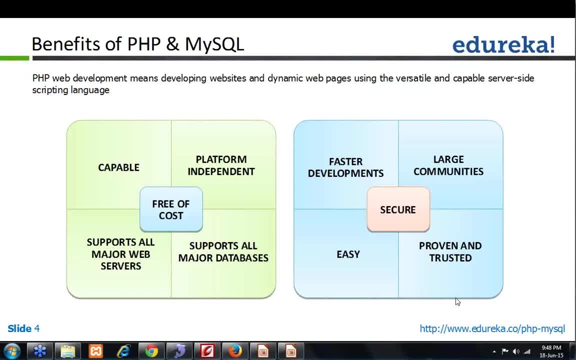 into Linux framework or Linux platform or Windows platform, it doesn't matter. It supports all major web servers So we can develop PHP on IIS or Apache or many other servers. Why we use Apache? Because it is the best suited web server with PHP. 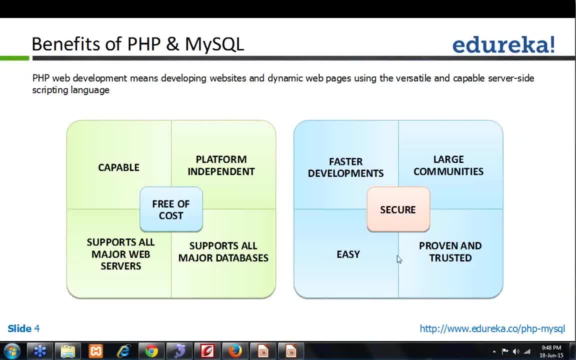 and it supports all major databases. We prefer MySQL, but you can use Oracle as well. So open database connectivity, ODBC connectivity is there That can be used to connect any database with PHP. So the wish: if you are having knowledge of C, C++. 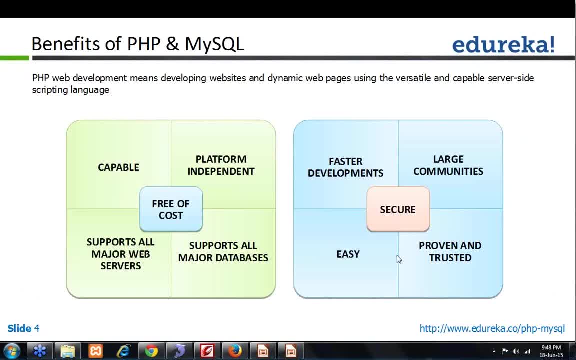 that is very good for you. You will find PHP very easy then Through difference between Linux and Windows. So Windows is a different platform. Linux is different platforms That cannot be discussed in this particular class, as this is regarding PHP. note regarding PHP in Windows. 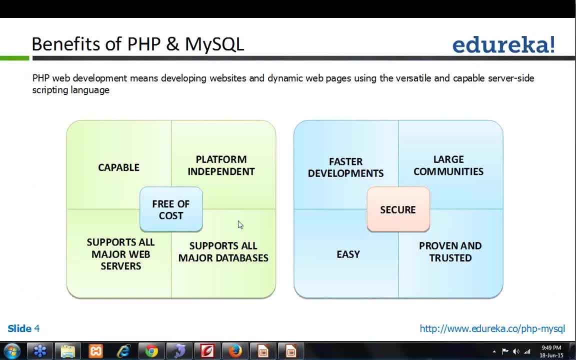 And, moreover, the second big characteristic of PHP is that it is secure. So faster development you can do with PHP. You simply write your code and refresh your browser And your data will be displayed there. That I will show you practically, don't worry. 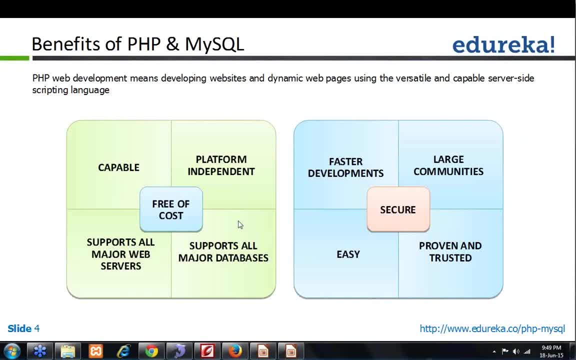 Everything what I'm discussing today. So let me some time so that I can show you people up everything practically. I will not take only conceptual thing, I will take the practical stuff so that you are aware of it and you get comfortable with PHP. 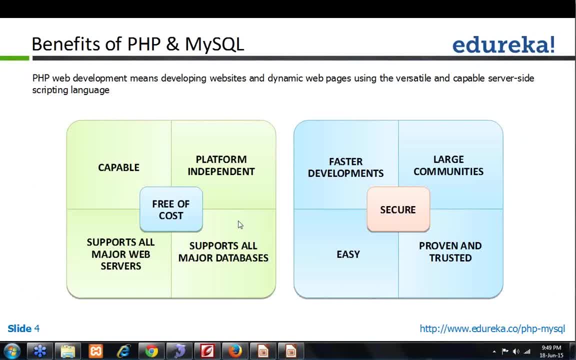 And large communities. whatever you can. you want to know about PHP. you simply write on Google and you will get a lot of information, So a lot of communities You work for PHP. You don't have to worry about whether I will find some particular thing regarding PHP or not. 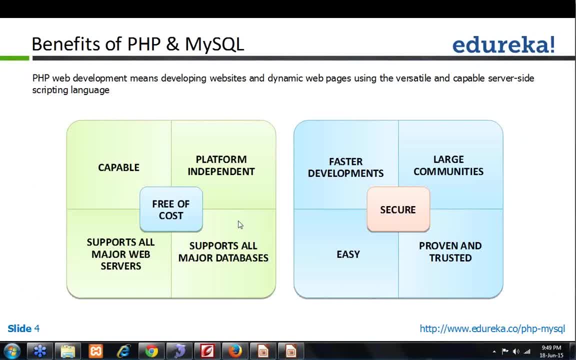 You will get everything. Reshma will be discussing on web search, launching How we create a website that will be discussing today, Don't worry. and then it is easy to learn, easy to implement and everything, And it is very proven and trusted. So, whatever you write in PHP, whatever you execute using PHP, 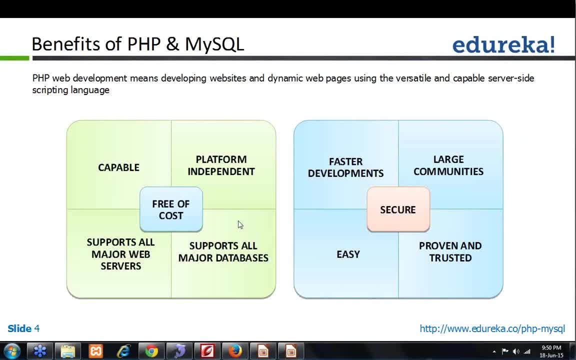 that is reliable. every time you will get The same result. It is not the case that once you will get a different, it is the result and next time you will not get the result. It is not the case. It is very stable language. 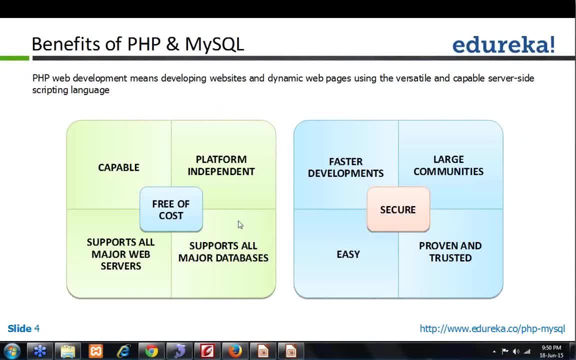 So through. if you compare PHP to HTML, we cannot compare, basically because HTML is all. HTML is a scripting. Sorry, it's a hypertext language that is on client only. It doesn't interact with the server. but PHP interacts with the server, like CNC plus plus. 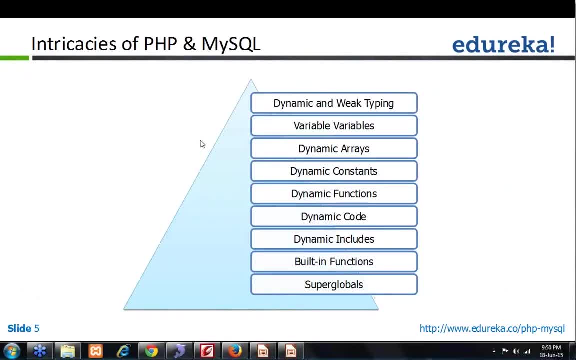 But it is on the web. This is the advantage of PHP. So here are some of internal characteristics of PHP. So first is it is dynamic and big typing. So what do you mean by weak typing, basically in PC or C++? let me start with some practical stuff. 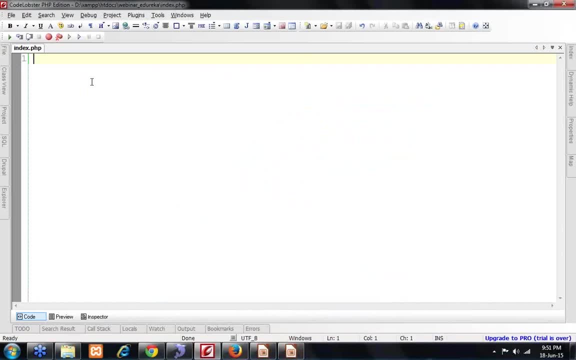 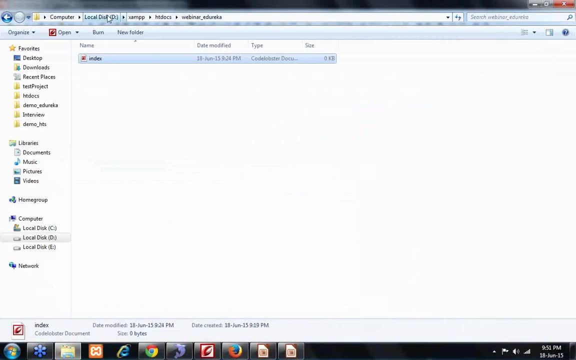 I think that would be better for you people to understand. So first of all, you have to install PHP on your system. The first thing is to install PHP. So here are two basic, basically two ways to install PHP onto your system. One is that because three things are necessary. 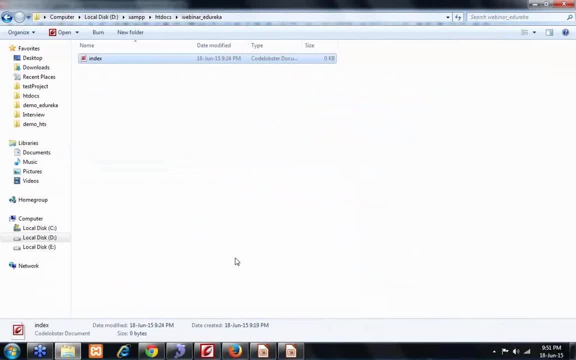 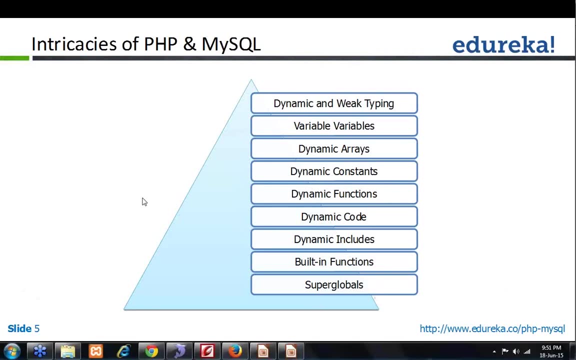 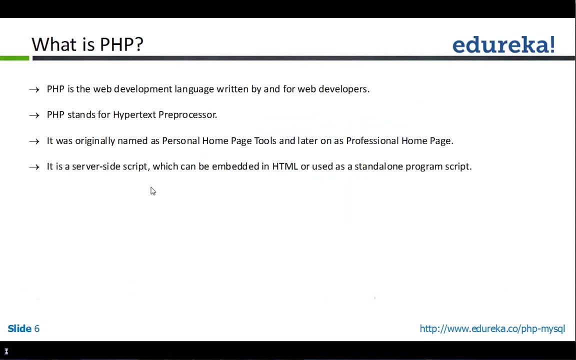 to do any kind of PHP development. No, CSS is not necessary to develop PHP. That is additional benefit if you know CSS, but it is not mandatory. So I will go to some next slides and then I will come back to these slides. So here are some of the things that are mandatory. 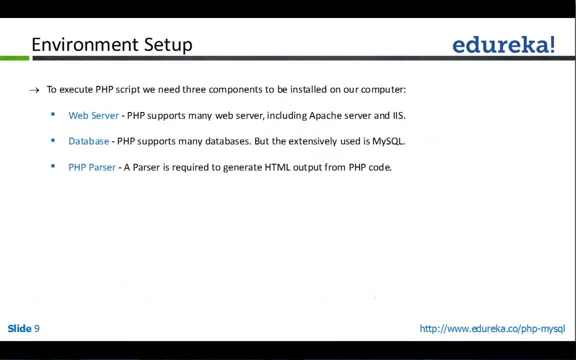 to do PHP development. If you are going to develop HTML sites, static websites- then you don't need any web server or database. But if you are going to work with PHP, you need three basic things to be installed on your system: Reshma. how do you? your question is: how do you? would you? 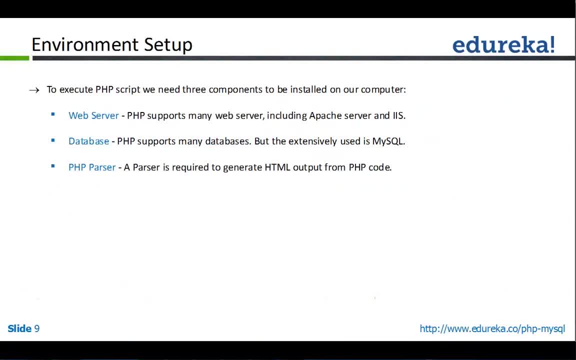 expand PHP. We will be taking it in this session, don't worry. First let me complete the slides, then most of your questions will be solved. Don't worry, I will be taking everything practically, Not the conceptual thing only. So for these are the three mandatory things. 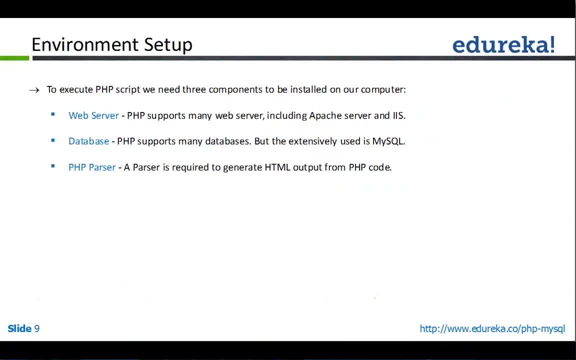 that are required to do any kind of PHP development First is web server. So server is a system that interprets your request, or you can say that answers to your questions. Answer to your queries that you do with your PHP language. So, Himika, you are not able to see my slide. 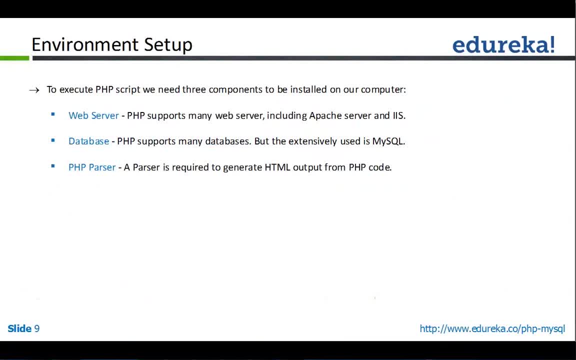 I think everything. everybody is able to see my slide, Himika. I think you should look into that. Yes, I'm on slide number nine. Yes, I'm on slide number nine. Right, everybody is able to see me. I think you should try out to reconnect. 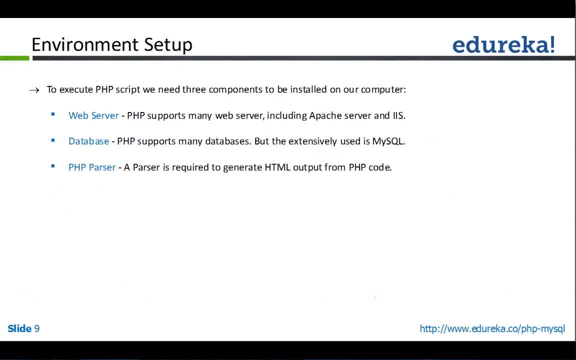 or just look into your system that why it is not displayed. It might be minibuys or like that. Okay, So web server is a system that understands your request and replies to that particular request. It sent respond to your request. It responds to your request. 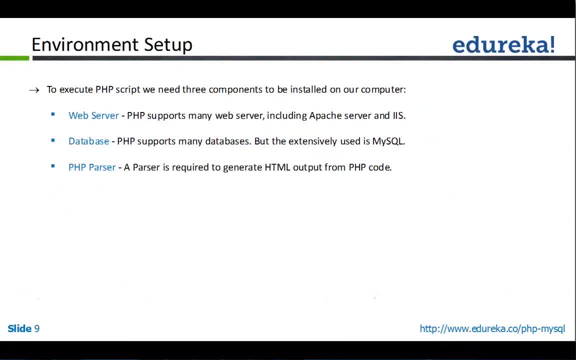 A database is a you can structure that can save your data permanently, that you can use for further use, and PHP parser. So parser would be associated with Apache, So that parser would be interpreting whatever you do and that will be replying. that will understand the request. 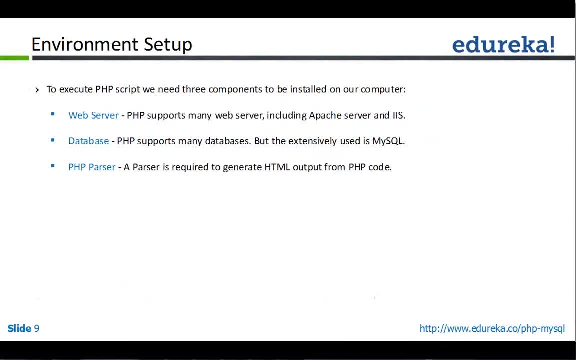 Basically, parser is required to understand your request. Yes, Mitesh, PHP supports Oracle database. PHP can interact with lot of databases. The thing is that some of the databases you PHP doesn't provide the internal APIs for that. you can use open database connectivity ODBC. 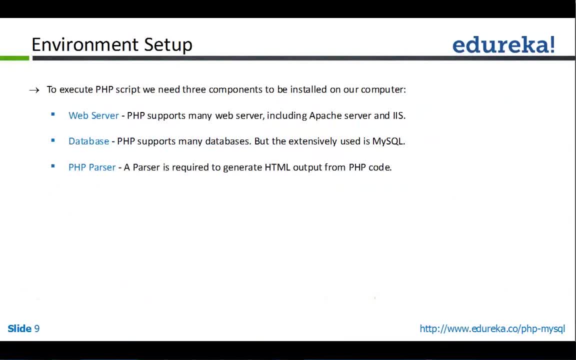 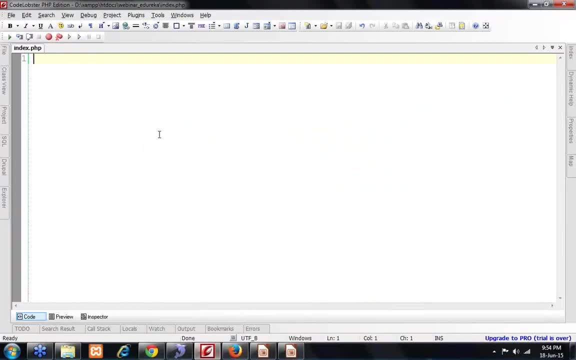 So whenever you search in PHP ODBC connection, you will get that information, that how you can connect Oracle database with PHP. So let's start with some basic PHP. So, first of all, I am telling you that these are the three things that you need to install. 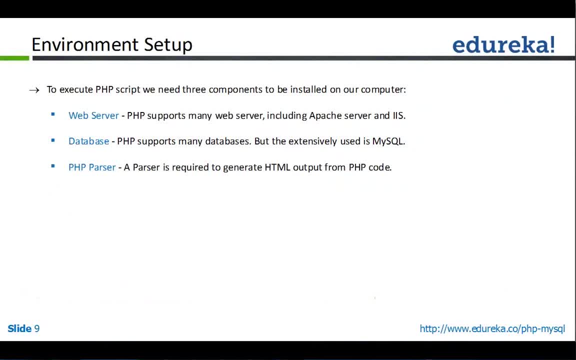 You need to install into PHP. one is Apache server, Then PHP and then mysql server. So first you will install Apache server, Then you will install PHP, Then you will install mysql. Yes, Yes, Neil, websites like Amazon, Google, Yahoo, Everyone uses PHP. 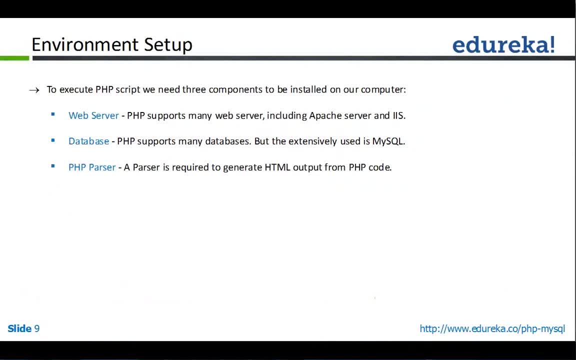 Yes, vendor. So let's start with how we install PHP, mysql and Apache on our system. So you can download Apache, PHP and mysql from the respective websites. Just write on Google download PHP, download Apache and download mysql. You will get their setups and you can install on your system. 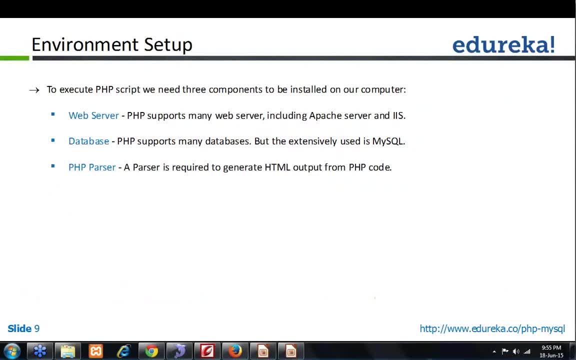 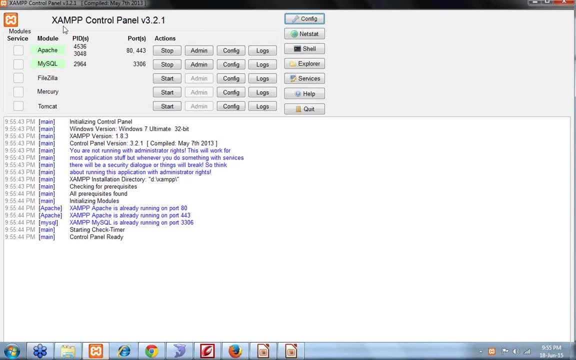 So first you will install Apache, then PHP and then mysql in this serial you need to install, or what you can do. There is a. there is a Package called Zemp X, a MPP. So this contains Apache. a MPP here means X, means extended a means. Apache M is mysql. 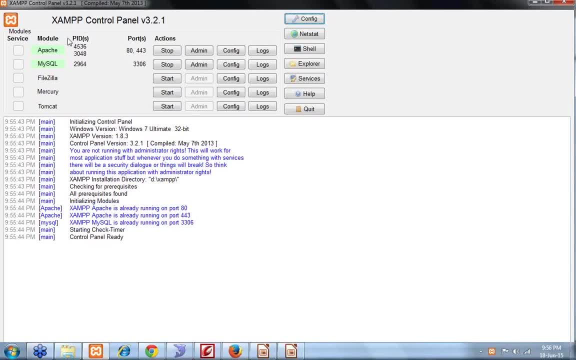 P means PHP and then again P means Pearl. So in this particular setup you can work with both PHP and Pearl, but today we'll be looking into PHP only. So with the PHP version that we are going to Learn in this course would be PHP 5, latest version of PHP. 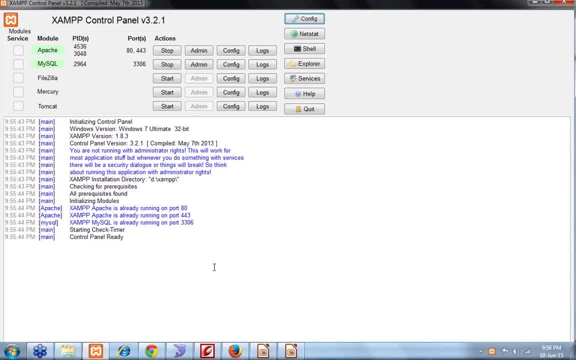 So PHP 4 is almost out of the market, So we won't be discussing about that. We'll be discussing about concepts of PHP 5 only. So this is the package called Zemp. So whenever you write on Google, download Zemp. 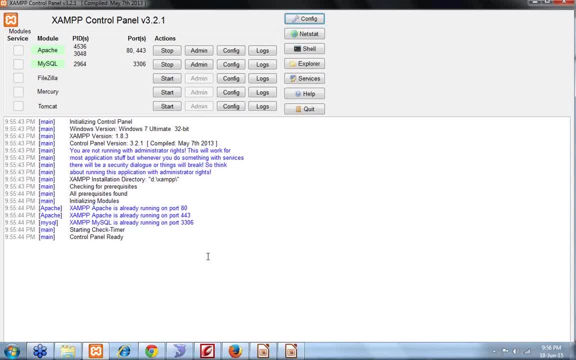 you will get a website called Apache friendsorg, So on that, Apache friends, door or door to RG, You will find Zemp installation for Linux servers, for Windows servers, So you need to install. if you are using Windows, you can use them for Windows. 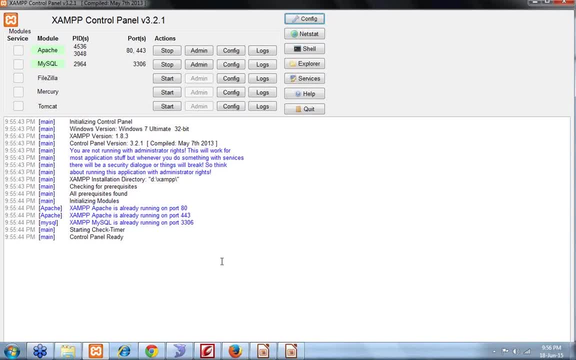 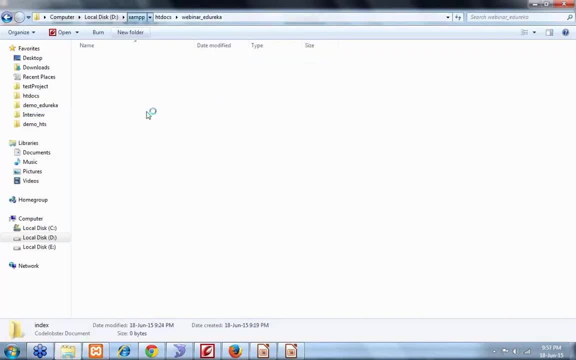 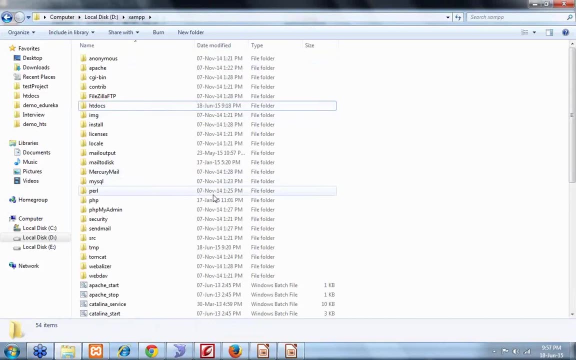 You can get the setup from there, download the setup from there and you will install. and as you will install it, So installation will create a folder called Zemp. So this is my Zemp folder. So installation you can do in in whichever drive you. 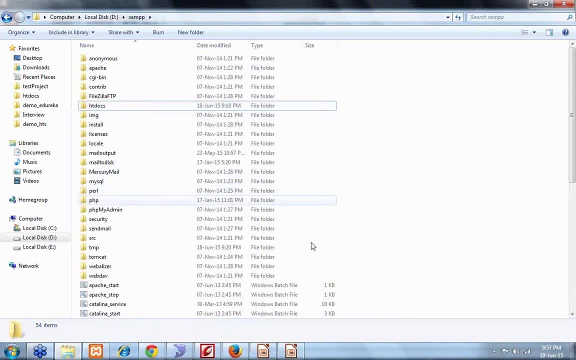 You are willing to do. you can use C drive or D drive or E drive, whatever drive you need to install. You can simply give the path while installation and you can install Zemp. So once you install Zemp here, you will get Apache folder for Apache, folder for my SQL, folder for PHP. 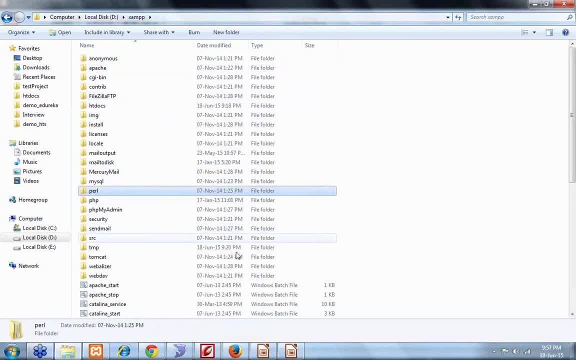 and folder for power. So everything in this package is installed automatically. You simply need to install Zemp package. Otherwise, if you want to install individual things, then you have to install Apache inducerly, then PHP inducerly, then my SQL inducerly, and only then you will be able to use. 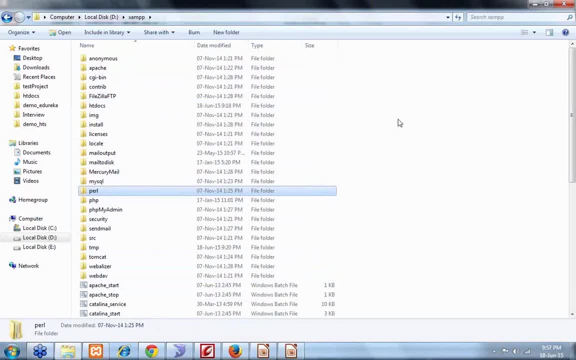 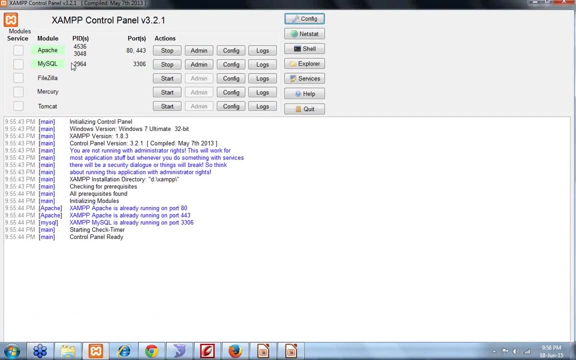 but if you are going to do your local development, you can just go with Zemp package and that will install PHP, mysql and Apache on your system. So when you, once you install Zemp, you will get this kind of control panel. So this control panel is having buttons. To start Apache server and mysql server. So through which server is popular, Linux or Windows? basically, PHP is better to work with Linux, but you can also work on Windows. There is not an issue. See, I've told you that PHP is platform independent. 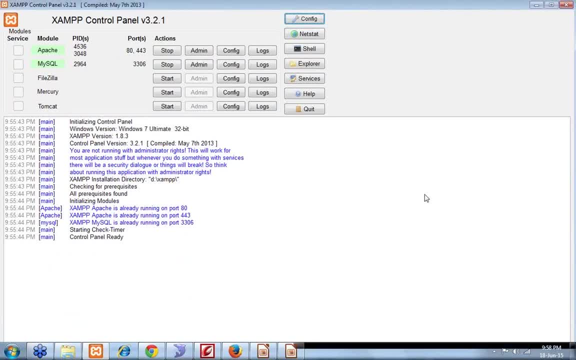 It can work on any platform. Yes, Yes, Yes, Yes, Arti, you can. you can record, and, moreover, this session is being recorded on my site as well, And this is also. this also will be recorded on a direct aside. Yeah, drove Linux is more secure and it is more sophisticated to be used. 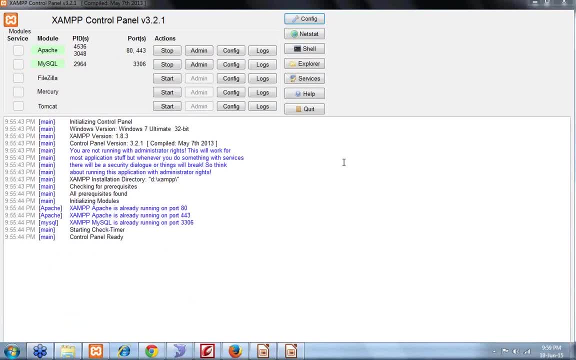 So let's discuss PHP first, then we will be taking other queries. So here you can see Apache and mysql, So let's stop them first. I will. when you will install Zemp for the first time, you will get this control panel. So Apache is a server. mysql is also a server. 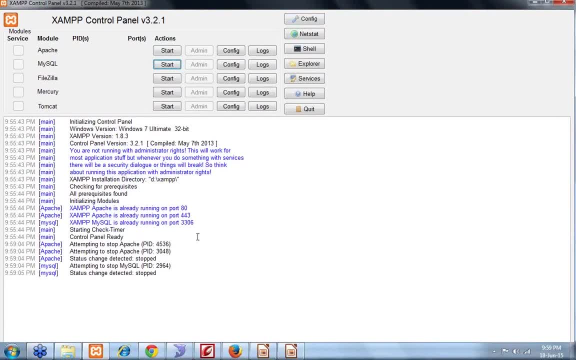 Apache is a web server and mysql is a database server. So in order to use a server, you need to start it. start the server. only then server would be able to interact with your parser. that is PHP: Ashish, tomcat. Yes, tomcat. 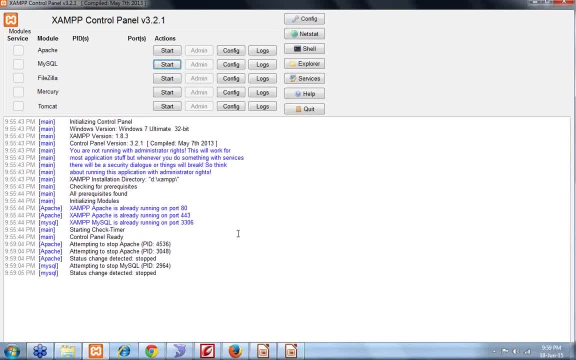 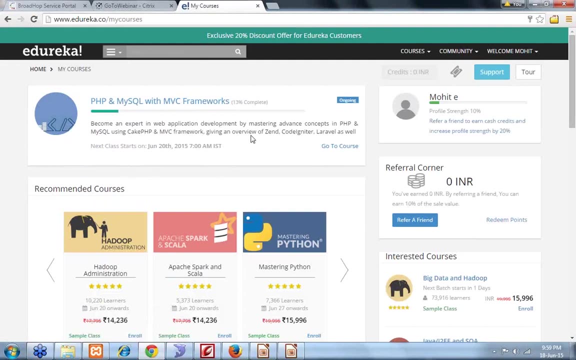 We can also use with PHP, but we are not going to discuss tomcat or Mercury in this session. Shikha see, when you register with The azureka, you get this login, you will get your credentials and you can log into that and here you will get the link. 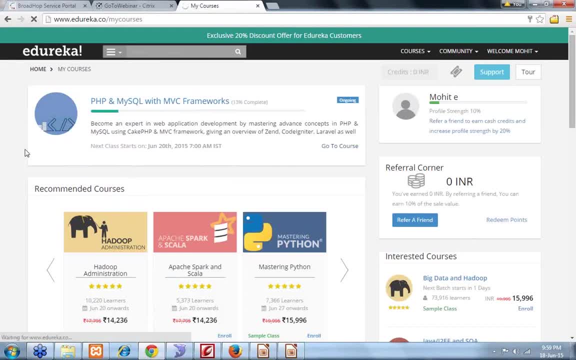 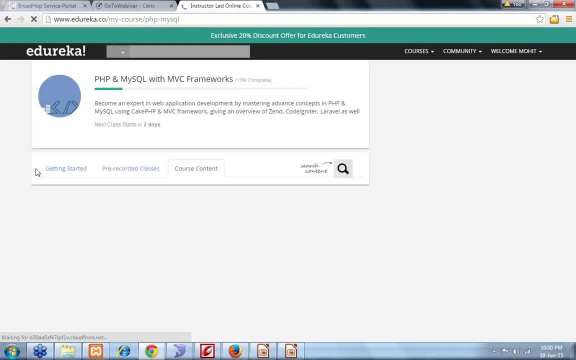 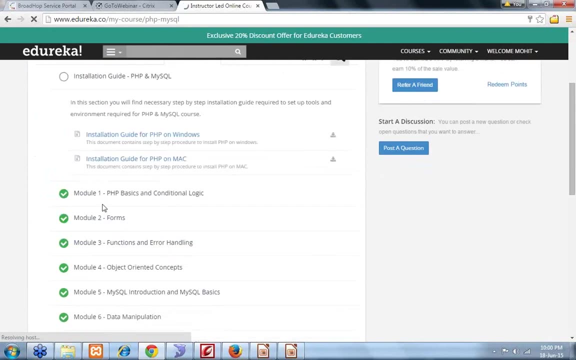 for your course And if you need recording, you can talk to azureka regarding that. they will provide you the recording. See, here you will get all the contents of your PHP. So once you get registered with azureka, you get a login and you are able to get your see your course over there each. 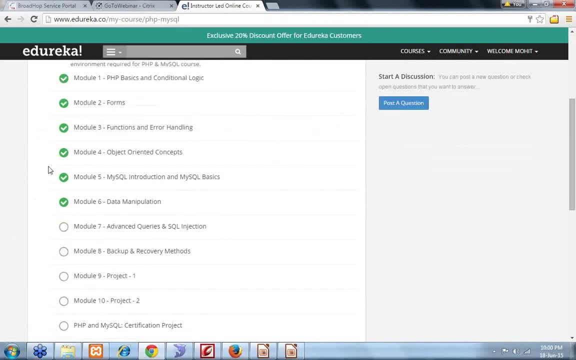 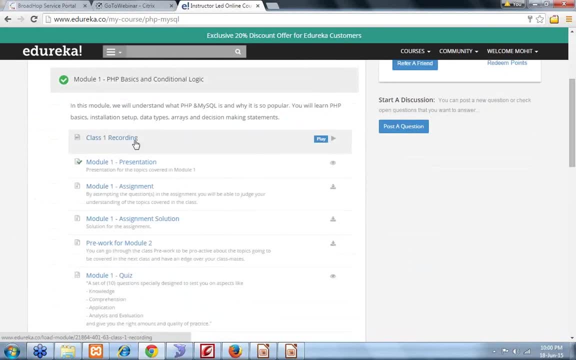 and every chapter you will be able to see and, moreover, with each chapter you will find the recording. here You can see class 1 recording. So, once you get registered, every class will be recorded. after that, and you can listen to a particular recording simply by login into your account. 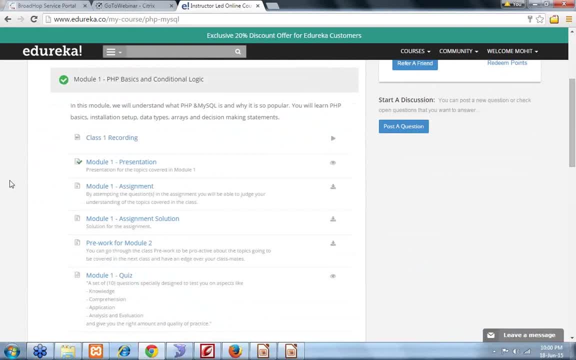 Kamlesh exam is basically for local systems. when you install your, when you do projects on the web servers, that is already installed over there. You don't have to install on a web server. when you are going to host a website on sub server, that server will already have be having PHP and magical. 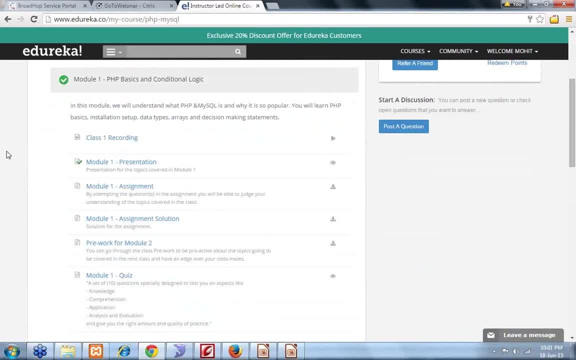 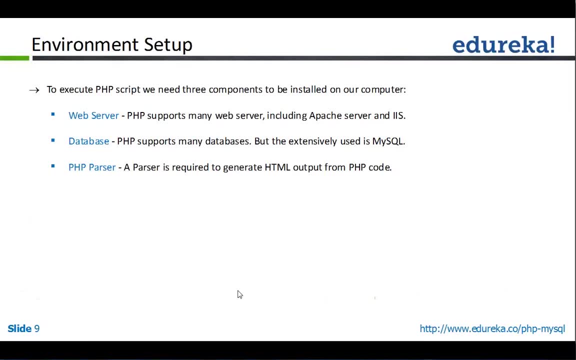 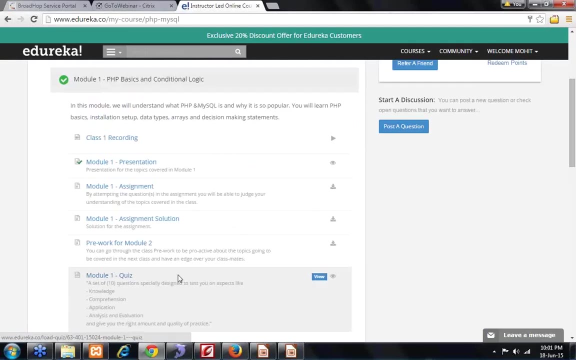 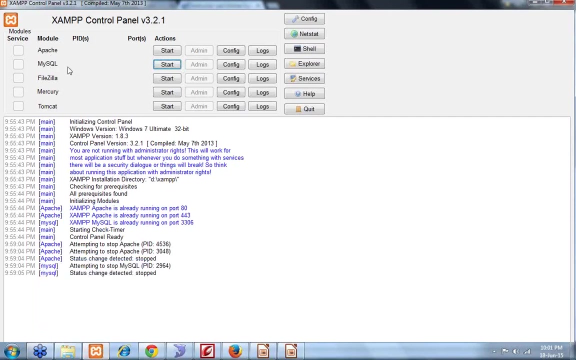 You don't have to install it and you can develop high-end projects with PHP. That is not an issue. So once we have installed Xampp server, you will get Apache and mysql. You are welcome Kamlesh Apache and mysql, So you need to start with first. 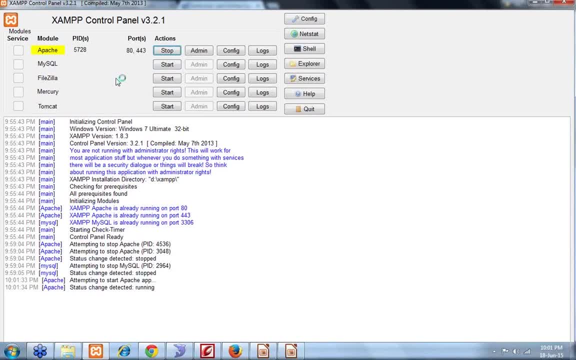 I will start Apache server. So remember one thing: Apache runs on two ports on your system. One is port number 80 and one is for port number 443.. Whenever you go to some secure website- secure like if you go to some bank's website- 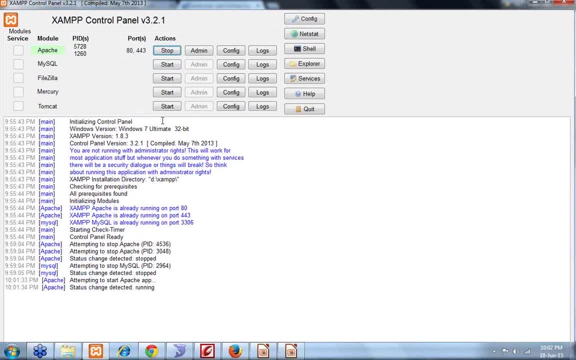 or some shopping cart website. instead of http you will find http, s, t, t, p s, then you will find sdfccom like that. So secure me that data is encrypted. That is advanced concept, So I will not be discussing it today. So Port: two ports are there basically that are used by Apache server. 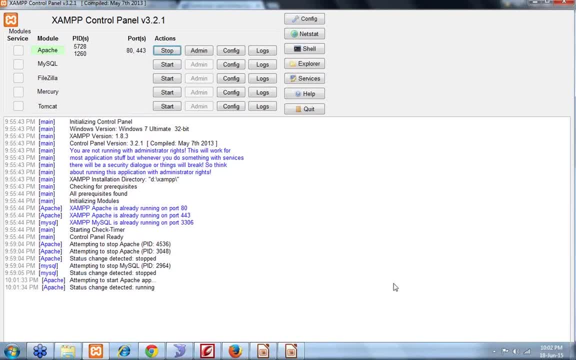 One is 80 and one is it 443. when we work with s t t p, we port it is utilized, and when we work with s t t p s, port 443 is utilized. And next we will start mysql server, and when both, the mother server will be started. 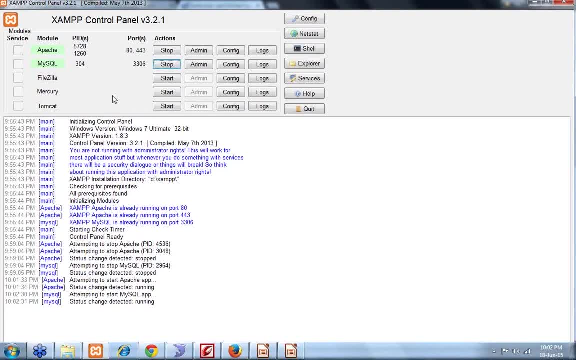 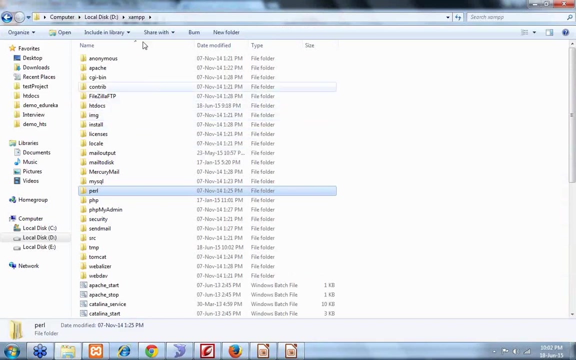 You will get green background for these modules, Apache and mysql. So mysql, by default, uses Number 3306.. So now my mysql and PHP has been started. now in order to start us project from scratch in PHP using XAMPP: when you install XAMPP, 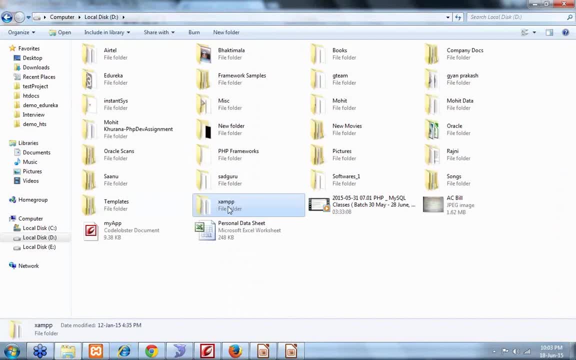 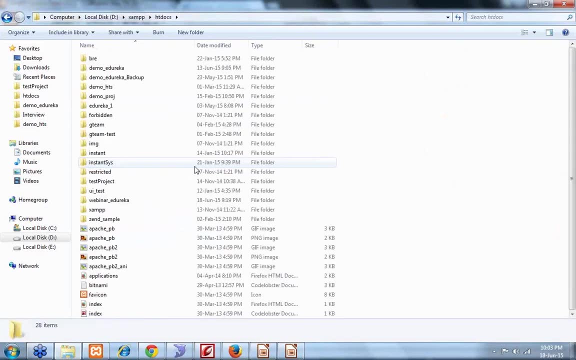 I have installed XAMPP on my D drive. here You can see XAMPP folder. inside XAMPP folder I will be having a folder called s3t- s3docs. Inside that s3docs I will be creating my own folder that I want to access. that would be creating my project files. 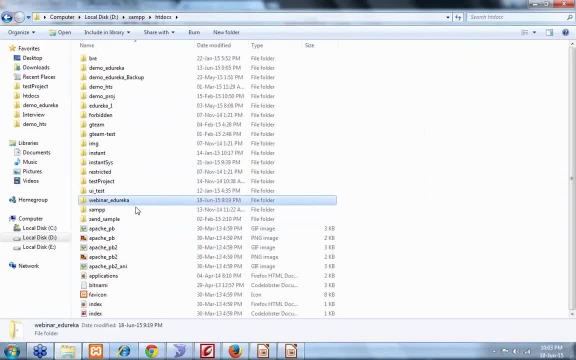 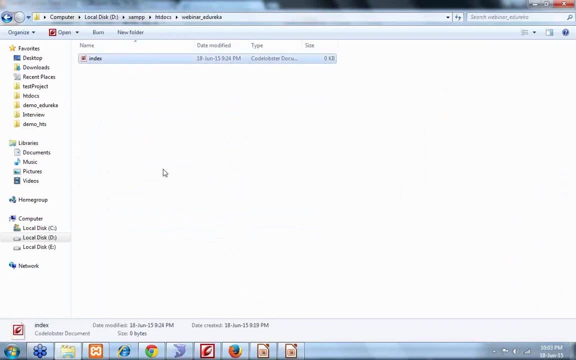 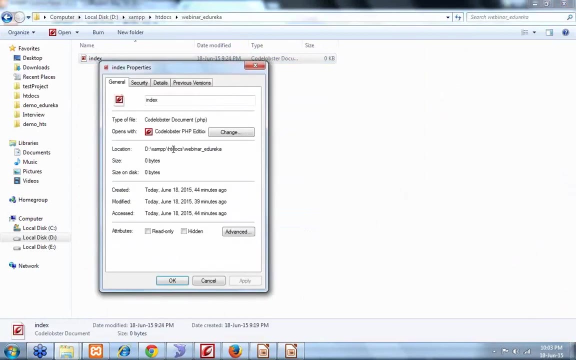 So I will be creating a folder. I have created a folder called webinar- underscore azureka. inside that folder I will create my file and that files extension would be PHP. So this files extension is index dot PHP. So see, it is PHP file. 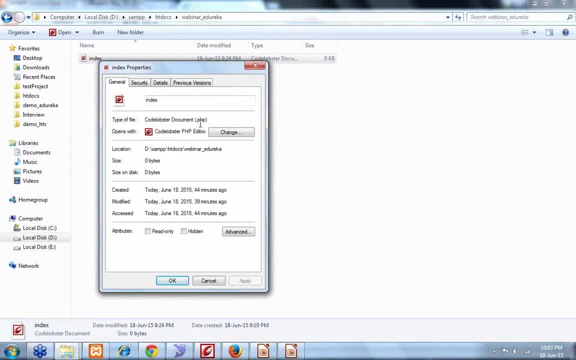 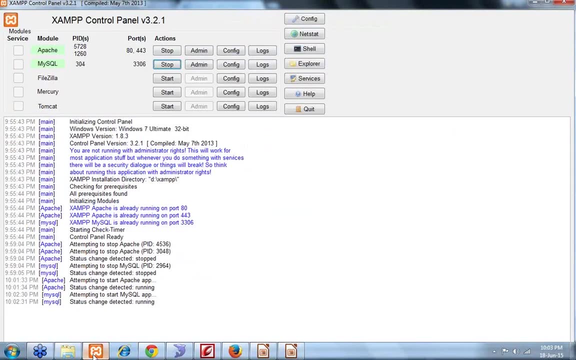 Dot PHP type of file. It is dot PHP file, So PID- you don't need to worry about PID. what PID means This is personal ID that is provided by the system. that is for internal use. You don't have to worry about PID. 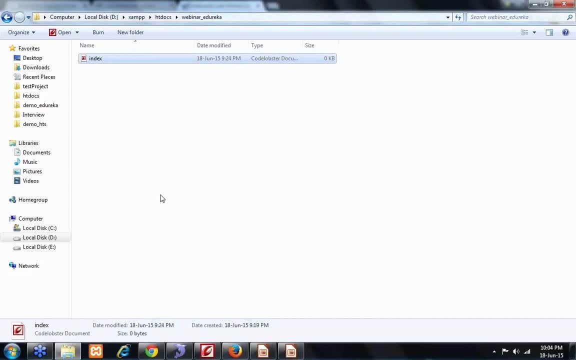 So here I created a file called index dot PHP. So every PHP file would be having an extension dot PHP. Otherwise it will not accept or it will not run PHP She cut that. you need to confirm with azureka, that course, how they provide. 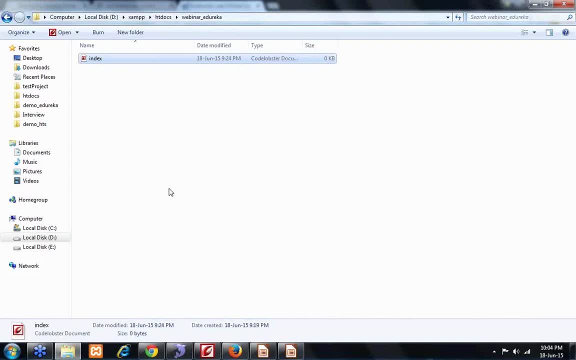 I think it would be with frameworks. I think it would be so. MVC is nothing, but it's a design pattern. It's a structure that we follow to develop our website. If you are aware of PHP, you can easily work with any framework, any MVC framework. 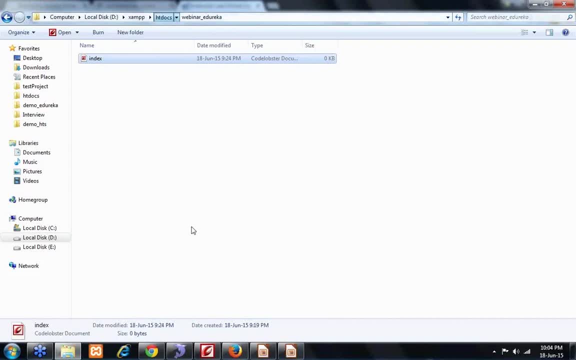 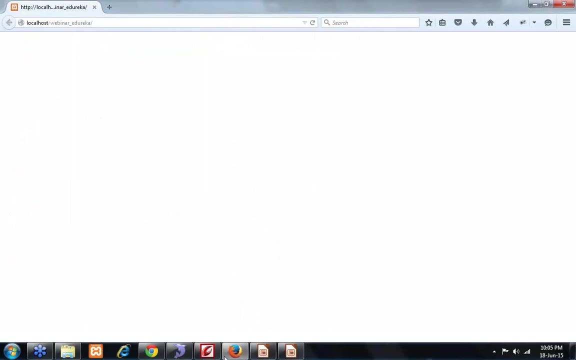 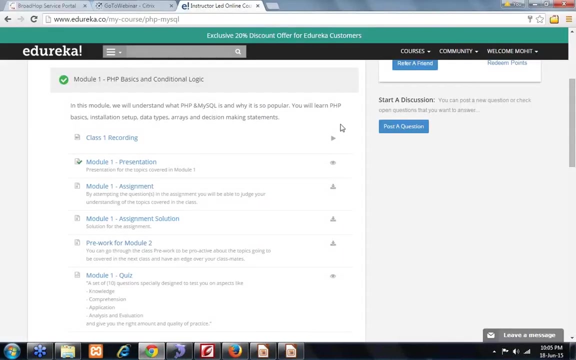 So I have created a file index dot PHP. I have created a folder in XAMPP XT dogs webinar underscore azureka, And in this folder I'll be keeping my file and my file name is net dot PHP. Okay, Shikha, on wwwazurekacom you need when you will register with azureka. 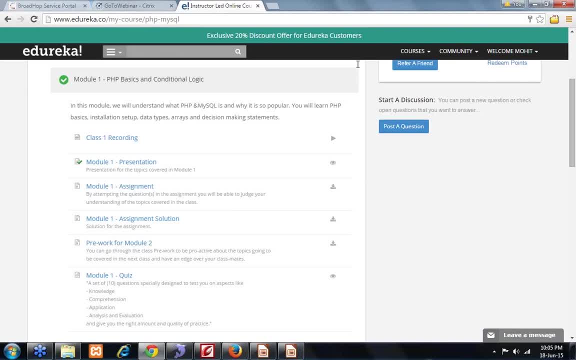 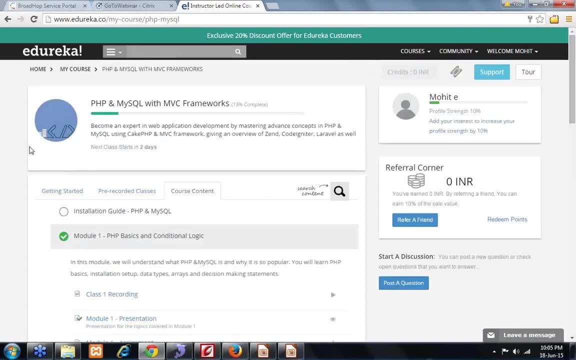 You will get your login credentials, You will get a link for login, You will log in and once you log in, you will be able to see your courses, my courses, and in that course, this PHP magical in my messy framework would be there. And then there would be. 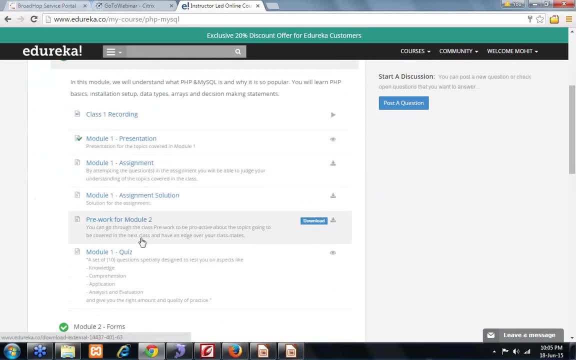 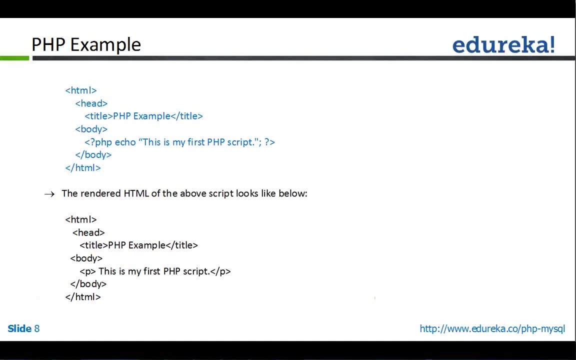 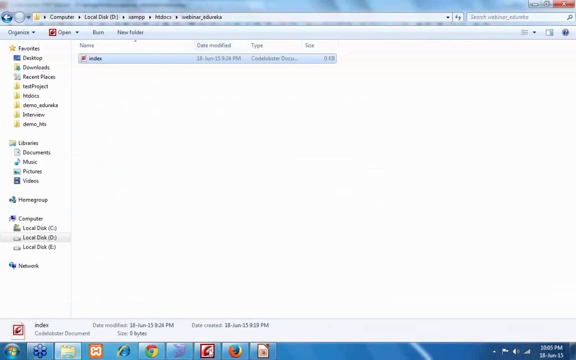 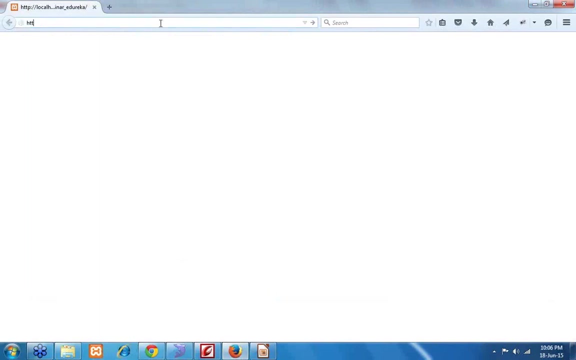 Basic recording, presentation assignment and lot of things for that particular Course. Okay, So here I have what I have done. I have created a file, index dot PHP. Now On my system, once my mysql server and Apache server started, I will write HTTP. 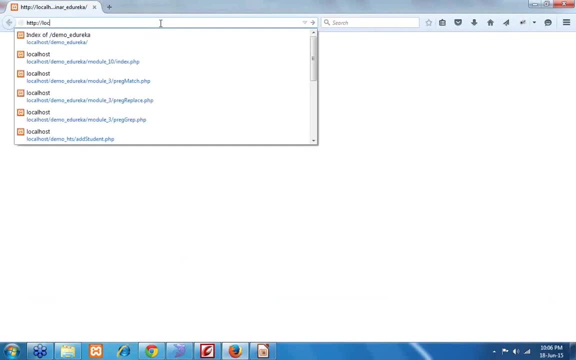 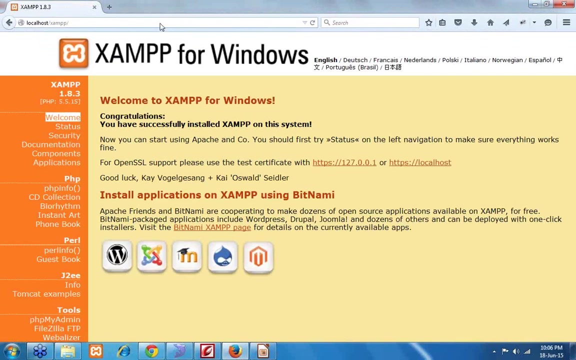 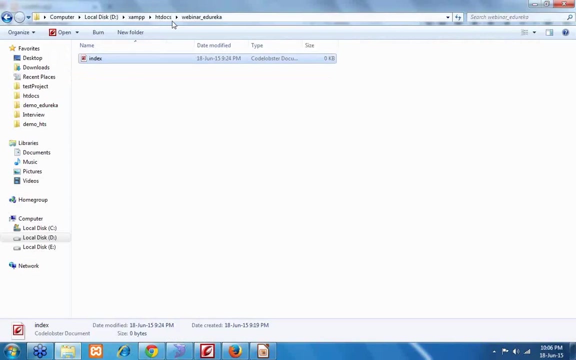 This is for local system only if we are going to use Xampp server local. So once you write localhost, You get a screen like this. So if you get the screen, this simply means that your PHP is installed Successfully. Now how you will access your folder that I created in stdocs. 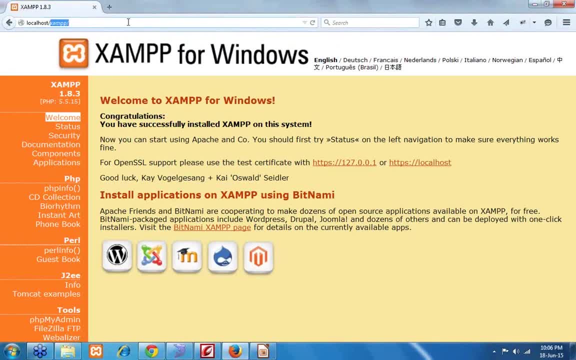 So for that you don't have to provide the complete, complete path after localhost. You will simply write your Folder name and file name. That's it. Now you will to run your file. Now. I haven't written anything in this file. 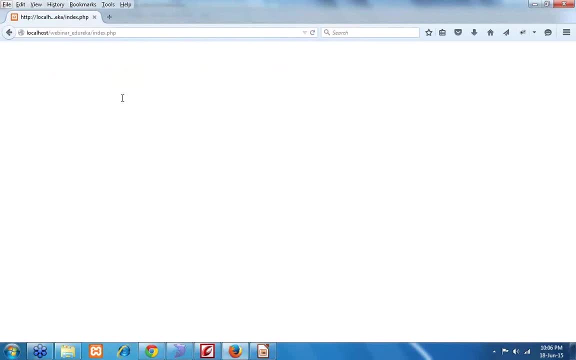 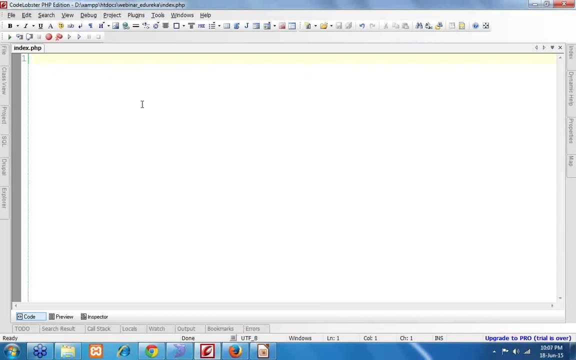 That's why you're you are seeing the blank page. Now let's try to understand How PHP works. So PHP basically starts with the tag and ends with a closing tag. So PHP starts with less than question mark PHP. So this is the opening tag of PHP and question mark greater than this is the closing tag of PHP. 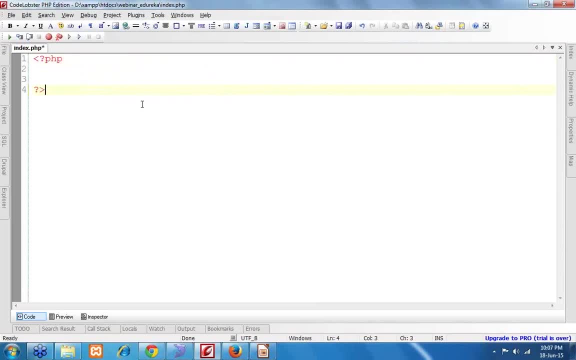 So, whatever you write, you want to execute using PHP. You will be creating a dot PHP file and inside that file You will be creating opening PHP tag and closing PHP tag, And inside that, whatever you will write, I'm writing print. This is my 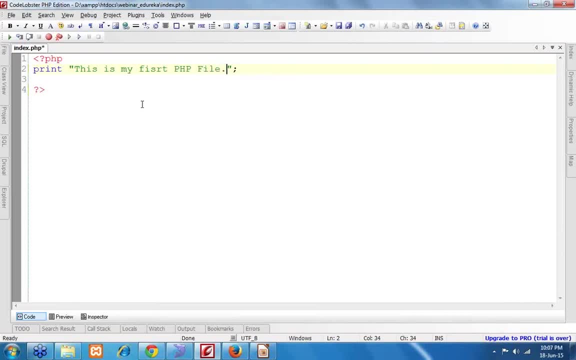 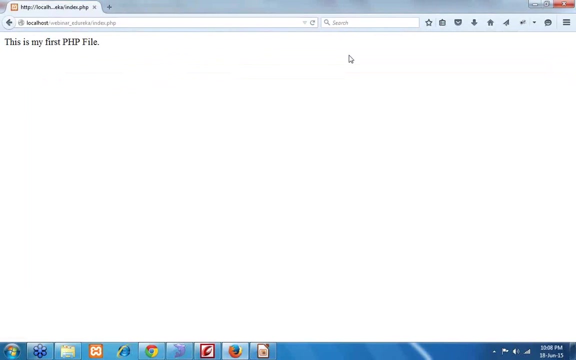 First PHP file. And now you don't have to do much, You simply have to go to your web server and simply refresh it. So here is the result: When you refresh, It prints the result. It prints this line, that particular statement. 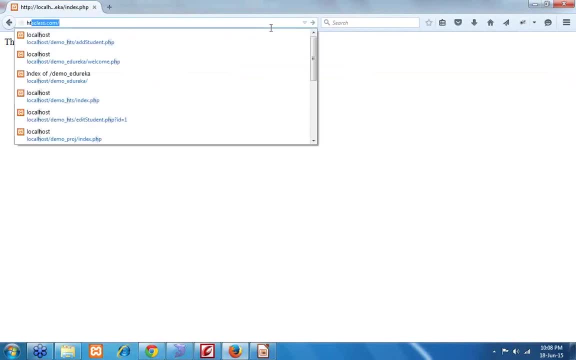 Yes, open that. you need to type in URL, HTTP, Local host, And then slash, then your folder, project folder and then file name. That's it. See, retic your PNPHP. We don't only print. we can do a lot of stuff there that you will see further that we cannot do with HTML. 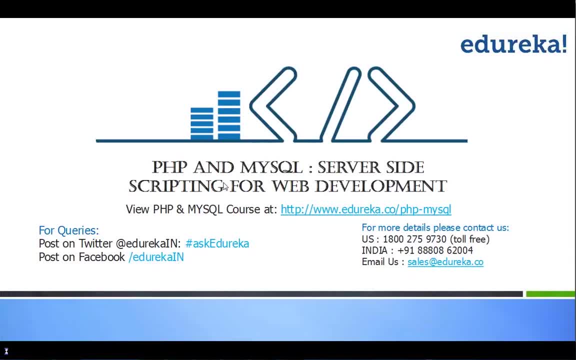 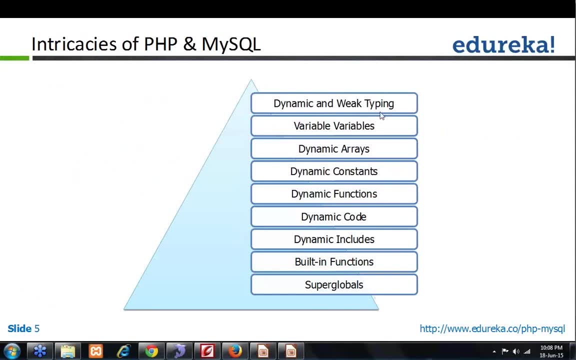 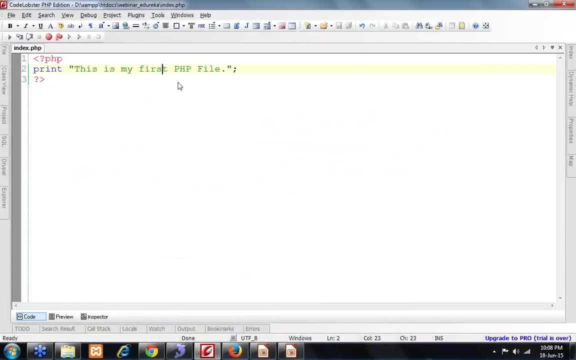 So let's go further and then we will discuss. So here are some of the characteristics that we missed and I will be discussing now: dynamic and web type, web typing. So dynamic, you have seen that whatever I change and, moreover, I can interact with databases. 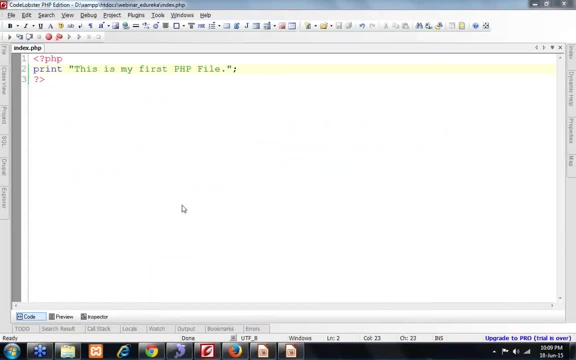 That is the best Dynamic city with PHP, but it is dynamic. It can respond to a request. Yeah, we shouldn't. you can. Ajay Kumar, you can open with You are sorry, port number as well. No issues. So this is my first PHP file. 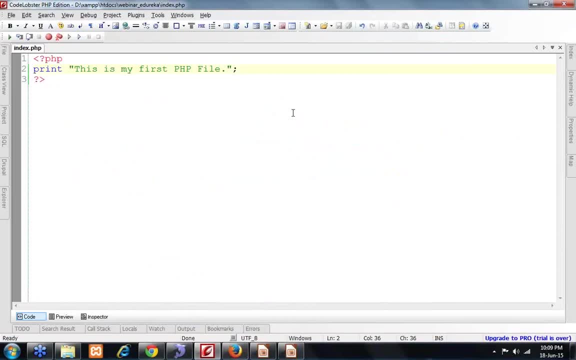 This is my first line that I printed in PHP. Now, if we want to create a variable in PHP, So variable is a thing that stores a particular value and that can be changed as per our requirement. That's why it is called variable. So in PHP, in cc++ like- unlike CNC plus plus in PHP. 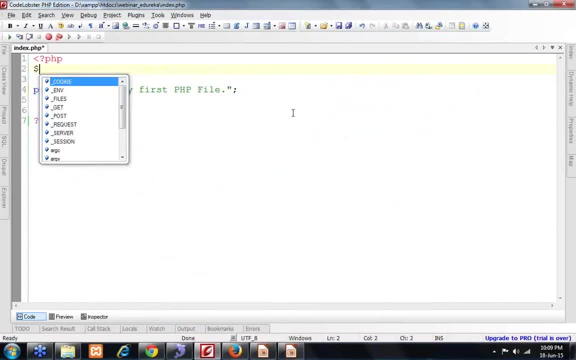 The variable is created with a dollar sign. first dollar, Like where, or I would write my first where and it can be this line that I have written that I printed. Then, instead of printing simply line, I will print my variable here: Dollar filter. 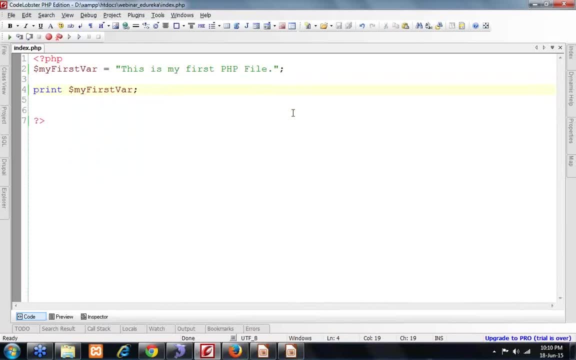 Where, yes, should. the PHP is case-sensitive, like see. it is similar, So syntax is almost similar to see, if you are aware of see. now, see, I have. initially I was printing my query, printing my string. Now what I'm doing? I'm writing the string in a variable. 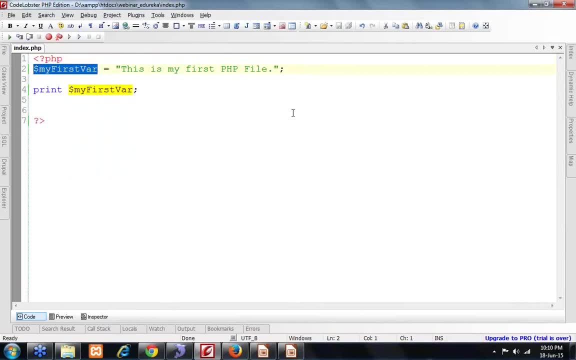 I'm storing this thing in A variable. Now this variable would be stored in the tree and now, instead of writing the same, I'm printing this variable Here. I will change a bit. Yes, they wish. data types are similar to see and place to see: plus, plus. 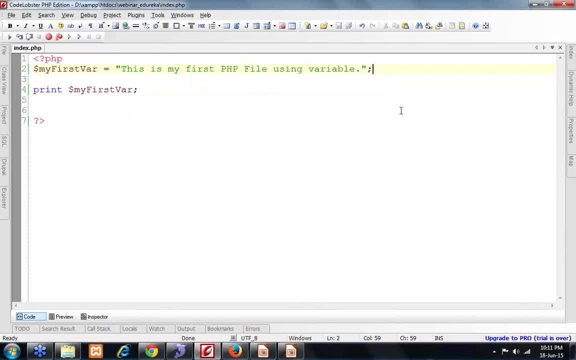 They are a data types in PHP, like a string, number, flow, decimal. Everything is there in PHP as there are in C or C++. Yes, Nail, basically you don't have to that I'm going to discuss further, Let me. let me complete this. 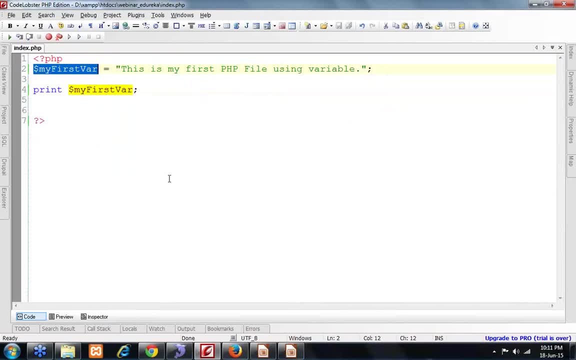 So I have Himika. There is no direct pointer concept in PHP. Well, there is, but we don't use it. Yes, so we go in order to define a variable in PHP. You cannot Remove this dollar sign. It would be there. 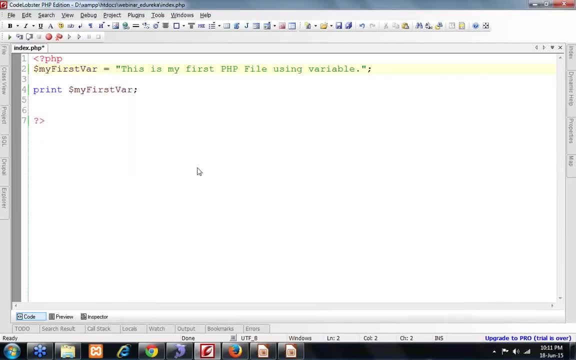 It is mandatory to have a dollar sign before a variable name. Okay, so you will take the brief at the last, no issues? So I have created a variable and saved my string into this variable and I'm printing it So when I refresh my browser. so this is my first PHP file using variable. 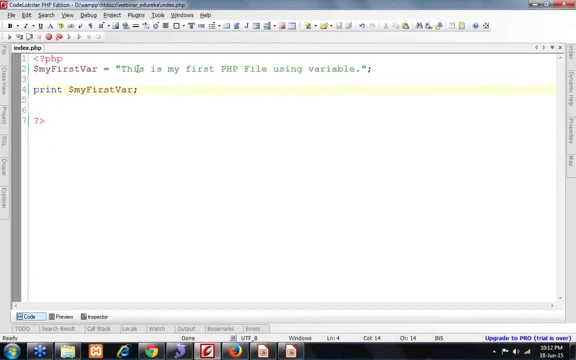 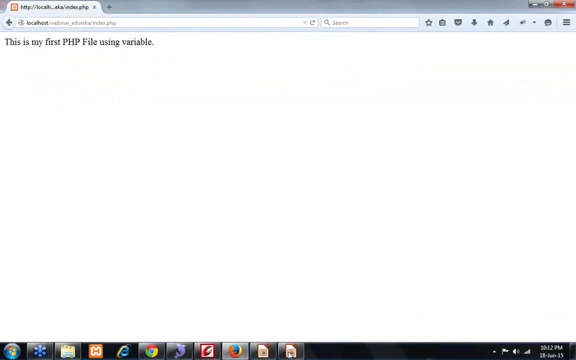 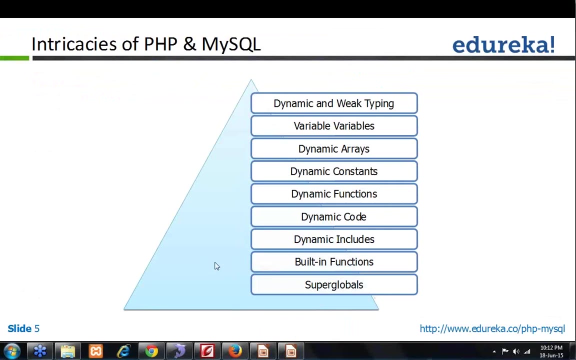 It got printed. So I created a variable, Assigned a value to that variable and I have printed it So you are able to see it on the browser. So this is the simplicity of PHP. You simply write your statements and execute it. You don't have to compile to any other stuff. 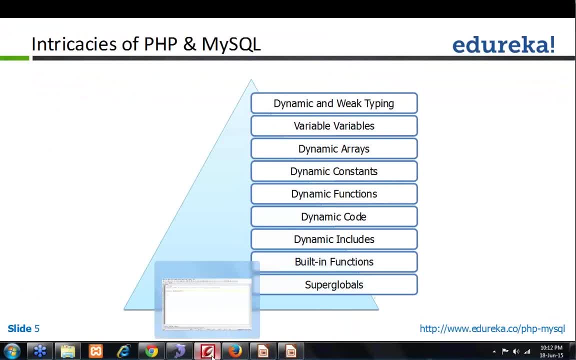 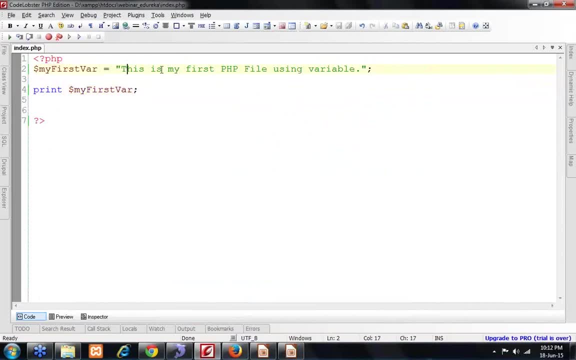 So you can see dynamic and weak typing. So here you can see: while assigning a variable, While creating a variable, while assigning a string to a variable. I didn't give any data type for this particular variable, Shweta. Yes, cold lobster is a ID for PHP. 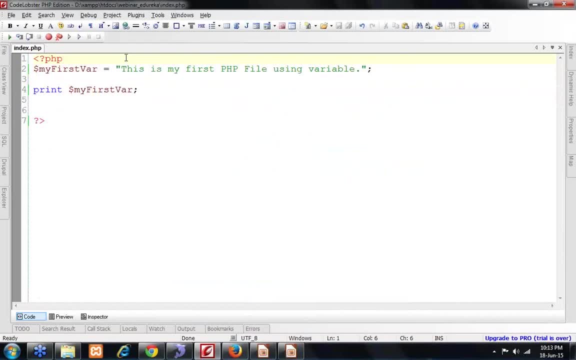 You can use it in notepad. Even there is not a restriction anywhere. You can write PHP code where you are comfortable. Just just search for PHP IDs and you will find a lot of options. So this is how I can print PHP, So I don't have to provide any type. 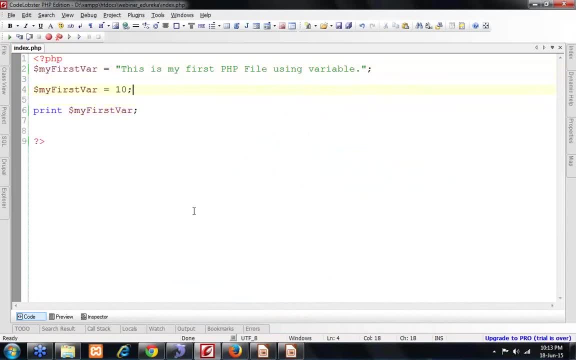 See, here I have given a string. If I assign a number to it, it will be taken. I don't have to define any data type, So it will print 10.. Now it will overwrite the previous value and it will print 10.. 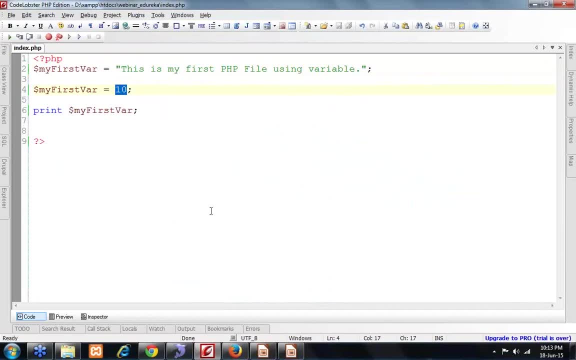 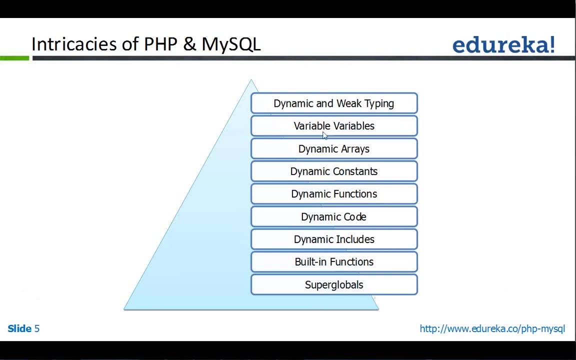 So no data type is required To define in PHP. It is for giving language. That's why it is called weak typing dynamic and weak typing variable variables, So we can have variable variables. a variable can further Be A variable stored in a variable dynamic arrays. 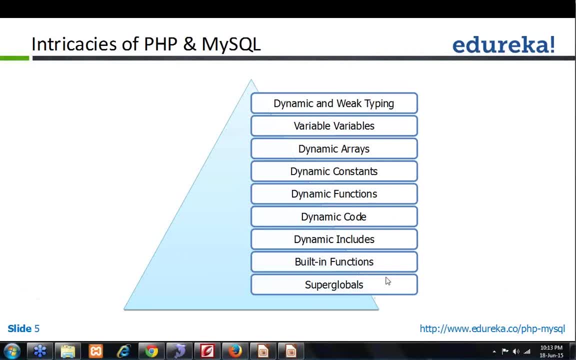 So errors can be dynamic, dynamic, constant. dynamic functions: We can create functions and reuse them wherever we want. dynamic code: We can write dynamic codes. dynamic includes: we can write a file and we can include that file in another file. So that is Kyle. dynamic include then built-in functions. lot of built-in functions are there in PHP that we can directly use and do our job. 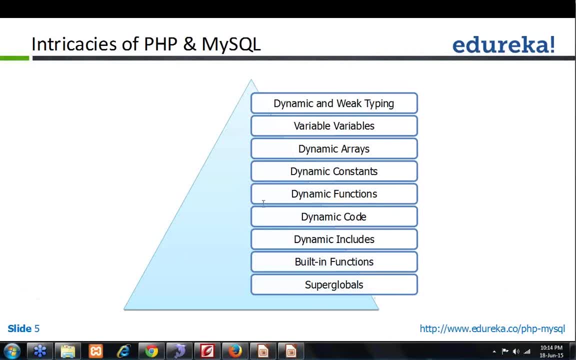 Not everything We have to do from Scratch, like combining two strings. that can be done directly. breaking a string into arrays- that can be done using built-in functions, Super Globals- lot of internal super Globals- are already provided into PHP that make your PHP development very easy. 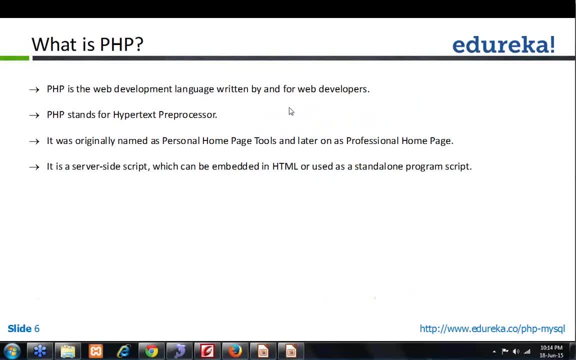 So here, what is PHP? We have already discussed that PHP is a web development language, That is for web developers. PHP stands for Hypertext preprocessor, because Why it is called hypertext preprocessor? hypertext is basically used for HTML, So what happens when we write any statement in PHP, like I have written the statement into PHP. 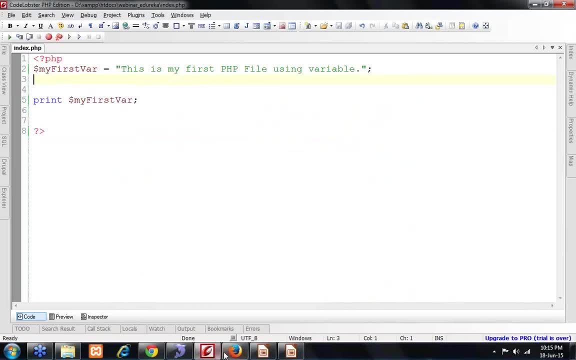 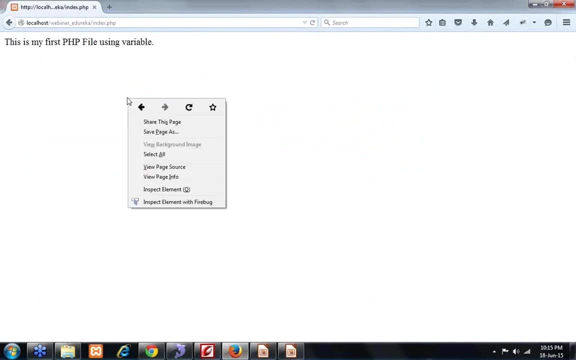 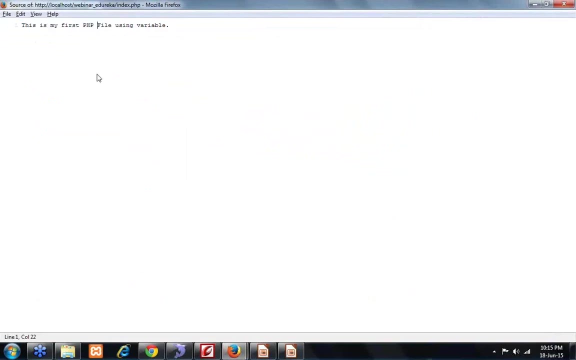 Let's move this for now. And when you execute on browser, you got the result. And when you see the source- You pay source- You can see that you are able to see this text only So it is converted to HTML. So whenever we execute something into PHP, it gets converted to HTML internally when it comes to the browser. 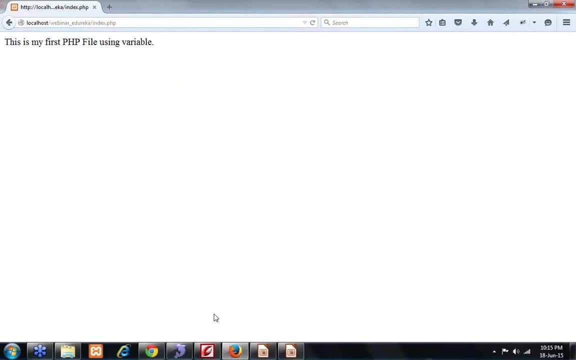 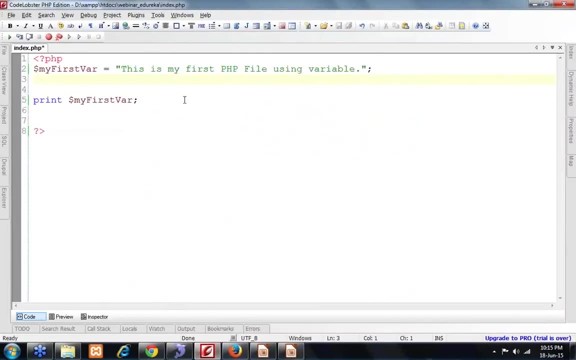 We see the HTML, static HTML, Mitesh arrays we can define in PHP. So if you want to define an array, this is simple thing. So array would be: $air is equal to Array, And then you will be giving your values: 1, 2, 3, whatever you want to give. 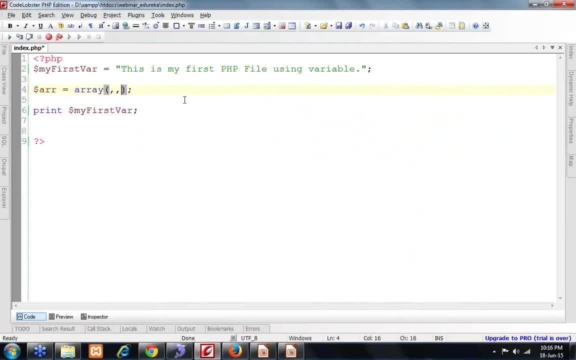 Or even you can give strings if you like, Like 1., 2, like that. So Your question is that. your question is, if there is an error, how you will show it. So let me skip this semicolon, So every PHP statement ends with the semicolon. 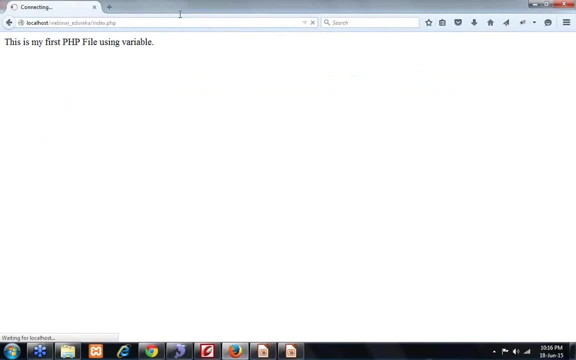 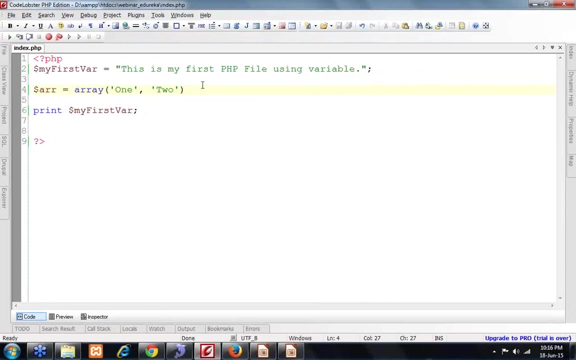 Let me skip this semicolon. Let's refer the screen Now. you simply see the error, syntax error, unexpected print in line number 6.. So line number 6? because why it is saying line number 6? because semicolon. let us know that this particular statement is ended here. 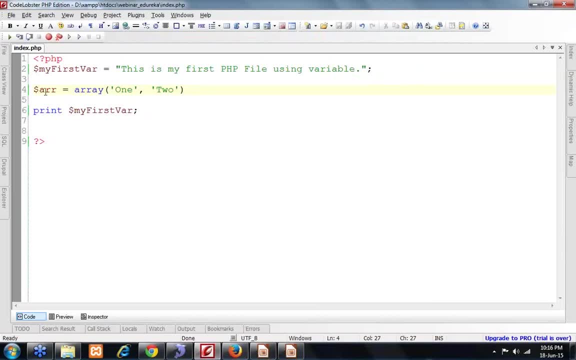 If, if there is no semicolon, it will continue and it will see that Two statements cannot be written together. So two statements cannot be written on a single line. There should be semi semicolon separating them. So here it is saying it is expecting that it is continued, but it is not continued. actually, 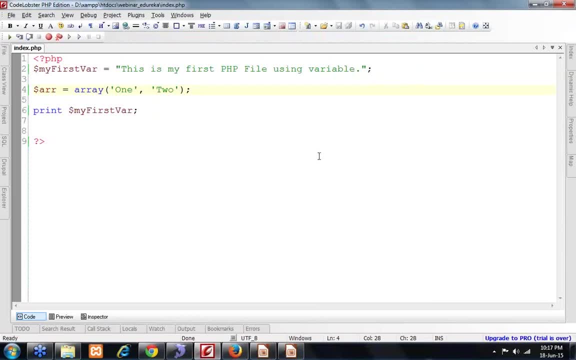 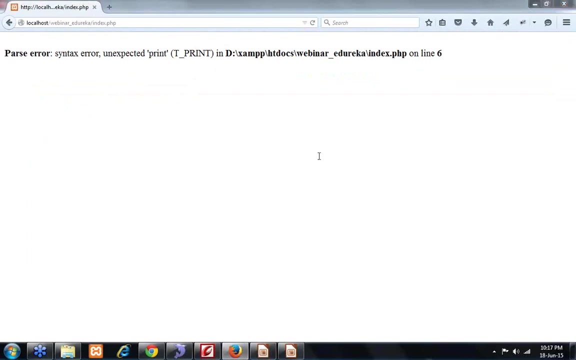 So we have to put semicolon to let us know that Thus statement is ended here. So in PHP it is not very difficult to get the error. just change the syntax, just provide a wrong syntax, and you will find the line Name, even that where you are having a problem. 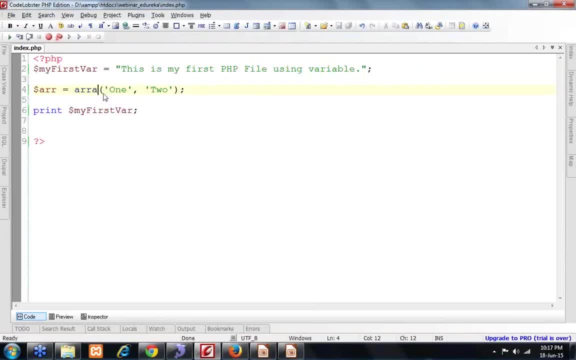 For example, if I put a double array rather than array Called one defined function, a double array on line number 4.. So this is line number 4.. So how simple it is to get errors in PHP and troubleshoot them. Divish PHP language is not compiled. 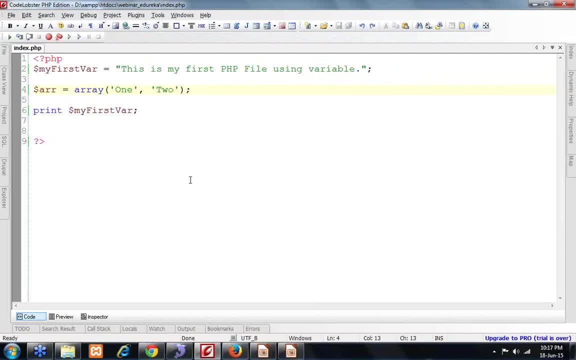 So you don't need any compiler Or writing main or something else. Shruti array can have multiple data types in PHP, So you can have like that. So this again, this is an array array. array can have multiple data types. So it is up to you that what value you want to provide to an array. 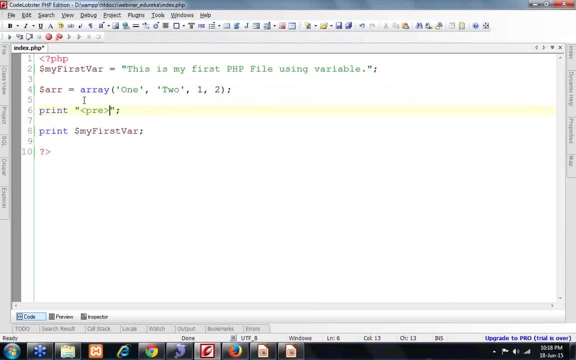 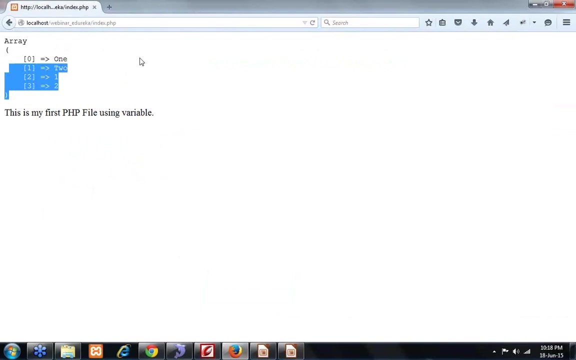 We can even print an array. So in PHP there is a function called print underscore R And your array name: Yes, nail, PHP is object oriented, So here you can see your array. array is having four values with subscript: 0, 1, 2 and 3.. 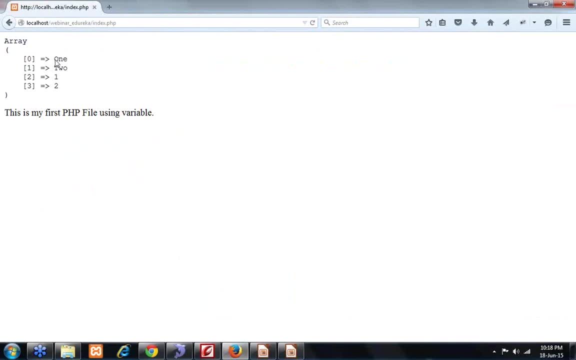 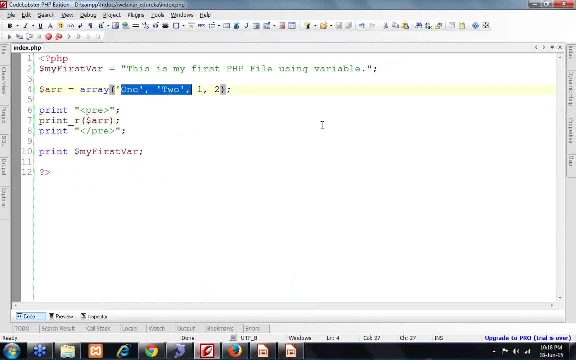 And values are 1- 2 and 1, 2, 1, 2 and then numeric 1- 2.. So what I have done here, I've created an array with four variables or different data types. So it is possible in PHP. 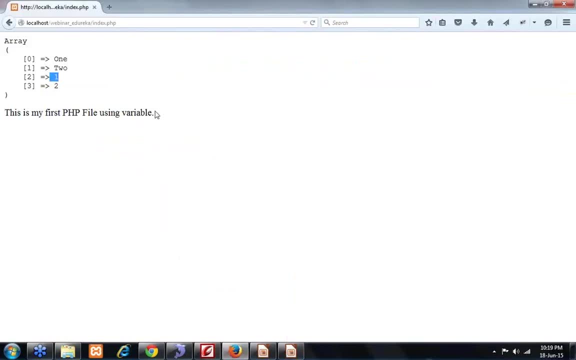 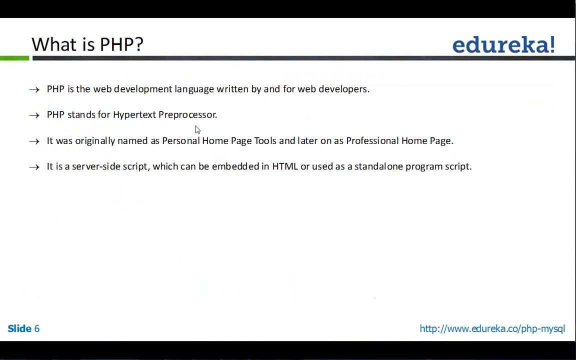 There is not an issue And, moreover, you are able to see this variable get printed. So PHP stands for hypertext preprocessor, because It is convert. once There is a response comes from the Apache, It is converted to HTML and we can view it on the browser. 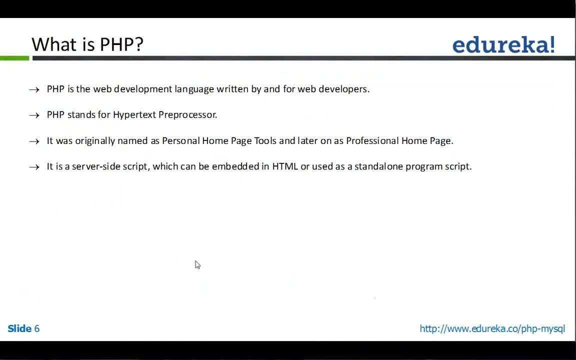 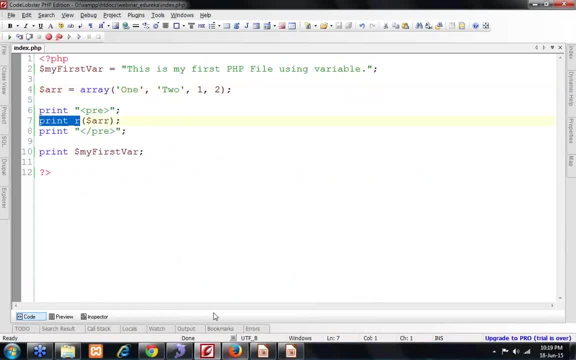 So source would be in HTML only. So Print underscore. R is a function In PHP to basically explain your array. It can open up your array and you are able to see it on the browser. That's it. It is used for testing purpose only. 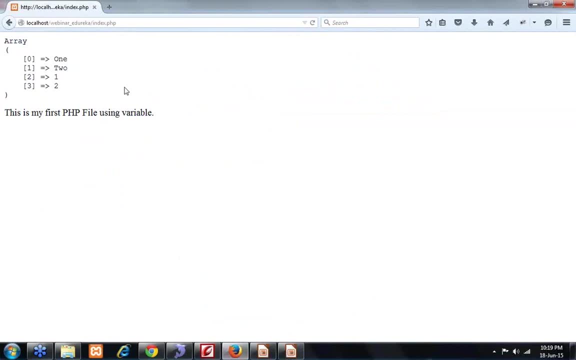 You won't be using it for clients Or it means it is not. It won't be used over your web portals. It would be only for testing purpose If you are getting some issue in your array and you want to print your annual on the browser. 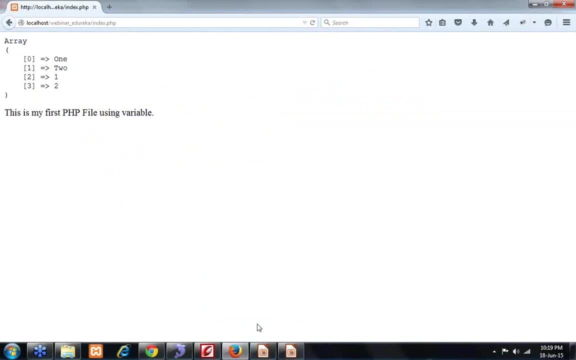 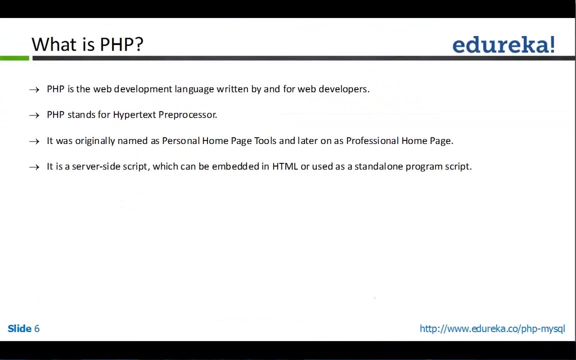 You can simply simply use print underscore R and provide your array name, and array would be printed on the browser. This is for testing purpose only. So when PHP came into the market, its name was personal home page. later on, when it started using into into the web development professionally, 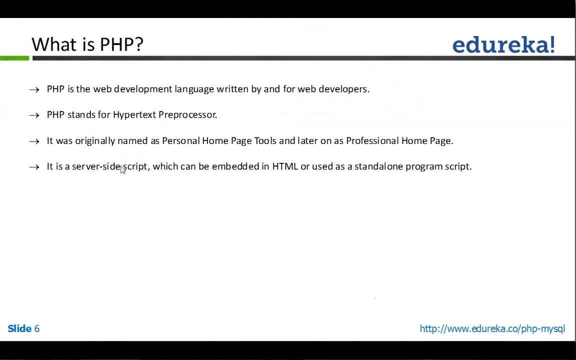 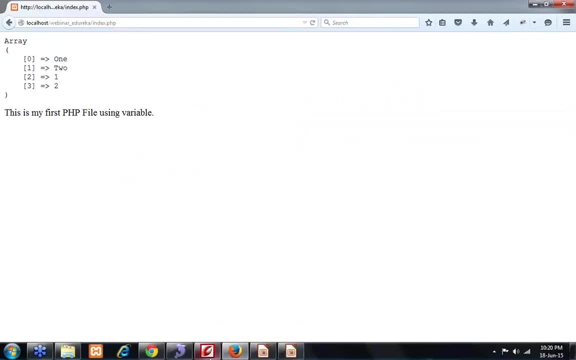 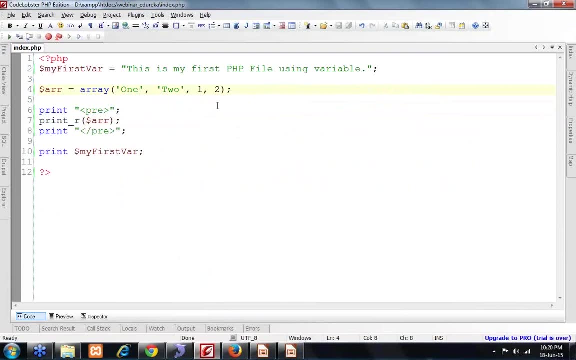 It got the name professional home page, So it is a server-side programming that can be embedded into HTML as well. Yes, Reshma, We can use multi-dimensional array with PHP as well. There is no time issue, any kind of dimension like CC++. 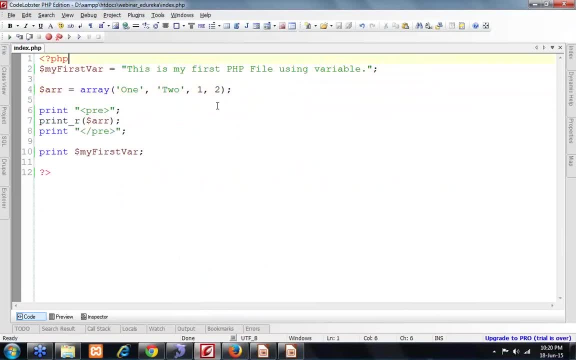 Okay. so your question is how we can comment lines. So commenting: there is two way commenting in PHP: one with: if you want single line comments, You will simply write double slash and then your comment. If you want to write multi-line comments, You will be simply writing. 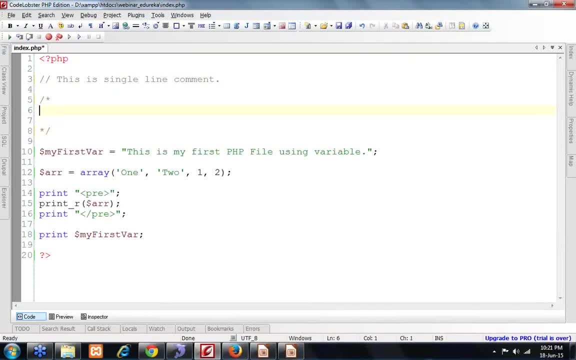 Slash star and star slash, sorry, And here you can write. So these are two types of comments in PHP. Above one is single line comment and below one is multi-line comment. So single line is by using double slash or you can simply use hash. both are okay. 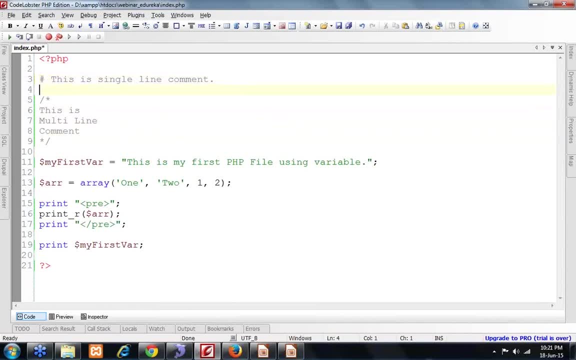 Yes, So we could- is similar to CC++, not an issue. And moreover, we can also use PHP with HTML as well. So here I can write- let me have some HTML code Then how. I will show you that, how HTML can be used with PHP. 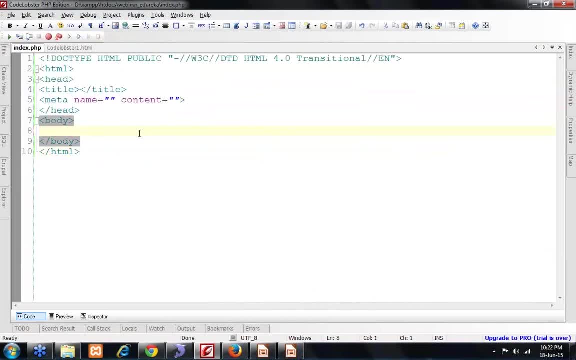 So this is my HTML And if I want to use it- PHP inside HTML- the simple thing I have to do I have to write PHP tag inside that tag. You will simply write your code. Simply, you will write PHP tag inside that, those tags. 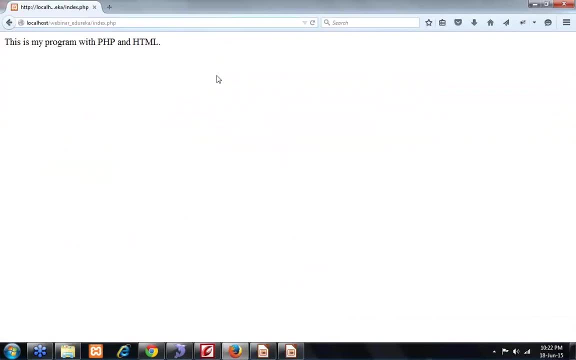 You can simply write your code. So here it is. when you see the source here, You can see that PHP code is converted to HTML. So it is inside HTML. There is not an issue. So Shruti server-side programming means that interacts with the server server like in your body. 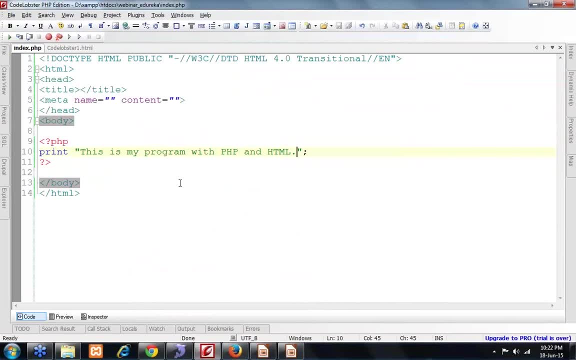 Your mind is your server. Whatever you have to perform, you talk to your mind right, And your mind returns the response. and that response you do. For example, if I'm speaking something even that is coming from my mind, I'm trying out. 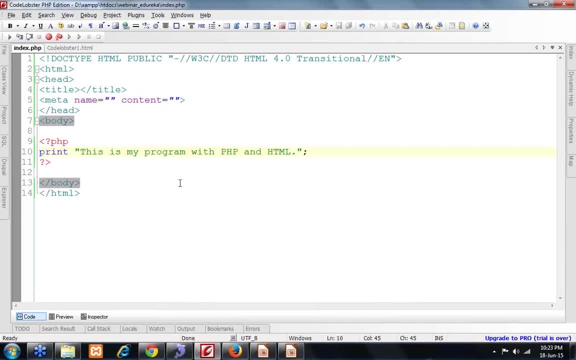 I'm allowing my consciousness To speak something, then that instruction is going to my mind and mind is interpreting what I want to say and that particular thing is coming from my mouth. So my mind is my server in my body, the same way You can. you can say: Apache is a mind of PHP programming. 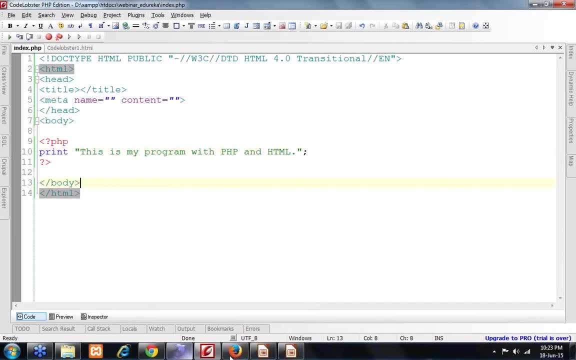 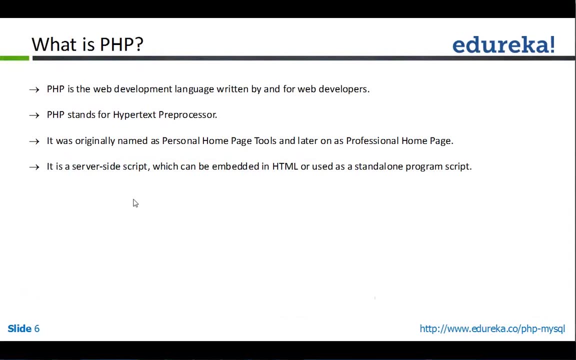 Loops will be discussing, Don't worry. So let me go through the session. A lot of slides are there. PHP can interact with JS or Angularjs. that is not an issue, because data client side and this is server side. So let's first do with it and we'll see how it can interact with JS or Angularjs. 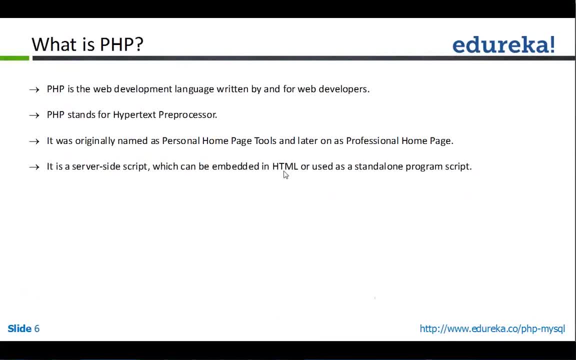 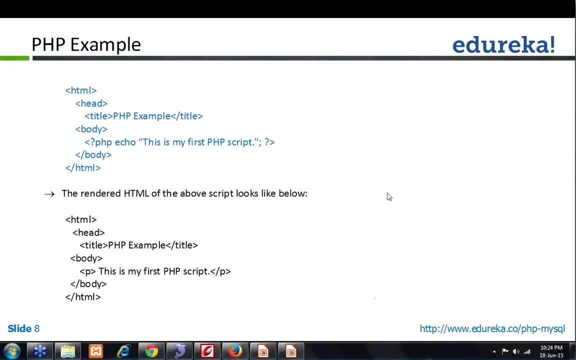 So here we have seen that how PHP can interact with HTML can be written into HTML or standalone- both ways PHP can be used. So this is the simple PHP example that we have just seen: that inside HTML We can write simple PHP tag and then we can write our code. 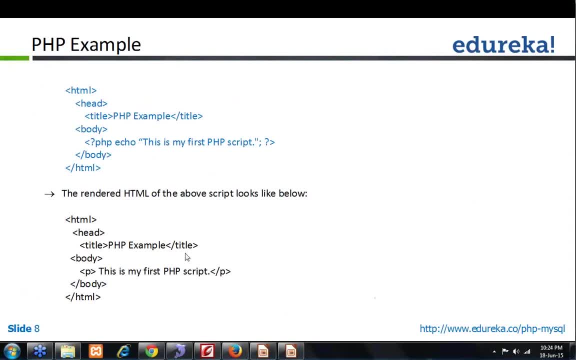 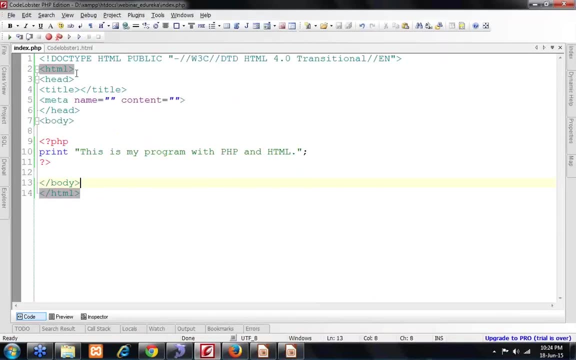 And what we get the result would will get in HTML only. Okay, Yeah, Neil, your question is how eco will work. eco and PHP, eco or print? We can use both in PHP, So it will print the same result, Don't worry. 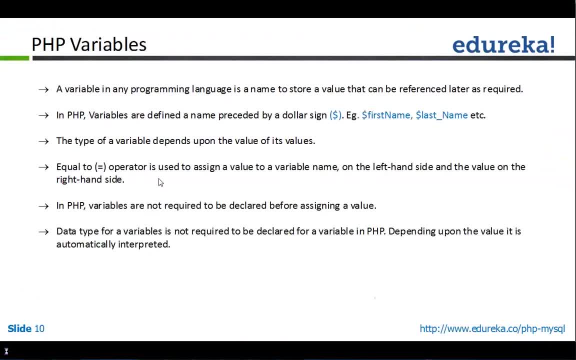 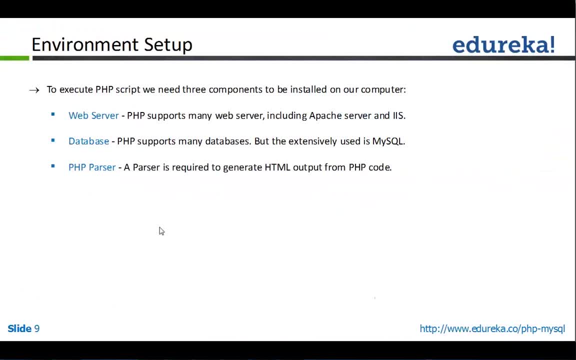 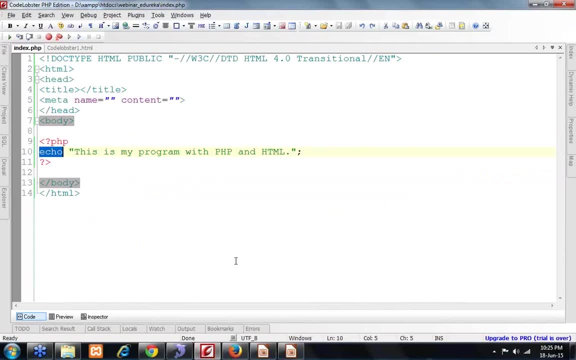 So this is the simple PHP example that we have seen practically So this slide. we have also have discussed regarding web server, That is, Apache, MySQL, and PHP that is required to do So. weak eco is also a function in PHP That can be used. 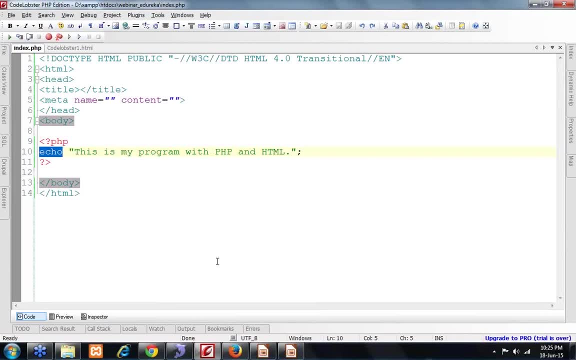 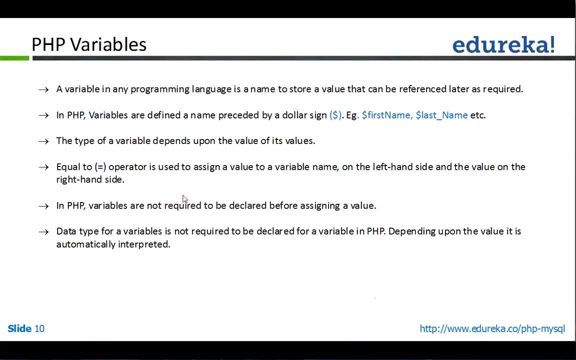 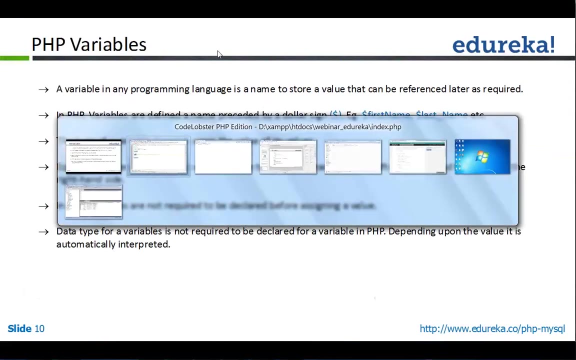 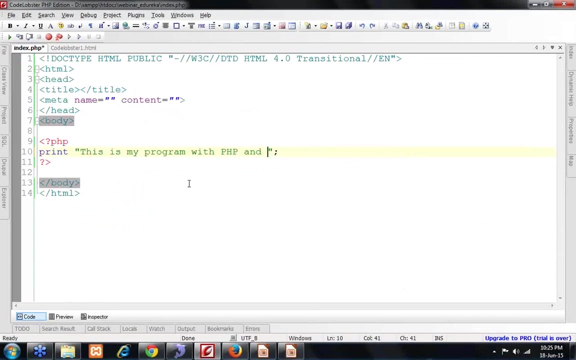 Along with our- you can say- alternative to print, Then PHP variables. So we have seen that A variable is any programming language, is a name to store a value that can be referenced later as required. So here you can see If we basically go back. 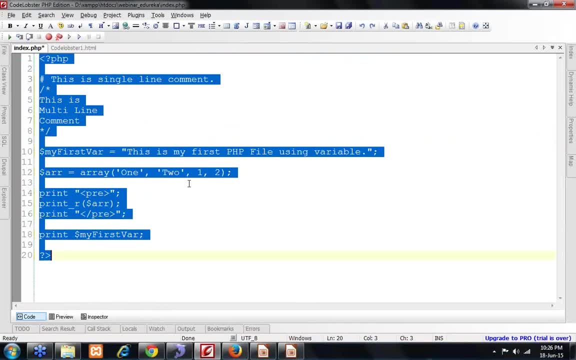 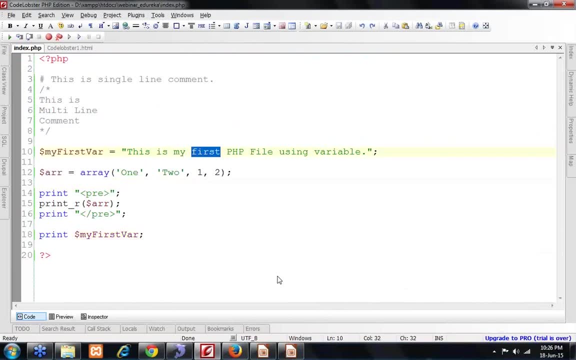 Shruti, that will see later that how we can relate PHP- PHP to MySQL. Please provide me some time and I will let you know. So here I have created a variable for my later use. Aditi Sorry, Adil. Yes, up where dump or pH printer and score are, can be used alternatively. 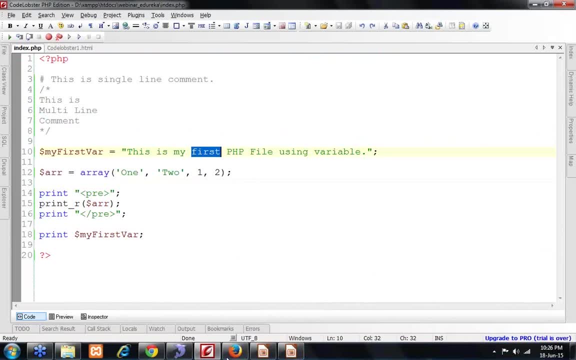 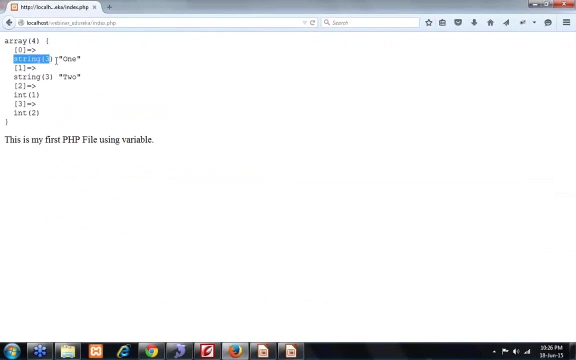 There is not an issue. So if you can use Where underscore dump, See here. but the only thing that you will get extra the type of the variable, type Of the array element. So it is string, This is string and this is integer and this is integer. 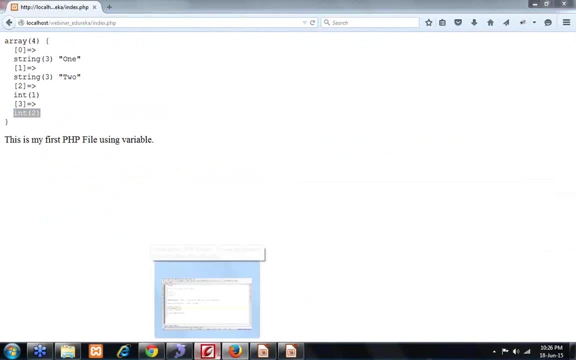 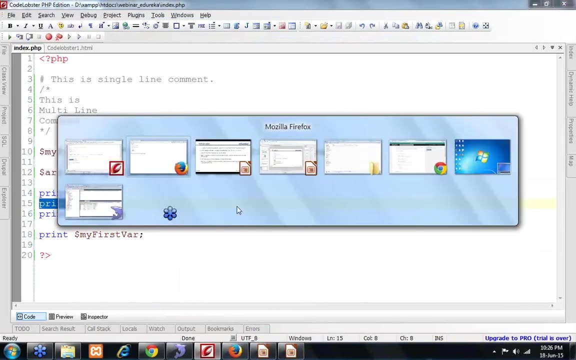 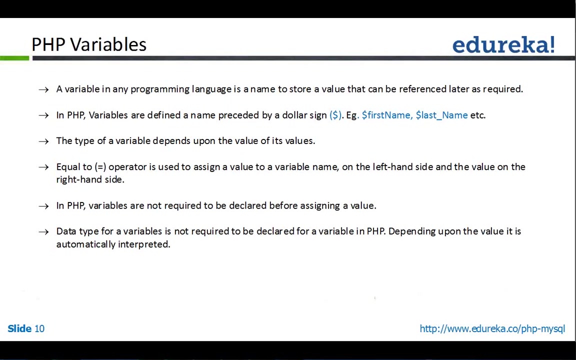 That's it. But if you simply want to see the array, you don't want the data types- You can use print underscore out Like this: So PHP in PHP or any programming language of variable is a name that can store multiple, that that can store a value. 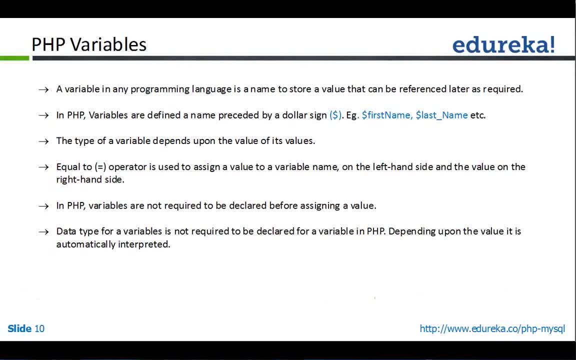 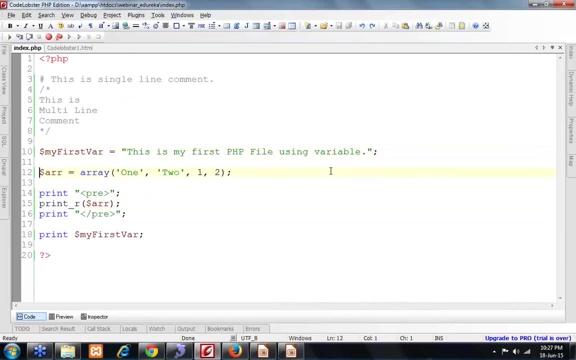 That can be referenced later as per our requirement. So a variable start with dollar. like dollar first name, dollar last name, that type of a variable depends on the value. So we have seen this thing earlier, that in PHP You simply assign the value and get printed. 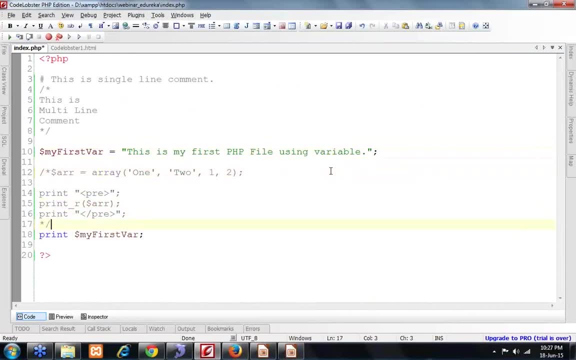 It will be used. You don't have to define any data type. Like I have shown you that my where take a has taken a string, then I will be taking It as integer, Or like this, and it will be converted to integer. So 20 will get printed. 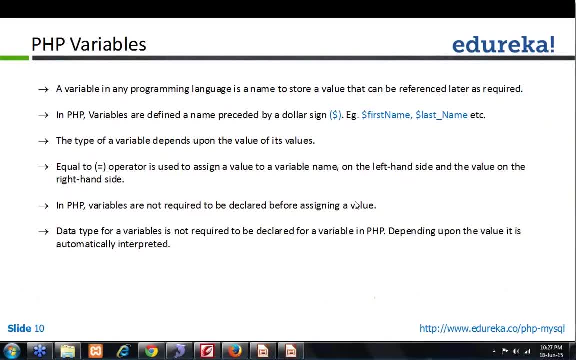 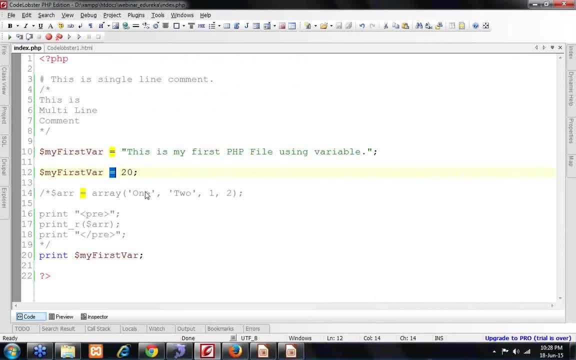 There's not an issue Equal to operators used to assign a value to a variable. So here you can see variable name equal to 20.. So this assignment operator is used to assign values to variable. in PHP, variable as not required to be declared before assigning value. 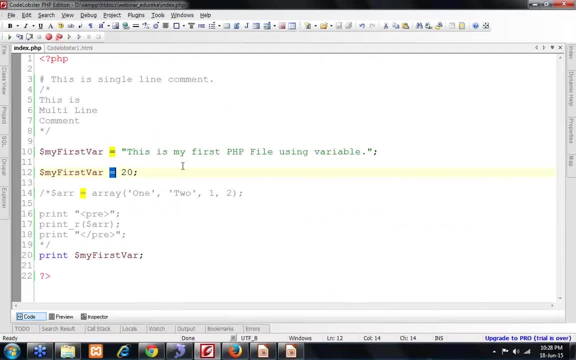 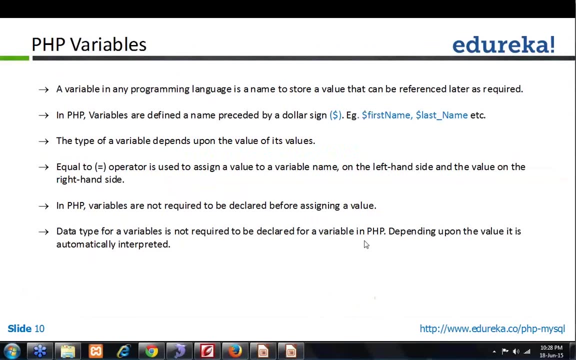 We don't have to declare a variable like we do in P, In C or C++ in order to assign it a value. Data type for a variable is not required to be declared for variable. in PHP that we have seen that we don't have to give any data type. 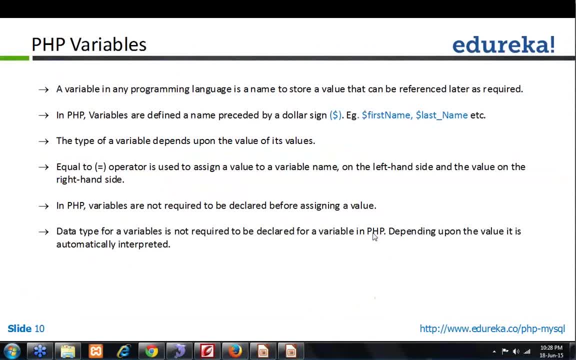 Whether it will be a string, It would be an error. It would be integer or decimal, depending upon the value, It is automatically interpreted. So this is the power of PHP: that it is weakly typed. It is bit forgiving language. You don't have to worry about data types and all. you simply give the value to your variable and use it. 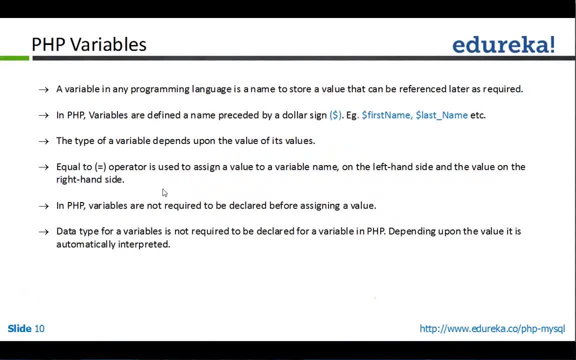 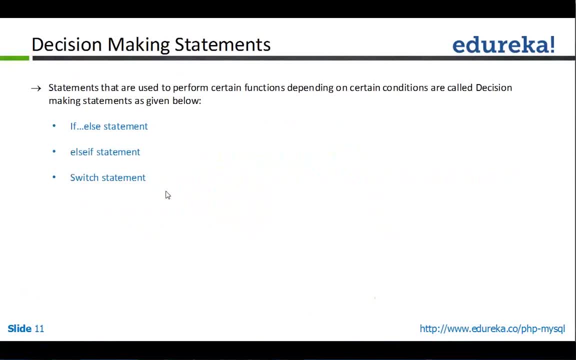 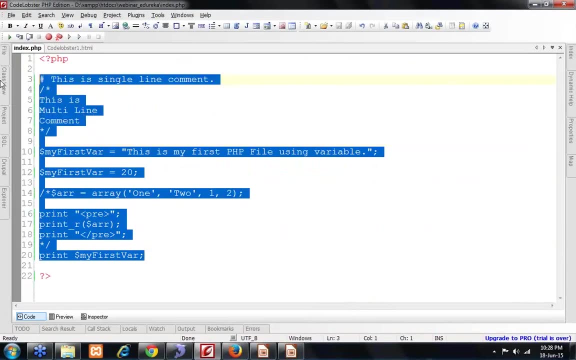 So that was all about some of the PHP variables, PHP basics. Now we'll see how we can make decisions, how we can make conditions into PHP. So this was my simple program. Now I will see that, how PHP can have conditions, For example. 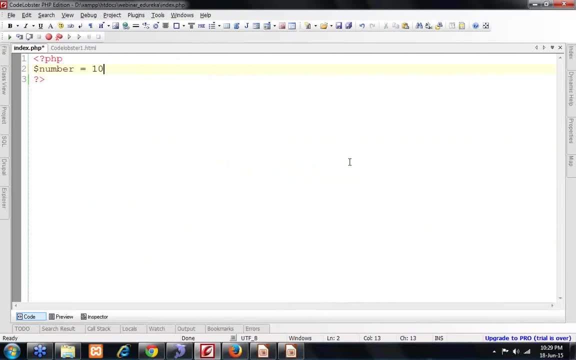 I'm having a number. dollar number is equal to 10.. Now I want to see, is this number no road? How I can check that. so in PHP there is a construct that is called if. So I will simply check if dollar number divided by. so we can divide in PHP using slash number: slash second number. 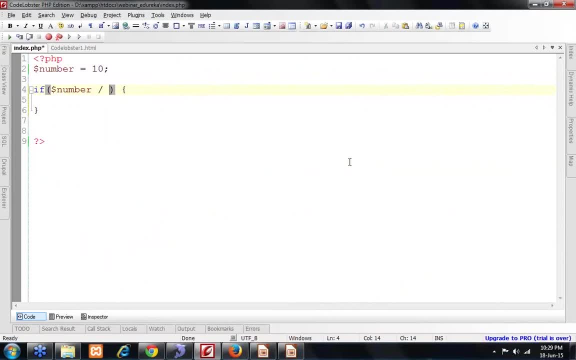 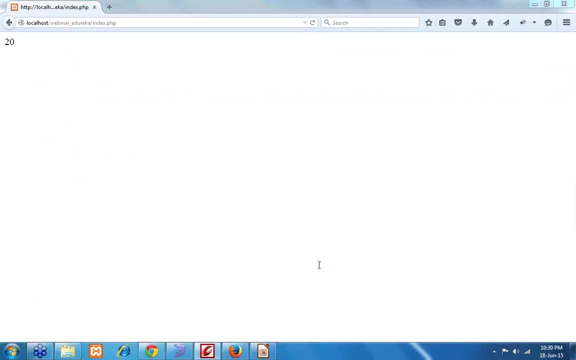 Then it would be a division. If dollar number divided by, or we can say it head up to, we will use modulus. So modulus is for you might be aware of plus if you had learnt mathematics. Yes, Shruti, We can also use switch statements. 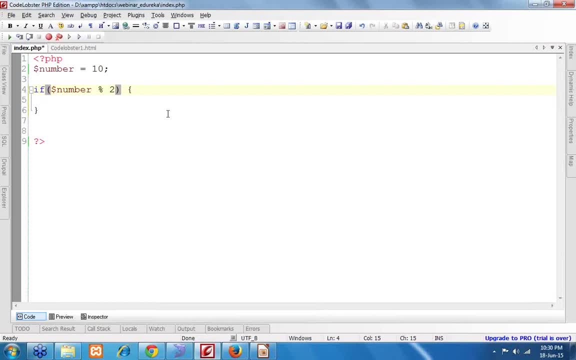 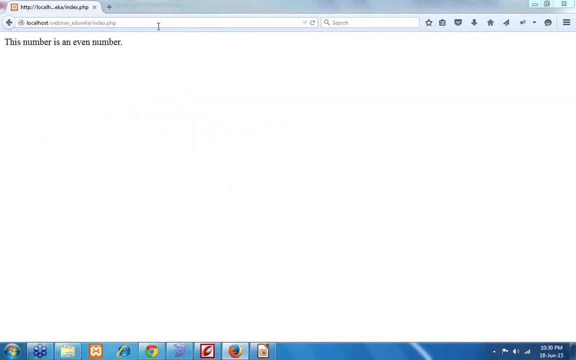 That is not an issue. We'll be seeing that, don't worry. by two equal Zero. if modulus of a number is equal to 0, then that number is even eco. This number is an even number. So whenever, when I refresh my browser, this number is an even number. 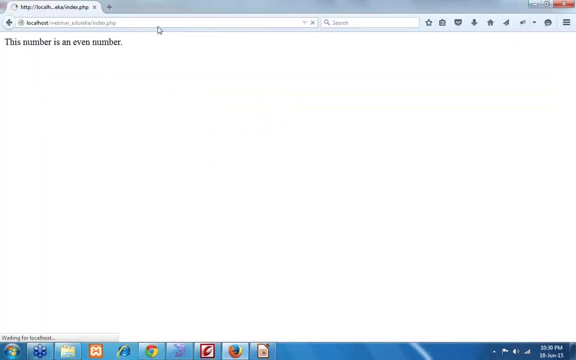 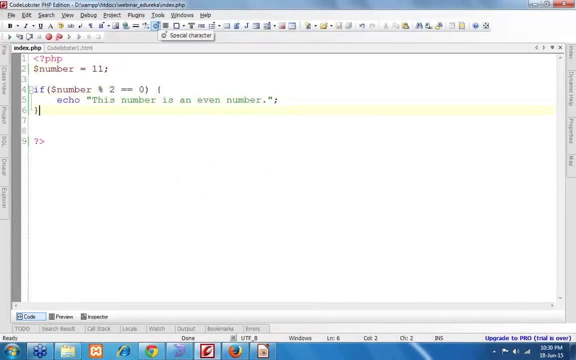 But if I make it 11. You won't see anything on the system. then in that case, even if it is not even number, We even then we might be willing to display the message. So for that we use else. if that is not possible, then something else else is possible. 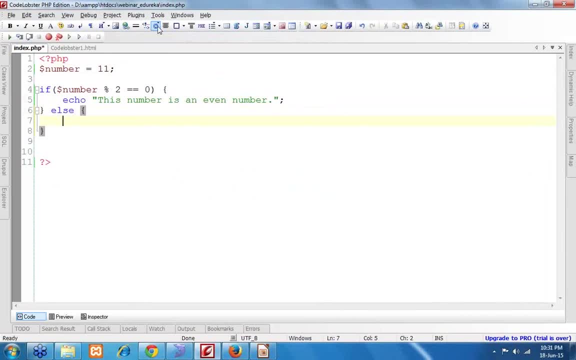 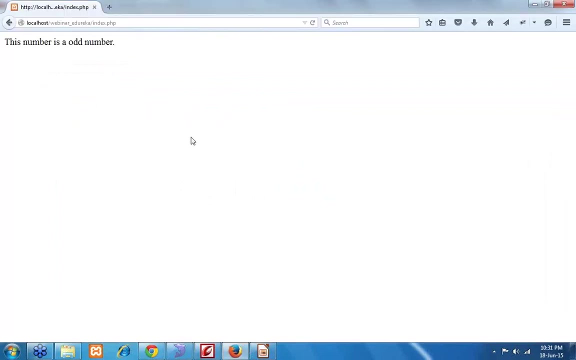 So if else block basically would be having conditions. If condition one is satisfied, It will go to if block, If not, then it will go to else block, else We can write. This number is n is a odd number. So if we give 11 it will print: this number is a odd number. 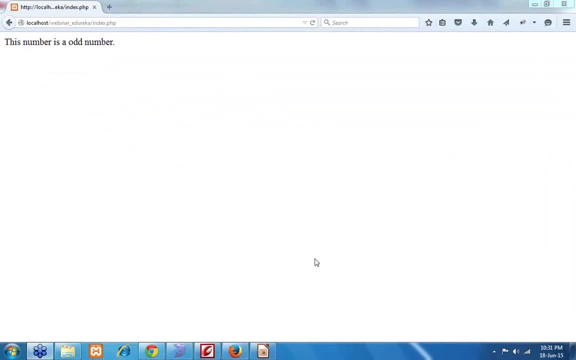 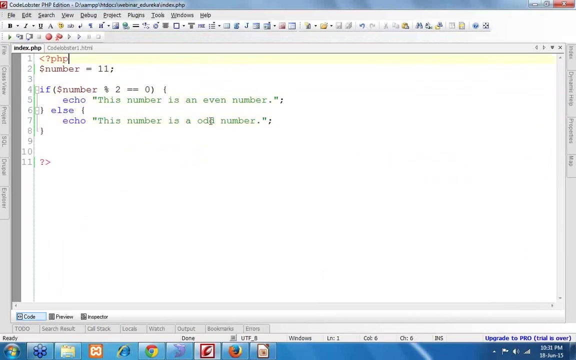 How to concatenate in. Okay, Yeah, Ajay. runtime simply means we'll be discussing the form, that how, using forms, We can give the dynamic values. Don't worry, We'll be seeing that concatenation. Yes, we can concatenate. concatenate two variables in PHP or two strings. 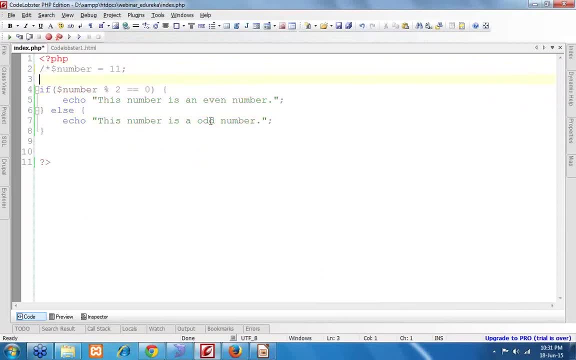 Let's see that. how we can do that. Yes, do I will be looking into. have patience, I will show you that- how we can use do while condition. So here I'm having str1 test, then str2 string. Now I want to concatenate it. 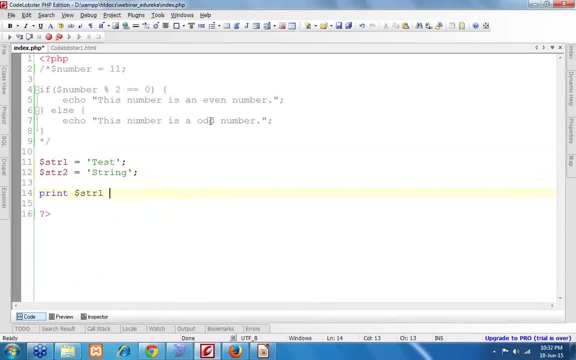 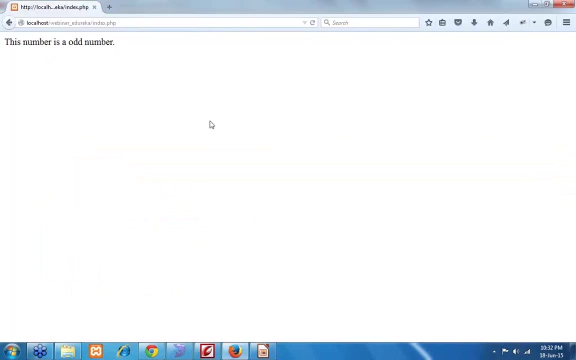 I'll do print dollar str1. dot is used for concatenation in PHP. I will add: Add a space and then I will write str2. have written string printer String one, then dot concatenated with the space, then again concatenated with string. to now: 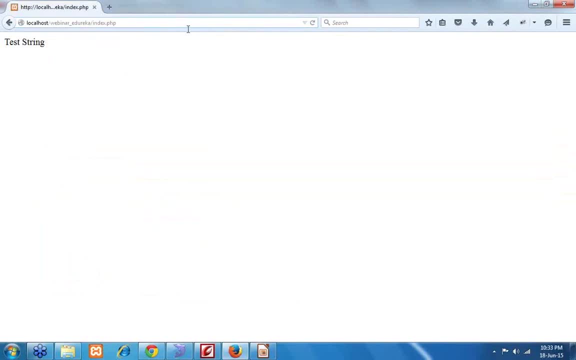 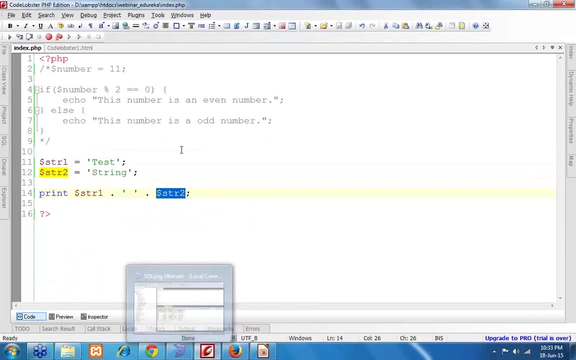 if we refresh test string so it is concatenated. So dot is used for concatenation in PHP. Okay, you want to print the number with the same, no issues. So, like an above method, now this concatenation. I will show you that how it will work. for the above example, this number, now we can concatenate here. 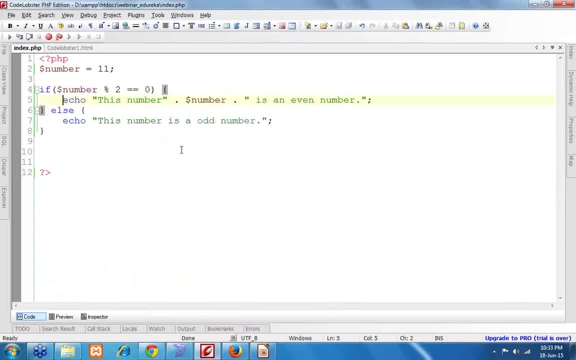 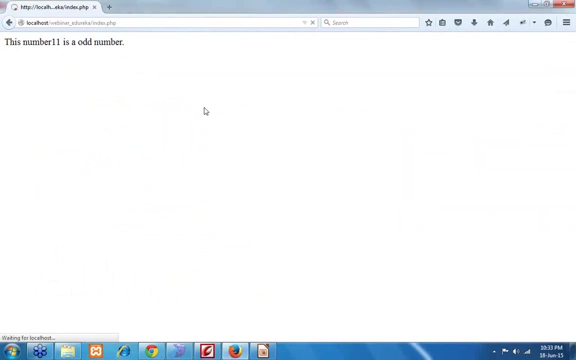 Here we can write dollar number, The same thing we can do below Like this. So this number 11 is an odd number. here We can add a space. So this number 11 is our number. So href isn't used, Prajot. 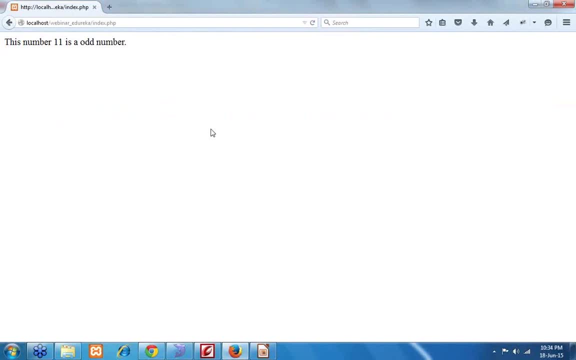 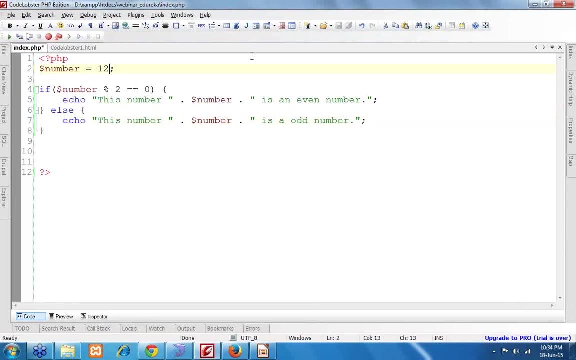 It's used in HTML. So anchor tag, a tag We can simply use to assign a URL. No issues, is our number. If we make it 12. It will become even number. So number 12 is an even number. So here I have concatenated a string and an integer, a variable. 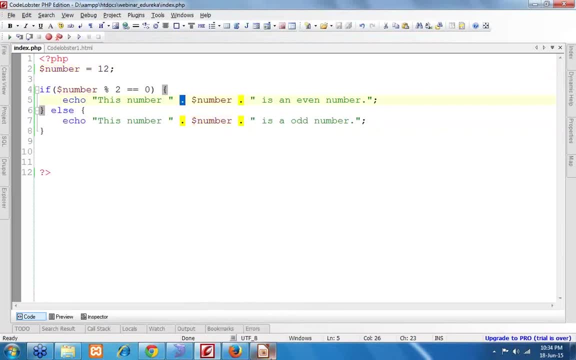 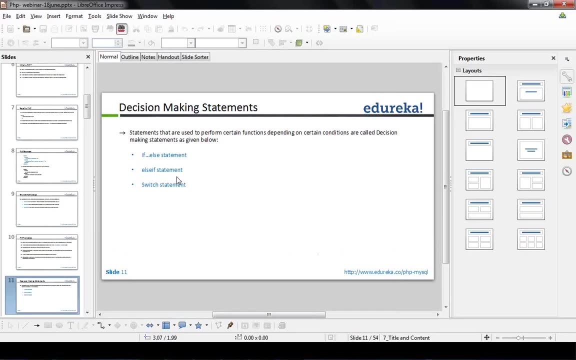 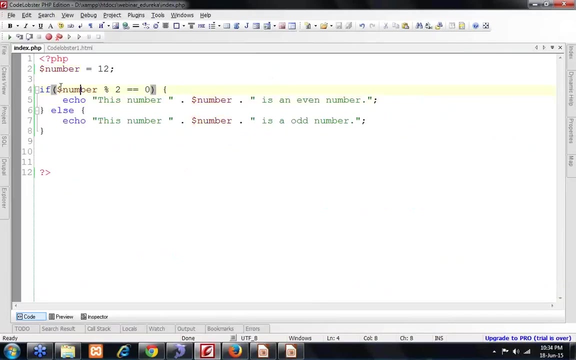 You can concatenate it simply by using dot, whether it's a string or a variable or a number, whatever it is. So this, we have just seen that if, how we can use if. if means inside, if there would be condition. if that condition is satisfied, code inside that if block will be executed. otherwise code inside else would be executed. 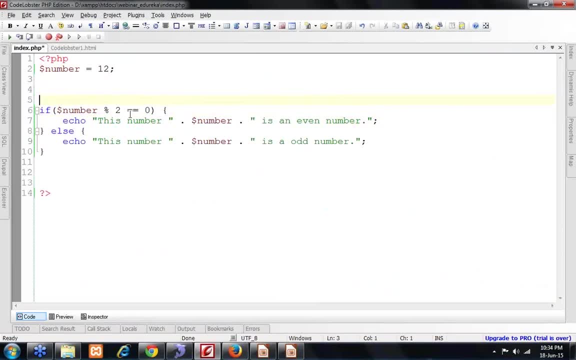 We can have multiple conditions as well. We can also use Like: if This is simply sample, and giving Condition one, Then again else. If any of some of the other condition condition to Like this, Then I can have more conditions. 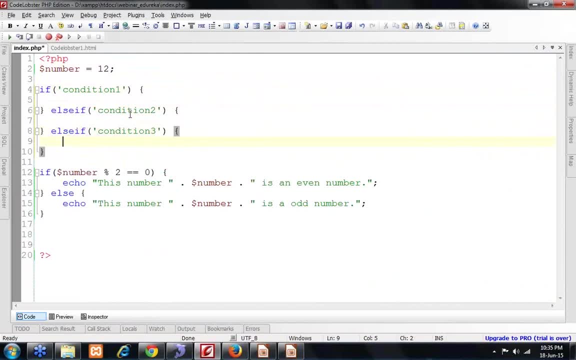 I can have condition three, Then I will. I can have else. So a condition, if condition can be, if else, if like that, Yes, nested. if is also possible, There is no issues. You can have multiple nested. if else else, if same like it, same like cc++. 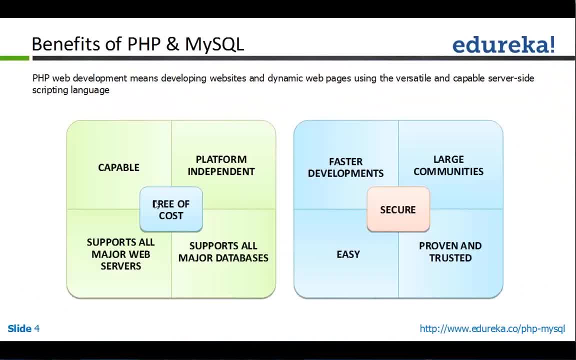 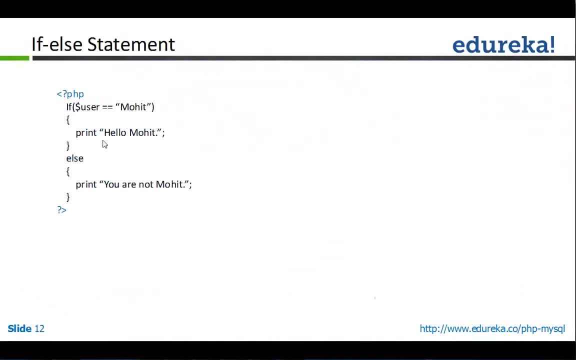 There is not an issue. So if we have seen, if else, if So, this is: if user is equal to mohit, print mohit, else print. you are not mohit. If else, if if D equal to 5, print 5 team members. if else, if D equal to 4, print 40 members. 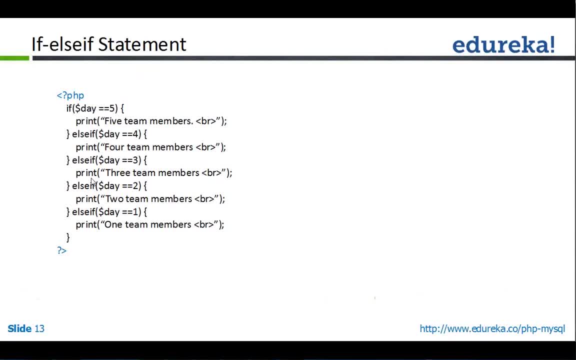 So like this, we can have L, if else if blocks. So here it is switch statement, as we can use, if else, if we can also use switch. so switch would be containing the variable that for which you want To have conditions. So if that day is three, it will print the golden rings. 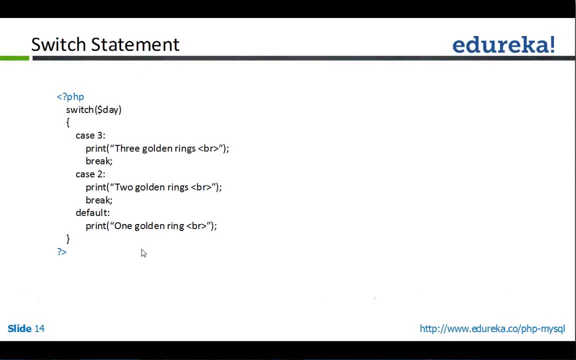 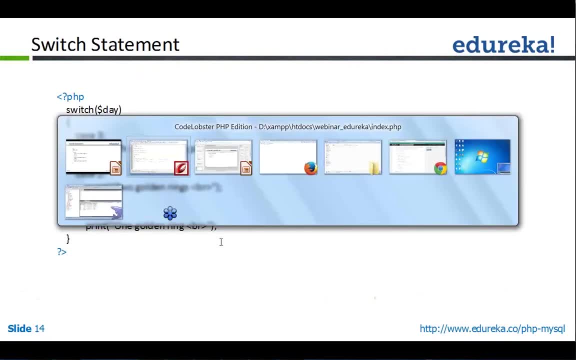 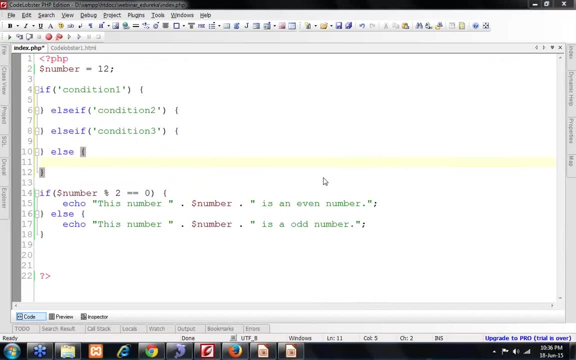 If it is two, it will print two golden rings. Otherwise, like else you can write, it will print one golden ring. Sovic BR is break. It is break tag. If you want to break two lines, you will simply give be a tag and both line will come on different lines. 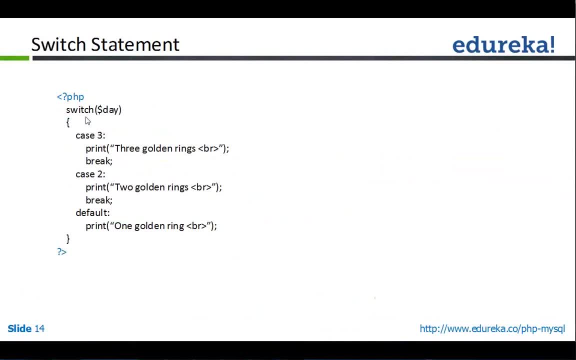 Oops, concept, concept device. I will show you that how we use it. So this is switch where you can simply provide your variable name on which you want to have conditions cases. So if that dollar day is three, it will print three golden rings. If it dollar day is two, it will print two golden rings. 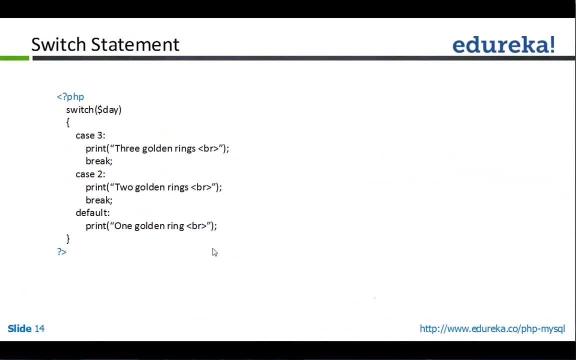 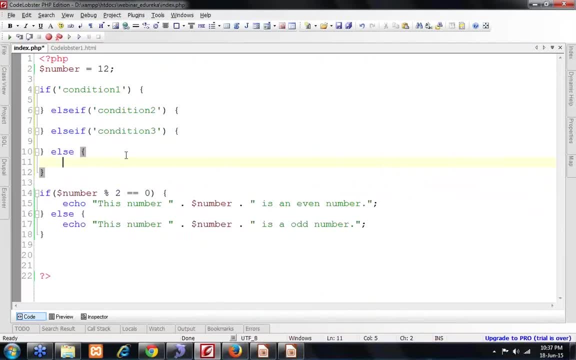 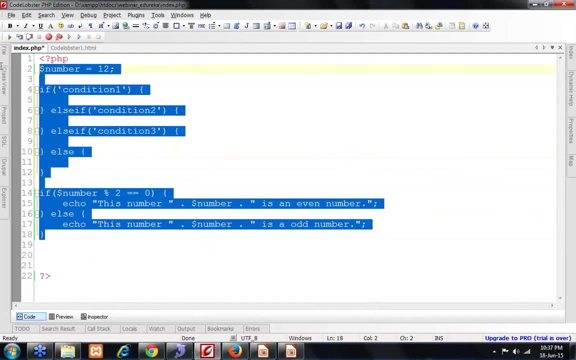 Otherwise it will print one golden ring. So this is the switch statement. Then we come to loops for loop. If we want to repeat thing, we can go ahead with loops. Open that you can use the single variable for any data type. There is not an issue, any data type. 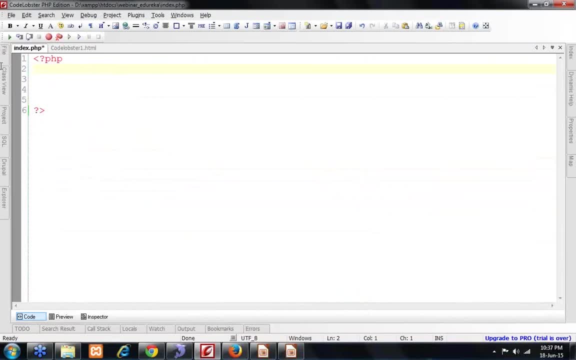 You can. any variable, any of any data type You can give in a single variable. There is no restriction. now for is used for incrementing, something like I want to print numbers from 1 to 10.. So I'll be doing for dollar. 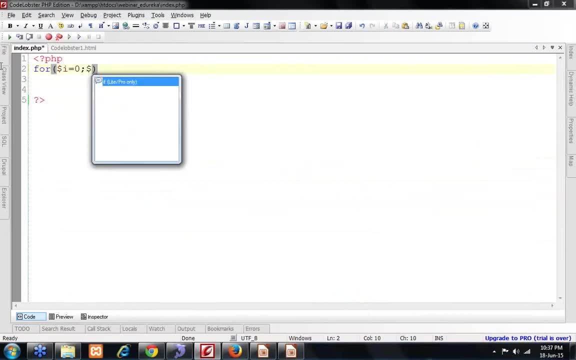 I. so this is called initialization. Then dollar I is less than equal to 10.. This is called limit, setting up the limit, and dollar I plus plus, this is called The increment. now I want to start from 0 or we can do. I want to start from 1, because I have to print from 1 to 10.. 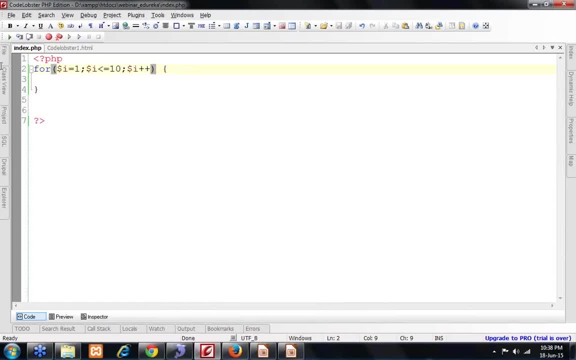 So I will start from 1 and go on. I will go up to. dollar is less than equal to 10.. As it becomes equal to 10., We will skip this particular situation. We will come out of the loop. You can use JavaScript in HTML. 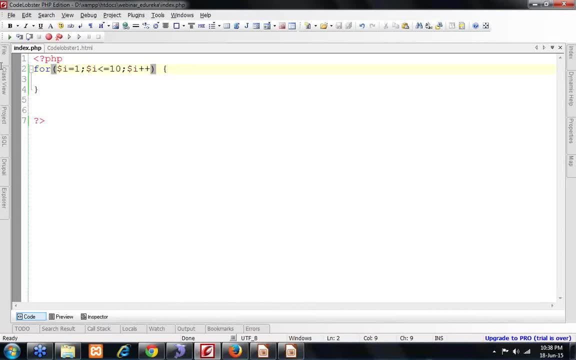 Yes, in PHP You can use, no worries, simply write everything into print or eco. that will be used, not an issue. Now I will do. print dollar I. now I will show the show you the use of break Tag that you were using earlier. print dollar I here. 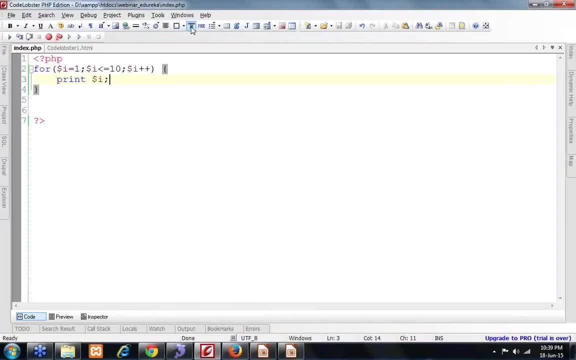 You can see 1, 2, 3, 4, 5, 6, 7, 8, 9, 10.. Now everything is printed on single line. I want to print, and on different lines, So I will be concatenating a break tag, that is a HTML tag. 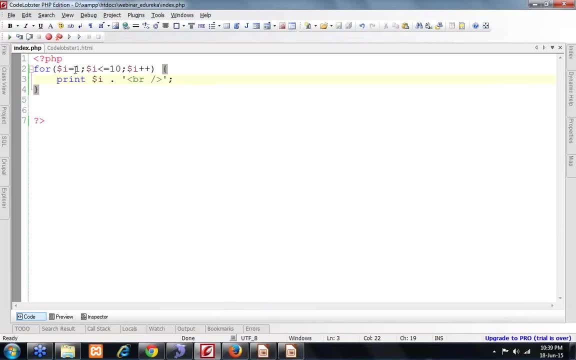 So it will make everything printed or different line. So first one will get printed, next It will check if one is less than 10.. Yes, it is One less than 10, and then it will increment 1 by 1. that will become 2, I plus plus. in PHP, plus plus is used to increment by 1, like if dollar a is equal to 10.. 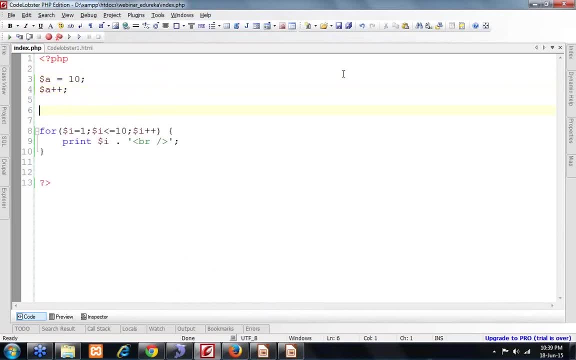 I do dollar a plus plus, so it will become 11.. So a dollar a plus plus equivalent to dollar a is equal to do layer a plus 1, so Both line number five and line number four are one and the same thing. So here I'm incrementing one a number dollar. I starting it from one, going up to 10, and incrementing it by 1 on every. 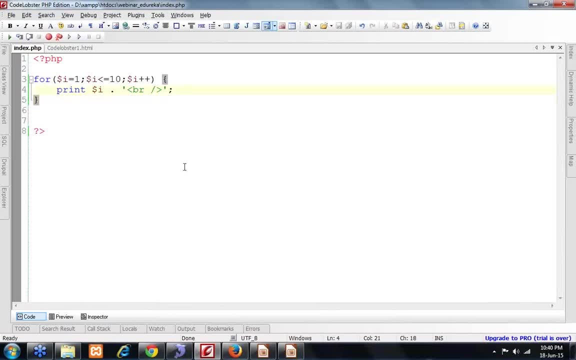 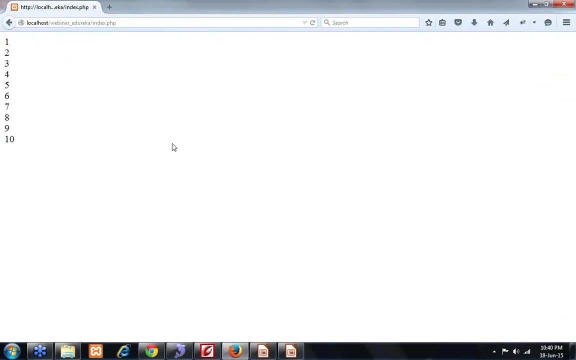 Increment. so print dog. then I concatenated break tag. Now you can see the difference. everything will get printed on different line. yes, aditya plus plus i is also allowed, so it is called pre increment. i plus plus is called proposed increment. it is the same concept as in c, c or c. 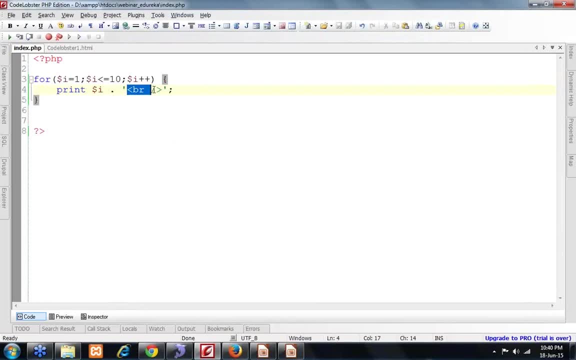 plus, plus. so now you can use the usage of break tag. all the numbers get printed on separate line. so dollar i is printed, then a break break means gets out of that line and comes to the next line. then dollar two, dollar i is incremented by one and that is printed with becomes two, then three. 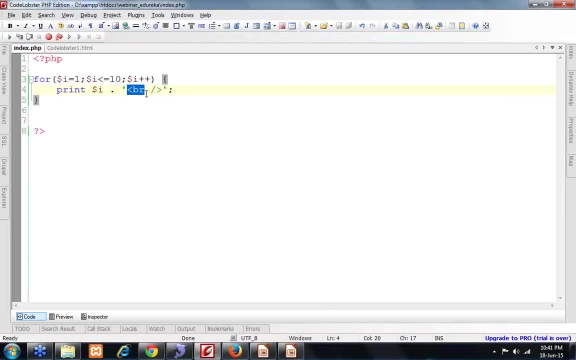 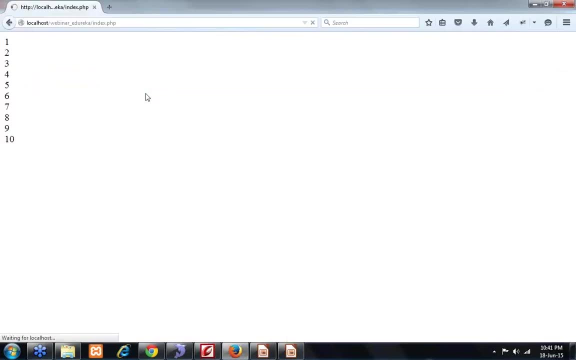 then four, like that. it goes up to it is equal to 10 and then it comes out of the loop. so this way, if we make it 15 now, records will get printed up to 15. so this is called loop shuti session. basically depends upon you people. lot of slides are there. 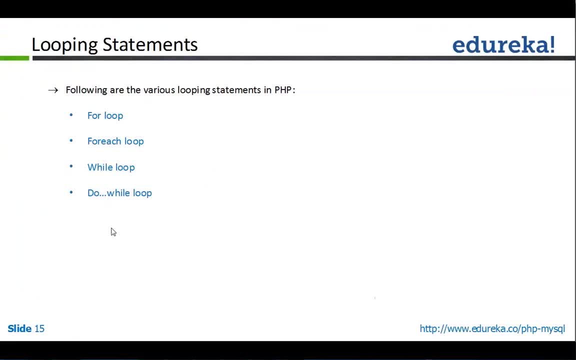 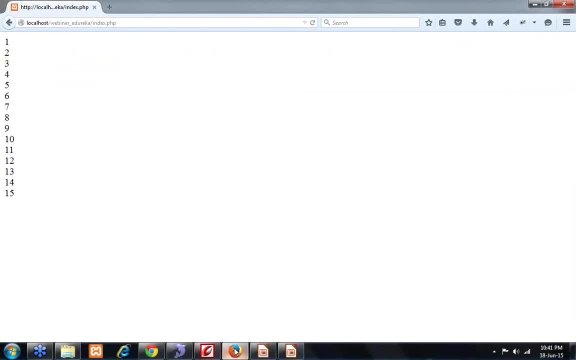 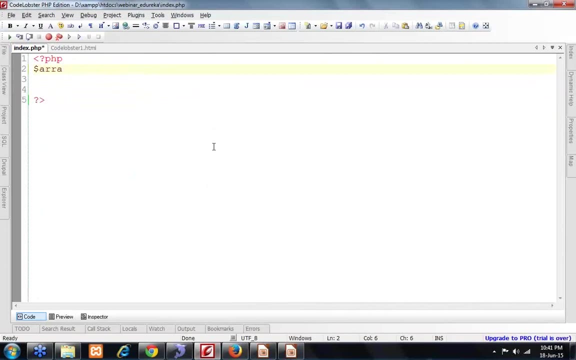 next. let's first let me complete the session. i will not take more than 20 minutes more and we can have your questions for each. so there is one more loop in php that is called for each loop. like i'm having an array here, i will show you that how array is used, array dollar, and we can take array. 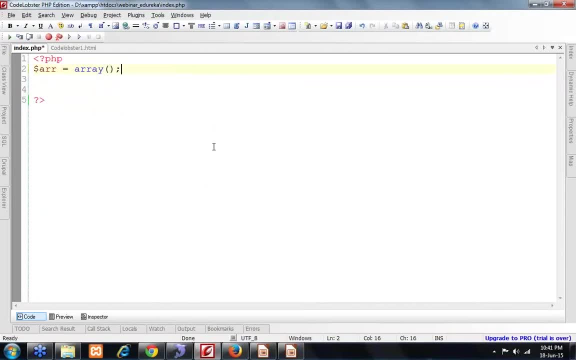 so two kinds of array are there in php. one is called numeric array and one is called associative array. so numeric array is if we take like this, or simply: yes, two, three, four, five, like. so this is called numeric array. why it is called numeric array, i will let you know. so i will take one more array, two, or we'll take up to three only. 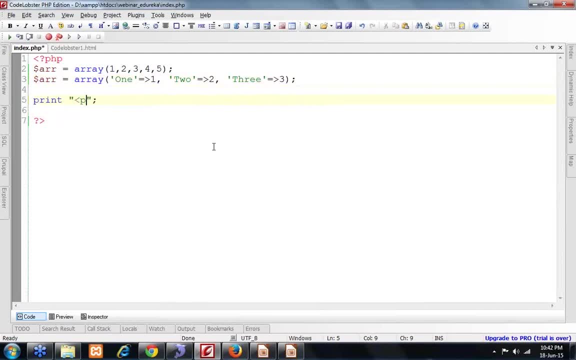 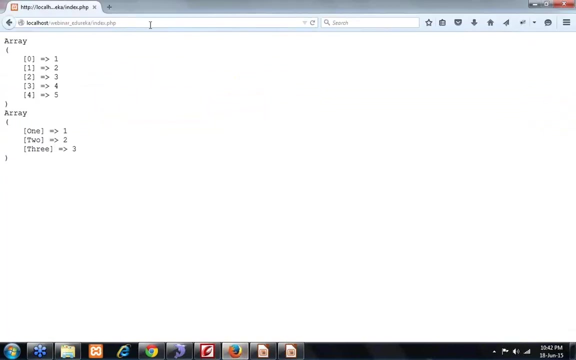 so i will be printing both arrays, print underscore r dollar, or will take array one and array two, one and array 2. now you will see that why i am calling them Lecture numerical and array and associative array. so here you can see the keys are 0, 1, 2, 3, 4, but here keys. 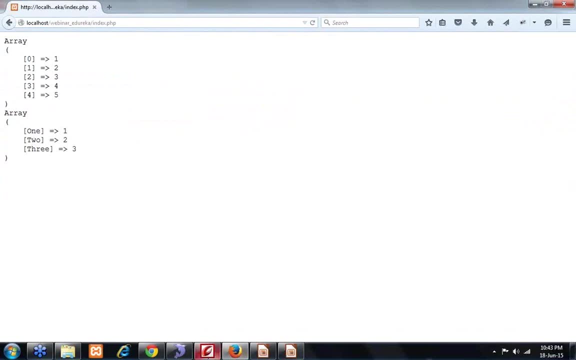 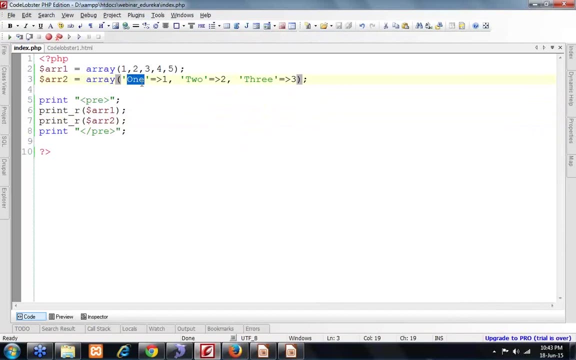 are 1, 2, 3 strings: 1, 2, 3. so wherever you can define your own keys, that is called associative array. that can be a number or that can be a string. here instead of one, I can write test. now, test would become my string in order to access that particular array variable. I will write print dollar array to: 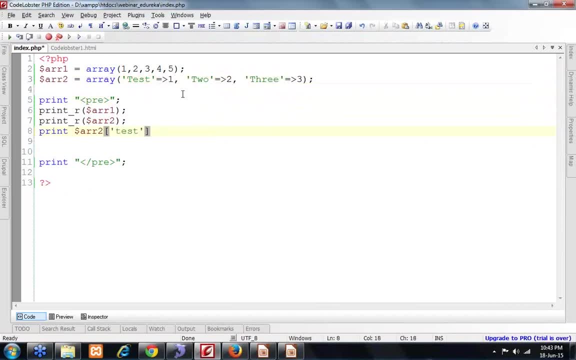 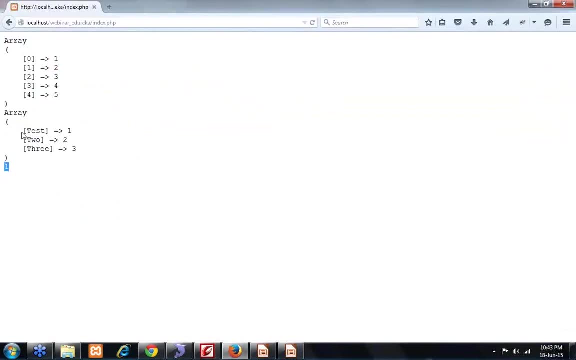 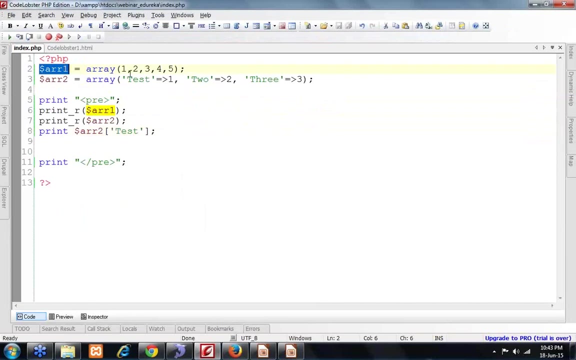 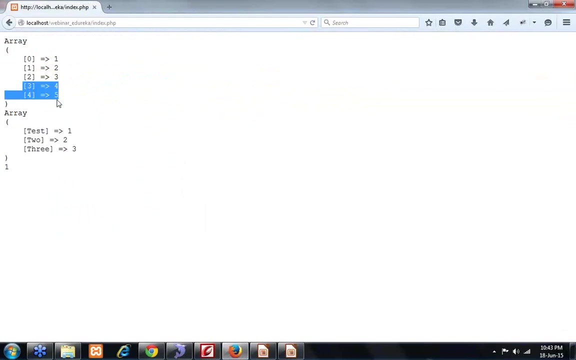 test. now I will be able to access that particular value. that is one line two. so this is numeric array, where keys are numeric, and this is associative array, where keys are strings or user-defined. so this is called associative array and this is called numeric array. so if we are 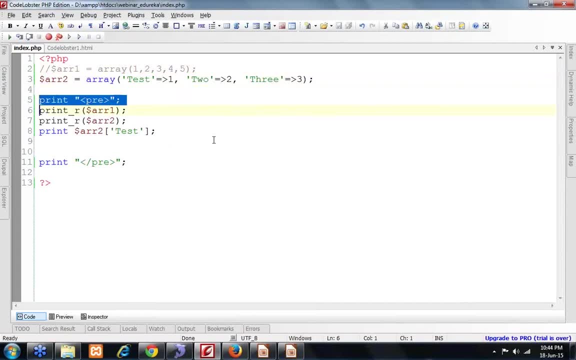 having associative array. instead of using for, we can use for each. so in PHP there is a loop called for each. we can simply give dollar air to as dollar value and we'll simply do print dollar value. so internally it will loop it automatically and print or the values. the same way. we'll be doing BR, so we don't have to provide any start. 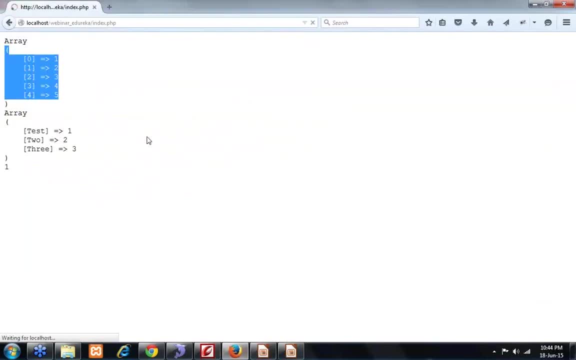 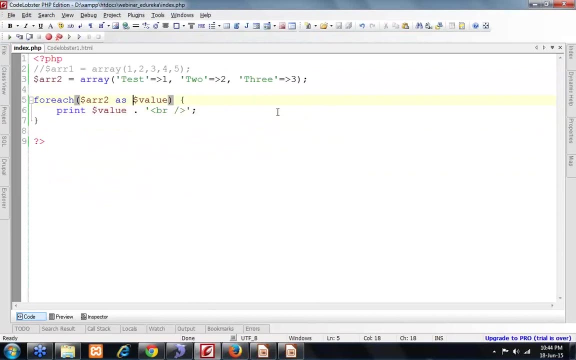 or end or increment, nothing we have to provide and we will get printed one, two, three, because it contains one, two, three and, moreover, if we can also print the keys, so we can write dollar key arrow, dollar value, so this is key and then value, or we can write it on: 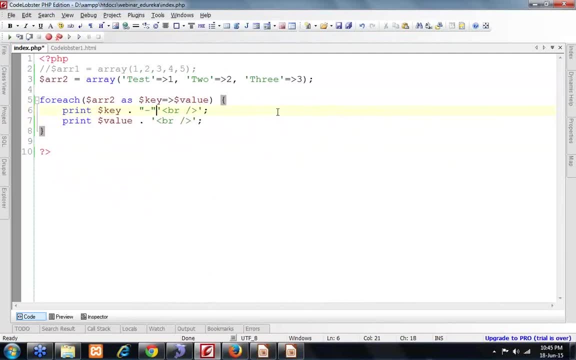 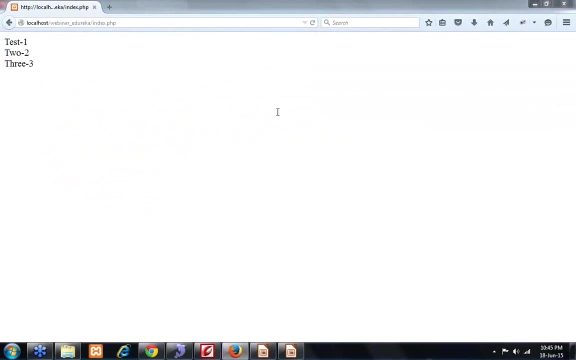 the same line key, then a dash and dollar value. so test one. test to test three, test 3, so this will print: are the column orders in hexagonal operations. so Team 3.5, this will be having this one. test two have been different because the hidden row is here. after that, automatic 0.4 x is equal to a fingers'AND that. so so, before I go and никогда been there. after that, automatic 0.4 x is an empty nano command. is there that deliberately make these labels each read different various things? you just to take a look. patentselect hadn't attached this. 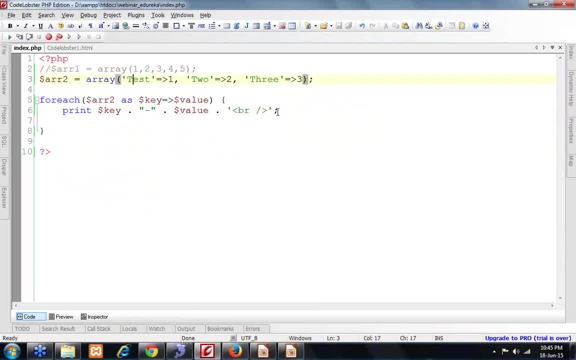 one. sorry, this can be made one. so it is 1, 1, 2, 2, 3, 3. so keys and values, both are printed now. so for each, your array, then key arrow value. so associative array is defined as key, then arrow, then value, then key arrow value, like this, and it is printed in the same way. 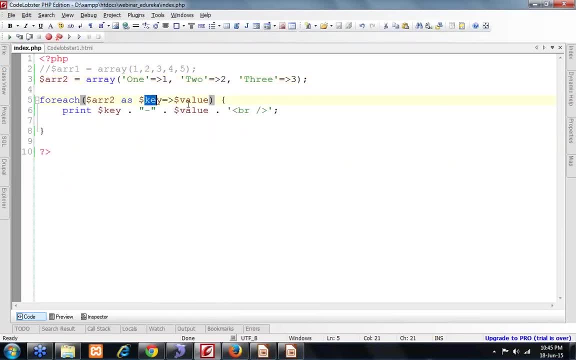 for each your array as the key arrow value. this is not a fixed thing that you will give key value. you can give like this, only anything you can give. this is a user defined variable. this is not going to be key value always. it is user defined. so here is the for loop as: 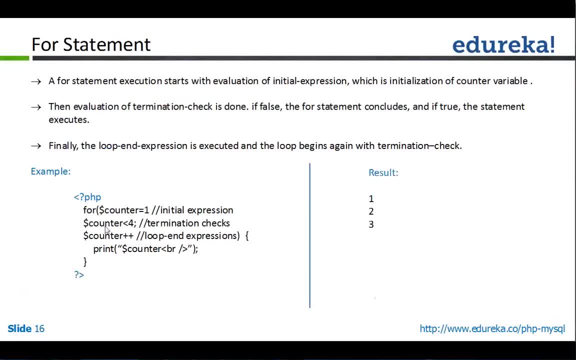 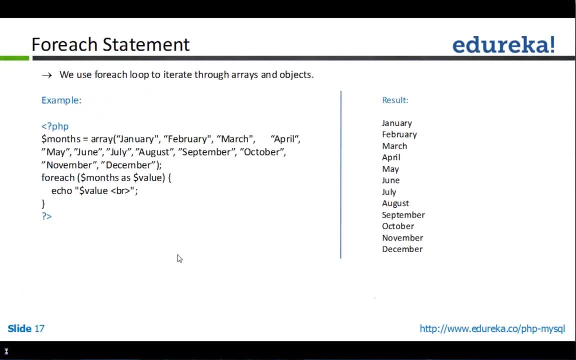 we have seen that you will give initial expression, initialization, then give termination, check or condition, then you will increment and you will get your value printed. and this is for each loop. we are having array for months- Jan, Feb, March, April, May, June, like that- and we doing for each. we are doing: 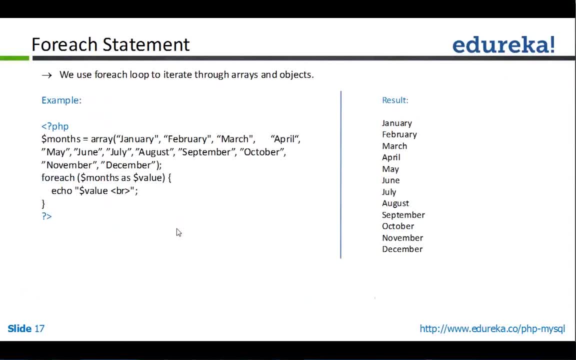 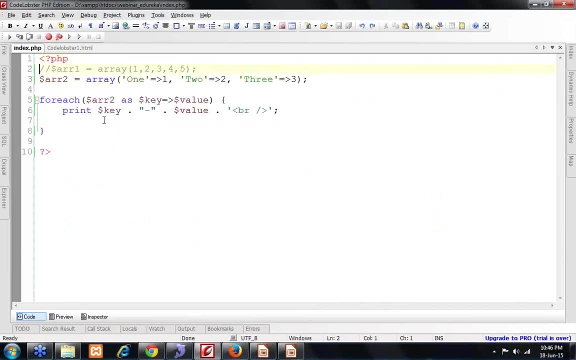 dollar months as dollar value and printing the value. so internally it will, it will increment and it will print it. so this is for each loop, next while statement. so that same way we can use while as we do another programming languages. so while, inside there will be a condition and till that condition is true, the loop will go. 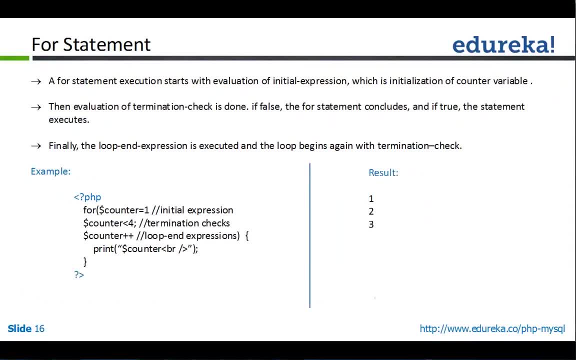 okay, slide number 16. you want to go ahead? okay, Okay, okay, what is the question, Ashish here? so what is your question, Ashish, regarding slide number 16? we have to be bit fast because lot of slides are still pending. so, Ashish, can I move for the slides? 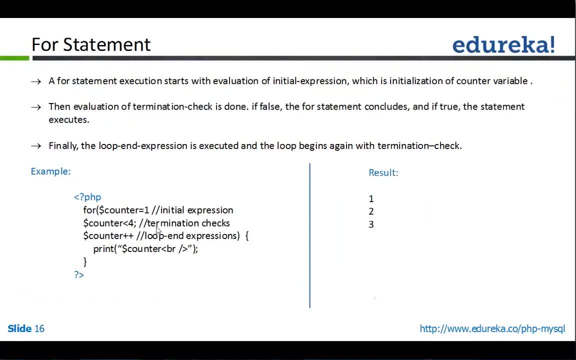 Ashish, for loop and for each loop are different. okay, four is used. both are having different is its own syntax. we can't say why, because it is up to the PHP interpreter, or you can say, the designer of PHP who designed PHP. he has provided two different loops for and for each. so for each, mostly we use for associative. 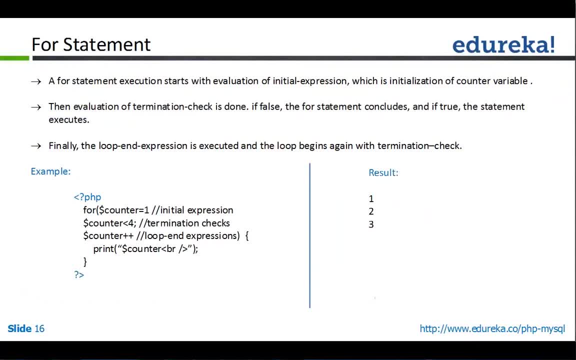 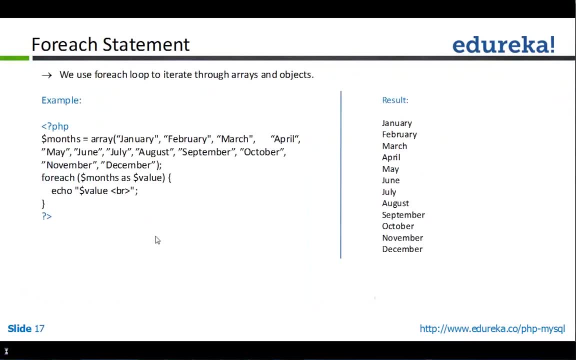 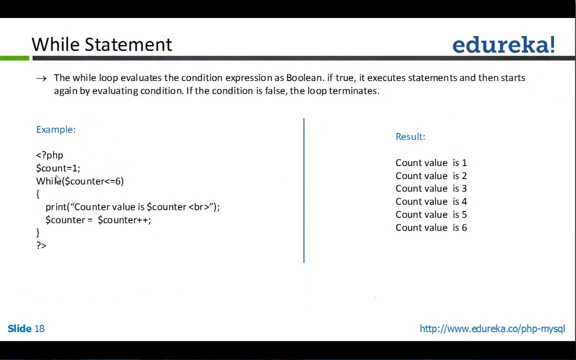 arrays where you don't need know the keys. you cannot loop over the keys. Aditya, this is the PHP syntax- that before every very be given dollar. so this is wild statement. so count is 1, while counter is less than equal to six. so it would. 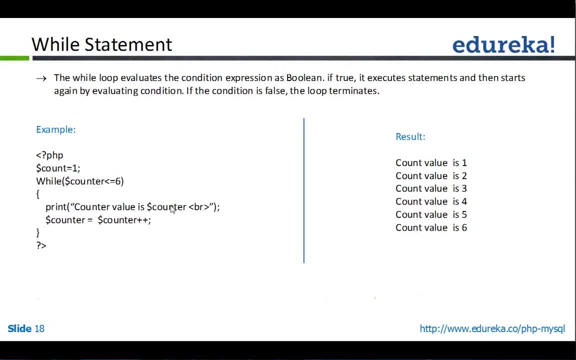 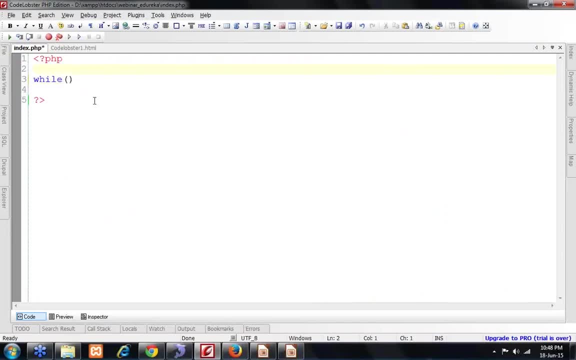 be counter equal to 1, while dollar counter is less than equal to 6. I am printing something and counter. I am incrementing counter by 1, so here I can simply write $ counter's problem. I had given dollar 10, counter equal to one, while counter is less than five. I will take, I will do. 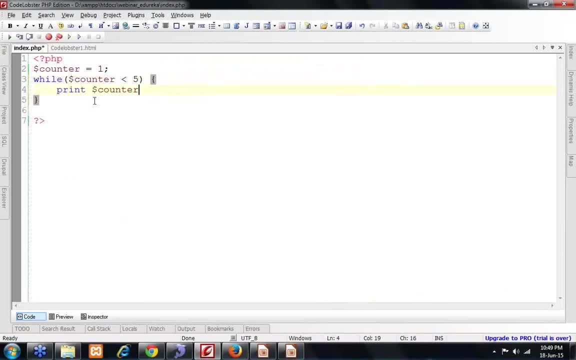 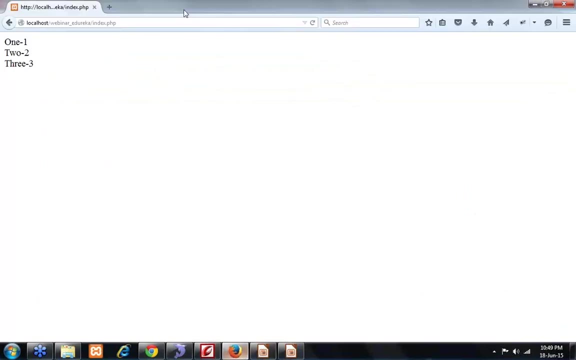 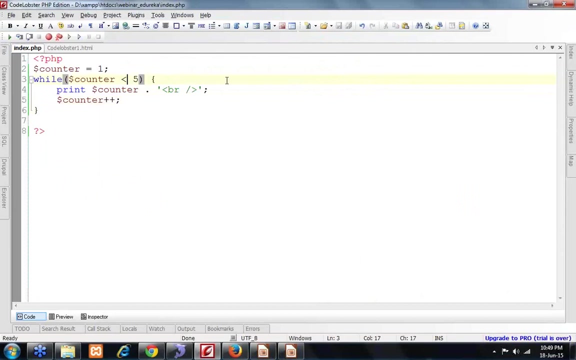 print dollar counter and then be a tiger, will be taking and then I will be incrementing dollar counter by one counter plus, plus. so it will print one, two, three, four, because as the counter becomes greater than four, because it is less than five, if I make it less than equal to five, it will print up to five. 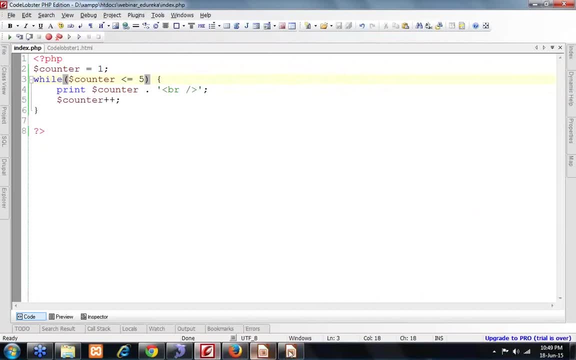 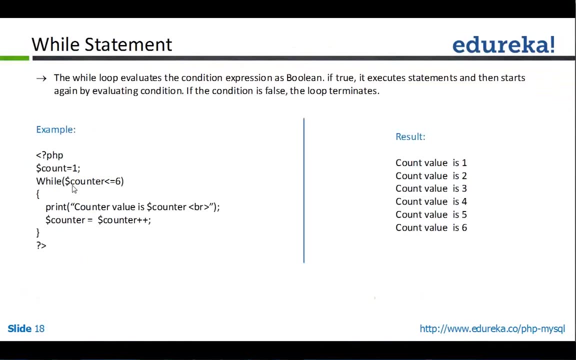 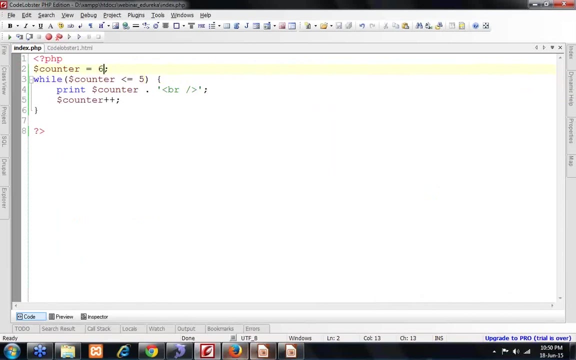 so as it becomes five, it comes after the loop. this is called while loop and next we have do while loop. so the difference between file and do well is that if condition is false in the beginning, for example, if I make it five, if I make it six, so now nothing will get printed because 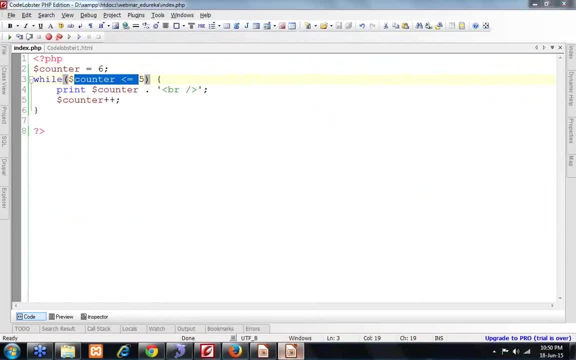 condition is false. here the difference between while and do while is that in while, if condition is false, nothing will get printed. but in B, if condition, even if condition is false, it will print at least once. if we do do or we will do, take the same thing. 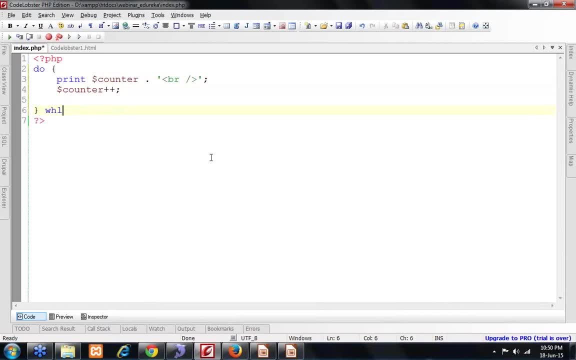 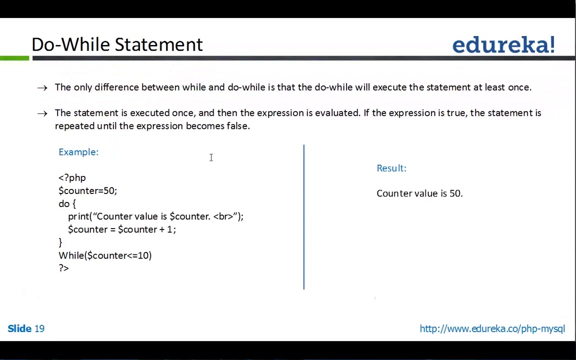 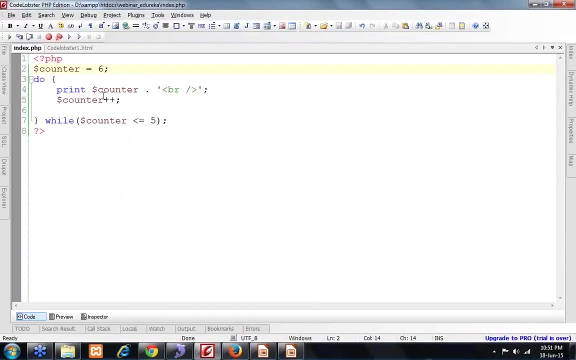 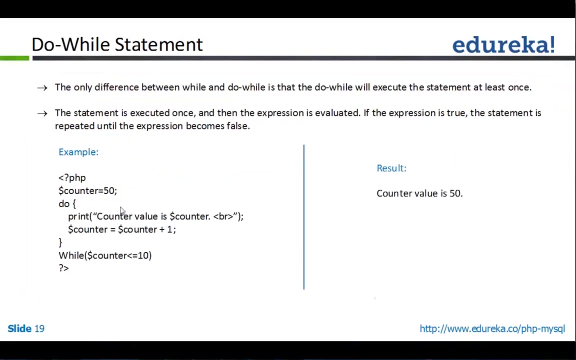 print, while dollar counter is greater than less than equal to five. now I'm taking dollar counter as six. now you can see it is printed once. do print your counter, then check the condition. so what do is doing? it is first printing the things, then checking the conditions. so so your result will be printed once. definitely it will be printed once because, first, 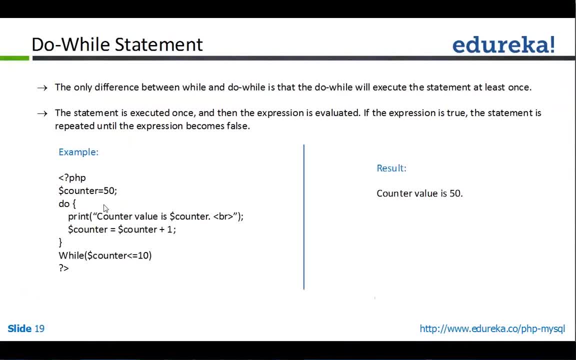 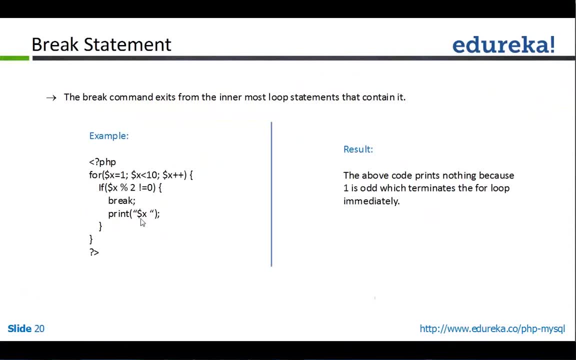 First it is printing, then checking the condition. On the other hand, while is first checking the condition, then it is printing. So this is difference between while and do while. So now it comes break statement. So break is to control the break in between your condition. 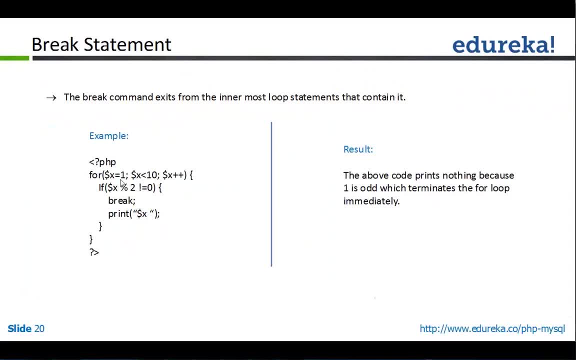 or inside your loop. So here I'm checking: $4 X is equal to one. I'm looping from one to 10 and checking. if number is not odd, then break. So here result would be: one is odd. So here my number. if number I've taken one, for example, 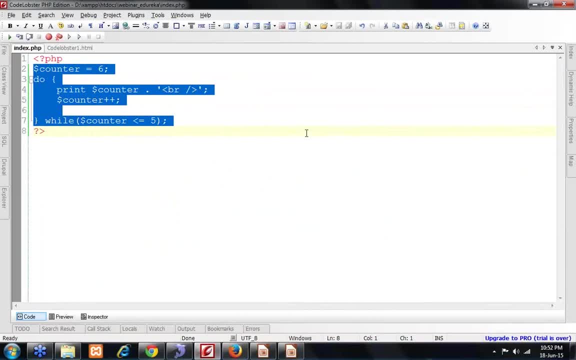 So there is no. basically both are different variations, So like. So what I'm using for $I is equal to zero, $I is less than equal to 10, $I plus plus. So I'm printing: if $I% two is equal to zero, then break. 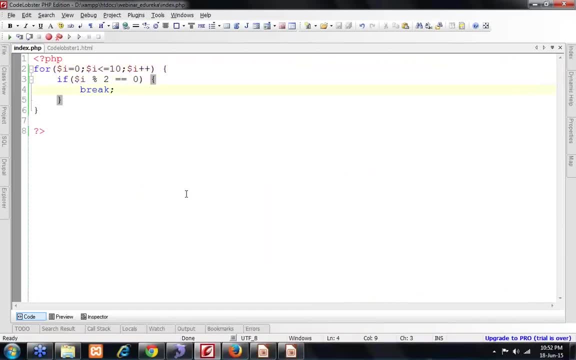 Print $I and then break. So see: first is zero. So let me start from one, then you will see the difference. Here see: two gets printed and break. It never runs the complete loop. First it checks If number is even. if yes, it prints that number. 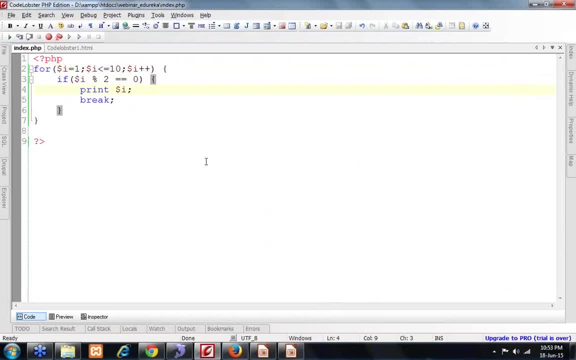 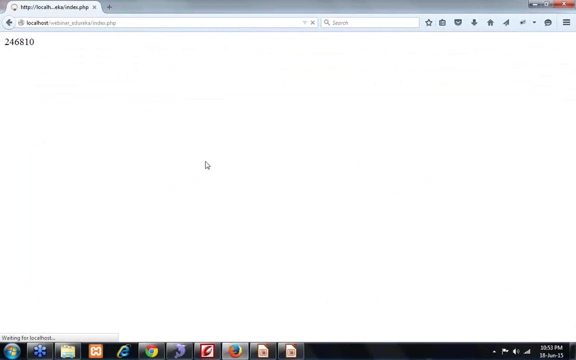 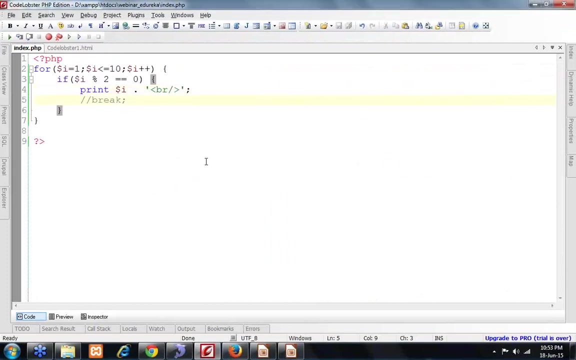 and gets out of it, gets out of the loop. It never runs. anything else, If I don't print, you will get printed. Let me add BR tag. So there's two, four, six, eight and 10.. All the even numbers are printed, but if you put break, 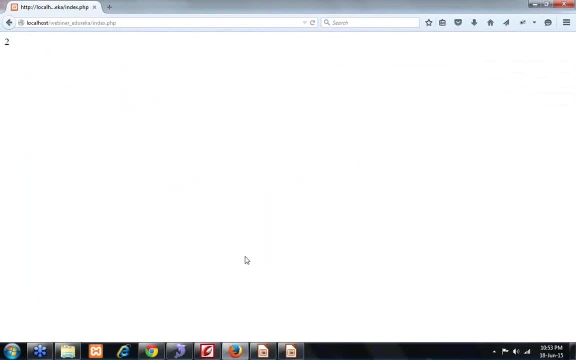 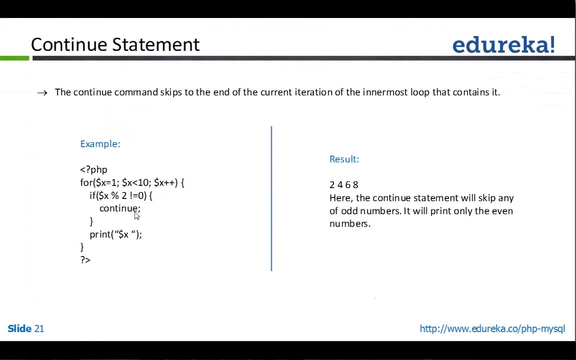 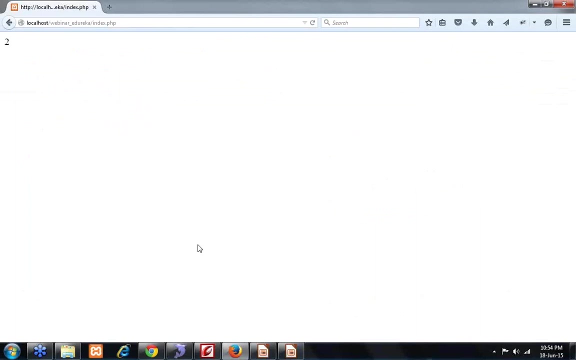 it will stop over there. So, after printing two, it will stop over there. It will break the control and come out of the loop. This is break And next it comes continue. Yes, break breaks out of the loop. It breaks the control over there. 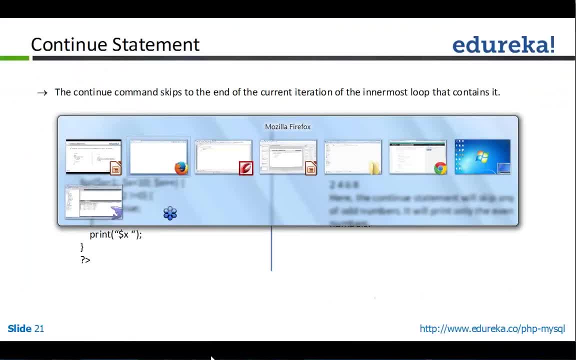 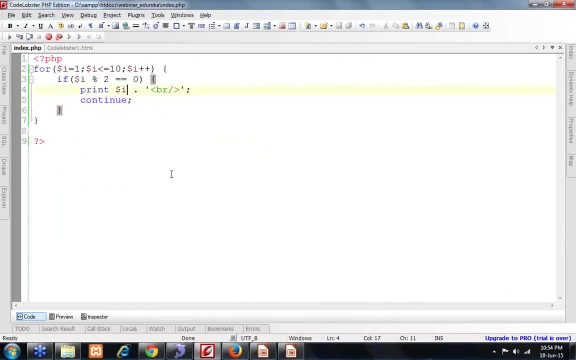 Continue means skip that particular record and move further, Like if I put continue here, Well, I'd rather print this outside the loop. So I'm saying that if I encounter an even number, continue, skip that particular number and go to further number. 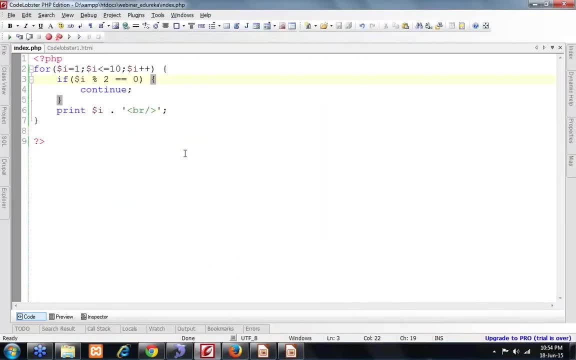 So it will print one, three, five, seven, nine means odd numbers. Yes, continue. skips that particular number and moves to the next counter. It skips that particular counter. So it means that when record one comes, it prints it because it never goes into the condition. 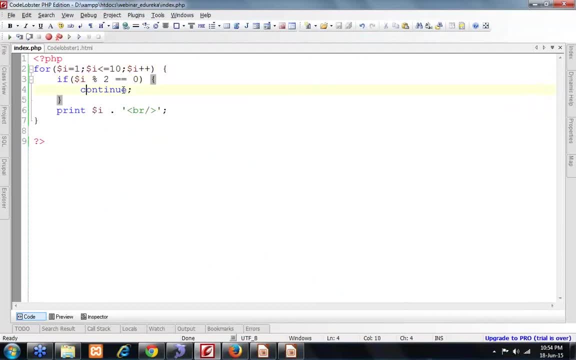 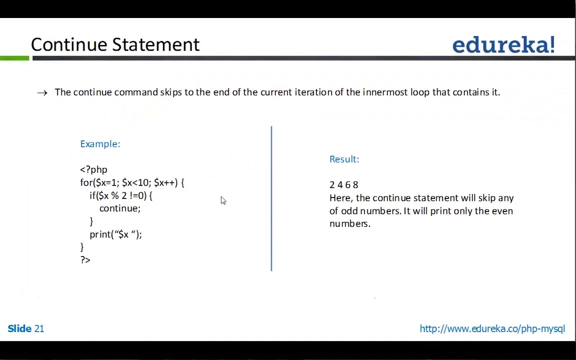 When two comes, it goes into this condition because it is even and it skips that two and increments the loop and comes to three, and then three gets printed. So continue means skipping that particular step and continue with next step. So print can have brackets. 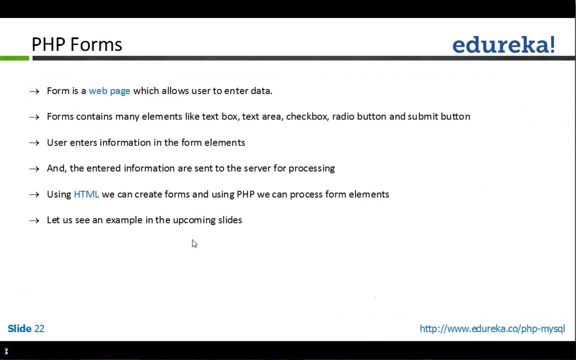 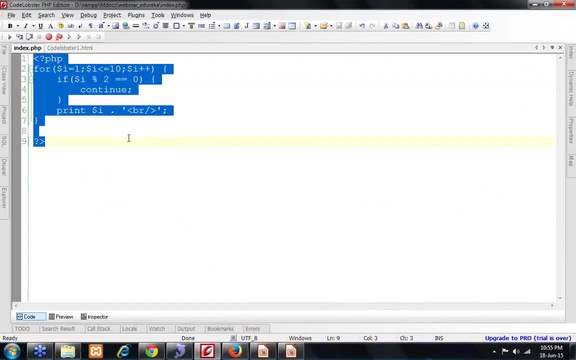 That is not an issue. Both ways we can use it there, Not an issue. Now let us come to PHP forms. So now I will show you that, how PHP can have forms. So here I'll be giving. input type is equal to text. 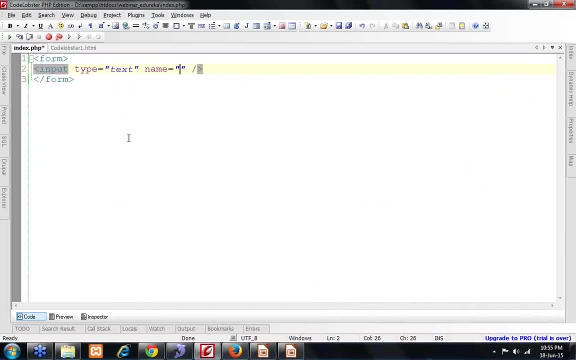 Name is equal to. I can write first name And I'll be taking first name as label. Then I'll be taking same thing for last name. Then I'll be taking same thing for last name. now I'll be taking break tags in between. 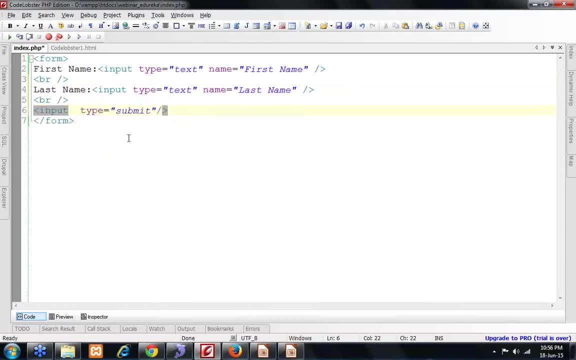 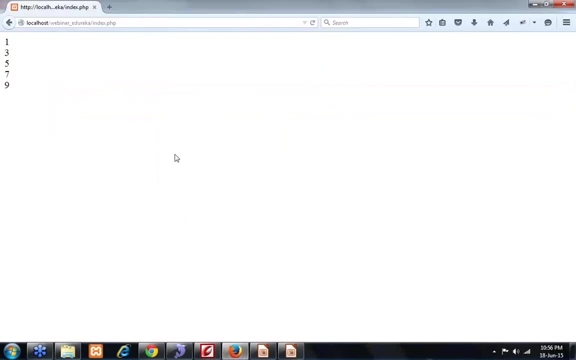 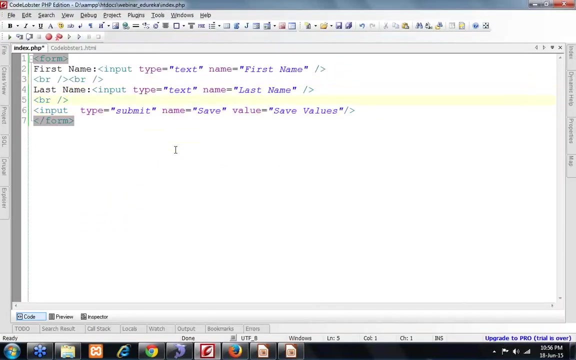 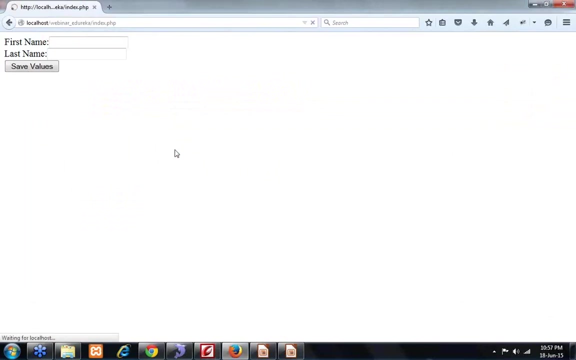 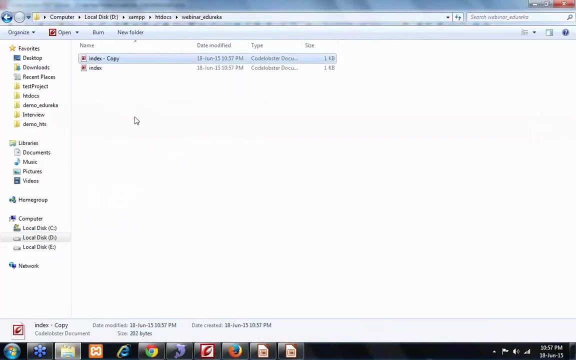 then I will be taking a submit button. so now it would be my phone: first name, last name and then a submit button. so now this is my form, simple form that contains first name and last name and there is a submit button. now, how are we'll handle this form? so I'll be creating one more: save data dot. data dot. 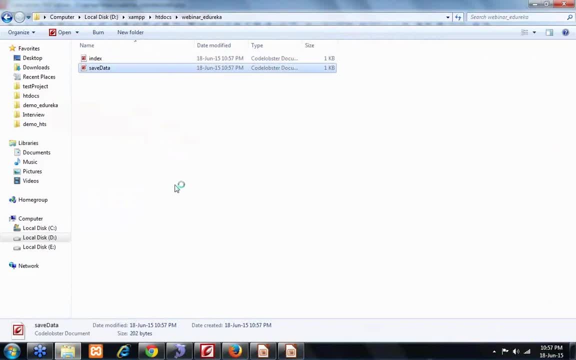 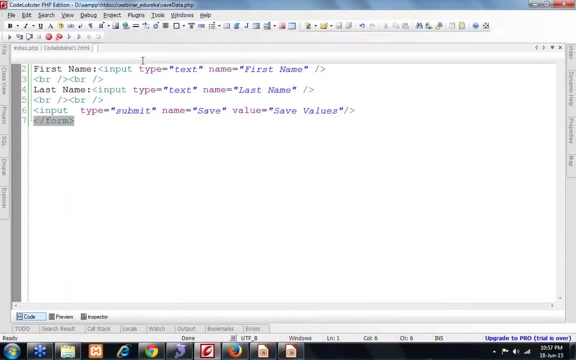 PHP that will be handling this form. so each form would be having a method. so method can either we get or it can be post. we will be looking into that, what get means and what post means- and then it would be having action. action would be PHP file that would be handling this particular form. 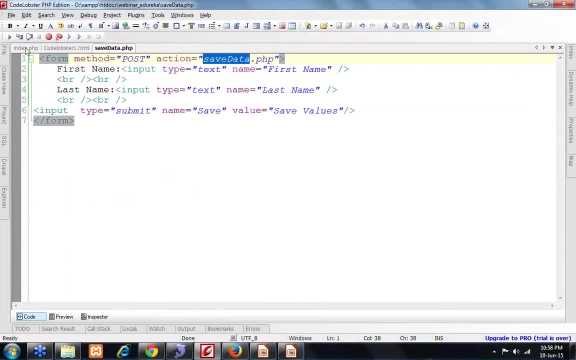 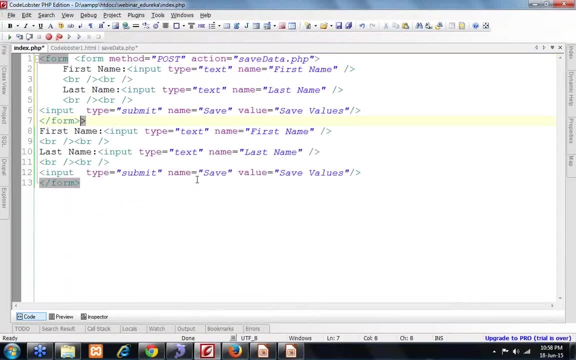 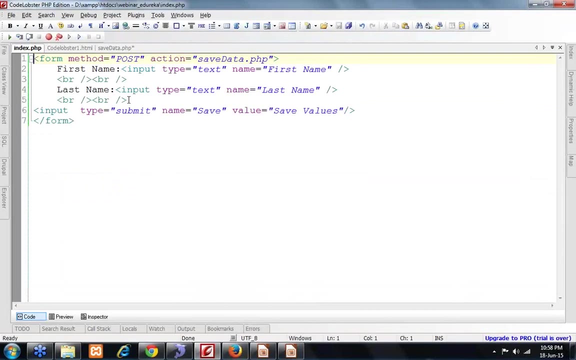 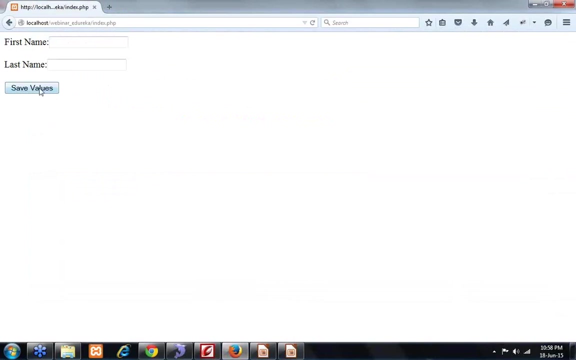 so save data would be the file where the control will go once we submit index file. so this is my index file where I'm having a form. now see, I have taken as save data and method and post and when I click on save values here you can see I went to save. 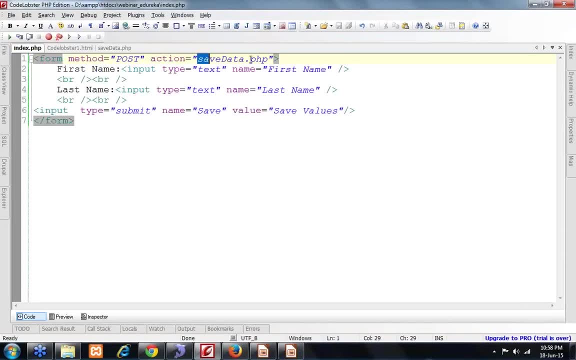 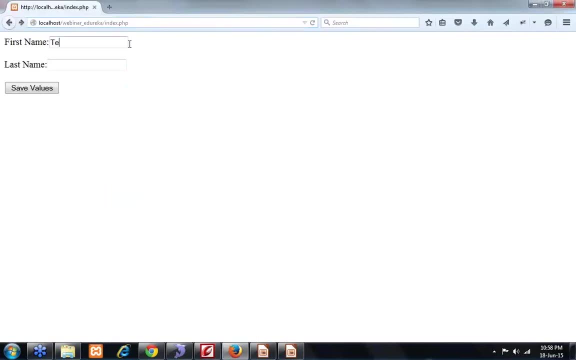 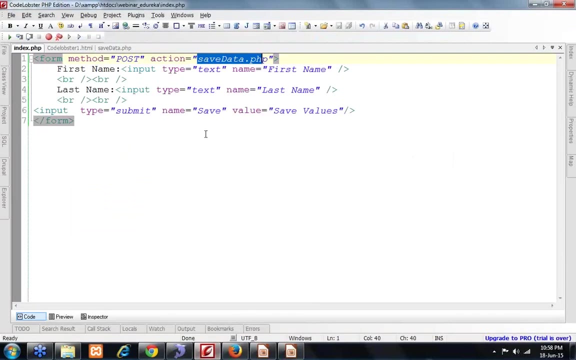 data dot PHP, because I have given action as save data dot PHP and this save data will be handling my form now. now I have put values as test test one and say values. now it goes to save data, but nothing happens. now save data is supposed to handle this form, so in PHP we are having two. 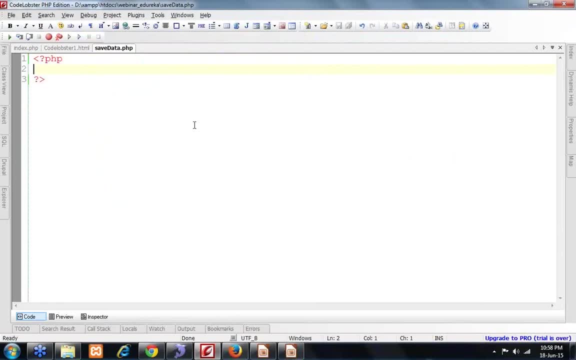 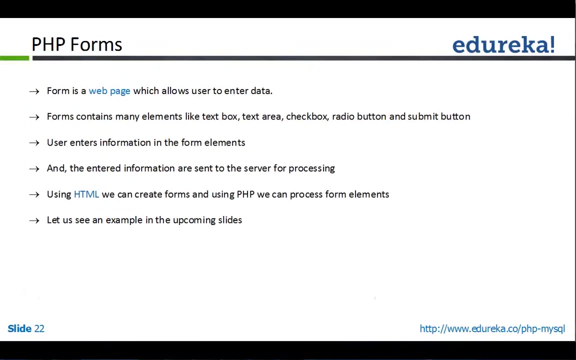 particular inbuilt arrays. that is called post array and get array. yeah, sorry guys, actually there is a update for you. right now I'm pleating all the slides and if you are having some blocking question you can ask immediately. otherwise you can just put your questions over the support. 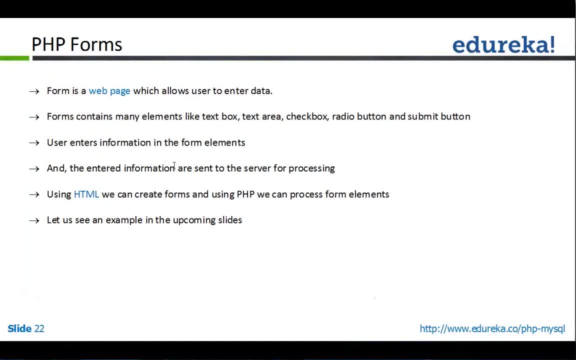 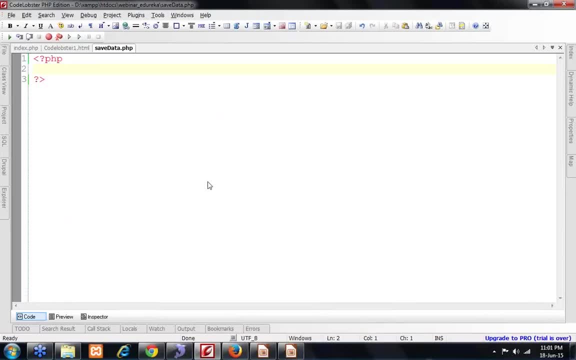 you can ask immediately, otherwise you can just put your questions over the support. you can ask immediately, otherwise you can just put your questions over the support, and support people will be answer to your questions. so let me finish up the things practically so that at least you are aware of everything now. in PHP there are two arrays called get array and post. 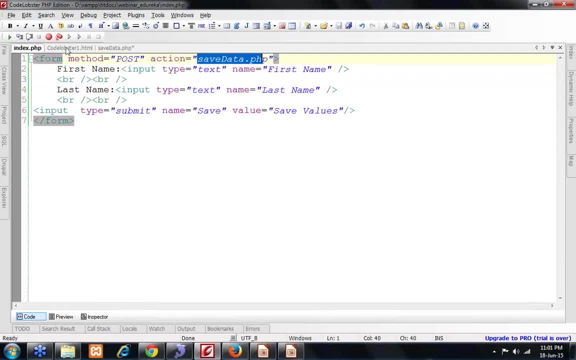 array that basically handles the form data based on which method you are using. if you are using post method, get data- you will get form data that you have submitted. you will get in post post variable. otherwise, you will get in get variable. so how we use that now let's see. so pre. so pre is a tag to 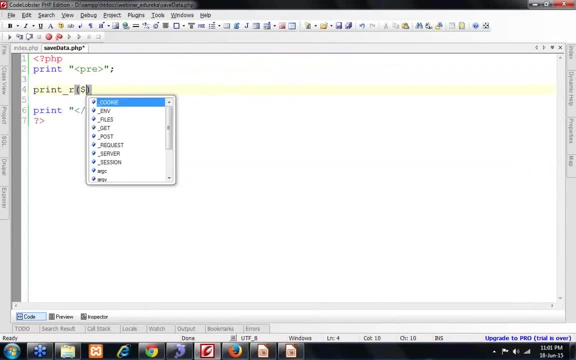 print your array. I will be doing. print underscore- our tolerance underscore post or dollar underscore post is an inbuilt PHP array that handles the values submitted from a form using the method post, so let's see how it handles what I have done. I have created a form with method post and action save. 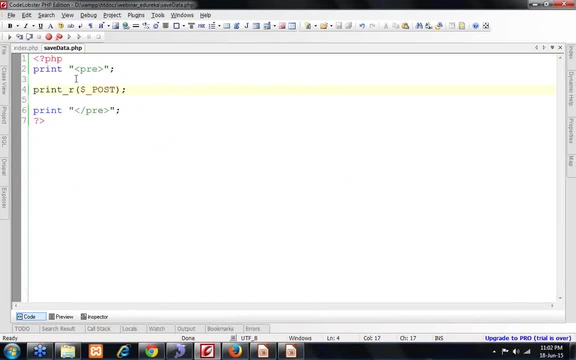 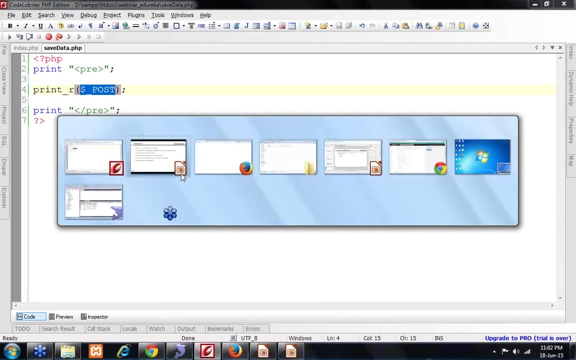 data. so save data will be handling this stuff. once the form will be submitted it will go to save data. so here I'm using dollar underscore post, so I'm having to input text that is first name and last name. so when I will submit my form- till now you have seen that I was able to see the blank save data- 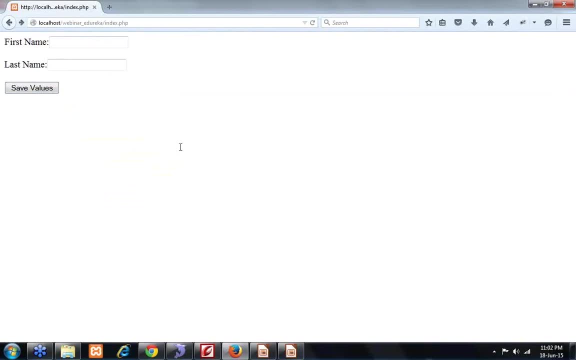 now, as I have taken dollar, printed dollars, got post array. now, if you write first name as test or you can see F or anything. test test one and click on save values. now you can see save data contains your array. this array is having three elements. one is your first name. your last name. 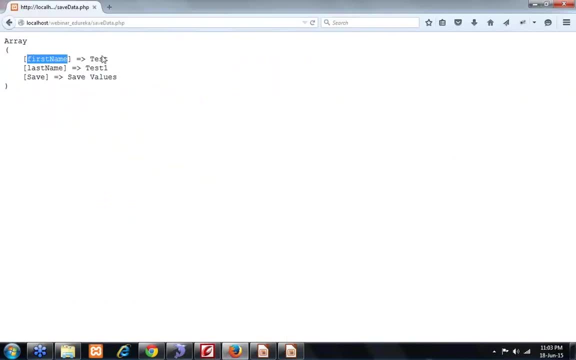 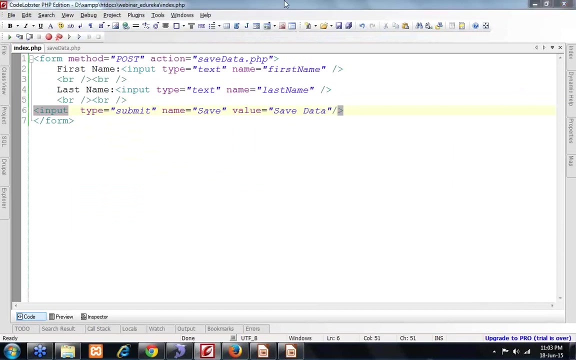 and your submit button, so it contains values of all. first name. you have given test. last name, you have given test one and save for save. we have values, save values. that is your first name and is the text being displayed over the button. if we change it. save to save data. now you've. 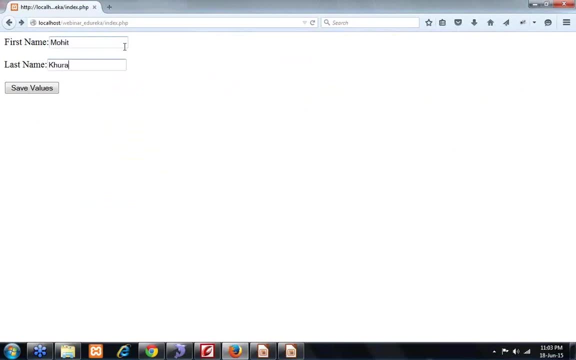 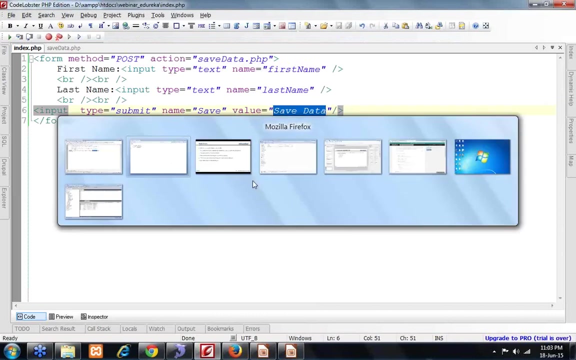 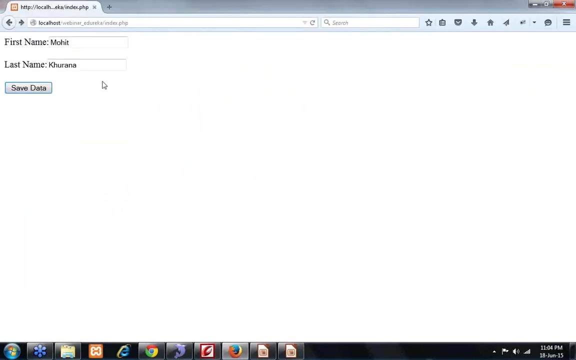 submit the form with like Mohit Khurana and click on save values. you can see your first name contains Mohit, last name contains Khurana and save contains your save values. so save data because we have updated value as save data now. if you change your method now you can simply see when I submitted my form, I came to save data. 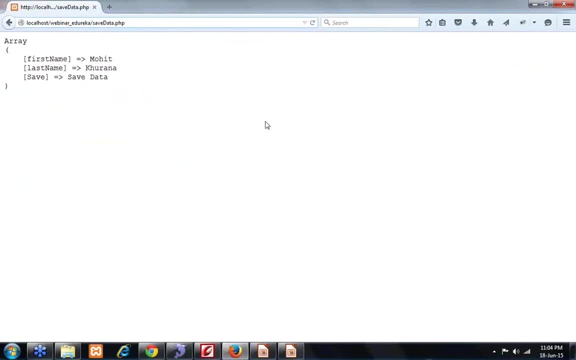 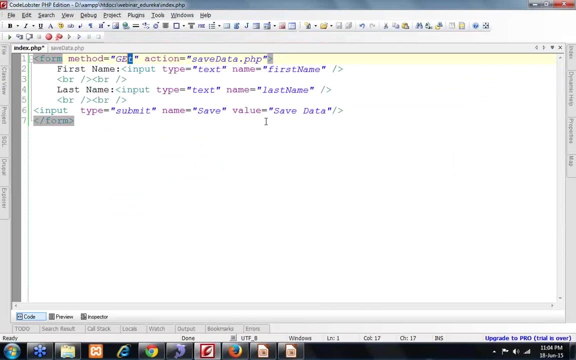 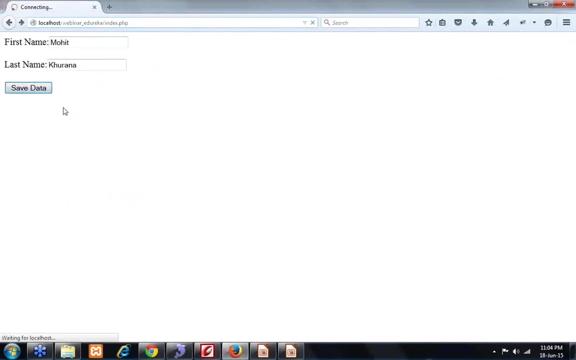 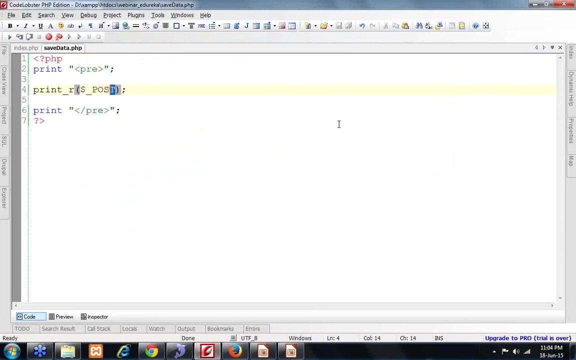 dot PHP. simply, I didn't have anything else with the URL, simply save data dot PHP. if you change your method to get and do the same job, you fill name and click on save data. now you will see blank array. why? because now you are using get method with form. data will now reach in comprended total score. get knot in. 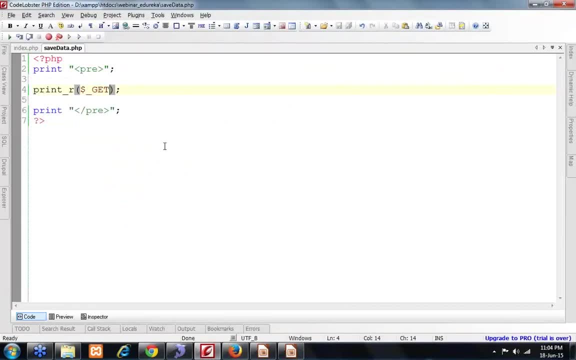 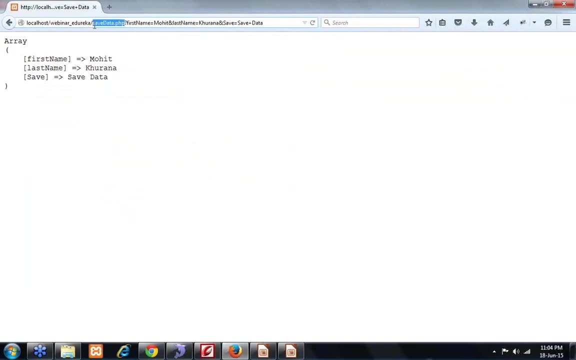 dollar- Youtube videoio. getJS top p associate. dude up all your values. all your phone data is now appended to the URL, with first name equal to first name, then M percent, then last name equal to last name, then M percent and then the third variable. so this is the difference between get and 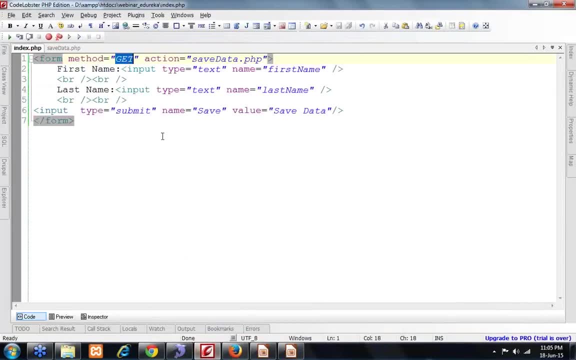 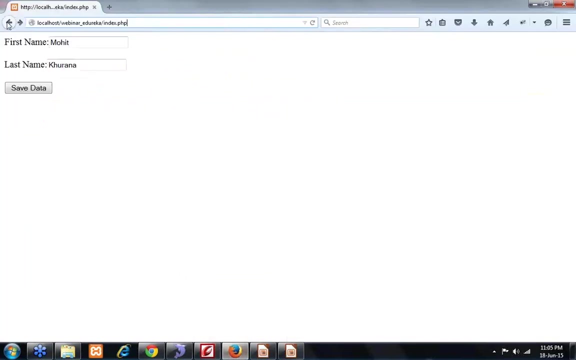 post is that if you use get first of all, every value of your form will be appended to your URL. and second thing, you will get the data in dollar underscore get. and if you submit the form with post first of all, you will get all the values in dollar square post. and second thing, 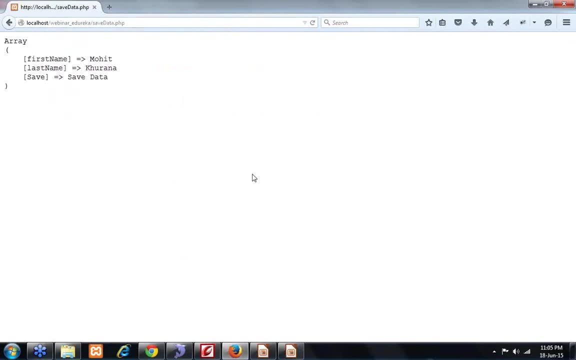 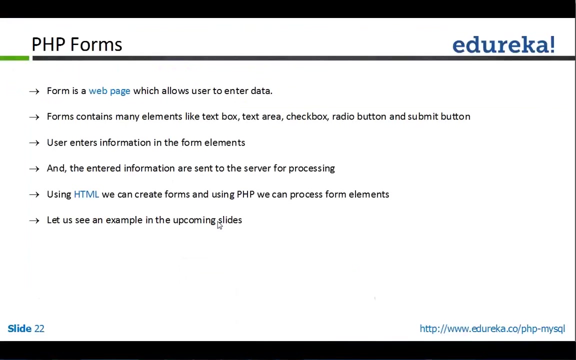 nothing will be appended to URL. everything will go in the back end. so that's it. GET is normally used where we want to bookmark our page, but POST sends the data in back end. so you can bookmark a page with POST. So this is PHP form- how we design PHP forms. 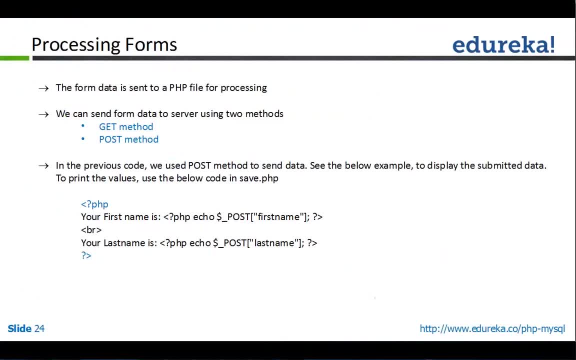 Then different methods: GET and POST. GET is basically advantage and disadvantage of everything in URL is that if you are logging into your email account and you put your email and password and if that email password is displayed in the URL, that is very risky and you can get that username password. 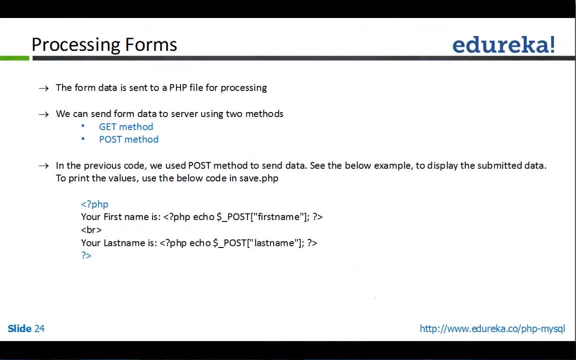 So any secure information if you are going to use, you should always use POST, not GET. But if you are working with static sites where you want to bookmark your page, simply use GET. You can use GET, but most of the time we use POST. 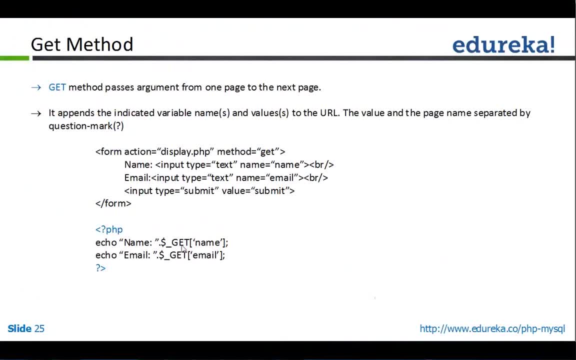 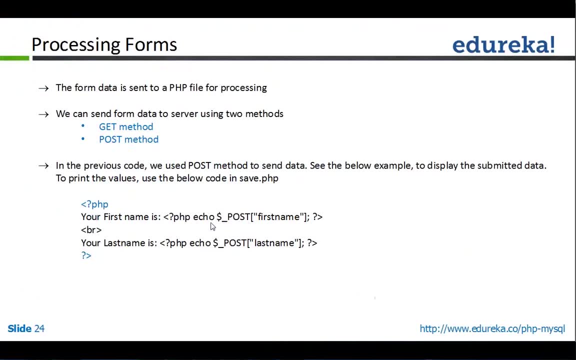 We prefer POST, So this is GET method. So POST is printed with $POST. Yes, Aditya, there is limit. site of GET. GET is basically a string, a query string, So it can be up to 2048 characters, not beyond that. 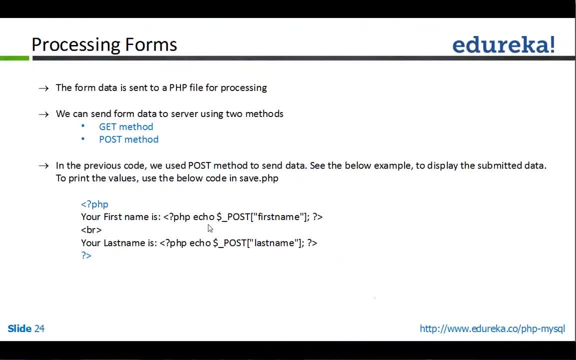 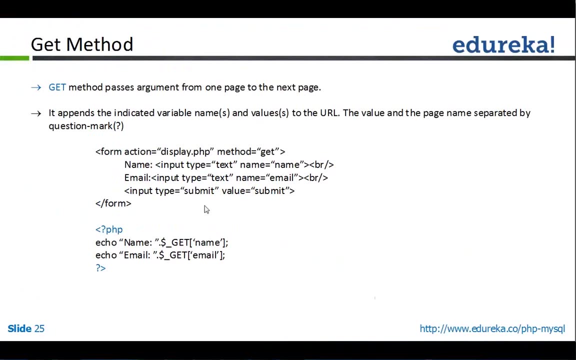 If it is more than that, it will be skipped. So GET is limited, but POST can handle much more data, So POST is always preferred. So here, $POST is used to print your POST data and $GET is for your GET data. 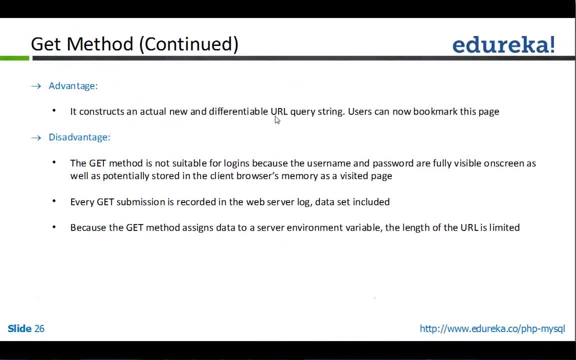 So advantage here is the advantage of GET: It constructs an actual new and differentiate URL query string. User can now bookmark that page. Now, if you bookmark a GET page, next time you will be able to see the same page, But in POST you won't be able to. 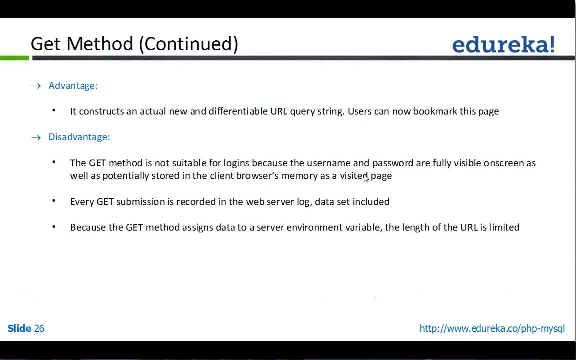 The GET method is not suitable for logins because username and password are very secure and they will be visible. Every GET submission is recorded in web server log, So data it is saved in history. But POST form is not saved in history, So POST is preferred because it can carry more data. 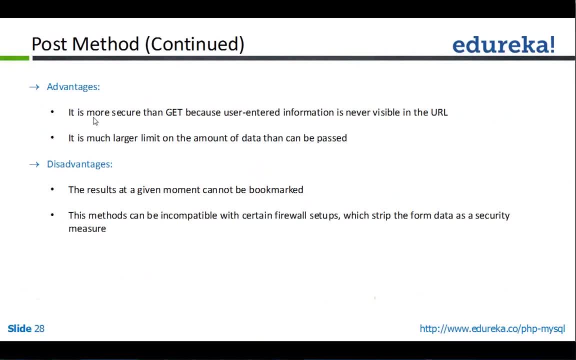 and this is the format of using POST. Advantage is that it is more secure Because it sends the data in the background. It can send much larger data. Disadvantage is that, first of all, a POST form cannot be bookmarked. 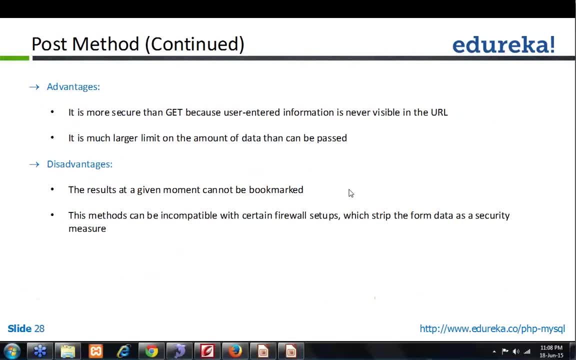 Second, the method can be incomplete with certain. if there is firewall installed on your system, so it will ask, means it will have to pass through that firewall first. Then it will be displayed. If firewall stops some POST data, you won't be able to POST something. 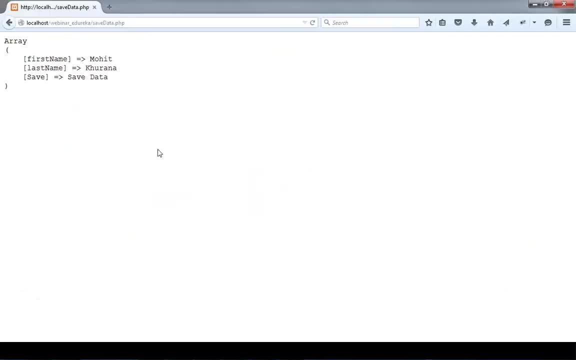 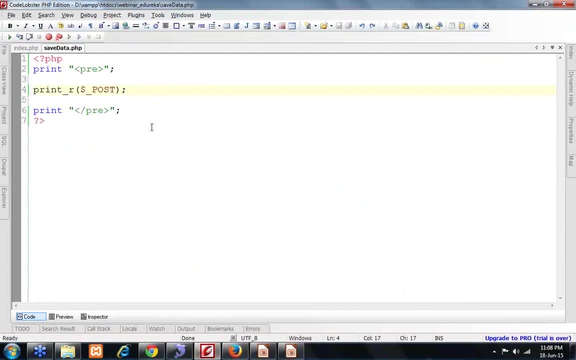 Now let's come to PHP functions. So till now we have seen how PHP prints, how, what are the loops, what are the conditions that we can use with PHP that are similar to CC++. Now we will see what are functions, how we can write functions in PHP. 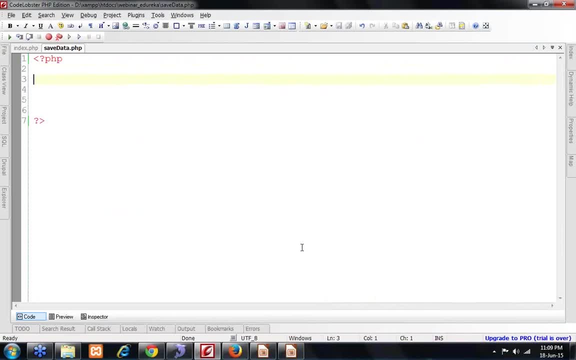 So let me explain function. what function is A? function is a block of statements that you can use repeatedly. I'm printing, I'm having a variable: dollar a is equal to 10, dollar B is equal to 20. I'm printing, print dollar a plus dollar B. now use, refresh your 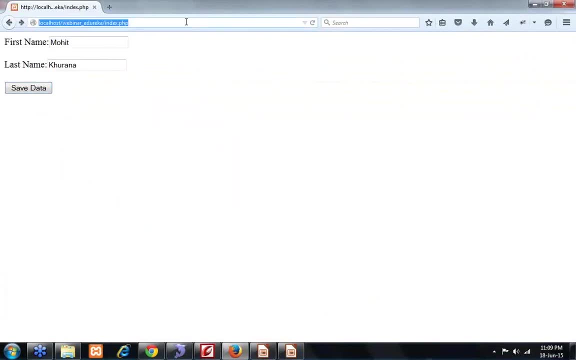 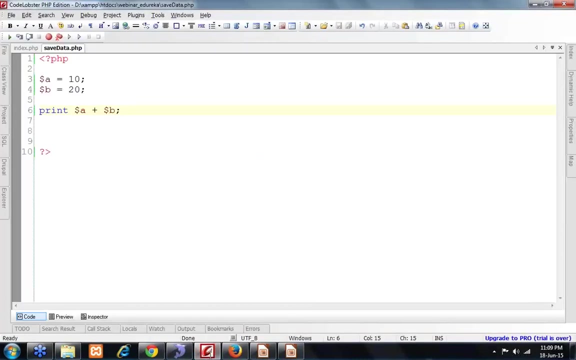 screen. okay, when using same data. you can see sir 30. now, if I want to reuse this sum, I won't be able to do that. so in order to do that, we create function P in PHP. in any programming language, we create functions for usability, function sum. 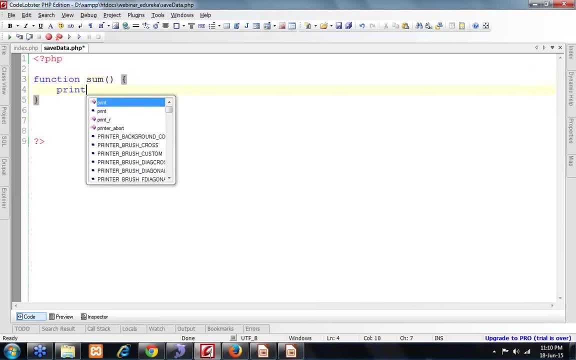 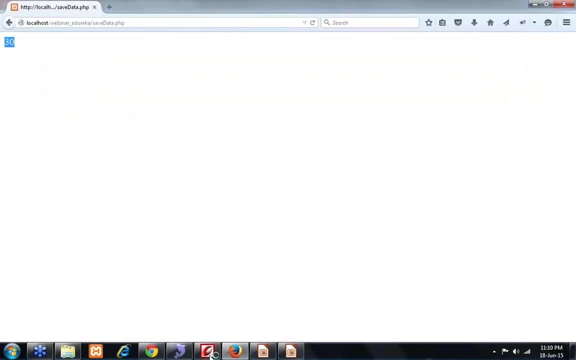 so I will be taking dollar a is equal to 10, dollar B is equal to 30 and I'll print dollar a plus dollar B. now, if you refresh your screen, you will get nothing, because you have created the function but till now you have not called up the. 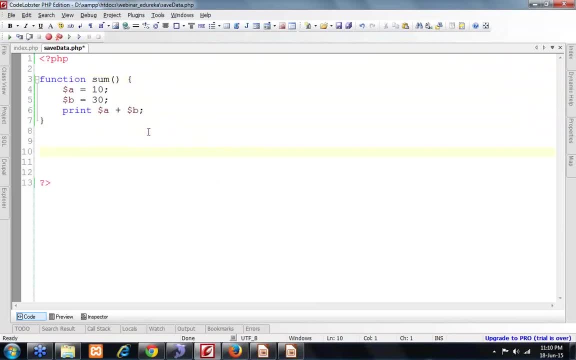 function. so function is a kind of bundle that contains multiple items. in order to excess each item, you have to open that bundle. the same way, in order to access a function, you have to call up that function. so I call up that function simply by its name and parenthesis, and 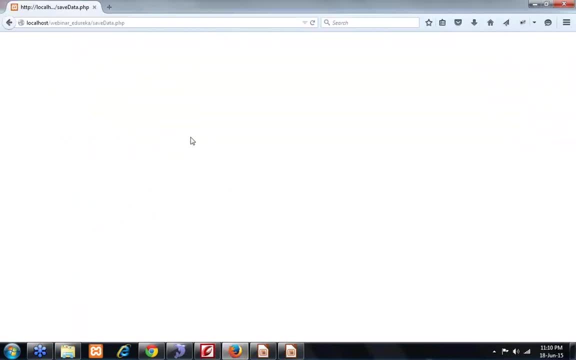 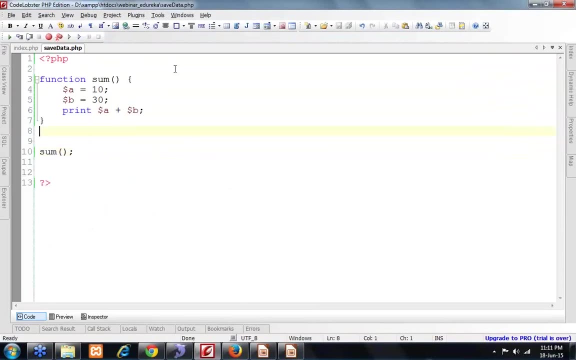 there's brackets. that's it, and now this function will be called and when you will be returned. now you can see. your drawback of this function is that the values are hard-coded inside the function. so if I want to add another, it's simply. if I don't want to add some, I want to subtract, so I will have to create a new function. 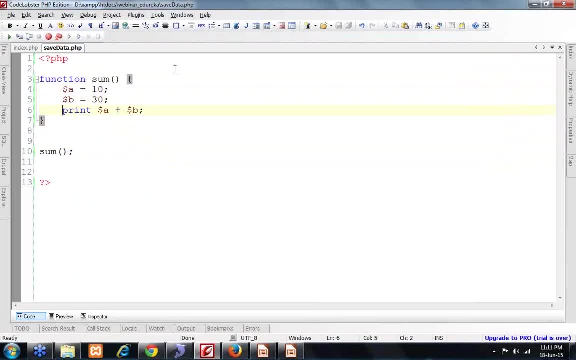 so that is a drawback, because this is a freeze formation that I'm getting. that is always to add. but if I want to do something else with this particular value, I don't want to add them. simply I want to do anything else. I won't. don't want to print it directly like 30, 40. 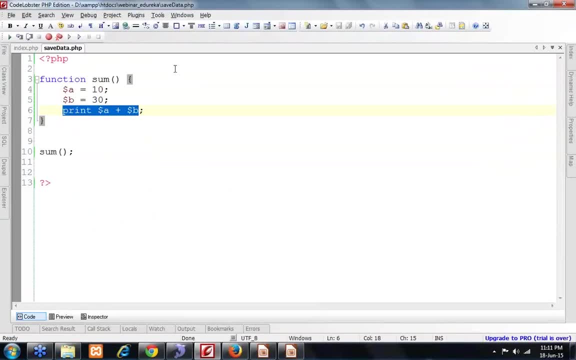 I want to print it with some variable, so in that case I can return the value from function rather than displaying it there. only I can return, or what I can do. $C is equal to $A plus $B, so I'm trying to make PHP simpler for you. some of you might be aware of it. 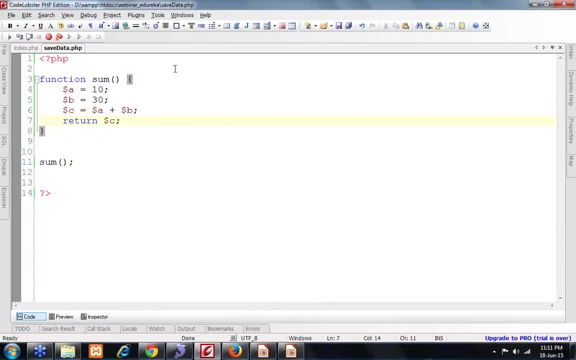 or more programming might have done, but I'm making it simpler for everybody because some might be newer to programming languages. so now, instead of adding the, only adding the value, or we can do: yes, I will add the values and I will return it now as I'm returning something. 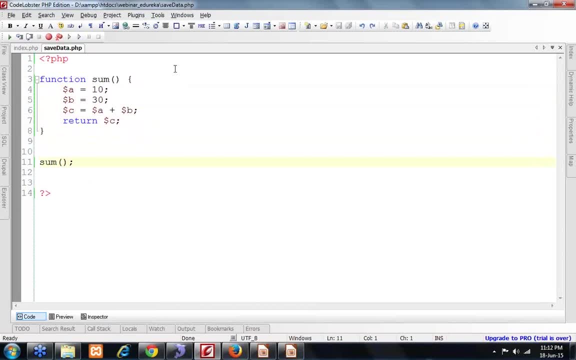 it should be kept in some variable. like: if I'm throwing a ball towards you, you have to close your hands to catch that ball. so the same way, if some function is in something returning something, you have to close your hands to catch that ball. so the same way if some function is in something. 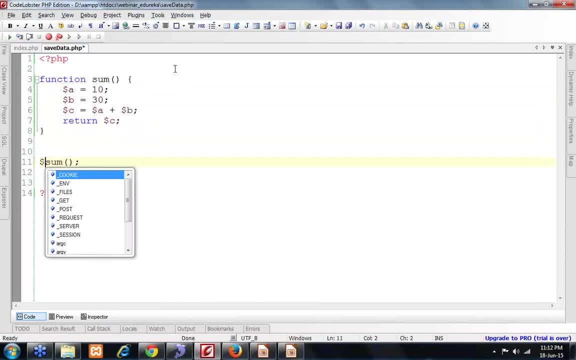 you have to catch that in a variable. so I will be taking one more variable, dollar sum, and I'll some- or it can be any user defined variable and I'm calling up the sum function now. I don't want to print like print sum, I want to print like print. this is my, some outside the function and then I will. 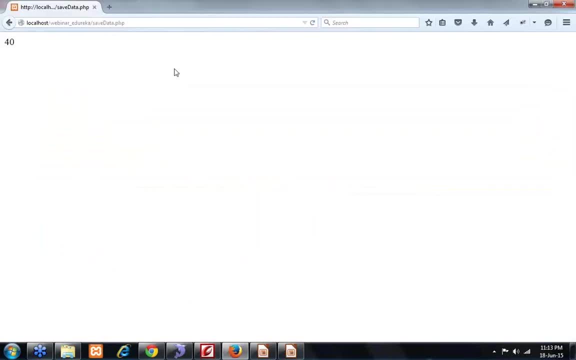 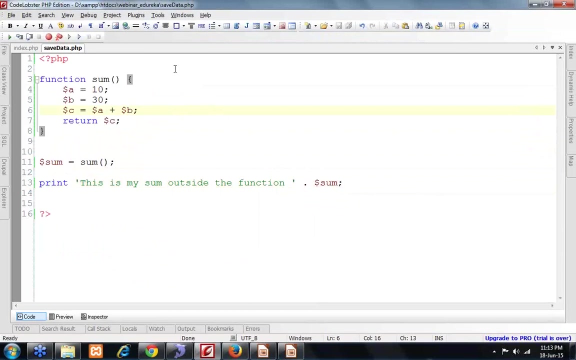 concatenate the sum. now, instead of simple value, you will get printed the complete thing, this is the complete thing. so now function became bit flexible that now, instead of printing the value only, it is giving me the value. now it is up to my wish. I can do anything with this value. even I can do. dollar T is equal to 50. 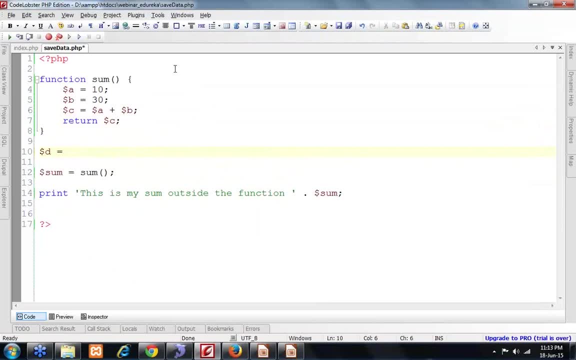 even I can do dollar. T is equal to 50 And I can do: $e is equal to $sum- that I got from the function- and $d I can do it because I got the value. Now it's up to me what I can do with this value. 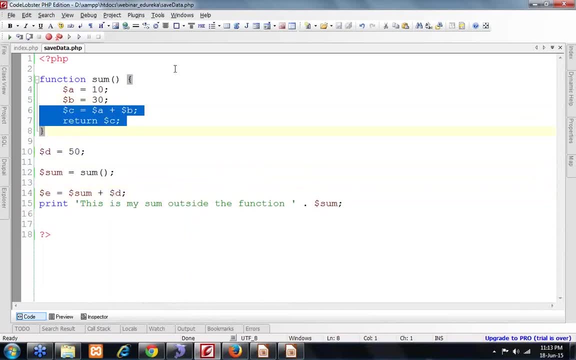 In the previous example it was being printed. It was like print $a plus $b, So you were restricted to simply get the value printed. That's it. Now it is returning the value. Now it is up to you: You want to print it or you want to do anything else with it. 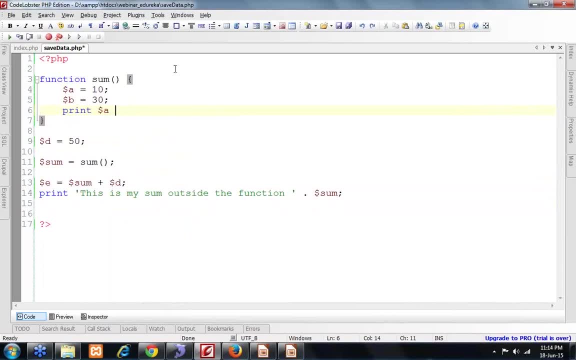 This is up to you. One more flexibility we can add to a function. Now you can note down that this function, the value it is only doing the sum of 10 and 30 always. But I don't want to make it hard code. 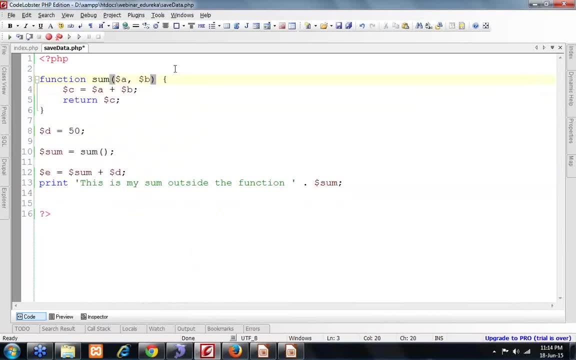 I can pass the arguments to it parameters. These are called parameters. So now, as I'm passing $a and $b as parameter, when I'm calling up this function I have to pass the values of these parameters. I'm passing 10 and 20.. 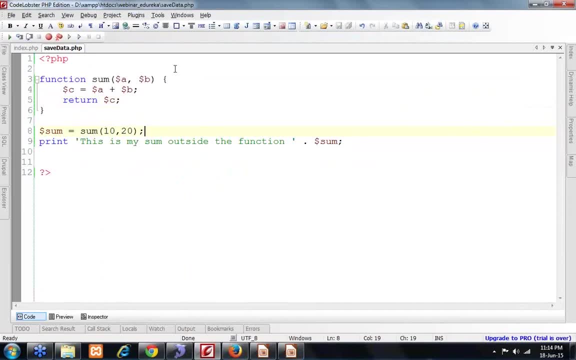 Here you can see: the sum outside the function is 30. If I different values, it got updated. it got updated to 60. So this way function became a bit more flexible that now you are free to print whatever values you pass. 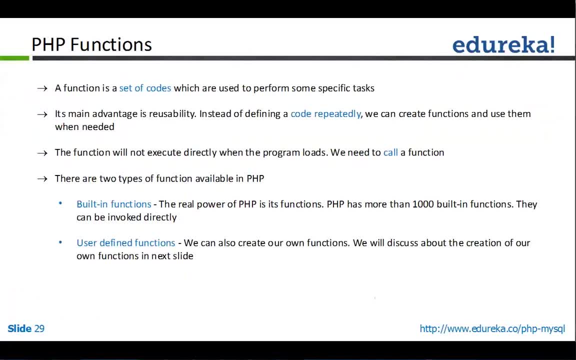 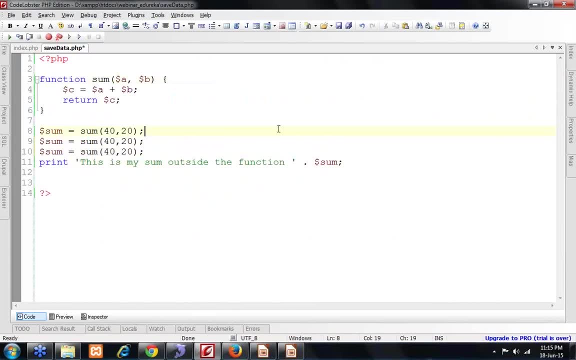 The sum will be accordingly. According to that, it will change accordingly. So this is how PHP functions are created And you can call up the functions multiple times. There is not an issue. Some you can make a sum 1,, sum 2,, sum 3.. 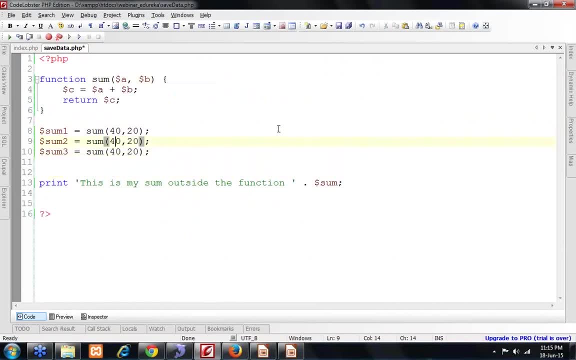 So every time it can print different values. You can pass 40,, 20,, 10,, 30,, 50,, 60.. So all these three will be having different values. Here a tag, you can append sum 1,, sum 2,, sum 3,, 60,, 40,, 110. 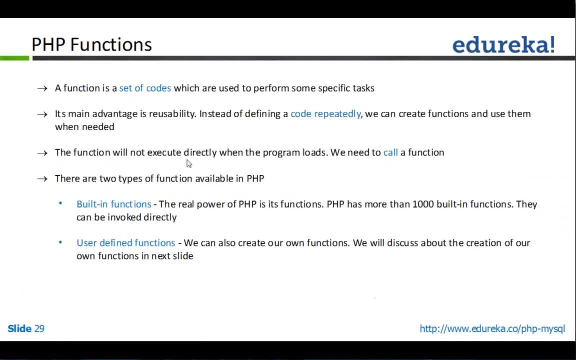 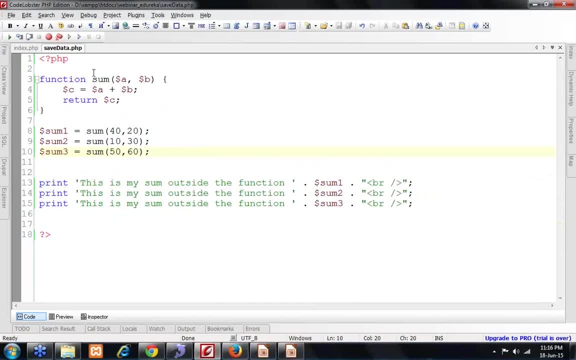 So you can call a function multiple times. This is why a function is used for reusability. So two kinds of functions are there. One is built-in function and user-defined function. This is user-defined function And we have also seen 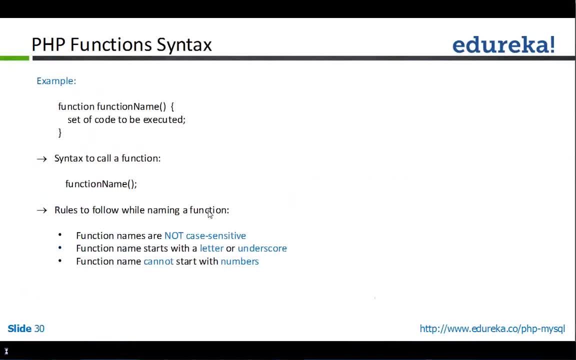 We can also see this. We can also see a lot of functions. I've told you that in built-in function are there in PHP that can be used directly. So here is the syntax of function we have seen. We write keyword function, then user-defined function name and then set of code. 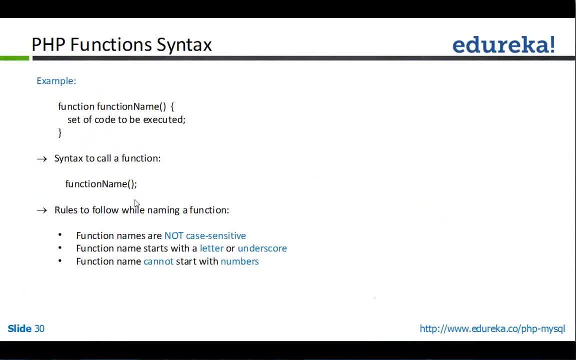 And call that function with name and brackets. That's it. So here are some of the rules. Function names are not case sensitive. So if you are using here sum, you can call sum with a capital S. There's not an issue. 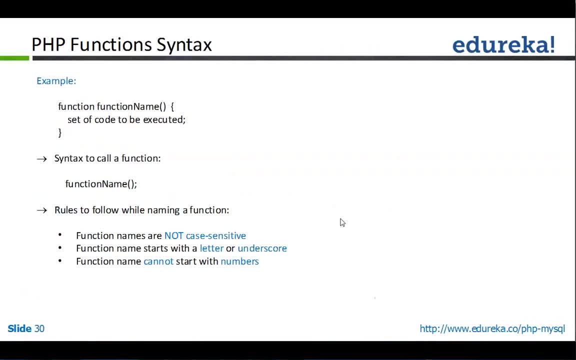 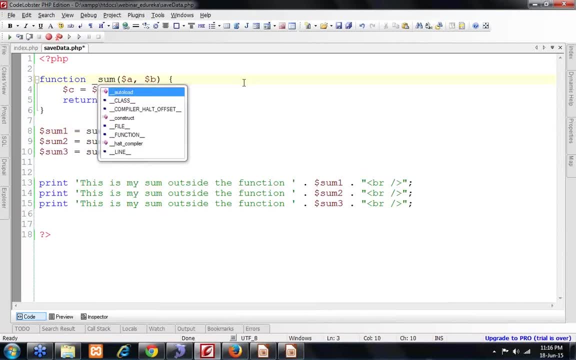 It is not case. sensitive. Function name starts with a letter and an underscore, So function cannot be like 1,, 2,, 3, sum It would be either it would start from alphabet or underscore And number can follow it like this: 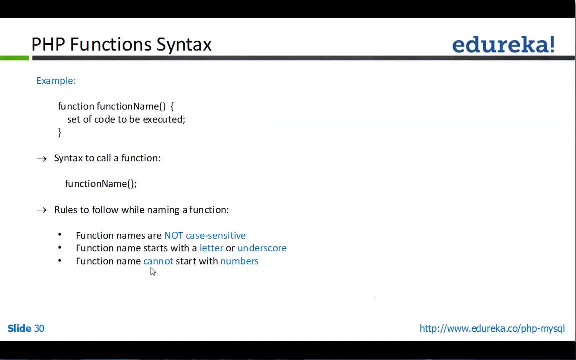 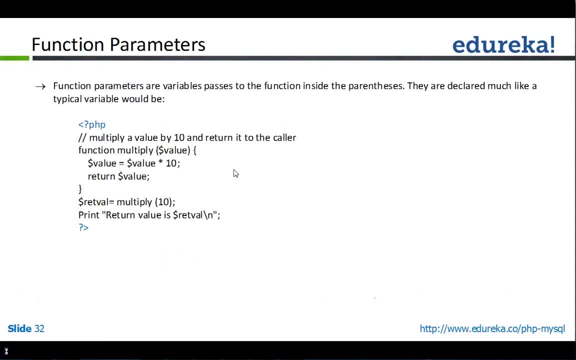 But it would not be in the beginning. Function name cannot start with numbers, So return value. we have seen that function can return a value And that value can be used later. So function parameters. We have passed two parameters here, $a and $b. 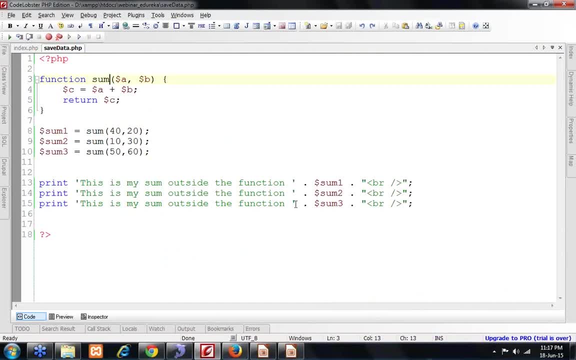 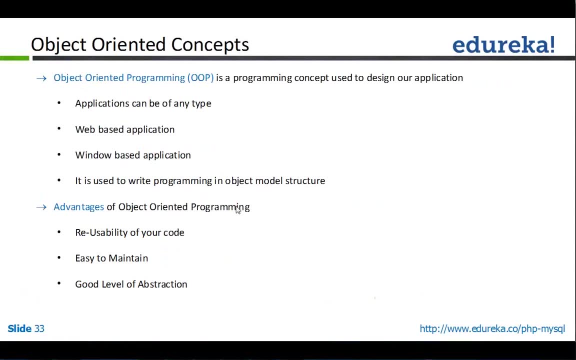 And we are passing their values by calling up the functions And we can simply print the functions. Now let's come to object-oriented concepts. Object-oriented means you can relate object-oriented concept to your real life, Like there is an object called car. 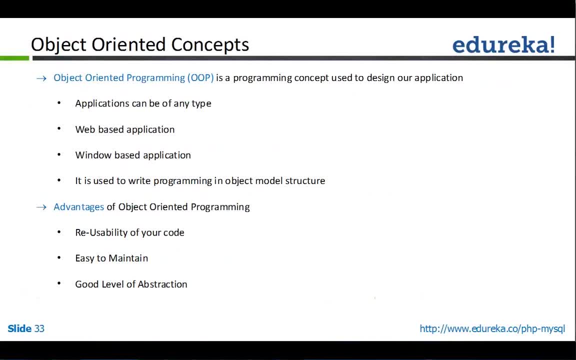 There is a class called car. Now there can be different varieties of that car, like Honda car, BMW car. So car is a class. Honda car, BMW car are their objects. So object is nothing, It's the instance of that class. 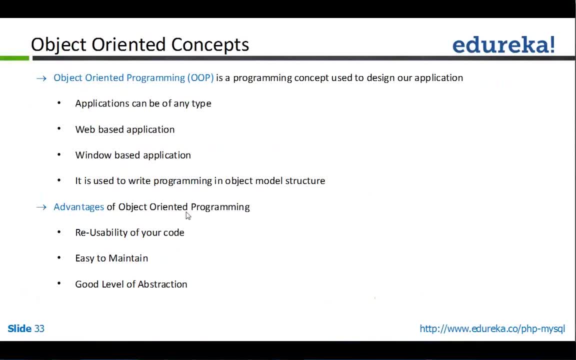 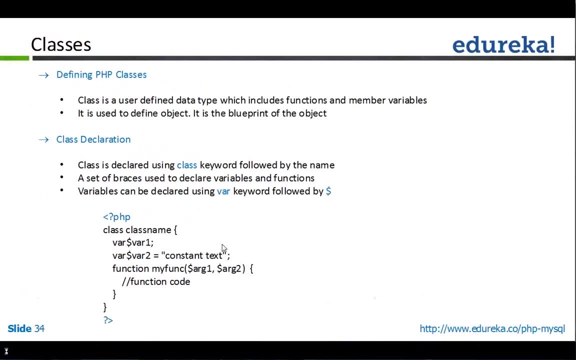 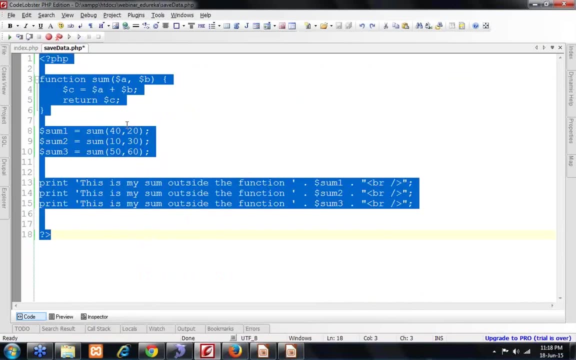 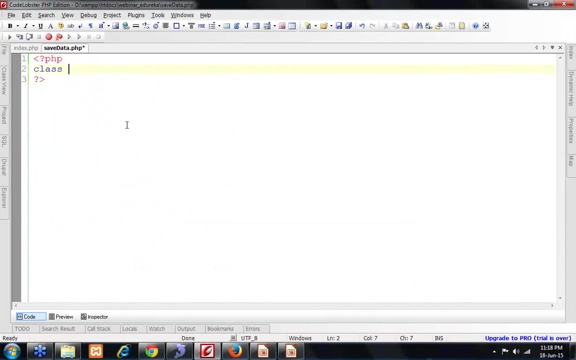 So the same thing we can create in PHP, We can create a class And we can instantiate a class and create the object of that class. Like in PHP, class is basically defined by Class. I will take a class, like we can say: car. 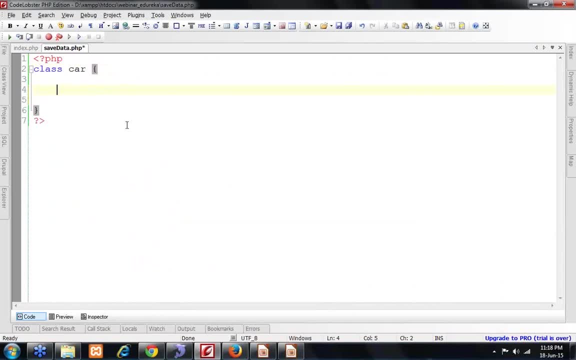 So inside car I can have either variable, but I can have either function. So I'll be creating a function Test Here. I'll be printing. This is my first class function, So here is my class. This is my class. 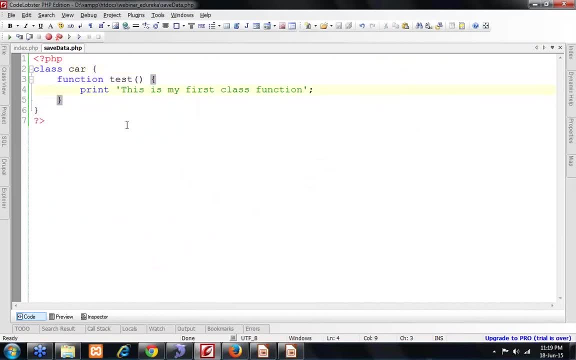 So I can define a class like this: I've created a class car And I'm printing, I'm using a function inside. Now I cannot call this function like that directly. It will give you an error. Call to undefined function. 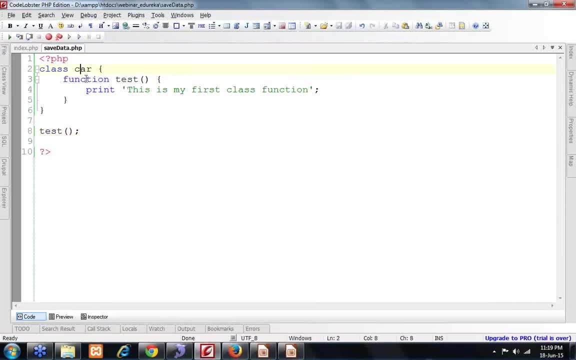 Because that function is now part of a class. In order to call that particular function you have to create the object of the class. So I will be creating object BMW. So new keyword is used to create the object of a class New. 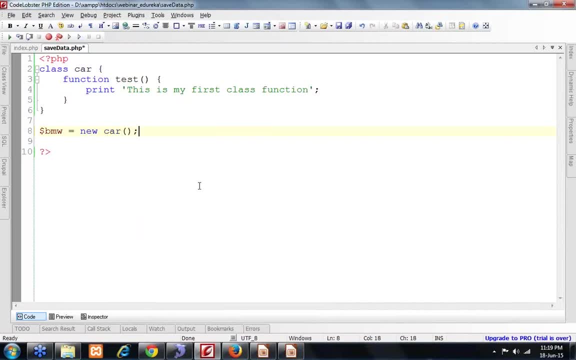 Then your class name. So this way you can create the object of a class Now in order to call the function of that particular class, Because this BMW is now an instance of class, So it can use the functions of the class. 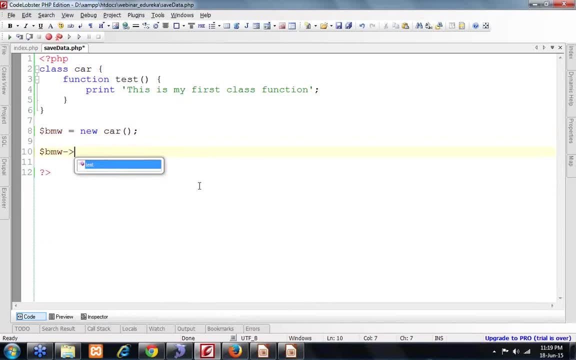 So it will be BMW, then arrow and then test. Now it will print the result. This is my first class function. So we define a class. Inside that class, we define a function And we create an object in order to call that particular function. 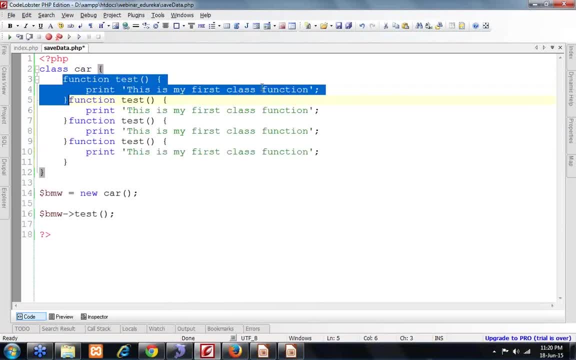 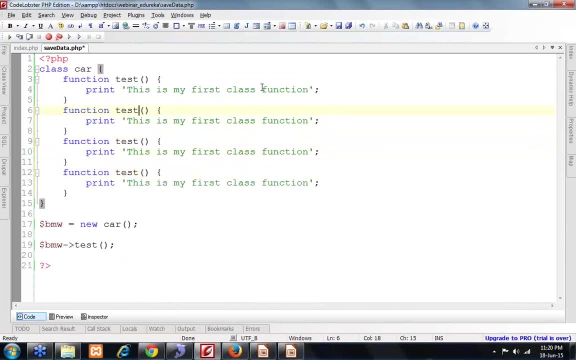 So, once the object is created, as many functions are there, like function test, test one or test two, test three, like that, so all will be called in the same manner. I can write. this is my second, third, this way. 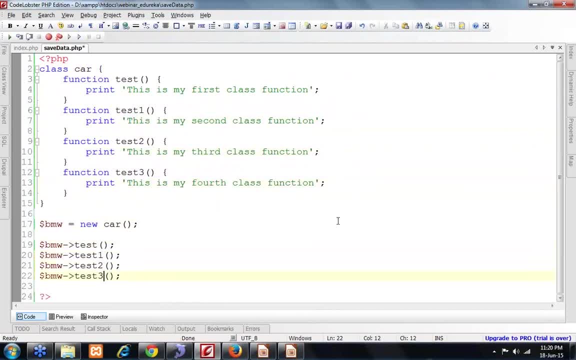 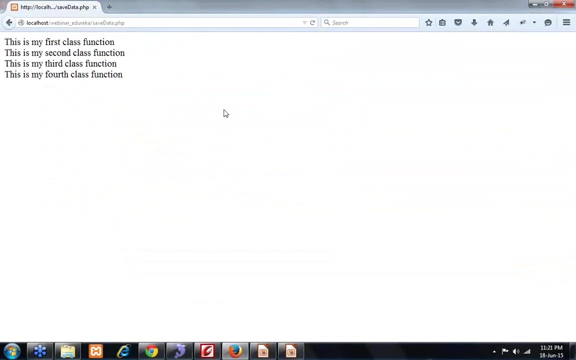 So I'll be calling up test Test one, test two, test three, like this: So all will be appended on the same line, So we can add BR tag Now. first function. second function, third function. fourth class function. 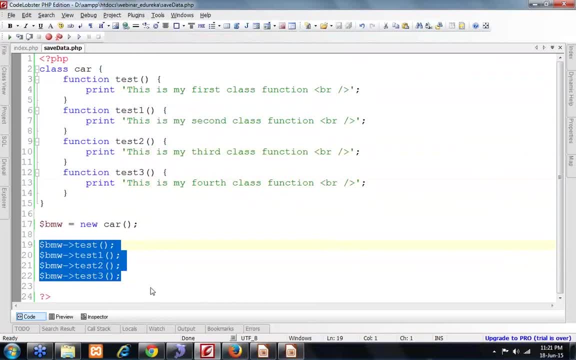 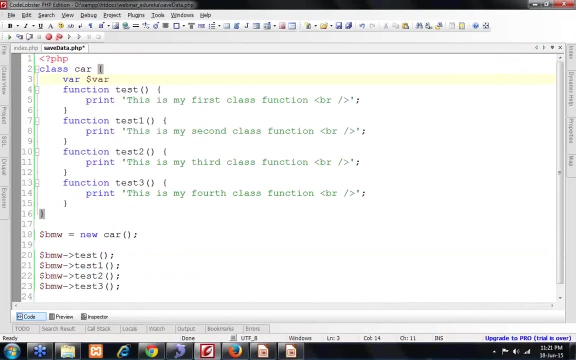 So this way we can create functions and call those functions out that particular class. So this is my class name. Then I can also define the variables inside the class, So where variable in classes I can define with where keyword, $where, $where one or $where two. 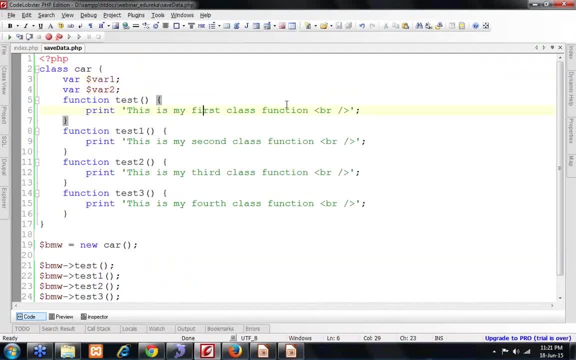 And in order to use the particular variable inside a particular function with $where I can write, I am going to append that variable. Now I cannot write directly $where one Like this. I will get an error: Undefined variable because class variables. 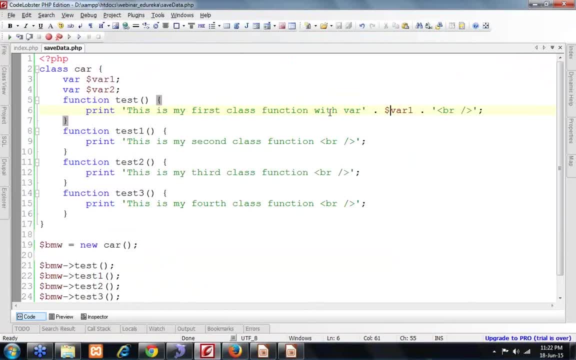 that we have defined. yes, we have access specifiers, right, But I'm taking the basic right now, So I will be using $this and then your variable name. Now it will print. this is my first class function with $where. 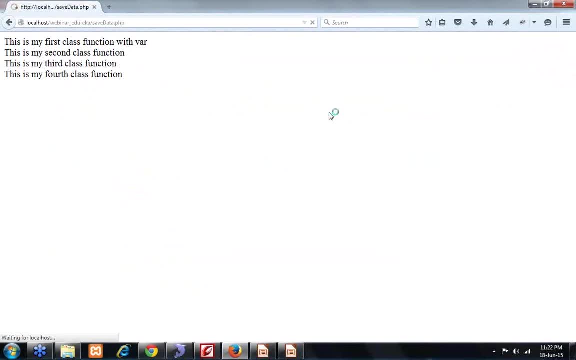 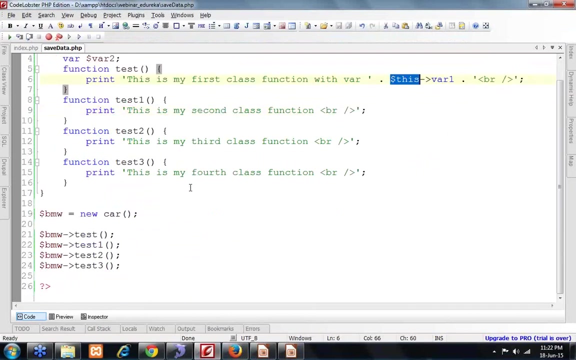 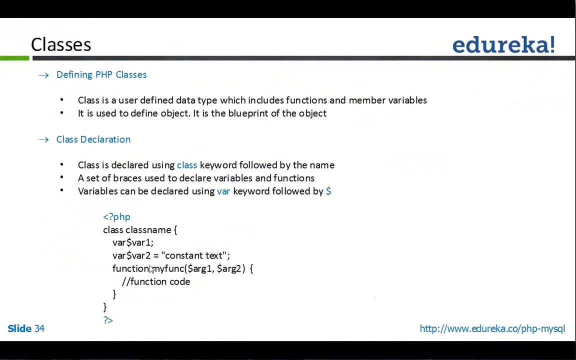 And $where. if I give any value to this, it will print the value Variables we can simply use by $this. So there are access specifiers- public, private, protected- as variables With other programming languages. So this is how we can declare a class and create the functions. 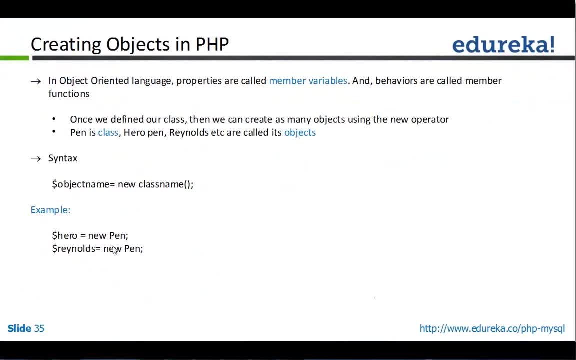 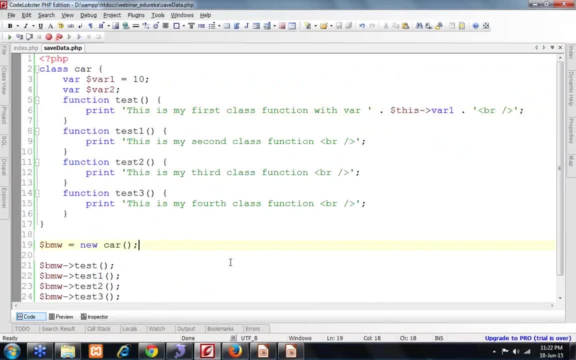 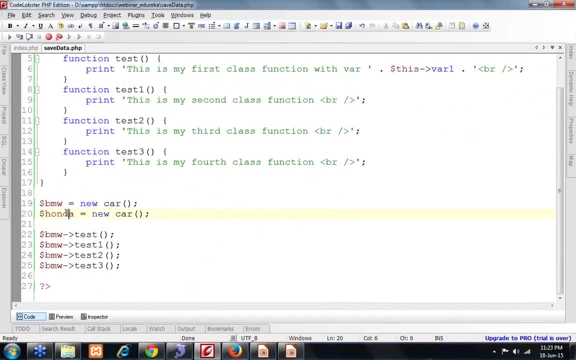 So this is the syntax of creating object for that particular class, And I can create multiple objects. So instead of a single, I can create BMW, Honda, So both will be having their own functions. Now this can call Honda can call the same functions. 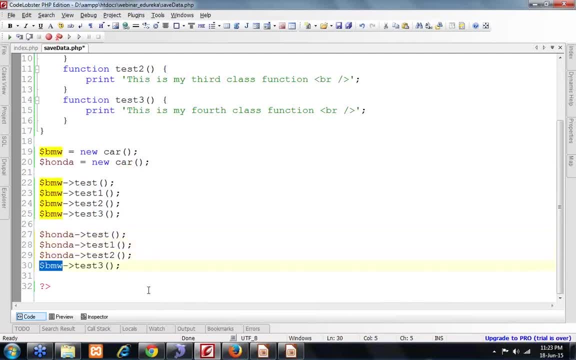 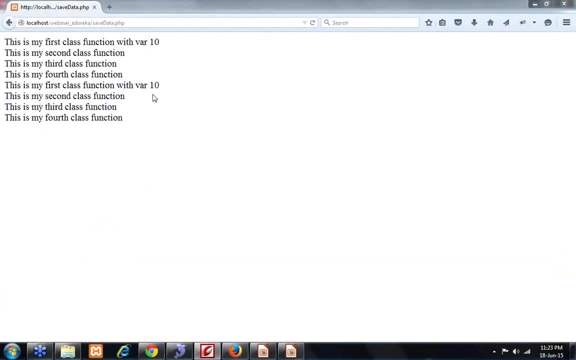 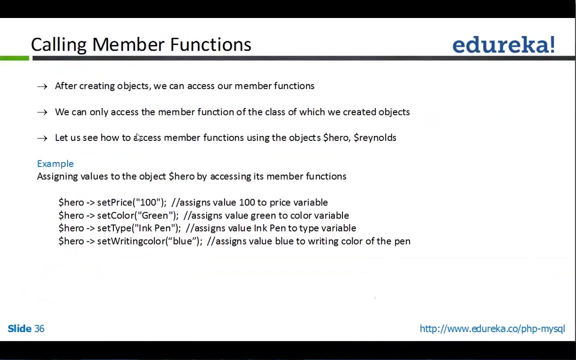 So Honda and BMW, both are different instances of the class car, So both will be having then their own functions and own values. So here is the example or method of calling up a function of a class with object, And then the other will be a function. 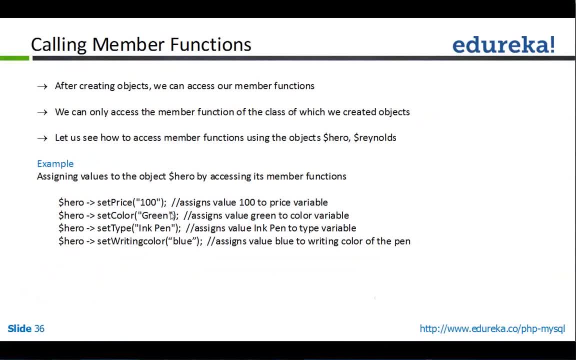 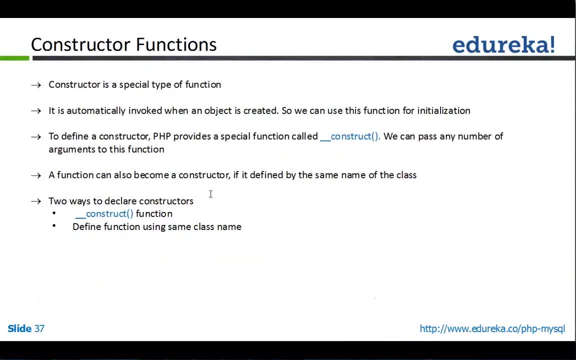 So here is the example or method of calling up a function of a class with object, then function name and then argument that you want to pass simply is the same way you can pass the arguments to a function, as we have seen while declaring the function. so 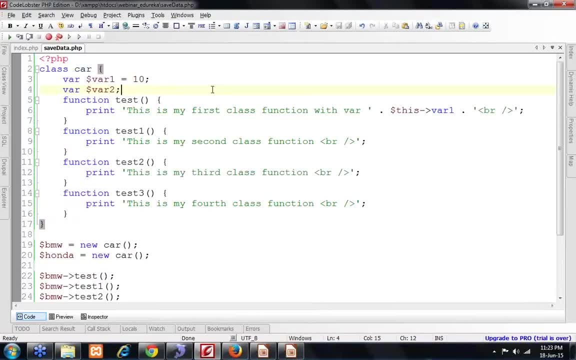 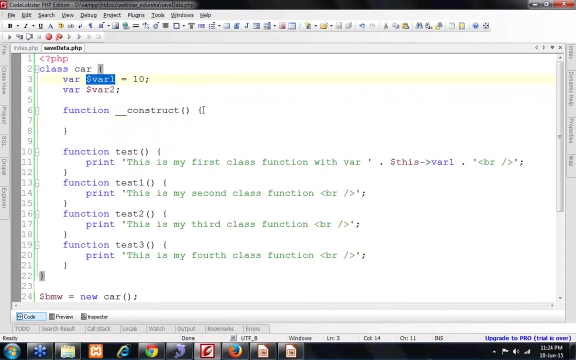 now there is a function called constructor. so constructor is a function that is basically used to initialize a class. so in PHP we take constructor functions with underscore, underscore, construct keyword. now I will let you know what this construct means. so I'm taking $v1, commando v2. now I will show you what that, what this constructor means, and we're taking. 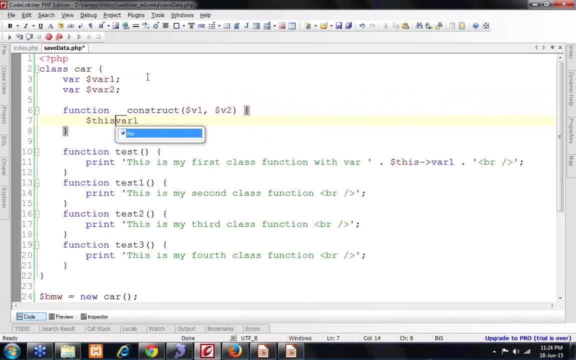 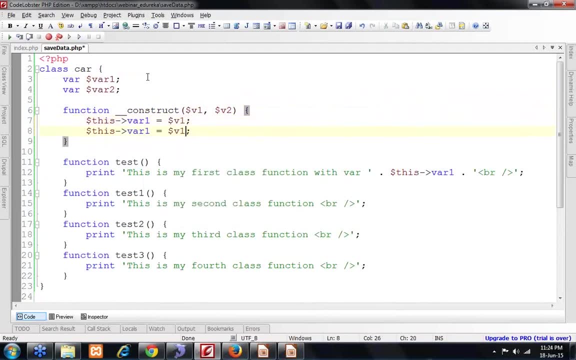 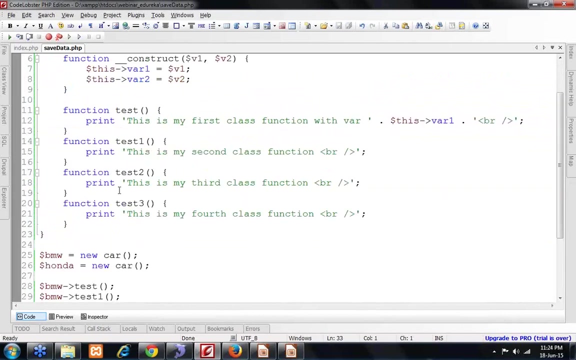 $v1. $v1 is equal to $v1 and The same way where to $v2. now, if I'm taking constructor with arguments, so constructor is a function that initializes a class. now, while calling up the class, creating the objects of the object of that particular class. like I'm 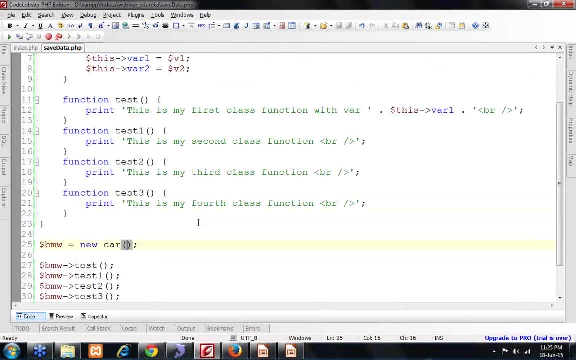 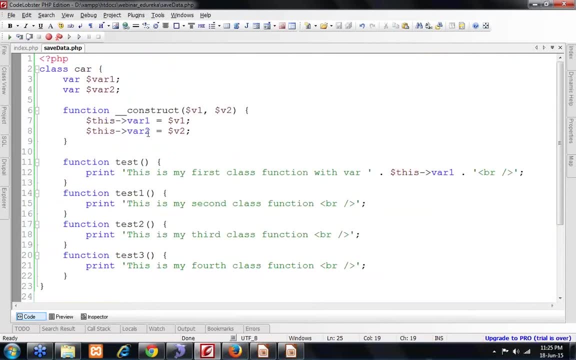 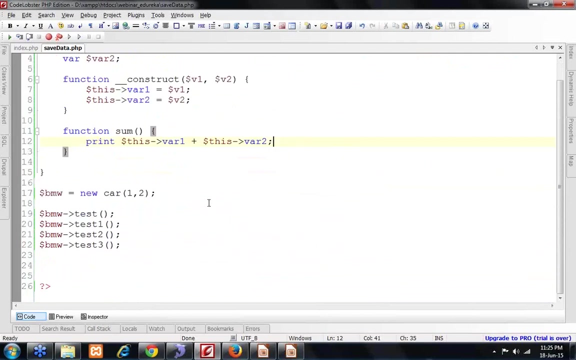 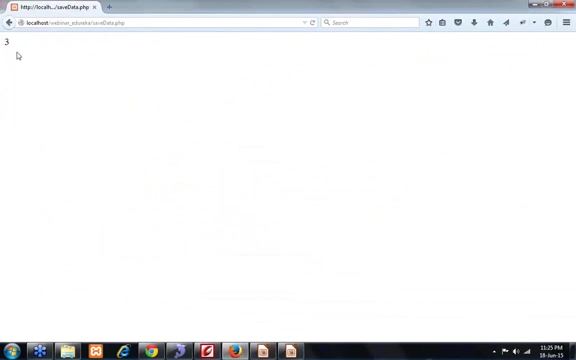 creating this BMW. I have to pass the values of both 1 comma 2. I can pass those functions toAngle class, thanks, and I can create a single function sum. print US this where one $ this. now I will call up the function sum. now you can see three get printed right, because what a constructor function. 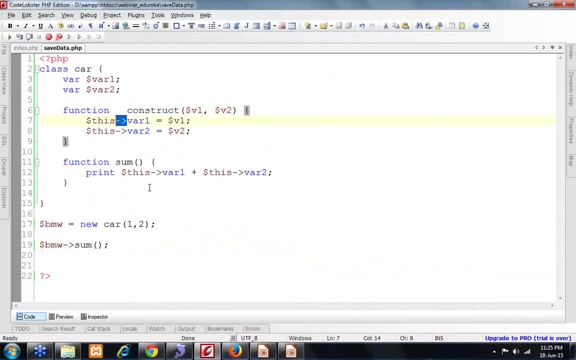 means arrow is simply two point to that particular variable. so constructor is a function that is used to initialize a class variable. so initialization means while creating the object of the class, you have to pass all the values that are being used in into a constructor. so here I'm using $V1. 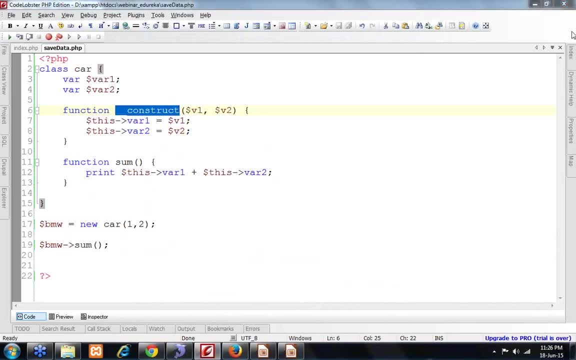 and $V2 in my constructor. so here it is $v1 and $v2. we got the sum of that. so constructor means that is used to initialize a variable, the class. I'm passing both the values and getting the sum. if I change the values to 5 and say 5 and 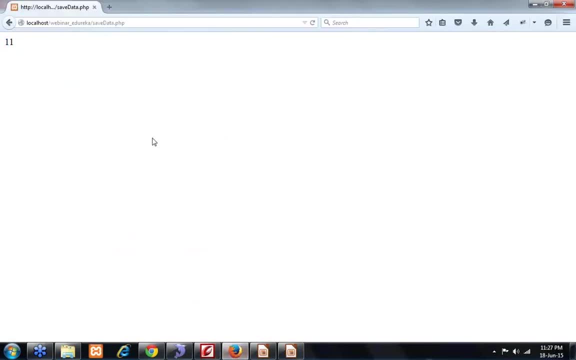 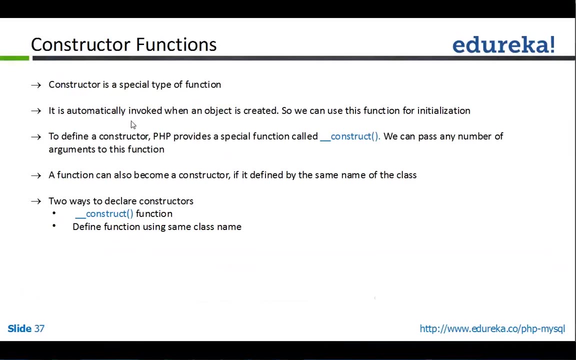 6 and I get it printed. it will print 11. so constructor is a function that is used to initialize a class. so construct is a special type of function. it is automatically invoked as the object it created. yes, destructor concept is also there in PHP, same as C or C++. automatically. 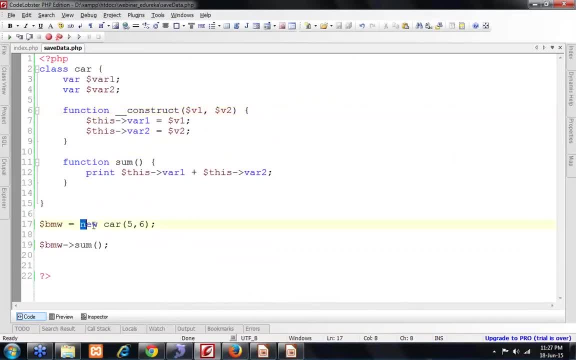 invoked when the object is created. so, as we created the object and pass the values, these are automatically assigned to where one and where two. we we are not calling up the constructor function, like we don't have to call up the constructor function like this. this would be: 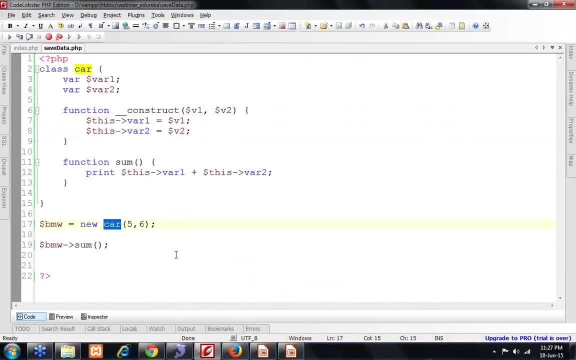 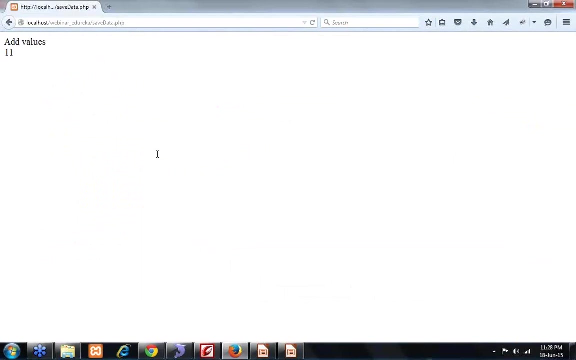 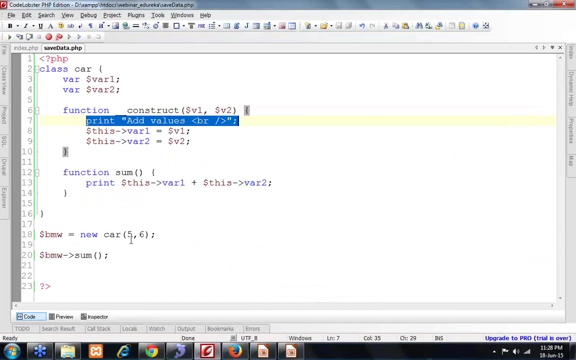 automatically called as we create the object. so as this object is created, this function is automatically called and these values are assigned. if I print something, add values like this: while values is printed, I don't have to call up construct explicitly. it is called internally as a created object. to define a constructor, PHP provide us special function called underscore. 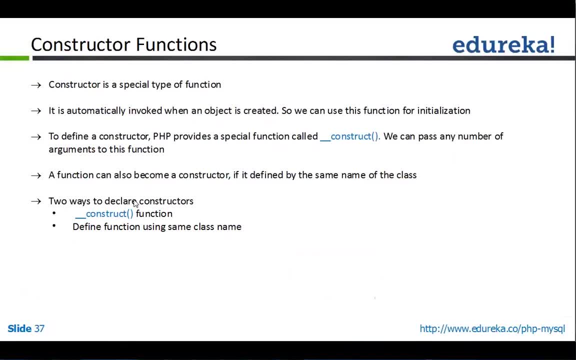 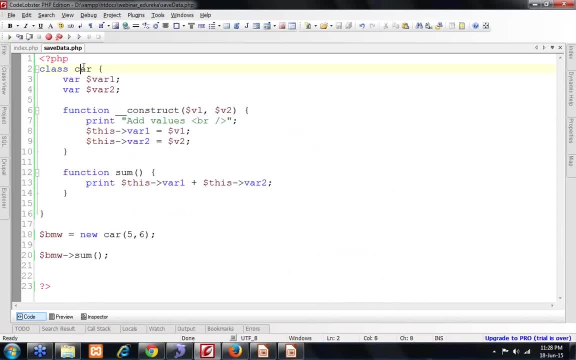 the square concept. we can pass argument to this function as I have passed. then function can become a constitutional ā. it is time so to. two ways are there to define a constructor in PHP. one is using underscore, underscore construct. second, we can take a create a function with the. 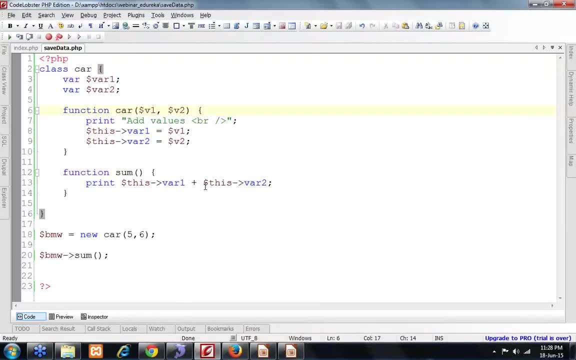 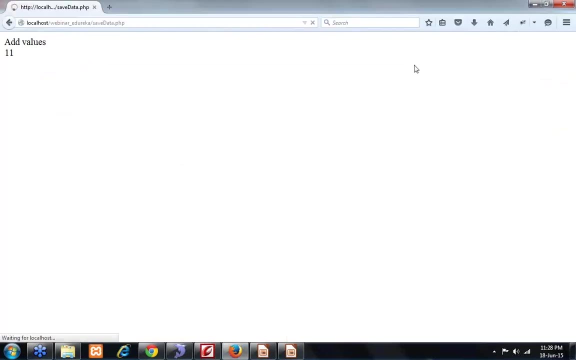 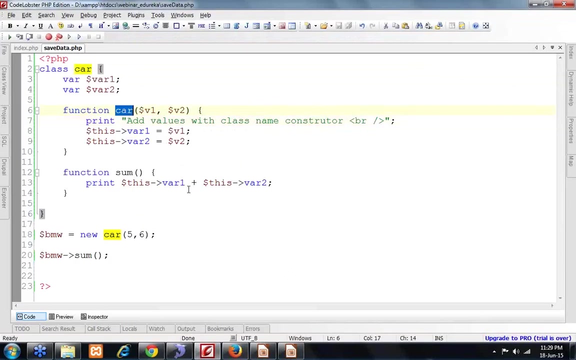 same name of the class. now both mean the same thing: add values with class name constructor. so here you can see. we can create the sector in two ways: either underscore cristo construct function or the same new function name as of the class, so it will be called automatically as we create the object. so two ways are. 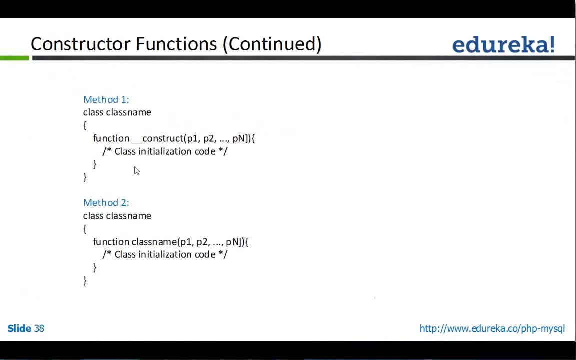 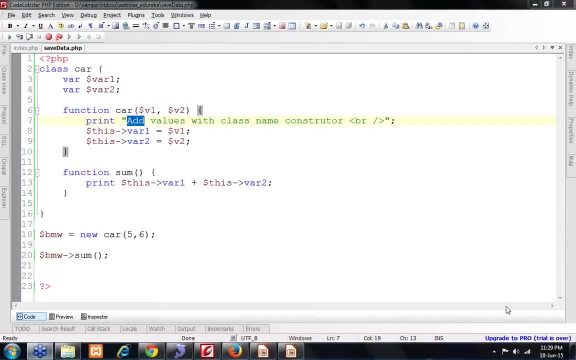 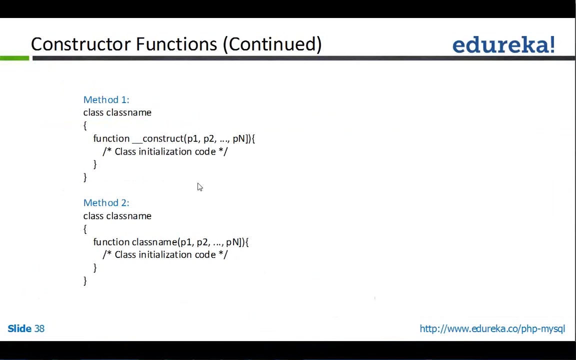 there to creative constructor. so here are two methods: one underscore into so custom, then the class name itself. yes, Aditya, print can have or cannot have beckets, they're not an issue. no, multiple constructors are not allowed. constructor is basically to initialize the value. so single function is enough to initialize the value. where to take? 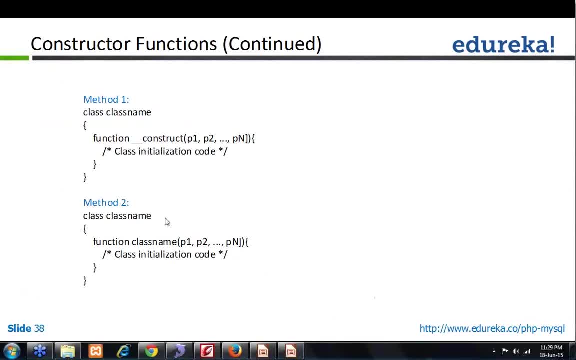 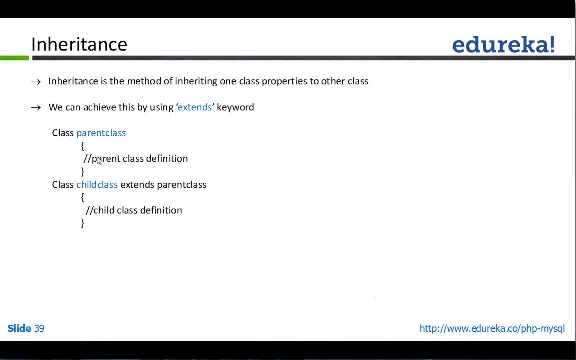 multiple functions. so two methods are there: one underscore, construct and then class name, now inheritance concept. this is similar to CC plus plus. you can create a class and a child class class you can create that will extend your period class. so same way as we have in P and PHP- and sorry, C and C plus plus. 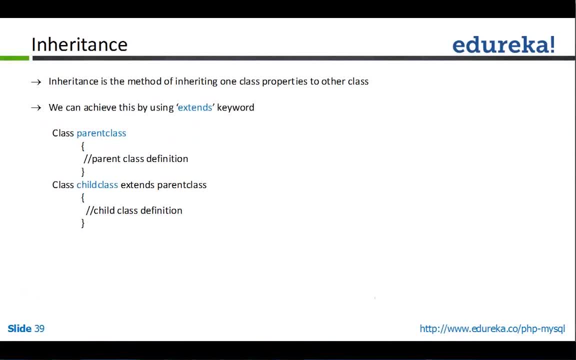 we can have parent class, a child class. for example, you might have inherited some of the properties of your parent, so you will be the child and your parent would be the master class- parent class. so a child class would be using the functions of parent class if child class is extending the parent class. so 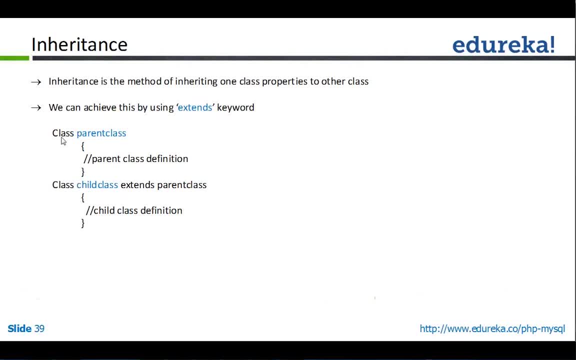 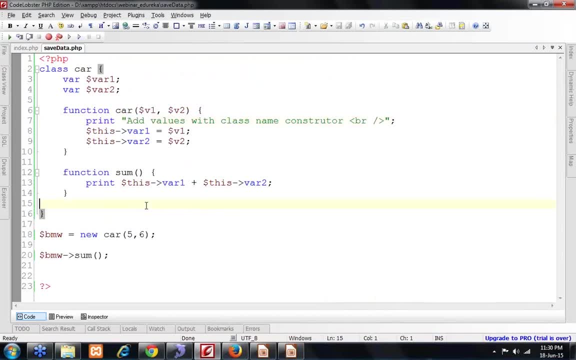 outstanding extension is done, inheritance is done. with this syntax, parent class, you define the as you are defining the classes. this is the syntax. you will be defining parent, this class, car and child class. you can define like class, child car, like that, and it will extends car. now, child car can call up the functions of car as it. 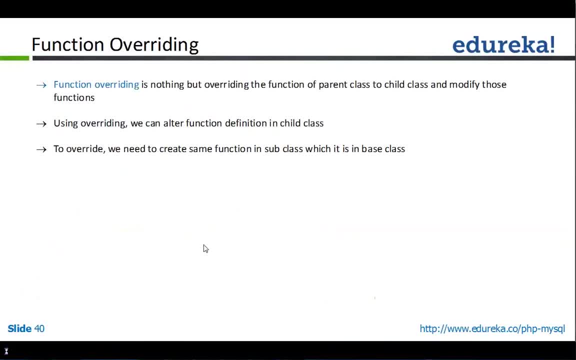 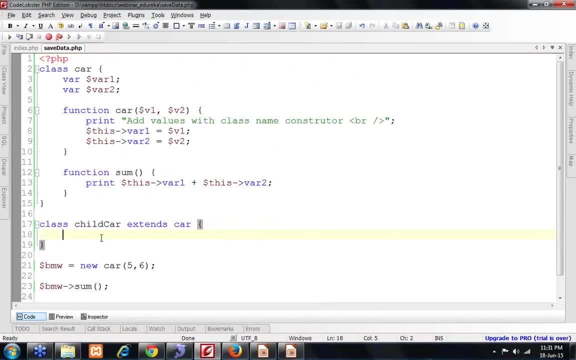 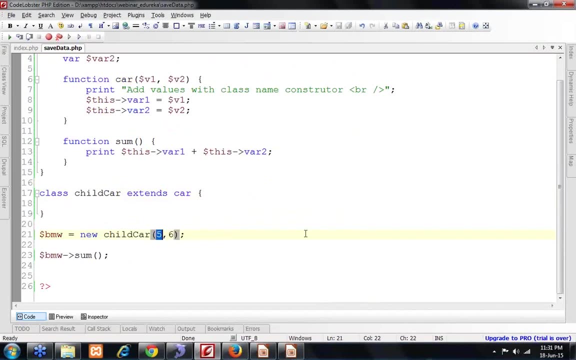 is the child of this car class, so function. so let's first see that how it can do. now I've created a child class that ends car. now what I will do? I will create the object of child class, so let's remove this. I'm doing the sum and 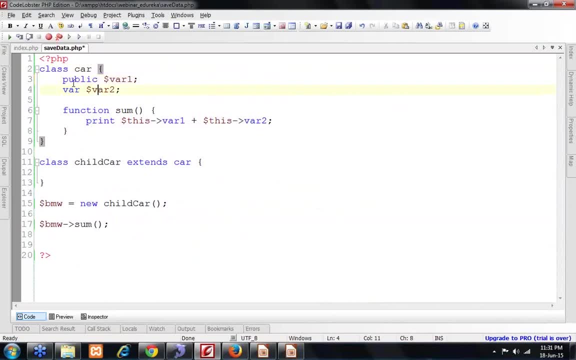 I can take it public. so public means that can be used publicly. so three things are there that we cannot discuss right now. three access modifiers are their public, private and protected. so I'm taking publish for now because I want to use it in my child class. now I'm creating object. 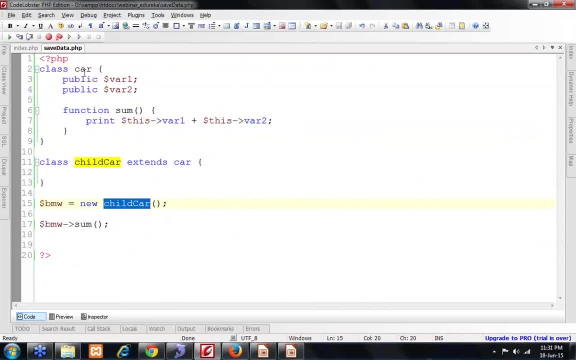 of my child class rather than parent class. now I will be taking, I will be defining value of variable. so three access modifiers are there: public, private and protected. so i'm taking. Now I will be taking, I'll be defining value of variable. sort: ну, I will say: 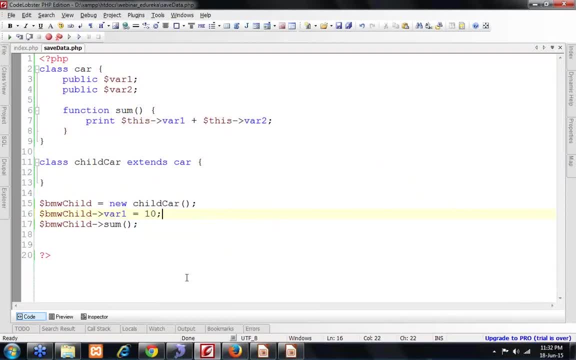 as variables are also part of class, I can give it values outside the class if they are public, where to then by child? I am calling C. this is the object of my child class, but I'm calling up the functions and variables of my parent class because child class is inheriting my parent. I haven't written anything for. 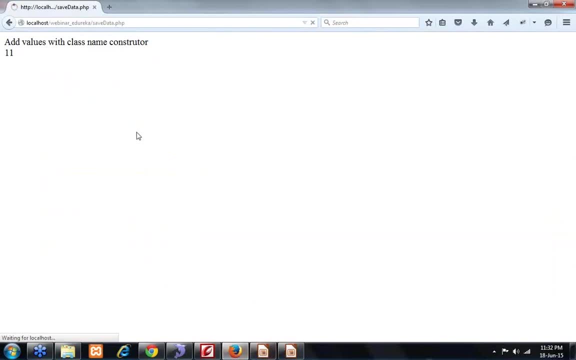 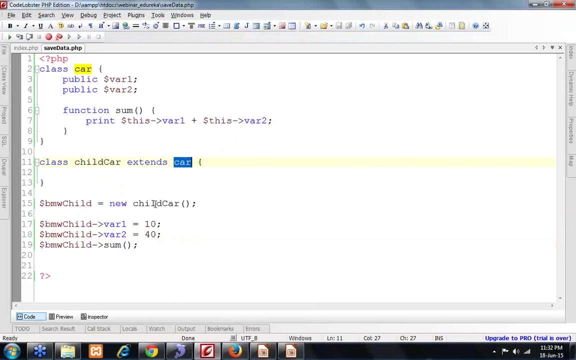 child class, so it is printing 20. if I make it 40, it will print 50. so here you can see. I have created a class- child class- that extends parent class, car, and I have created object of child class, not of the parent class, and I'm using 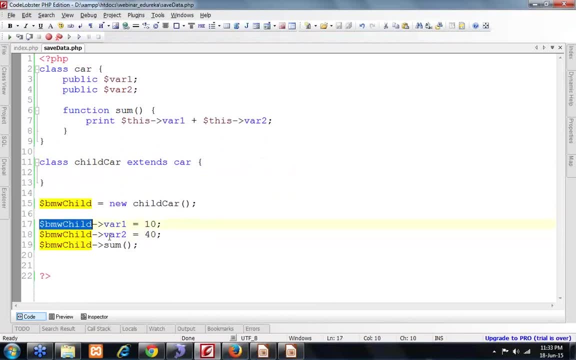 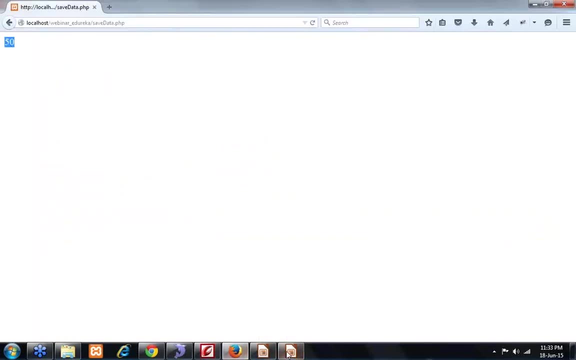 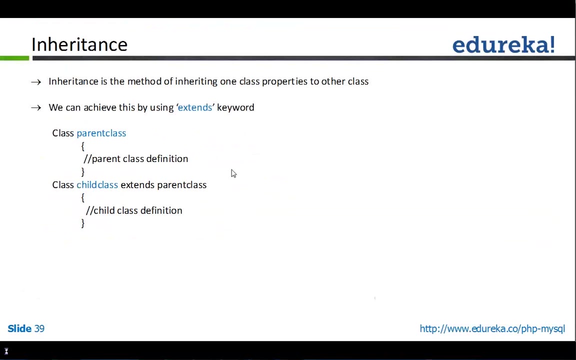 variables of parent class. throw object of child class and use a calling of the function of parent class and it is doing job. doing the job it is printing up because if a child is created for a parent, child is free to use parents functions or variables. this is called. 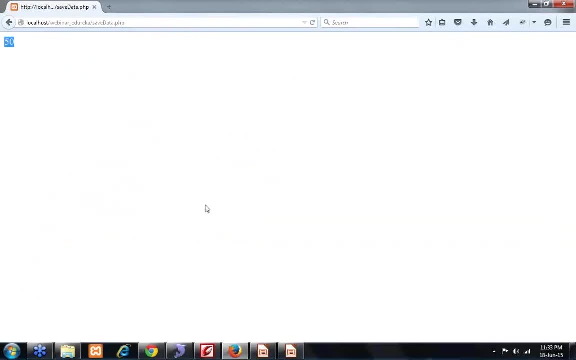 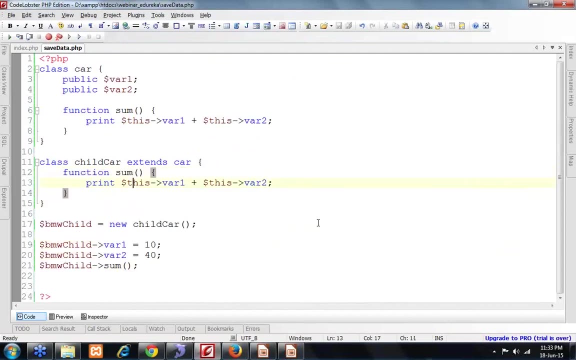 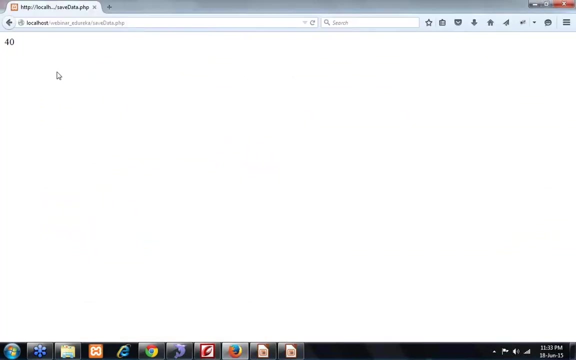 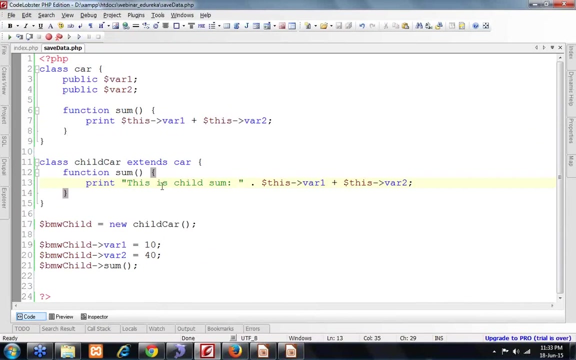 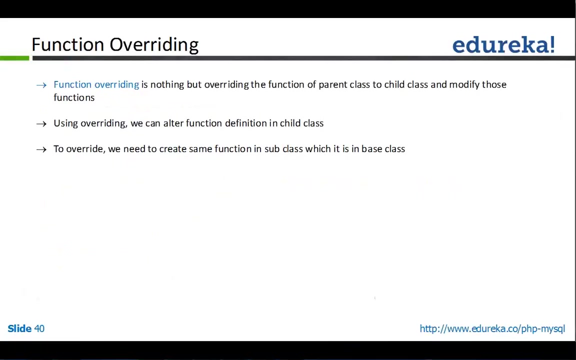 inheritance. now we can use function overriding. overriding means if there is a function in parent class and I create the function with same name in the child class and if I call the function now, now it will print. should print. okay, let me check. so function override is nothing but overriding the function of the parent. 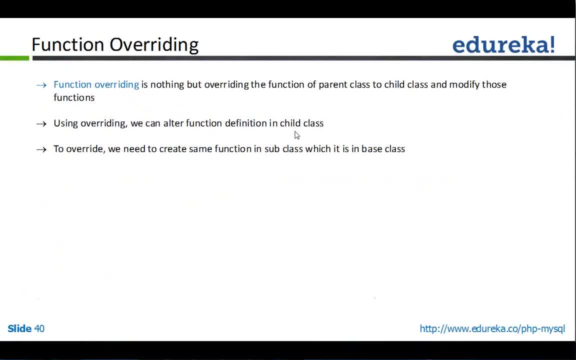 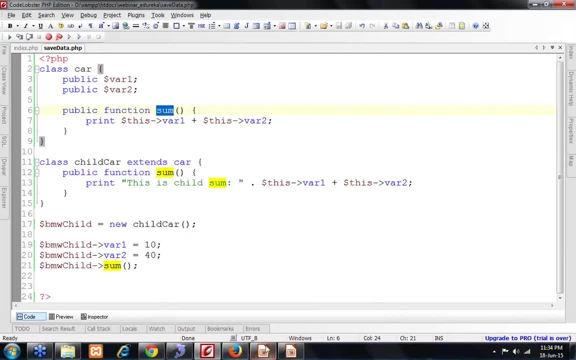 class to child class and modify those functions overriding, we can alter the function. so basically, the same function that is in the parent class you can create in the child class and that will now override the parent function. I don't know why it is not overriding here. I'm going to just do the duplicate second one and then come back for a second. 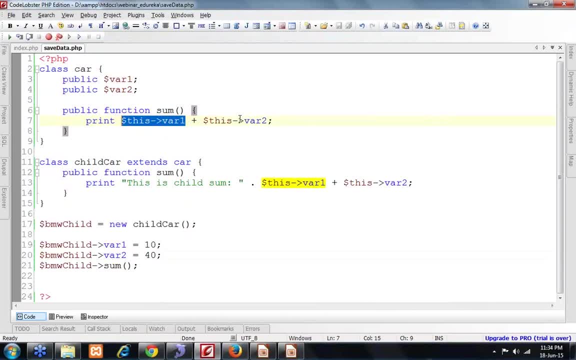 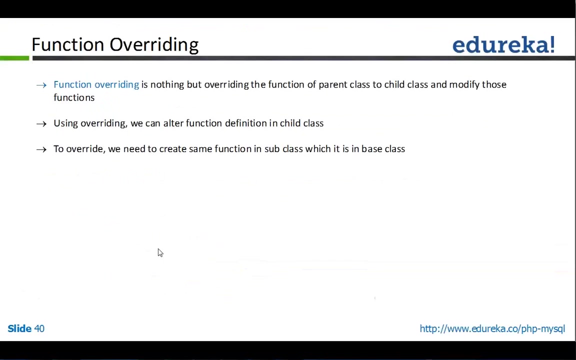 okay. so now, in last instruction I put, there is the function of the parent house. this function can't be turned down. this has to be subject聊: motivo um. so it should be fine is some issue? but in this case this sum. this sum should get printed, not this. 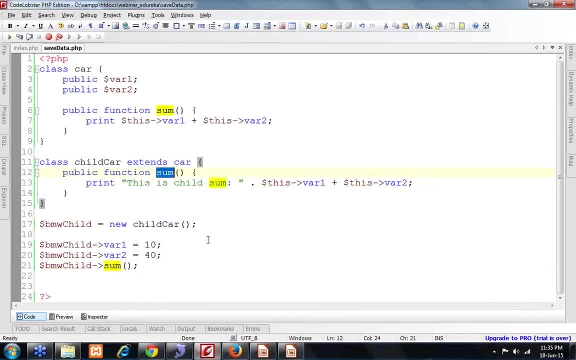 sum. this value will get printed because this child sum would override the parent class. yes, Aditya, we can create the object of parent class as well. there is not an issue like this. we can create the parent as well and a call of the parent functions, but parents will not be able to call the child functions, only child. 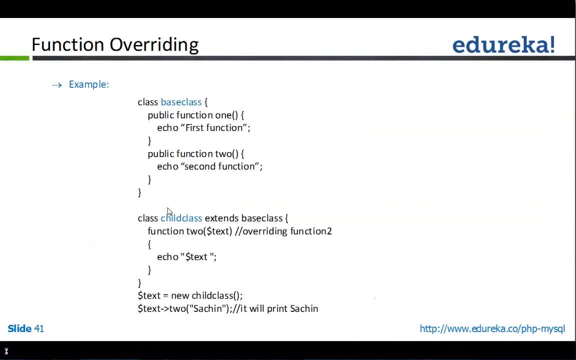 will be able to call up the parent functions. so here you can see. let's zieee the example. I have created function one and function two and same function two is now created in child class. and. and now if I create the object of child class and call up two, not two of child class, will? 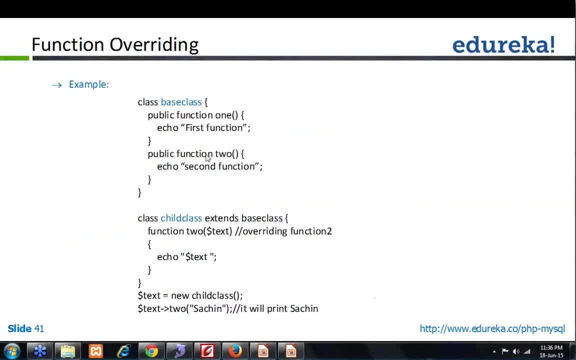 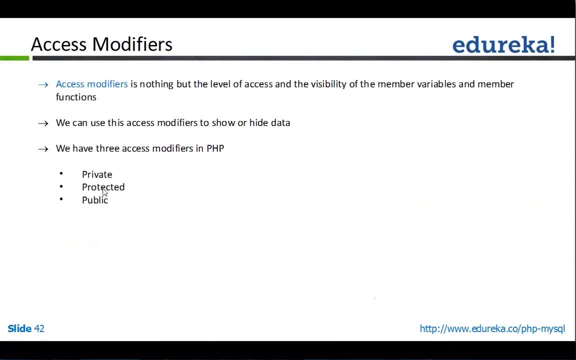 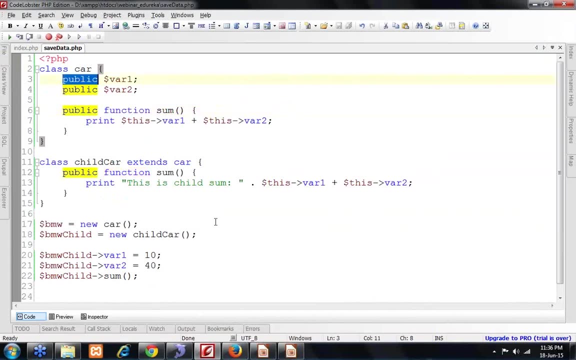 be called, not of the parent class. this function will overwrite the function of parent class. so access modifiers private, protected and public. so public means that I can use that inside my class or outside my class, anywhere I can use so here, if you see, I have created these two. where variables public, I'm able to access it out if I make it private. 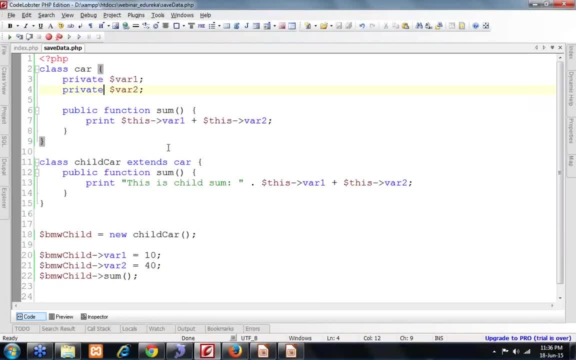 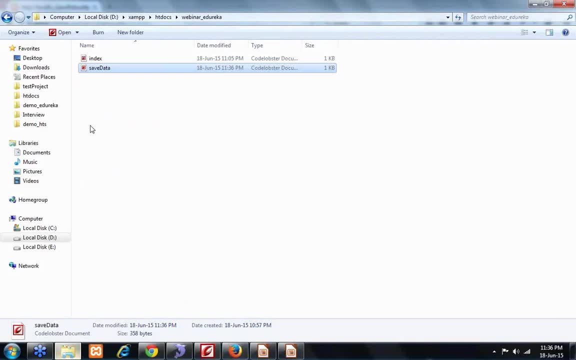 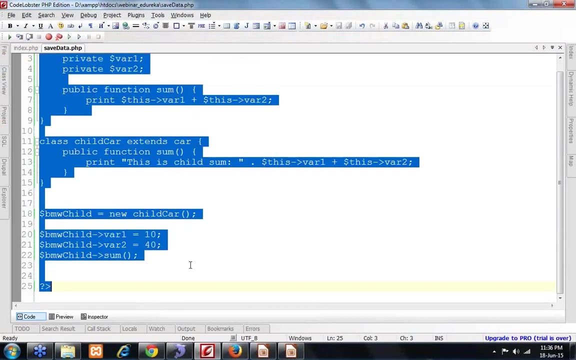 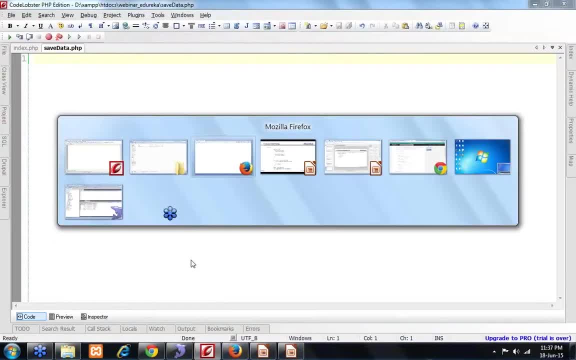 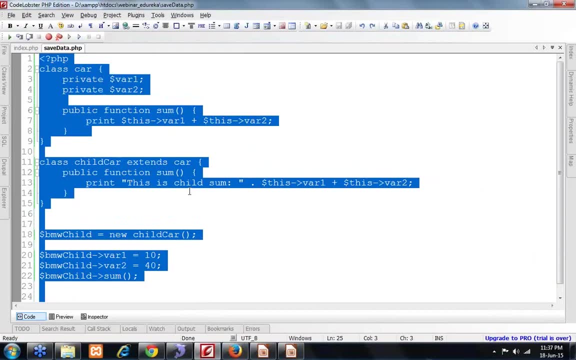 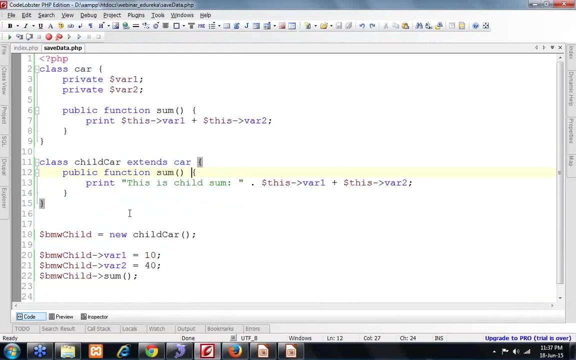 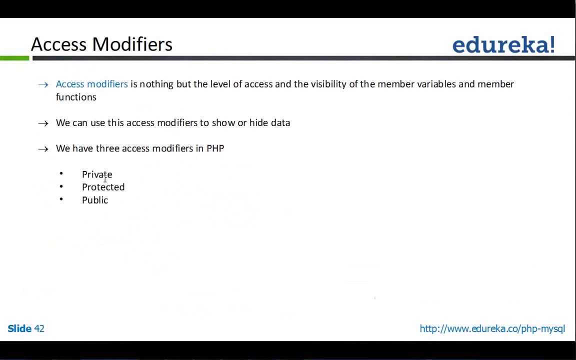 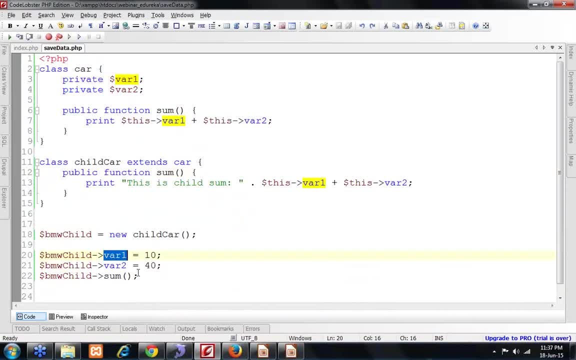 define it private, I won't be able to access it outside as I'm accessing if it is public. only then I will be able to. if it is protected, even then I won't be able to use it outside the class. I can use it inside my if I want to use inside. 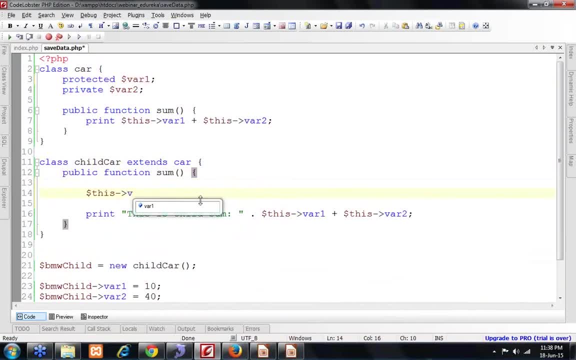 my child class $. this where one I will be able to. if it is protected, I will be able to use it inside the class, inside the child class, but not outside the class. if it is protected, if it is private, I will be able to use it inside the class. 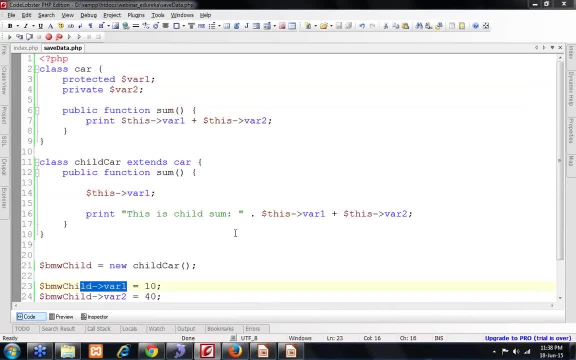 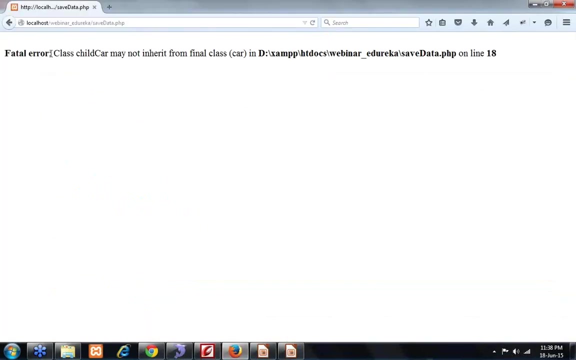 only not outside the class like this. so these are called private, public and protected access modifiers. yes, it is present. so final keyword simply means that if I put final keyword in front of some class, that class can can. now we cannot inherit that class here. if I put 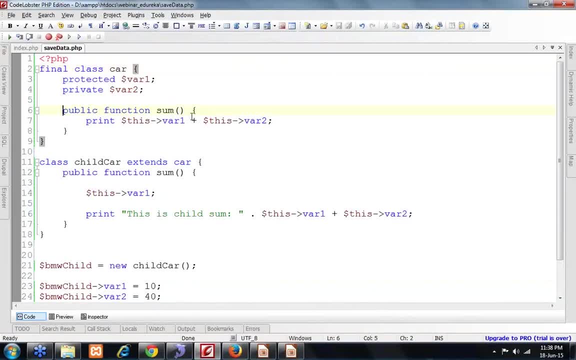 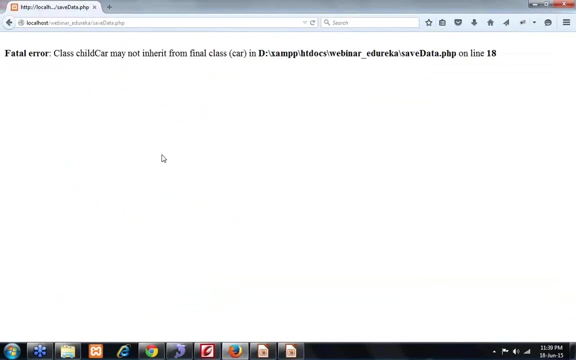 final in front of a class, or if I write final in front of a function, that function we cannot overwrite. and if I write final in front of a class, that class cannot be inherited now. so the class, child class, may not inherit from final class that is gone, fatal. 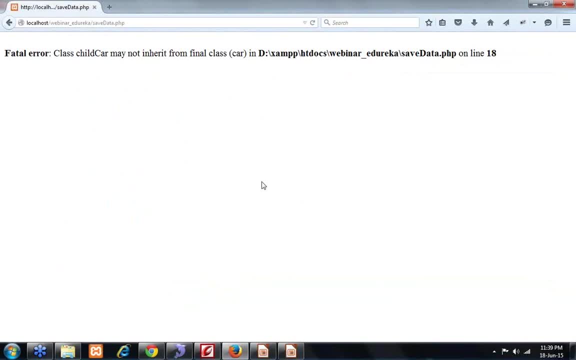 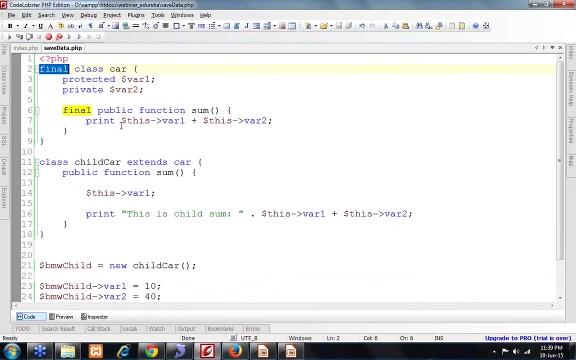 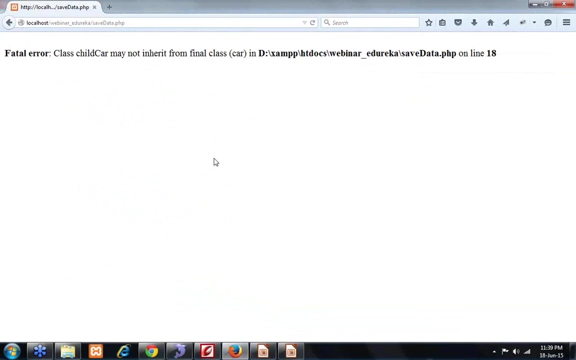 error means there is some error in PHP. you can say syntax, your syntax is wrong, or Logic is wrong, You cannot do it logically. That is called fatal error. So if I put final, that particular class can now not be inherited. Yes, VHP doesn't multiple inheritance. It uses interfaces that Java uses. 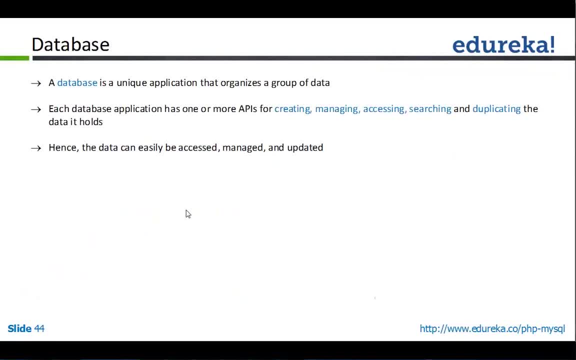 So this is the use of final keyword. So a database. database, you can see, is a unique application. Just give me a moment please Now. inheritance concept is same in PHP, So as of Java, so now I'll be looking into database. 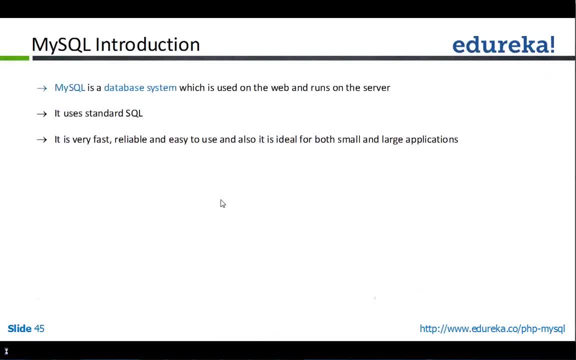 Database is a unique application that stores data basically. So MySQL is a database system that can run on multiple servers. It uses simple PHP SQL queries to execute and it is reliable and can be used for any size of application. So, using PHP. now we can connect to MySQL server using PHP. 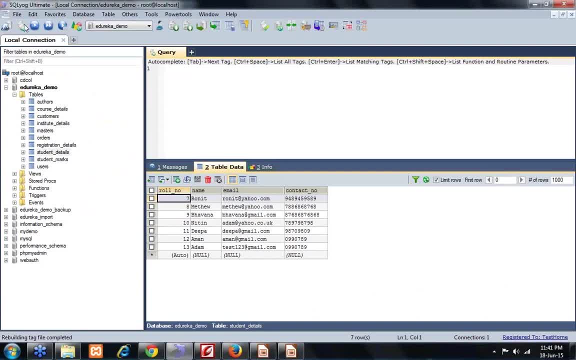 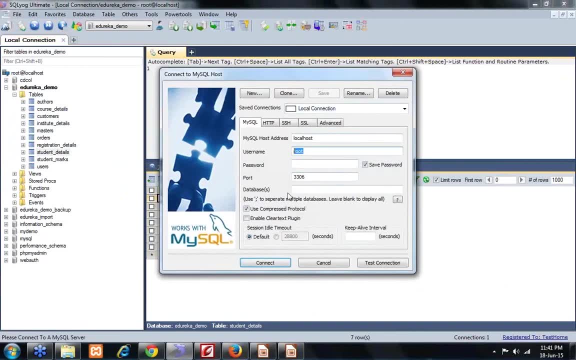 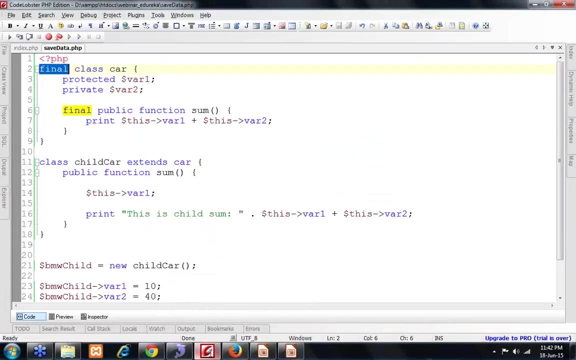 So this is MySQL server. So this is the MySQL server. username and password is blank in my case. Now, here I'm connected to MySQL server, but now how I can connect to MySQL server using PHP, that I will see. that we'll see here. 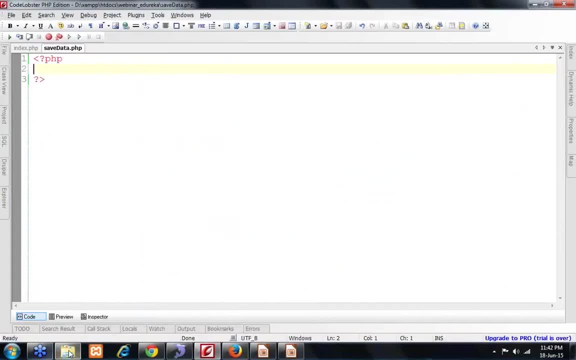 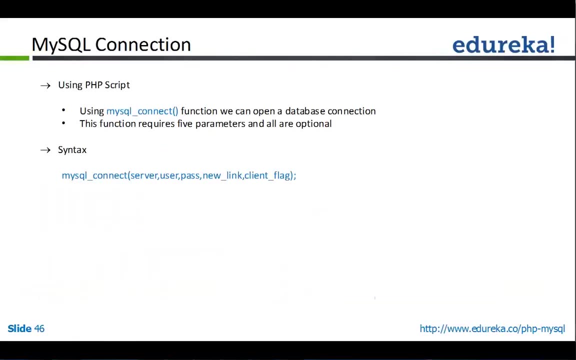 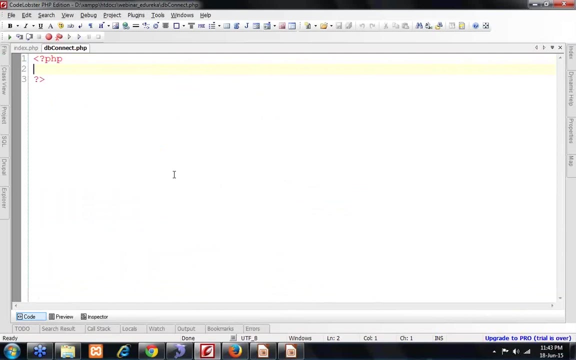 So. So here we'll see that how we can connect to MySQL server using PHP. So for connection I need three things. One is your host, So in our case it is localhost. as I already explained, your localhost Then it would be username. 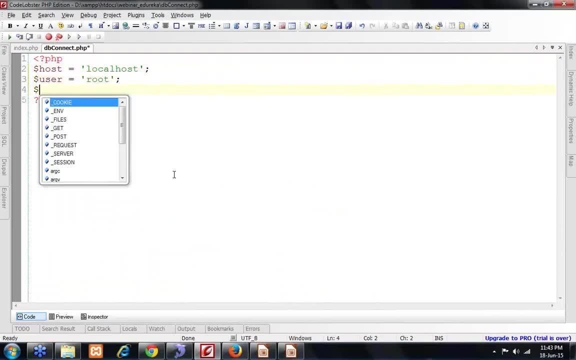 So in my case username would be root and dollar password. So that is blank in my case. Now I can connect to MySQL server by MySQL underscore connect function. I'll be passing host, Then I'll be passing username and then I'll be passing password. 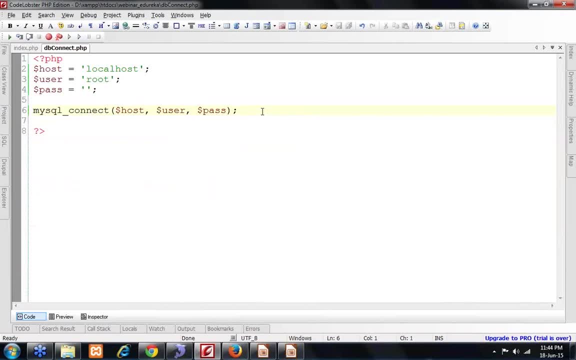 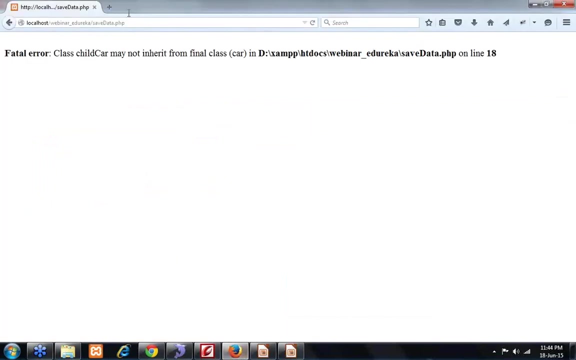 So Now my connection got created. Now how I will check my connection got created or not, I'll be creating this very connection in, You can say, a resource kind of resource variable. Now, if I print this DB, connect dot PHP. 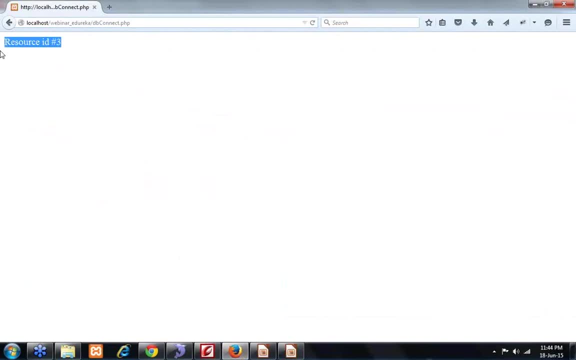 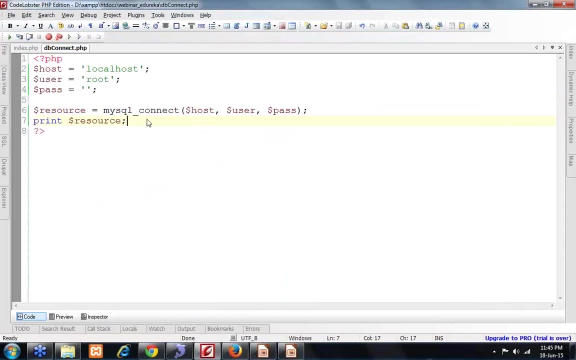 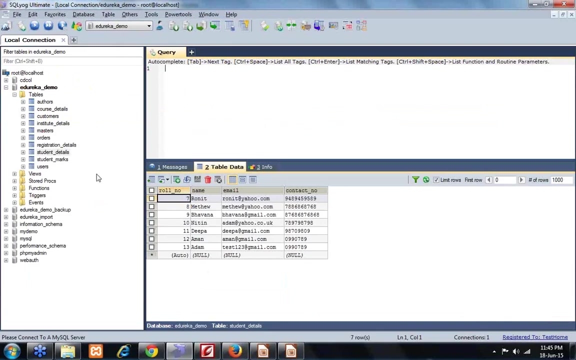 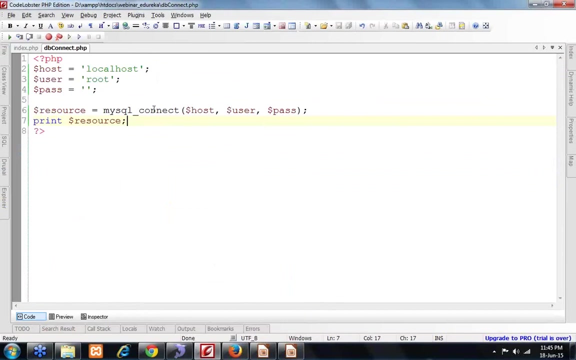 Resource ID 3.. It simply means that my connection got created. Now I'm connected to MySQL server using PHP. So here I'm connected to MySQL server using a client that is SQL yoga I'm using here. but I can also connect to MySQL server using PHP with a function called MySQL and connect. 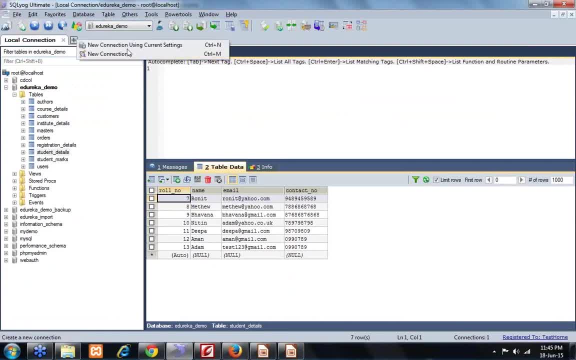 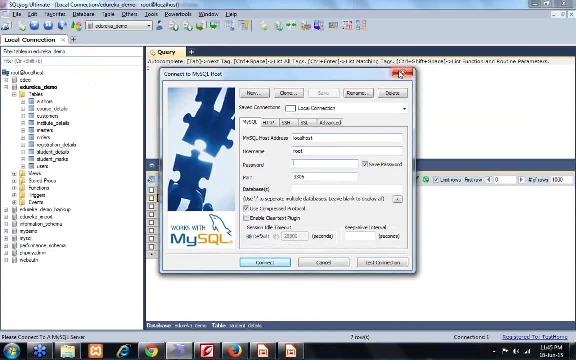 So three things are required. If you even connect from the this interface, you can see three things are there: Hosts, username and password, which are mandatory in order to log in to your MySQL server. So host in my case is localhost and user is root and password is blank. 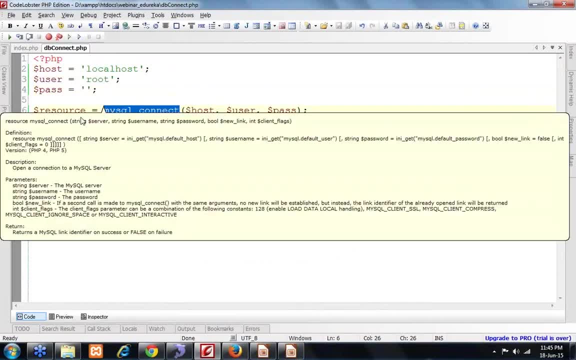 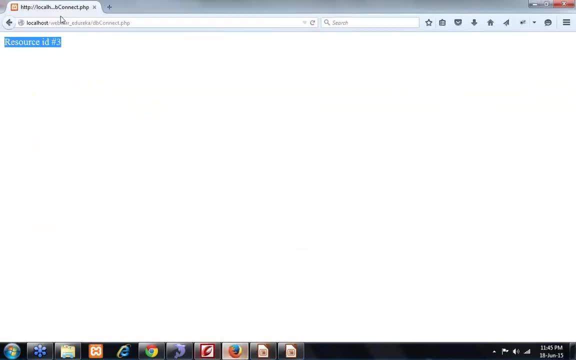 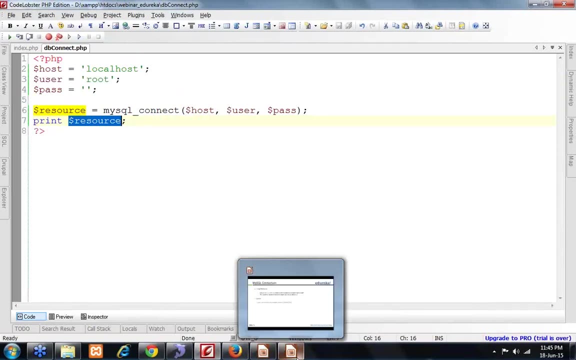 So I will simply pass all these values to my school to connect function and I will save it in a variable. That is a resource variable and resource value. But when you print this resource variable I can see resource ID. So this simply means that if resource ID is printed, simply means that my connection got created with MySQL. 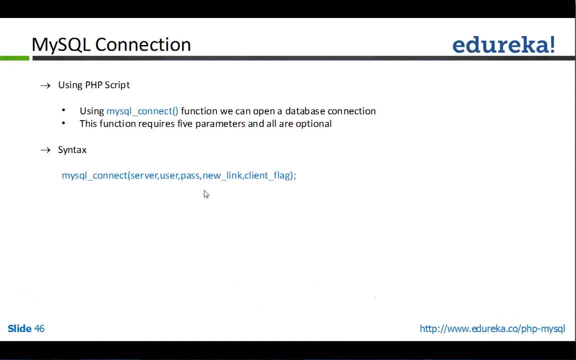 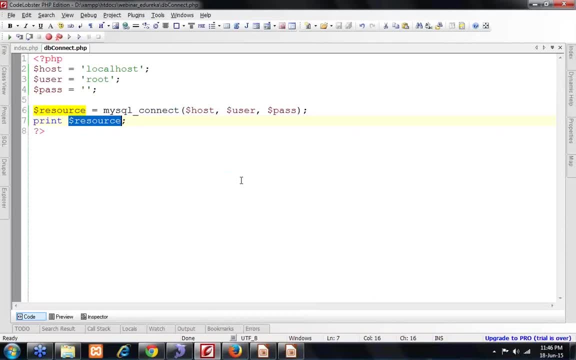 And PHP now, by a PHP, has connected to MySQL server, So we can have two other parameters. that is, new link, client flag to new link means that every time, if I put this value, one every time, it will create a new connection If I pass this value as zero. fourth argument: if I pass it as zero, it will see if an existing concept connection is there. 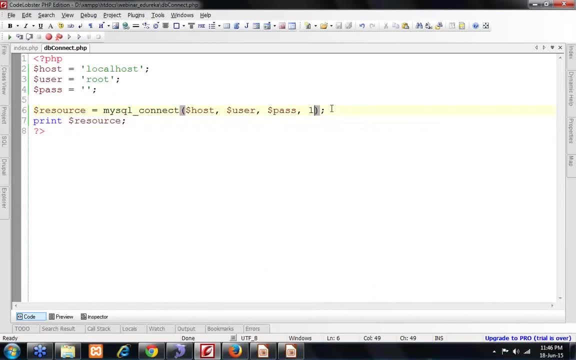 It will use that connection. if I pass it one every time, it will create a new connection with MySQL. This is the difference. And client flag means if it is a secure connection, it would be one. if non-secure than zero mean STTP. 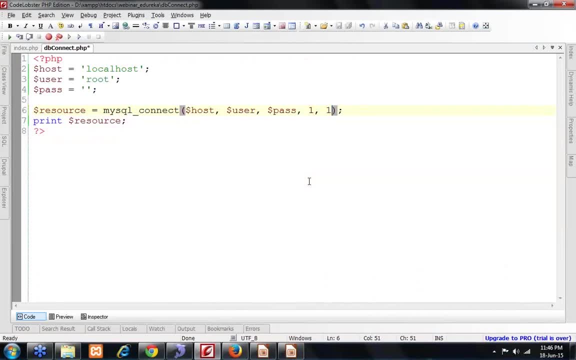 It would. it can pass be passed as zero. if STTPS, it will pass as one. Now we have created the connection the same way. Once we have done with our connection, We will be closing up the connection, MySQL underscore close And we will be passing up the resource type for which we created the connection. 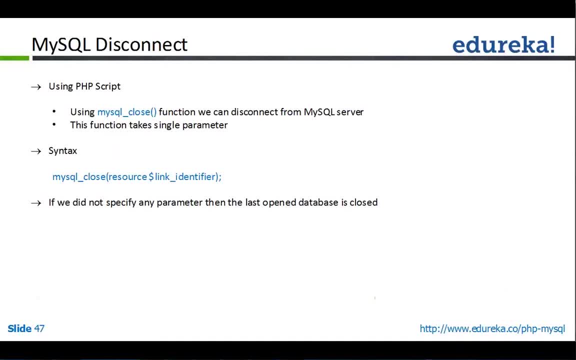 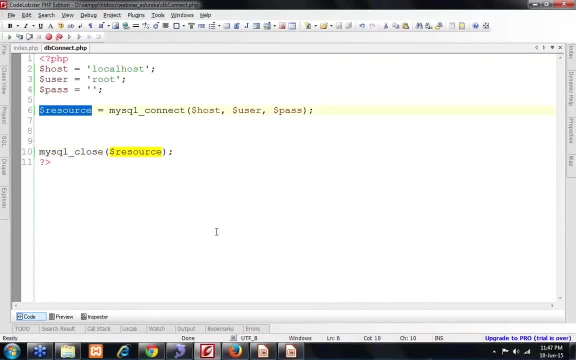 Now this will close the MySQL connection. So the syntax is: MySQL underscore close and your source link identifier means this resource that you created. that was the reference, That was the pointer for the connection. use that pointer, use that reference to Close the connection. 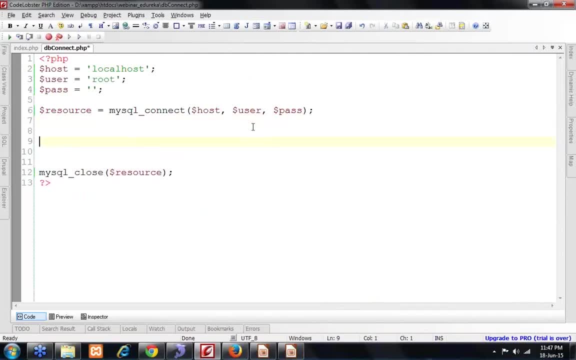 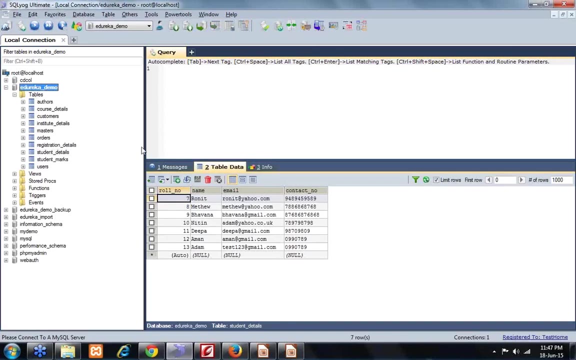 In order to run a query in PHP. I've connected now you in order to run a query like I want to select something. So first of all I will have to select a database, Like if I'm going to use MySQL, I have to select a database here. 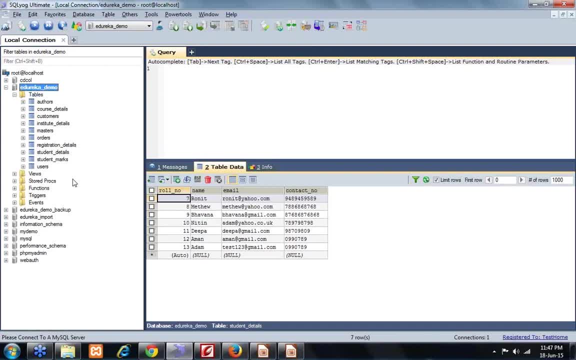 I've selected that. you're a contest for demo, So it is bold here. You can see it: You're a contest for demo, selected. Now, if I do, if I take a table like student details, If I do select star from or select star from. 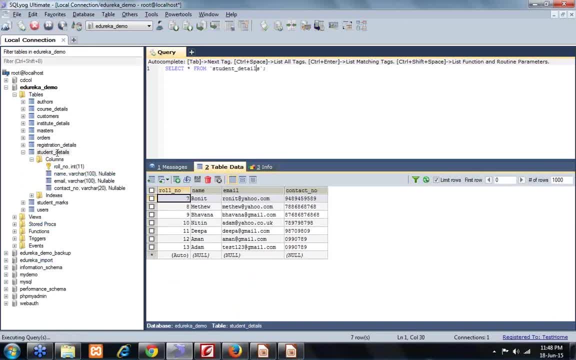 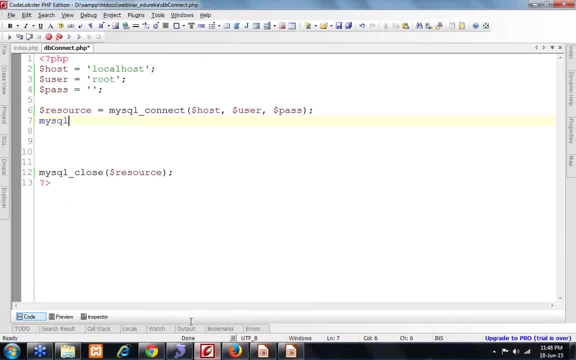 Student details. Here is the list. You got all the records into student details. Now, the same thing you can do with PHP. So, in order to do it, I will be first selecting the delete database, that which database I want to use- The function name is my school- and, of course, select underscore DB that I will be using to select a database. 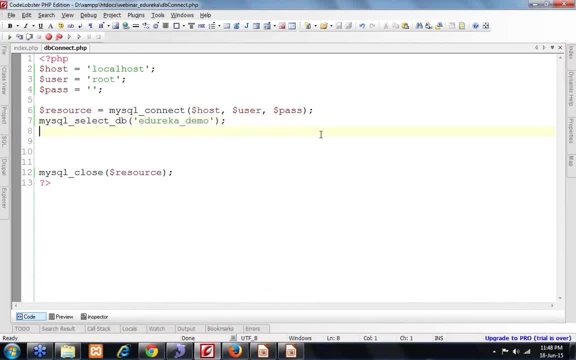 Then I will be giving azureka underscore demo. Otherwise is MySQL server will not get to know that. which database to use. There can be multiple databases on a MySQL server. I will be giving my second to select underscore DB Function and then value the database name that I want to use. 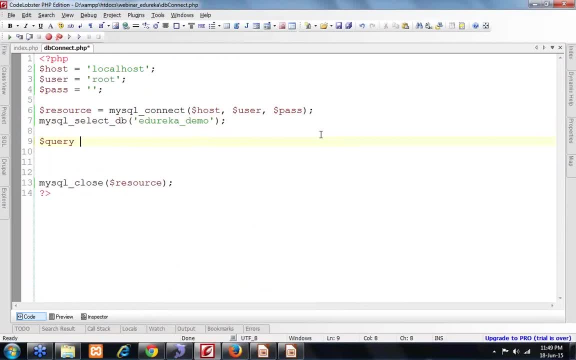 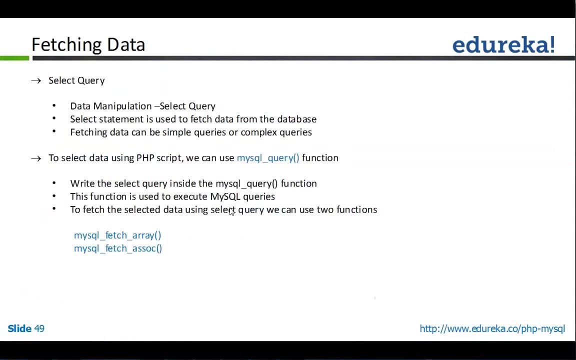 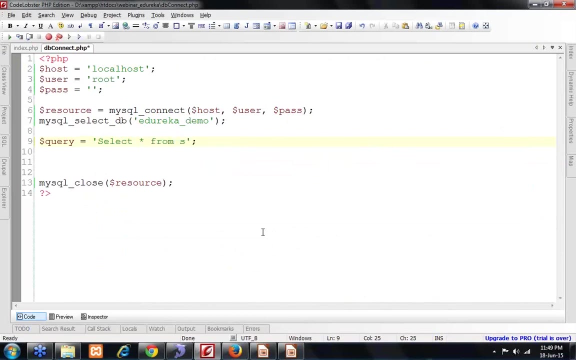 Then I will be writing my query Select Star from Student details. Now I'll be using dollar Data Or I will say object data: OBJ data Is equal to. I'll be using a function called my secret underscore query and I'll be passing my query to this function. 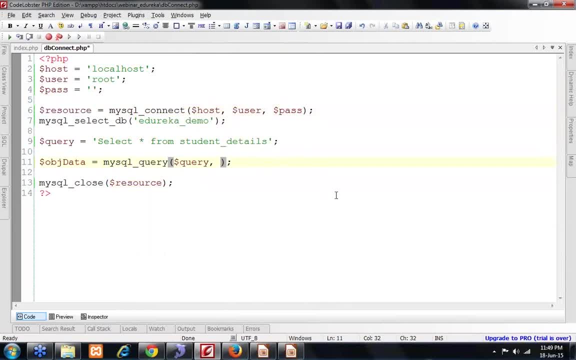 With the resource identifier that I created, so it will let me know that for Which resource, which MySQL connection I'm running this query. So my school does not query- then query and then resource data type. Now, If you print this, You will see resource ID again, because this is returning a resource, but like it is returning a packet. 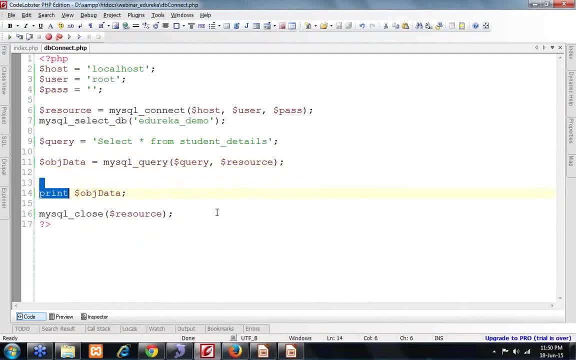 Now we have to unpack it To get the values Soon PHP. There is a function. We use the while loop to fetch all the records from the table. We do dollar row because I will be fetching each and every row. So there is a function in PHP called MySQL underscore. 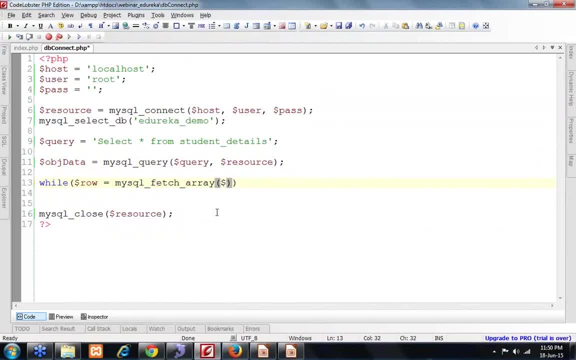 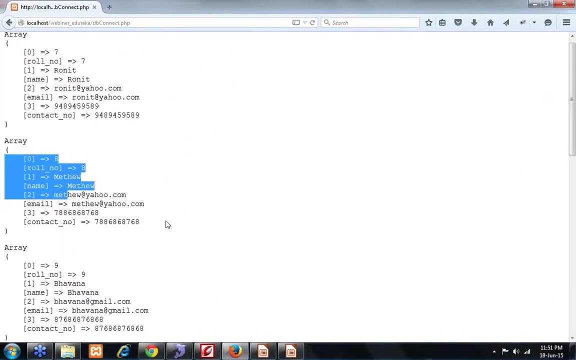 Fetch underscore array And I'll be passing My object resource to that and I'll be printing. I'll print each and every row now. I will do print underscore R: Dollar Row. Now you can see I got values of my data from the database. 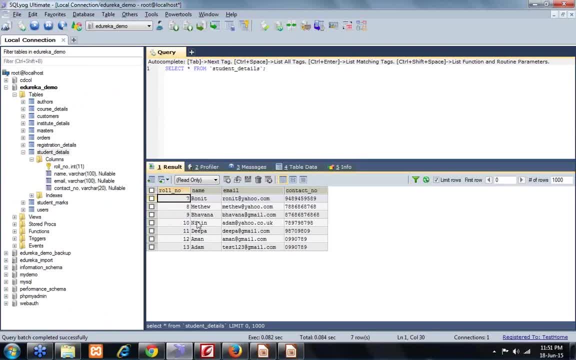 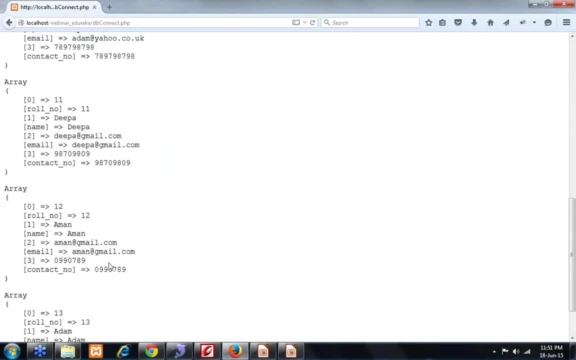 I mean I'm having these two, these much of records: 1, 2, 3, 4, 5, 6, 7 records. I got 1, 2, 3. 4 and then 5 and then 6 and then 7 records. 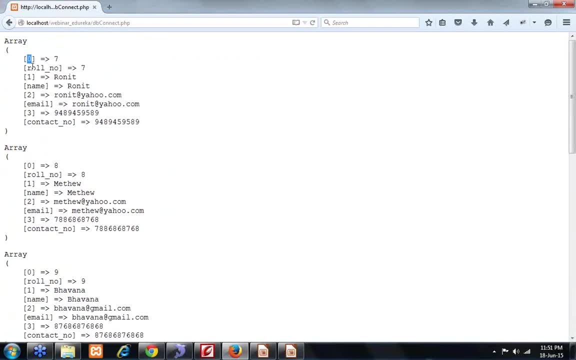 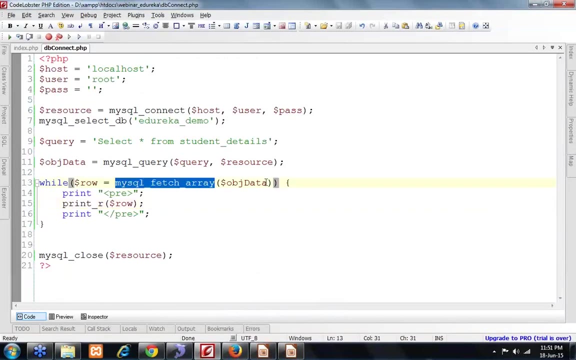 Now you can see. I got both the subscript 0 and then roll number 1 and name 2 and email. So both are have duplicated, one with the numeric key and one with the associative key. So data would be returned in this way if we are using MySQL fetch array. 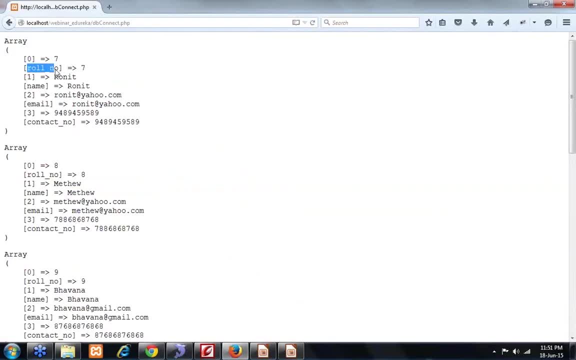 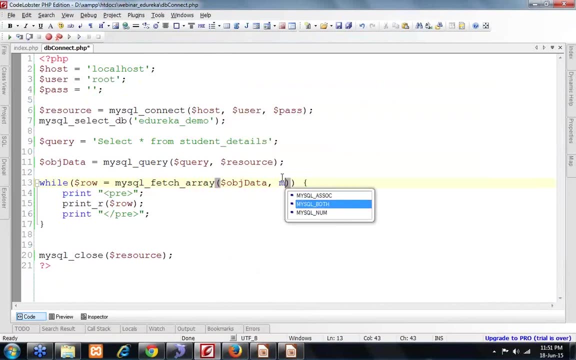 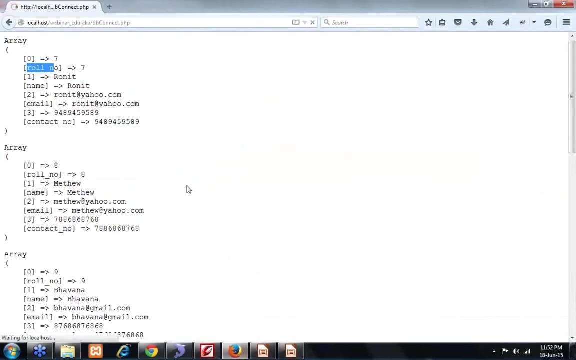 So in order to restrict it to either Value or associative value, We have to pass a second argument to this function, That is, MySQL underscore. if I want to only associative array, I'll be passing MySQL underscore, Ashok, So this will give me only associated. 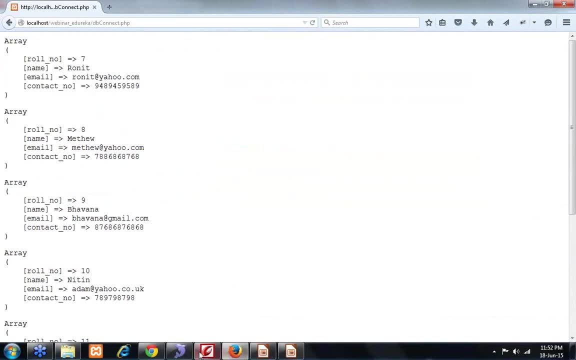 So this roll number, name, email are the column names in the database. You can see roll underscore number, name, email and contact underscore number. So these are the Column names. now, if I want only the numeric keys, note the associative keys. So I'll be passing MySQL underscore num instead of MySQL underscore underscore Ashok. 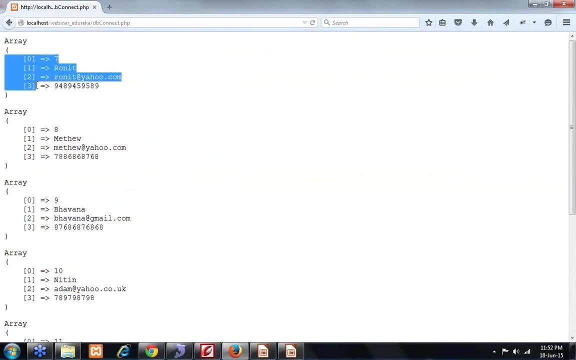 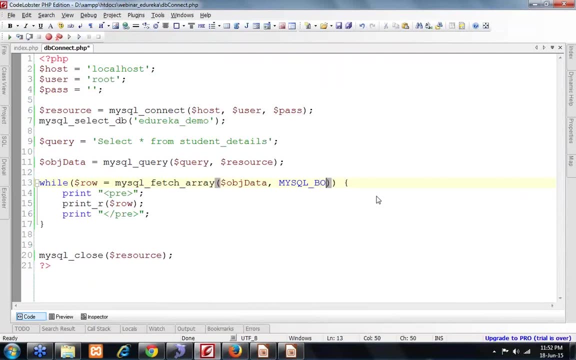 So I'll be getting, instead of key names, I will be getting numbers for the keys: 0, 1, 2, 3, subscripts Or it, if I want both. so I can either remove or I can pass one more argument That is called MySQL underscore- both now. 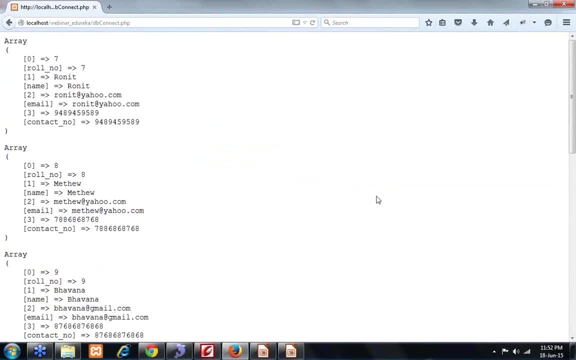 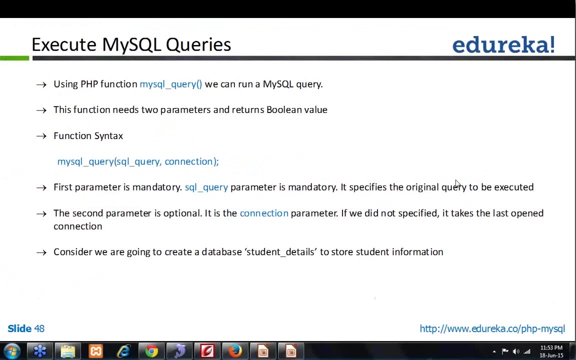 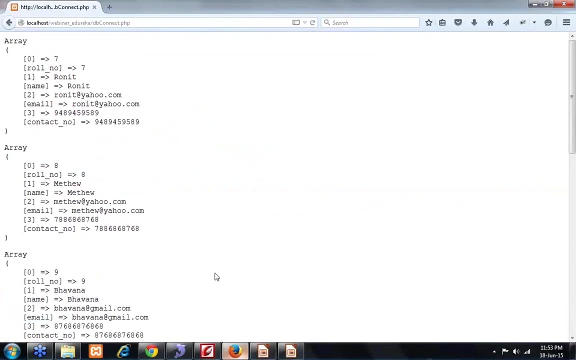 It will return me both Numeric is and associative keys. If I remove it, it will do the same same job. So this is how MySQL query is used to fetch any query and MySQL fetch Underscore array is used to fetch the data. 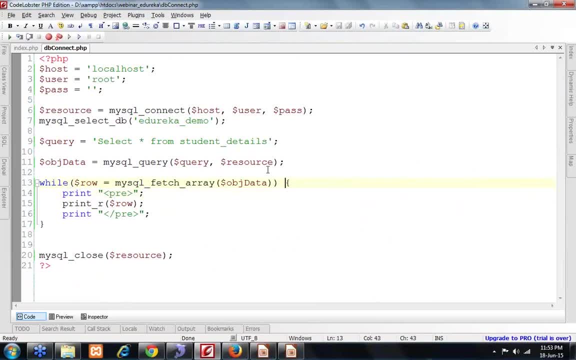 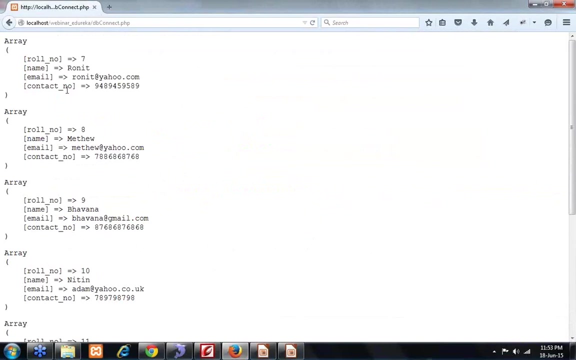 So if I want to fetch only associative array. so two ways are there: one to pass MySQL underscore Ashok, and another way is there is one more function That is called MySQL underscore. fetch underscore Ashok. Now it will do the same job- job as passing the second argument as MySQL underscore Ashok. 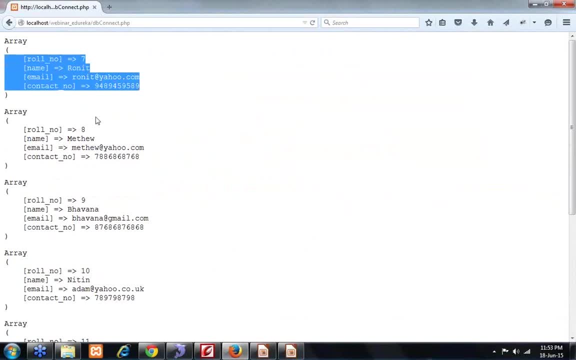 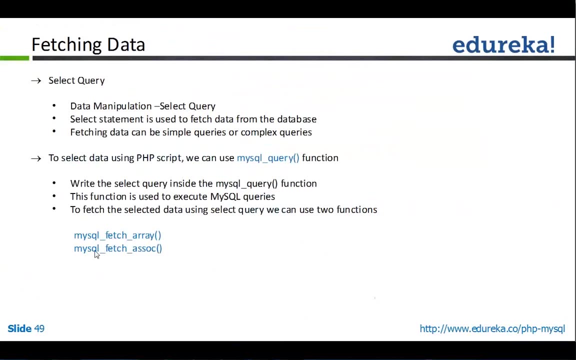 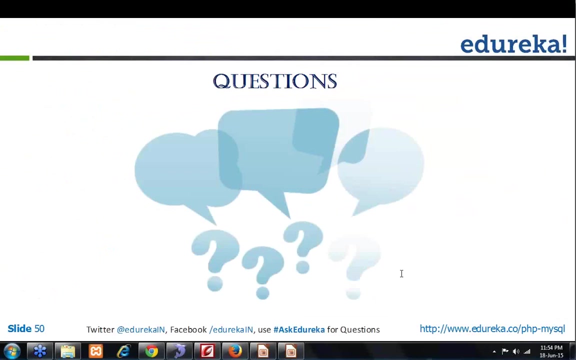 So it will return all the records in associative arrays From the database. So two function: fetch underscore array and MySQL. So these two can be used to fetch data from the database. So that's all about today's session. Any query, any question you can ask, or you can later on contact with support and they will reply to you. 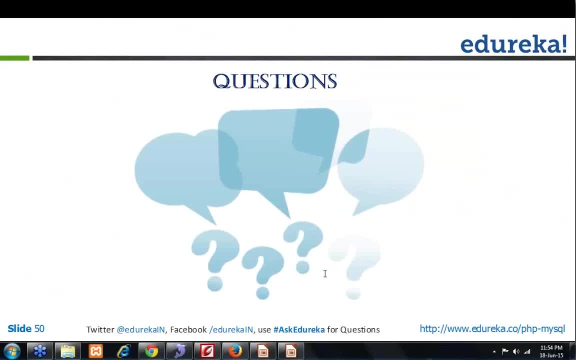 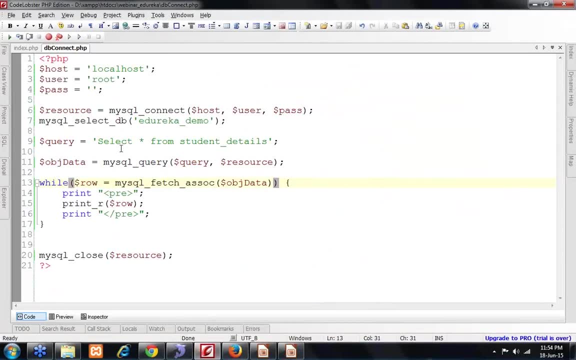 So this was how I think. now your question of how PHP interacts with MySQL is clear, because you have seen that. how I can run here, I'm running select query, Using the query and fetching all the data and printing it on the screen using printer and score our PHP method. 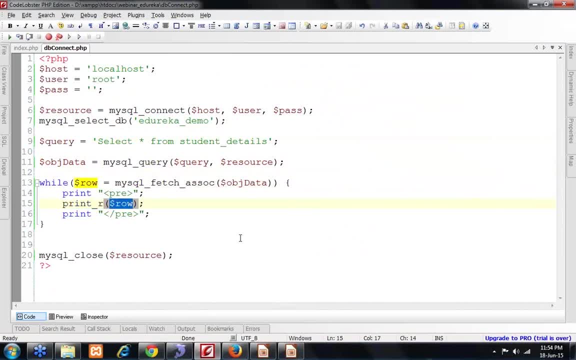 I go to the array of the data. Okay, by the new question: MySQL underscore, MySQL underscore underscore I and versus PDU. So PDU again can be used with PHP. That is not an issue. MySQL I is upgraded version of MySQL. It is. 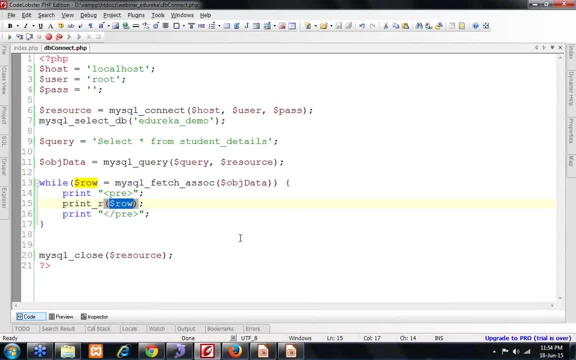 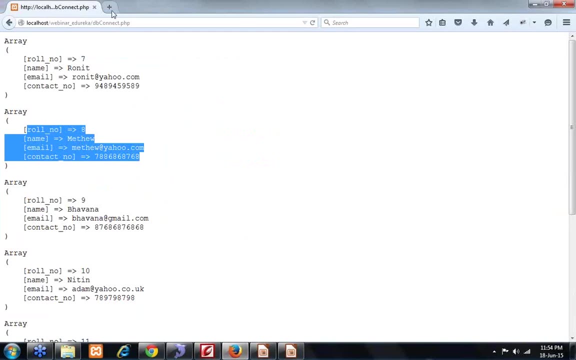 It is, You can say, bit more flexible It is. It is more flexible than MySQL and, moreover, It is object-oriented. PHP MyAdmin- see, here I'm using SQL Yoke. You can use PHP MyAdmin as well. Let me show you what PHP MyAdmin means. 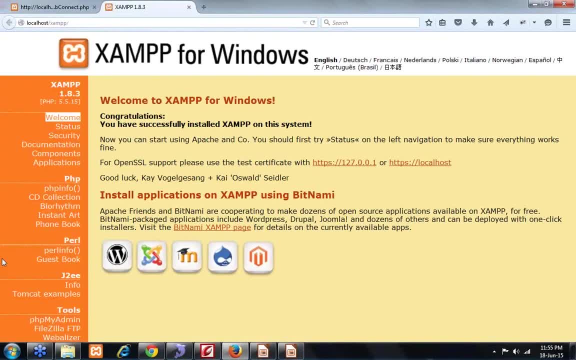 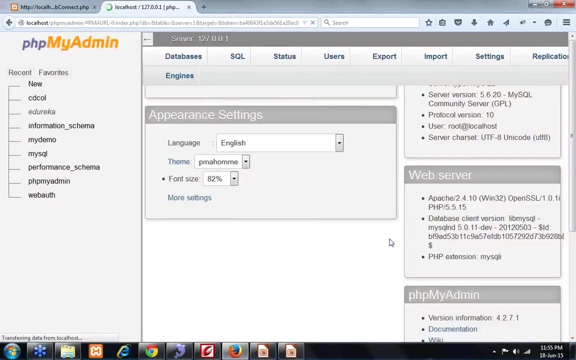 It is nothing, but it is a MySQL client. when you install Zemp, write localhost, You will get here PHP, MyAdmin, Drupal. if you are going to develop a secure site, like if you are going to work on some secure banking information or kind of financial information or kind of shopping cart. 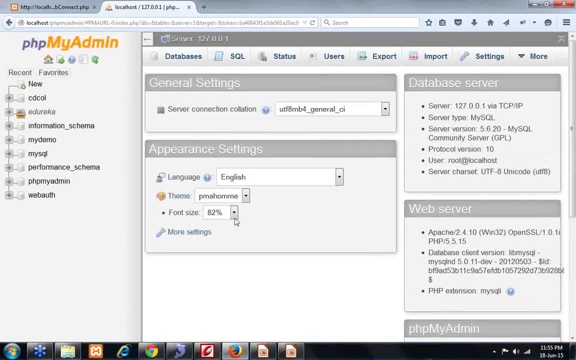 Then you should go with the HTTPS and you can purchase the HTTP certificate then. So here the same thing. you can see. I can access my database, That is, Azure underscore demo, Azure underscore import. Same way I can access in this SQL Yoke. 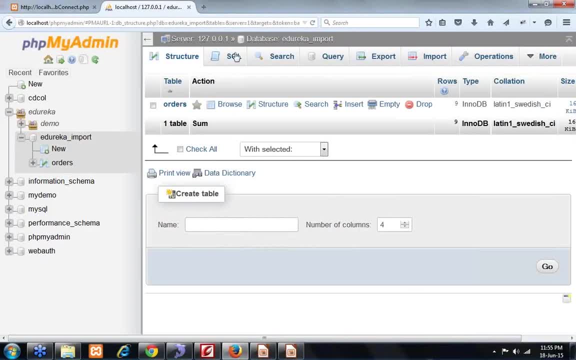 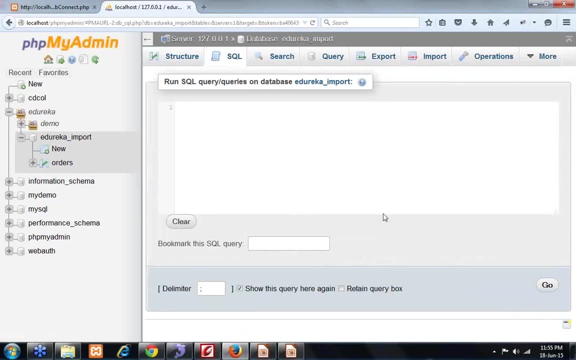 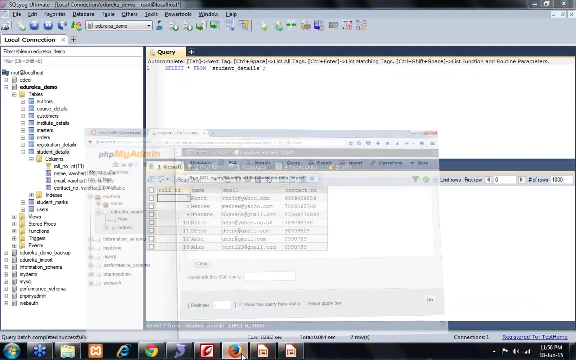 So it is nothing but the client to access your database. So, using SQL, you can write your query, You can import, export your data, You can search your data. A lot of things you can do you using PHP MyAdmin. So the thing is that once you have created your site, like on your local system, using this, like this, have coded: 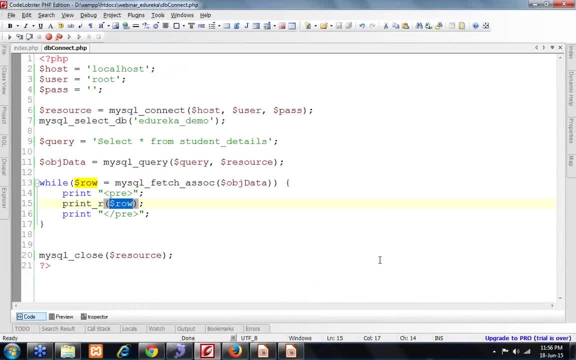 You can simply upload your code to the server. Right now we are not going to cover more MySQL, But yes, if you are going to do the complete PHP course from Azure, you will be getting MySQL in more details. PHP and MySQL in more details. 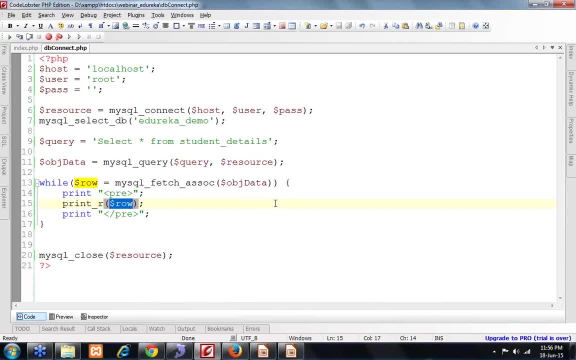 Oracle workbench is different, Ashish. there is one more called MySQL workbench That is similar to Oracle workbench but that works with MySQL. You can use that MySQL workbench. PHP doesn't build the mobile apps. It acts as a backend for mobile apps. 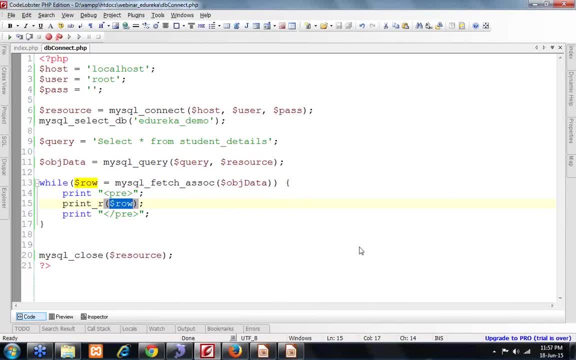 Yes, Raj, there is lot of career scope in PHP, Because PHP is the best web programming language these days And it is now extending day by day. More and more modules are being added to PHP, More and more frameworks are built in PHP. That is more secure and fast. 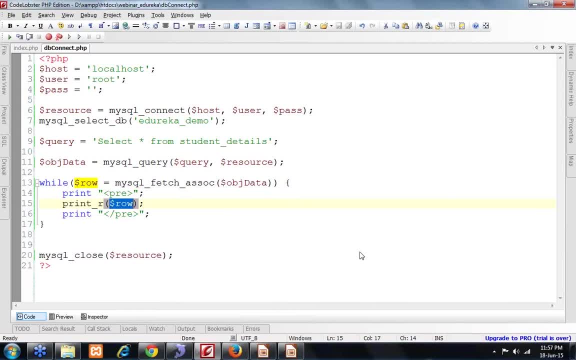 I have spent 11 years in PHP and still working in PHP, So there is There are very good chances of employment in PHP. This is not an issue, Because you not only learn PHP when you work as a PHP developer. You learn lot of things, including PHP. 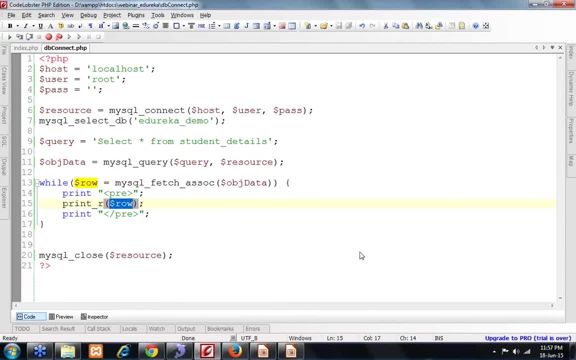 You learn PHP, You learn HTML, You learn JavaScript, JQuery, Lot of things. Definitely it will help you to build web programming career. Definitely it will do. See, PHP alone is not used. PHP, MySQL are basically used together, But you can also learn JavaScript, JQuery, JSON, etc. 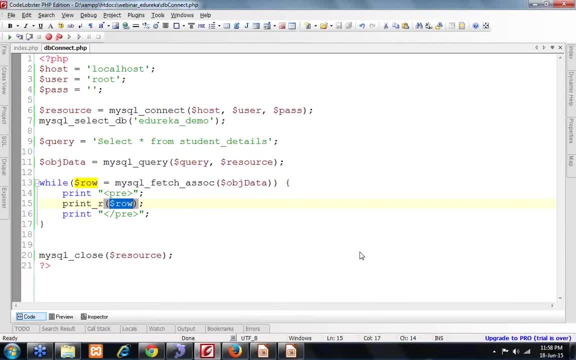 EdgeX, etc. If you want to build a career in PHP, Ok, then. If this is enough, Then we can just leave for now, And if you have any other question You can just put to support. Yes, You can upload videos. 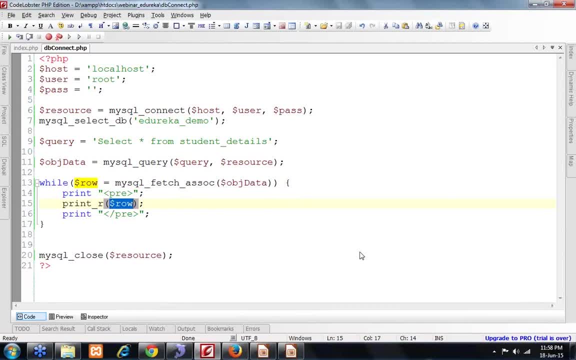 And you can download whatever you want to do, Everything you can do, Upload, Download Anything you can do with PHP. Thanks, Ovik. Thanks a lot. Actually, I had lot of things to explain But due to time shortage I was not able to explain everything. 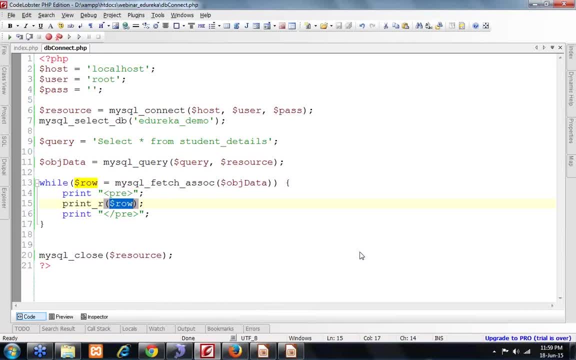 So it is very vast subject. You cannot complete it in three hours. It might take three months, Even if you discuss on it, But as limit of the time I won't be able to explain much. Ok, Thank you, Bye. 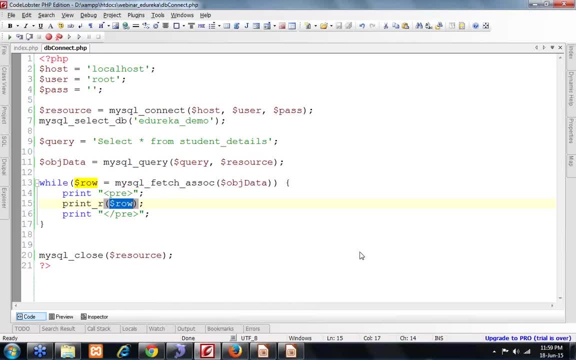 Bye, Bye, No problem, No problem at all. No problem, Rajah, I think you should contact Azureca. They will let you know how to reach me. Yes, I'm saving this video, Recording this video. You can, as Azureca to provide you this video. 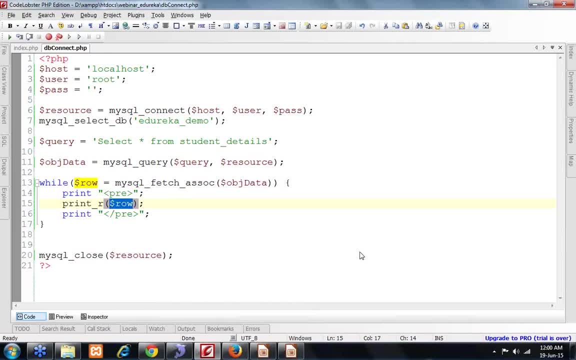 No issues. Ok, Thanks, folks, Thanks. Thanks a lot, Balik. thank you, thanks. thanks a lot. yeah, bye, take care. yes, Mitesh, mysql is the best choice. you can work with the Oracle, but mysql is the best choice because it provides functions. 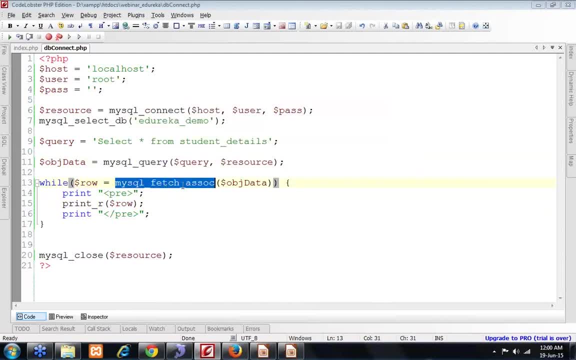 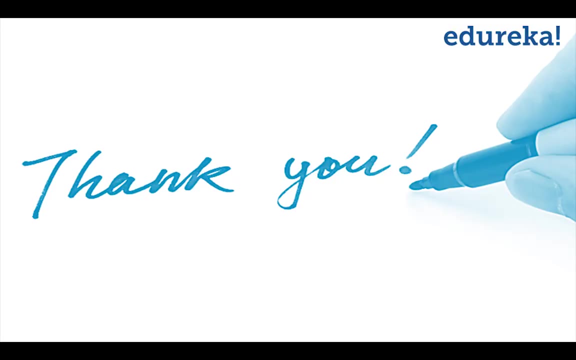 you have seen mysql query fetches, so, but it never provides functions like that for Oracle. yes, you can build a good website with PHP, okay then? okay, everybody, thanks, thanks a lot. okay, I'm going to end this session. If anything else, let me know, otherwise I will end this session. yeah, thanks, thanks, Mitesh. 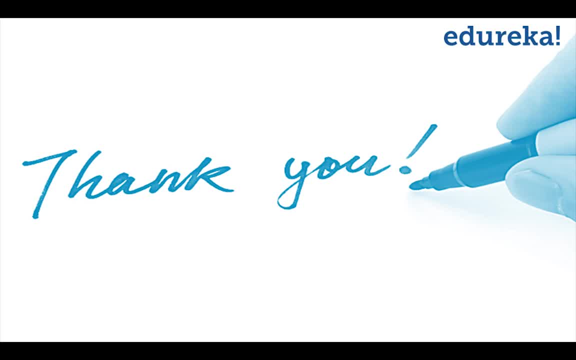 thanks, Shruthi. yeah, thank you, thanks. bye, take care. I think, Raj, you should get in contact with the Azureka. Thank you Same to you, Raj. you should contact Azureka. they will let you know about the next session. 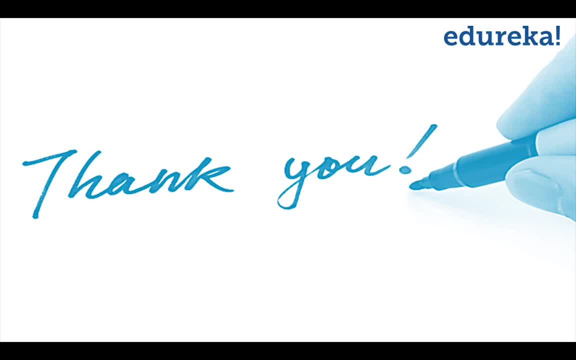 okay, thanks everybody. I'm ending this webinar. thanks for your time. can PHP record are doing in a website? what do you mean, Aditya? I'm not getting your question. actually, PHP provides every kind of functionality. a lot of modules are there in PHP. yes, okay, videos you want to download from Azureka or from? 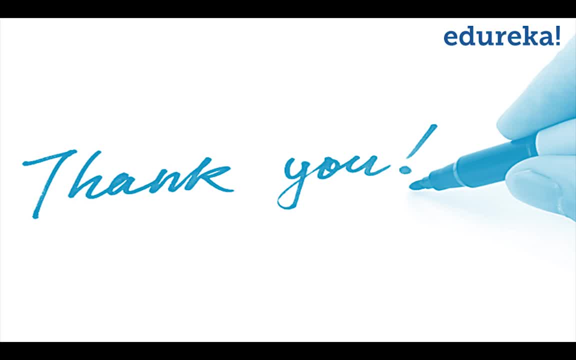 the Google. Okay, Okay, Okay, Okay, this video. you can talk to azurek and they will provide you. yes, they will provide you how to download this video, provide you the information. talk to the, they will help you out. definitely, they will help you out. 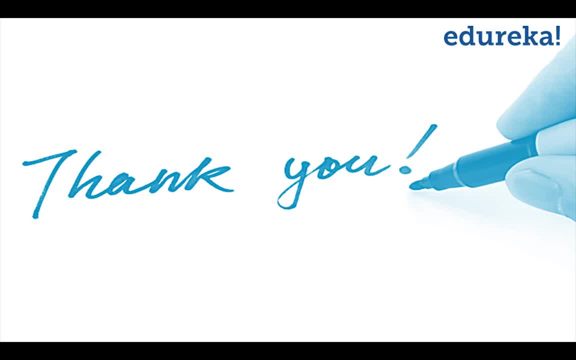 Mitesh, you contact azureka, they will let me know. if there is something you can, you can talk to me through azurek only. so talk to them and refer that you want to talk to me and they will. they will facilitate this thing. I will be able to.